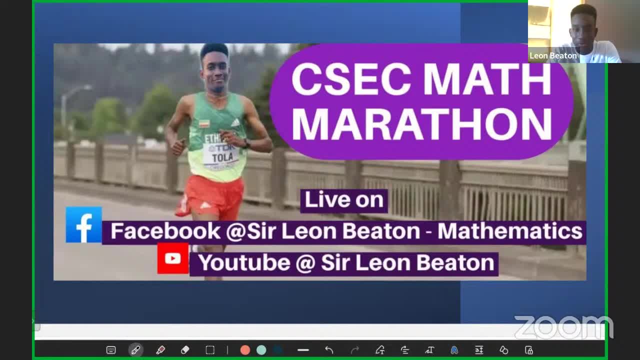 So, yeah, Yeah. So let's see how things will go. So we're live on YouTube as well, for those of you who would like to hop over to YouTube and look at it. Do we have for the NGSA, unfortunately. 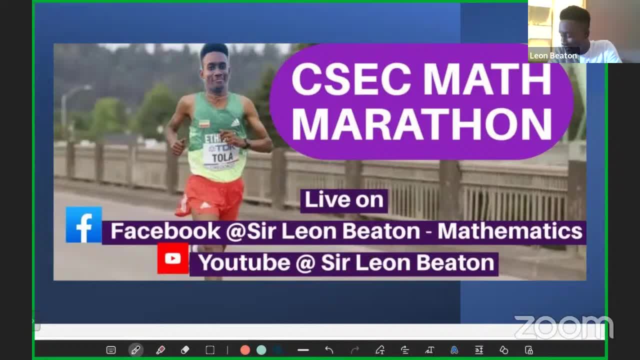 Ah, not this year, Probably next year. It's Sor Vela, on Paris, who is doing some lovely YouTube videos for NGSA, So yeah, I could check out. We're going to do it. I think his name is on YouTube is V-P-G-Y. 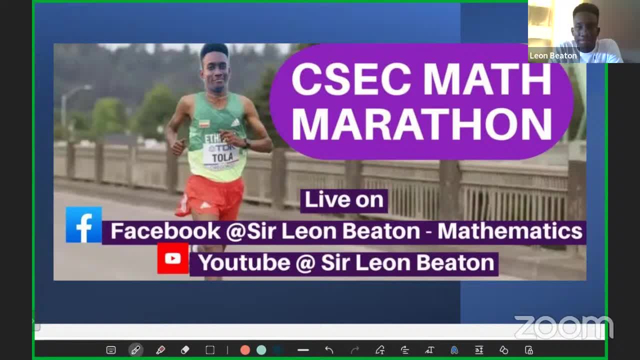 Yeah, All right. So I'm here with some of my students- A few of them, a very handful of them- who are bringing up to come live as well with me, So you will be hearing the voices of them as well throughout the live video. 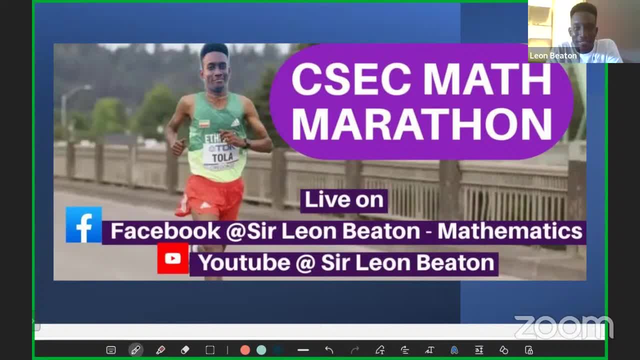 So a few of them, a very few, a handful, So you'll be hearing their voices throughout the video. All right, The purpose of this live is to, you know, get some practice. You never know how many of these questions, or type of these questions, you may come across in the exam. 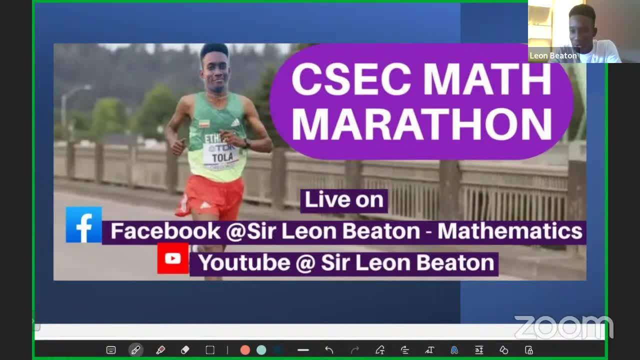 You know they say, oh, you saw us. or work this on Facebook live at the end you know you score, you got a mark to those questions. They never know that those marks that you get can determine if you get a passing grade or a failing grade. 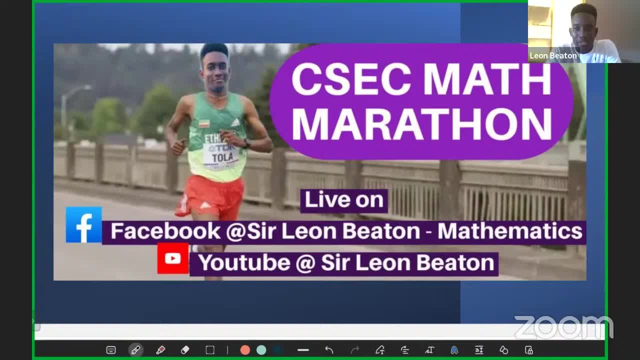 So yeah, So let's go. So this live will take two parts. I'll be working with some people- two kind of questions- and some people. people want questions, people want type of questions. I should say All right. 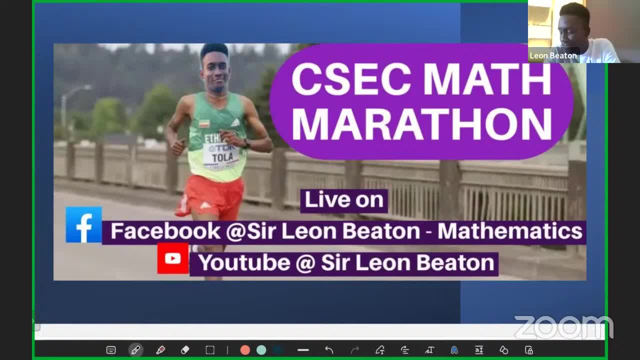 So let's head straight into it. So as you come on, you can probably share the live so that other people can benefit. I know we have at least nine, but here we are All right, So let's go. 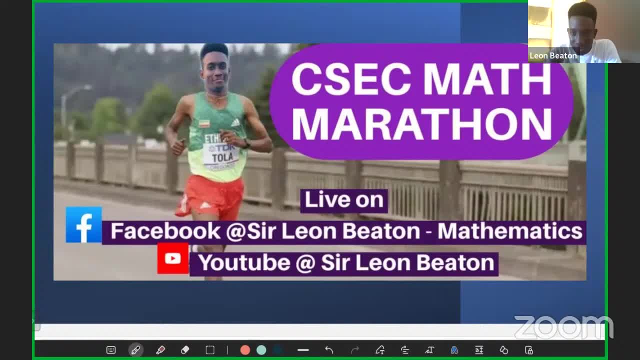 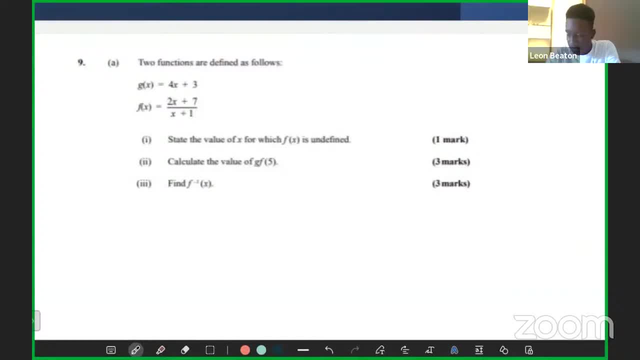 So the first thing you want to look at, let's go So. this question says functions. I think functions is a favorite for many students. It's because it's very simple. So let's see. The question says two functions are defined as follows. 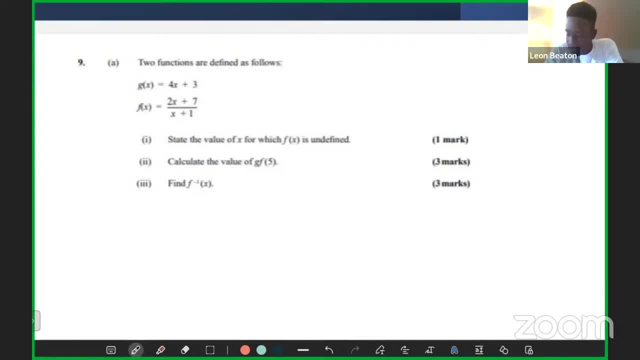 And we have g of x equal to 4x plus 3.. And f of x is equal to 2x plus 7, all divided by x plus 1.. And the fourth one: It says the value of x, for which f of x is undefined. so i have some of my students here um, they're on. 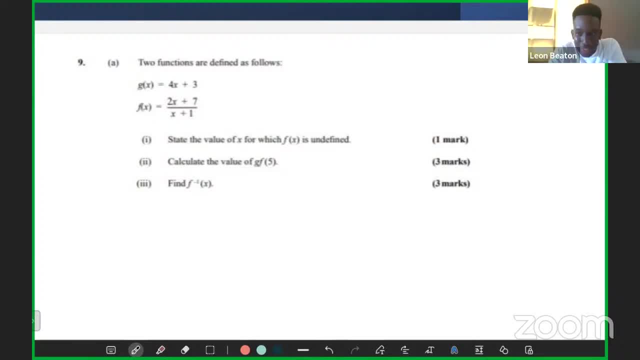 the live as well. they're on with me. so anybody um, let me just throw it out to you- state the value of f of x for which f of x is defined. can anybody remember when f of x would be undefined? sorry, when a determinant is zero determinant, you're sure the determines you weren't looking. 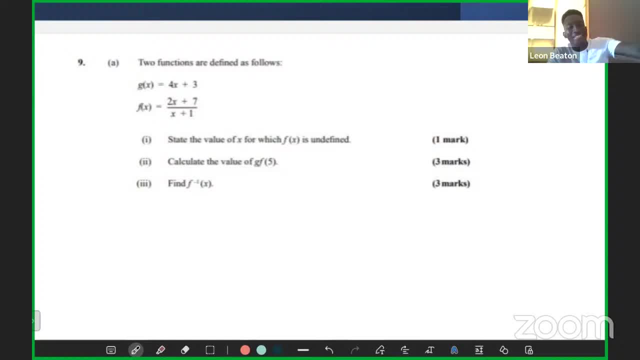 for sorry, sorry, now you determine the denominator. denominator: excellent when the denominator is equal to zero, um, that is when it is undefined. excellent, excellent, lovely, so, um. so the fourth one, so we have f of f of x is equal to 2x plus 7, all divided by x plus 1, and larry said it's undefined when the denominator 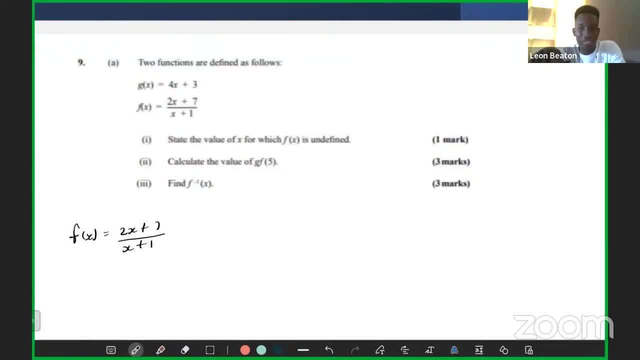 is equal to zero. so there is: how can we um find when the denominator is equal to zero? what can we do to the denominator part of the function? so we solve x, solve x, and we equate it to what zero, equal to zero. since we want to find when. 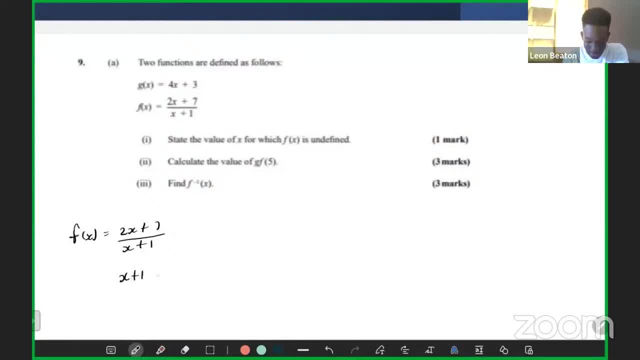 it's equal to zero. so this will be x plus 1. x plus 1, uh is equal to zero. and then we, you know, solve x, so x will be equal to uh. this is the one is adding. we think double subtract to zero. subtract one will be negative one. so the value of x for 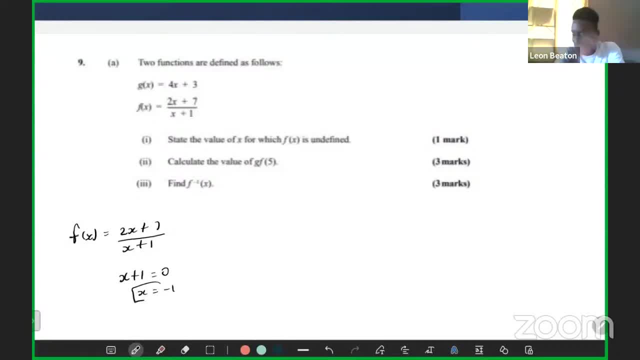 which f of x is undefined is x is equal to negative one. that's right, and that goes for one one, and this goes to any um fractional function. uh, if you want to find when f of x is undefined, uh, it must be equal to zero. um a function is undefined when you have it in this form. let's say: 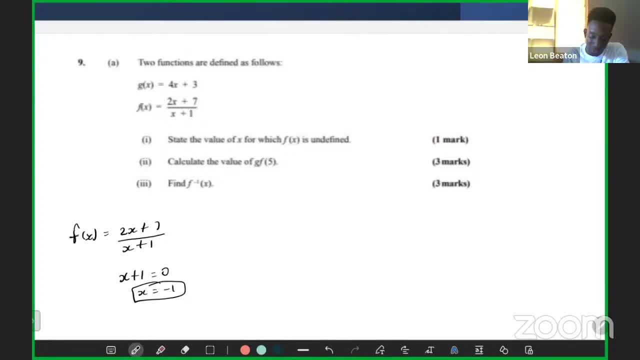 two over zero. this is undefined because the denominator is equal to zero. so to find when this is undefined, we have to equate it to zero and solve x, and i'll give you the value of x, for which f of x is undefined. well done, held on the race. so next one, uh, calculate the value of g of f. 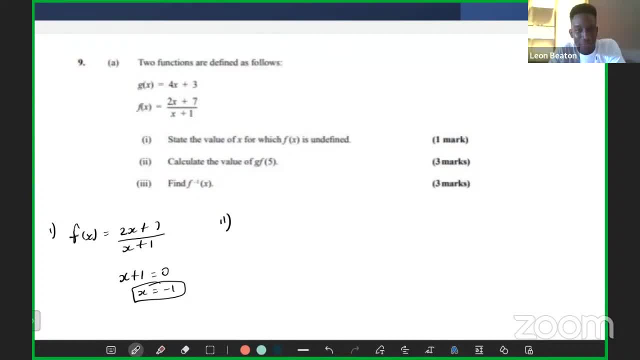 of five, the g of f of five. uh is a tight one, so we have a composite function there. um, we have a composite function, uh. so what we need to do, we need to take f of five and we put it inside the g function. all right, so we have composite functions. 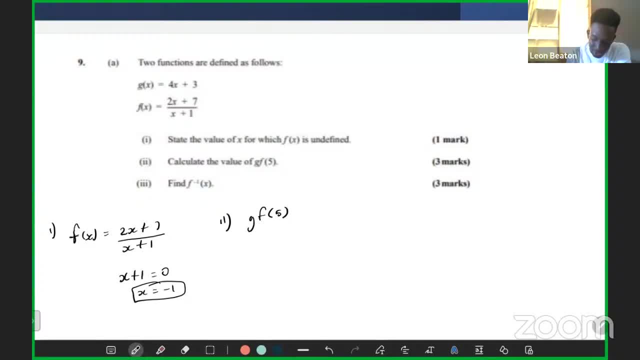 for example, g, f of five. you're taking a function- f of five- and you're putting it inside the g function. so a nice thing to do is to find what is the value of f of five, and then you take that value and you're putting it inside the g function. 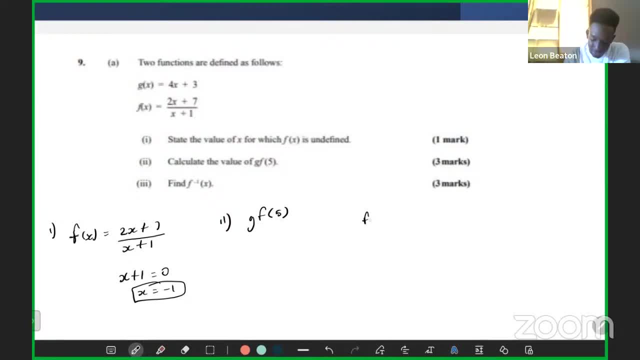 all right, so we can find for f of five. uh, f of five. all right, so we can find for f of five. so f of five would be: you're putting five inside of the f function, so this would be two x instead of x will be two times five plus seven, all divided by x plus one, and we 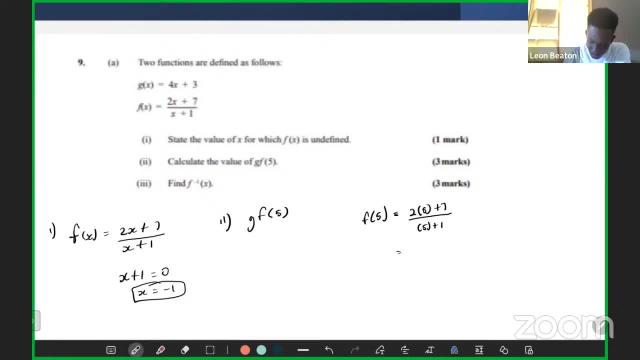 know, x is five, so five plus one, so two five is ten. ten plus seven. all divided by five plus one is six, so ten plus seven would be ten plus seven would be seventeen over six. so this question is going for three marks, so 17 over six. so we gotta find gf of 17 over g, of 17 over six, because 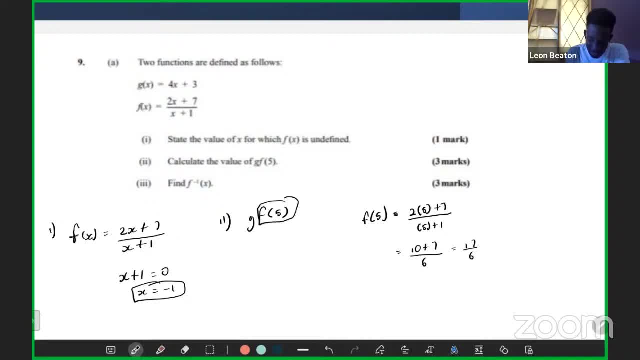 f of five is equal to 17 over six, so this will be: g of 17 over six is equal to: so we take in that and we put it inside of this function. now this would be four. x instead of x would be four times, uh, 17 over six plus three and four times 17 over six will give us what. 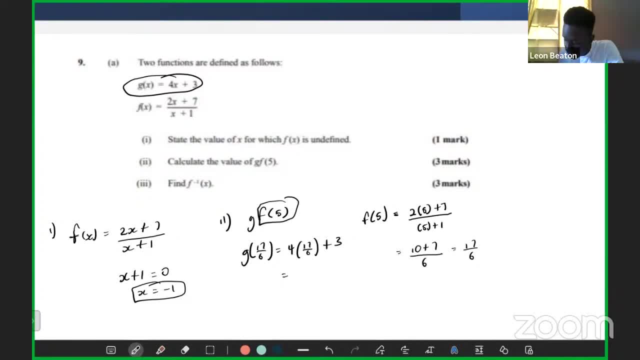 the four times 17 will give us 68 to 68 over six plus three, that would give us, uh, 14, one on one over three. so, gf of ah, this question, look, kind of this. this here looks, i wonder if i did i made a mistake, did. 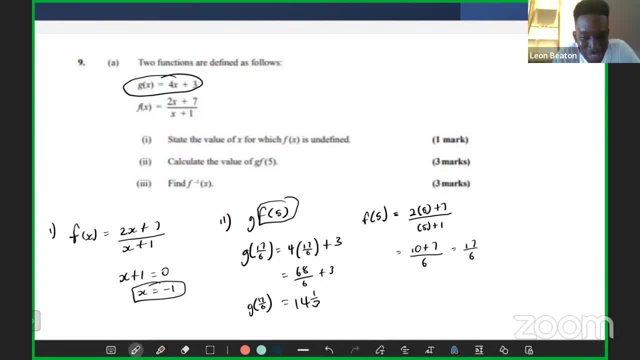 i make a mistake, or cx gave us this fancy um answer, but you definitely. we did everything correct. so the first thing we had to do was find um f of five. so we found f of five to be two times x plus seven. so two times five, which is ten plus seven, is seventeen. 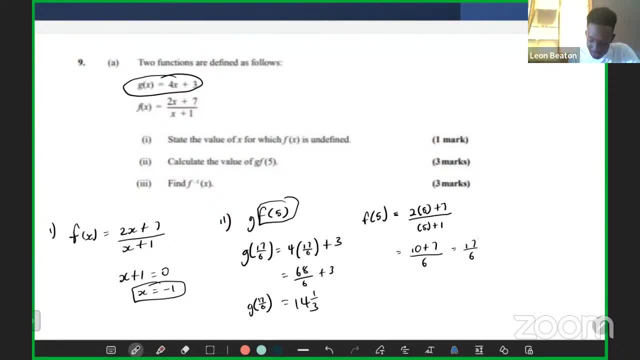 and five plus one is six. so ten plus seven would be seventeen divided by six. so that is f of five. and then we take f of five and we put it. we put it inside: uh, the g function, and this is the g function. so this will be four times x plus three, and we found x to be seventeen over six. so this will be. 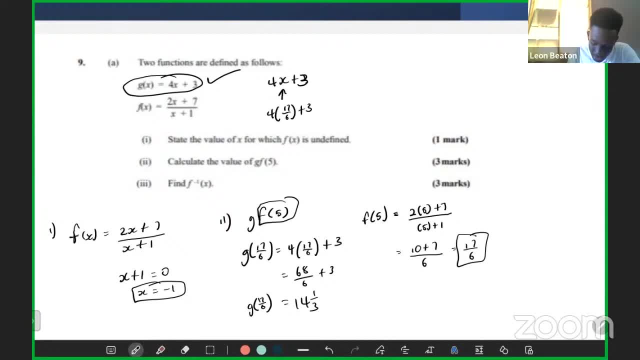 four times seventeen over six plus three. yeah, that's what we did, right? so our answer is fourteen and one over three. the question went for three marks. i guess that is why. where do you go that? yes, sir, yes, sir, all right. so those you know joining, i have a few, i have a few of my students. 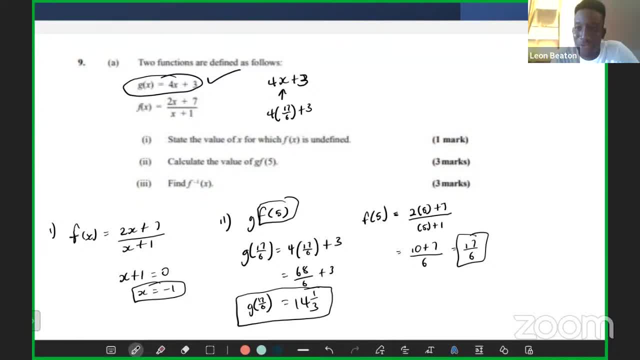 um, in class here with me, because we've been going for a long time and it would be very- i was uncomfortable, very strange, talking to myself for a very long time. so i had to get some company. i had to get some of my willing, willing students to come and join. very brave. 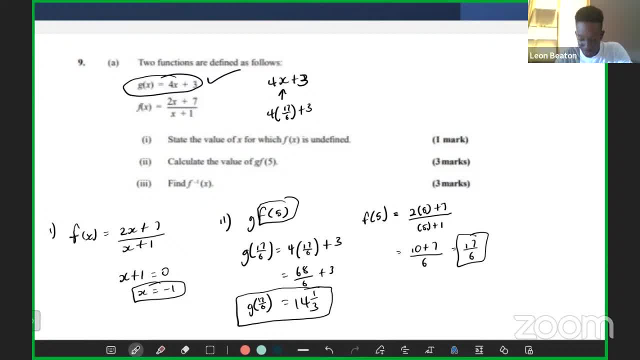 all right. so i now went for three marks. so we had to do some monk of words. there you find for composite functions. you're taking the outer function, i put it inside the inner function. so in this case we had to find g, f of five. so before we force, find f of five and then we take. 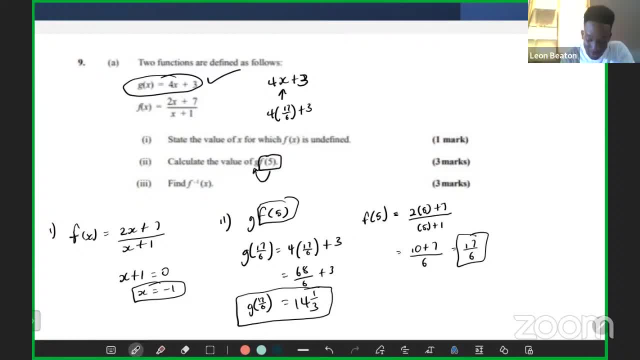 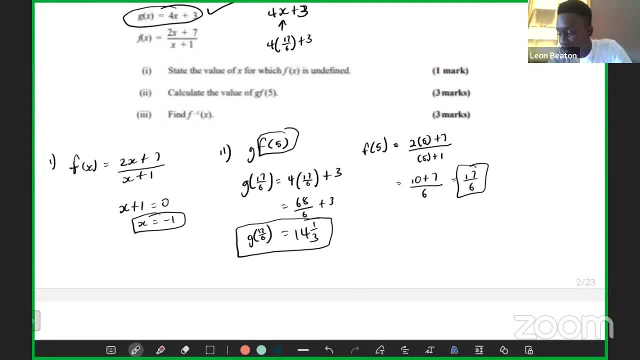 that value for f of five and we're putting it. we put it inside the g function, all right. so that's it for that one. so, last but not least, for three marks as well. now, for the time you see a question is going for three marks, that means um, they gotta do some amount of work right. cxc will not give away. 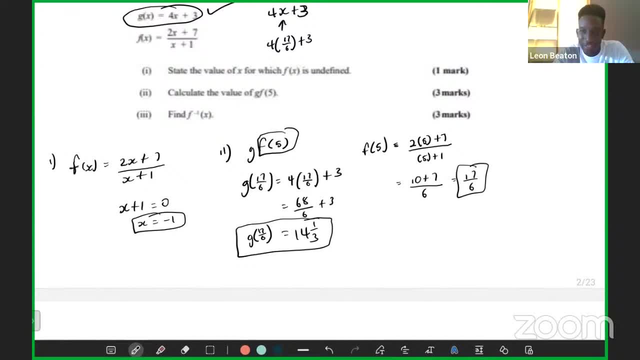 three marks like that. so you can a question- you can't see a question- for three marks and then one, do one line or two line. i'm easy doing something wrong if you do one line or two lines for three marks, all right. so the marks: direct correlation between the marks and the 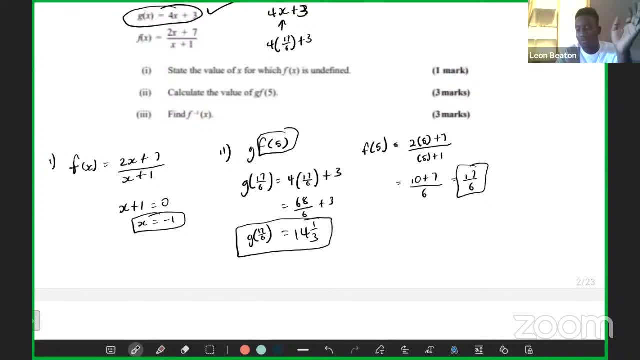 amount of work that you gotta do. one mark, very simple. two marks, yeah, a bit challenging. all right, three marks, you gotta do some amount of work. so f inverse of x. so you want to find f in the force of x. so we're dealing with the f of x. 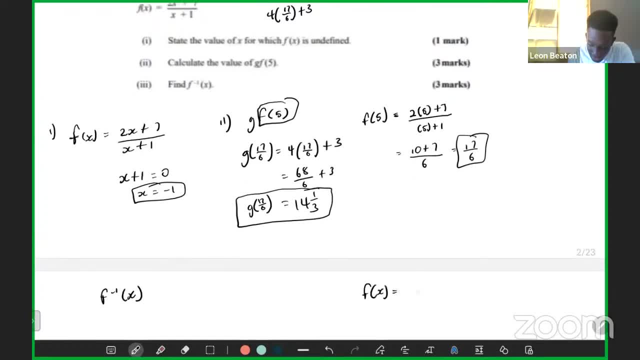 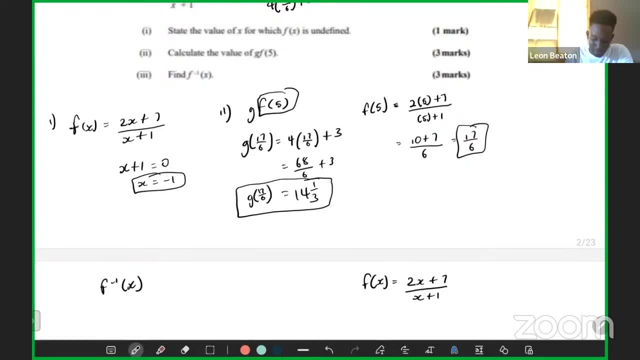 function which is um. suddenly right about the f of x function: uh, 2x plus 7, all divided by x plus 1.. so anybody um if inverse of x. let me see who can remember how to solve this in the future. let me see who can remember how to solve this in the future. 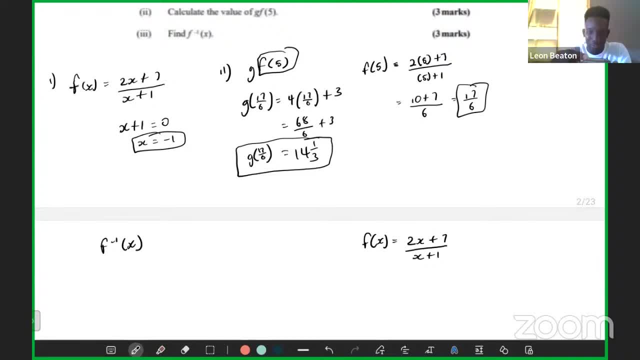 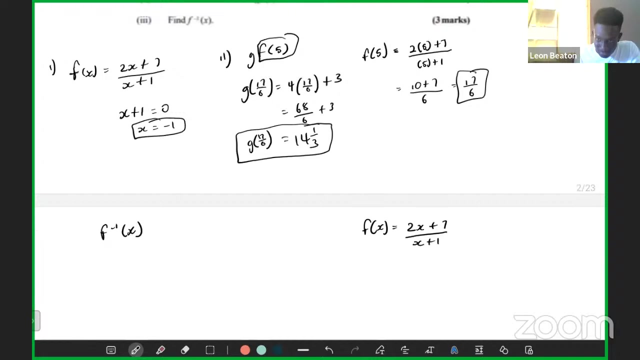 how to work all this, anybody. we change the um f inverse of x into y and then we switch the y and x values and then we work from there. all right, excellent, excellent, excellent. so we switch, we, we change the f of x to y. So when you're finding the inverse of a function, 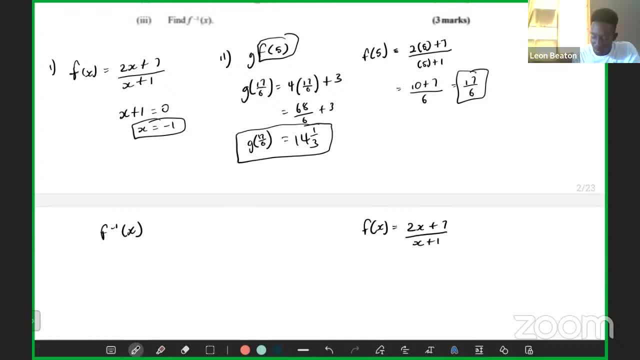 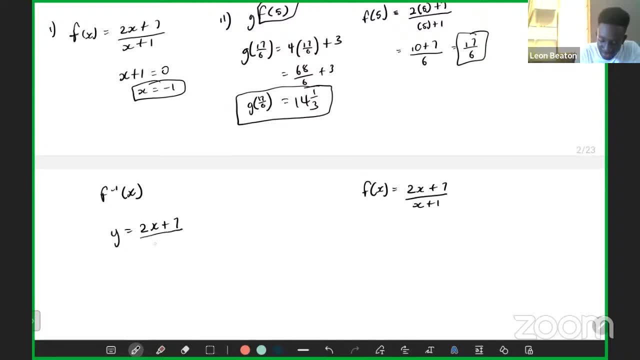 you basically follow some steps, Forcing and changing f of x to y, So we'll have: y is equal to two x plus seven, all divided by x plus one. And then what do we do next? Change the x and the y, right. 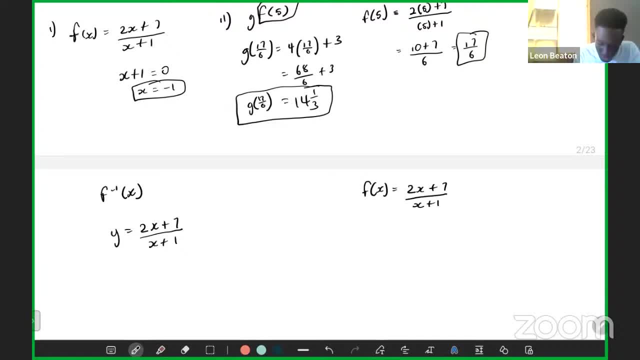 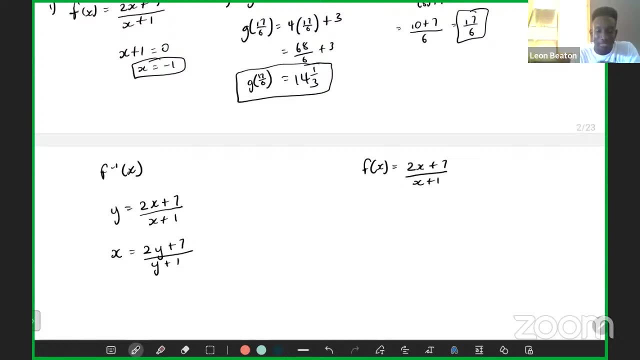 So we have: wherever you see y, you put x, Wherever you see x, you put y. So this will be: x is equal to two y plus seven, all divided by y plus one. So now, after we finish doing the nice part, 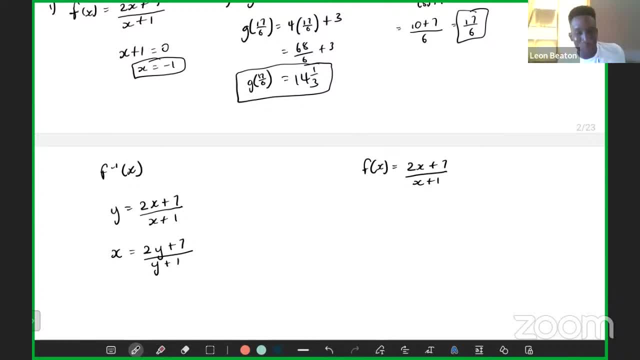 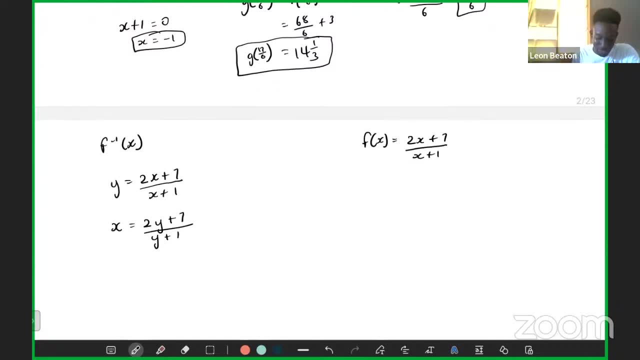 after we finish doing the nice part. we gotta make y the subject now, And you know, this is where the challenge will come in. So let's go make y the subject. So anybody? what's the first thing we should do? Let me not work it out. 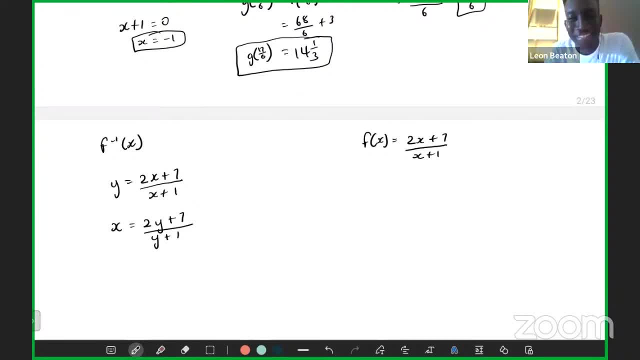 Let me give you an opportunity to shine. What's the first thing we should do? You know, you carry over x, y plus one, sir, Carry over y plus one. So the y plus one is divided. So we take over that y plus one. 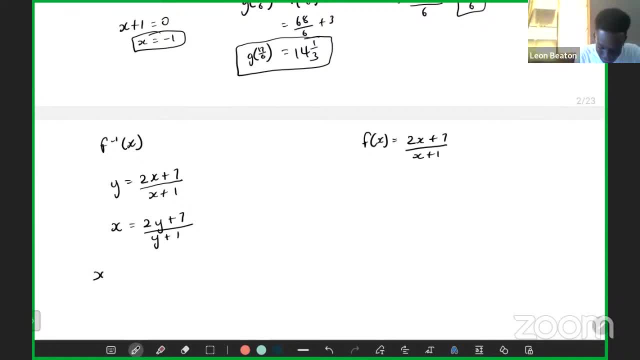 It will multiply right. So we'll have: x multiplied by y plus one is equal to two, y plus seven, And then we multiply. We do use the distributive law. We should be able to do the distributive law in our sleep. 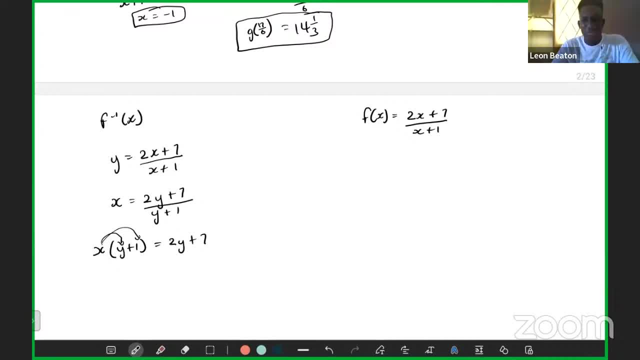 given that the exam is a few months away, So we'll have a few months. Did I say months, Weeks away? So this will be x times y, the xy plus x times one of the x, And that is equal to two y plus seven. 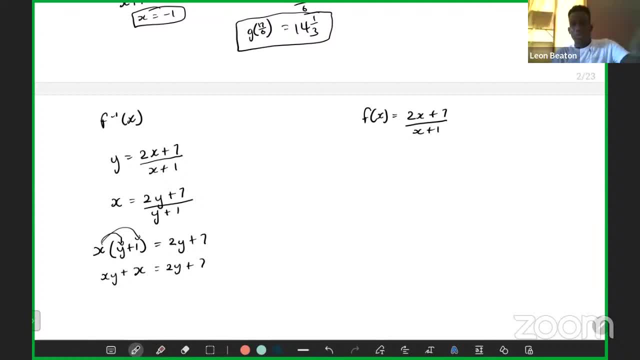 Good, What next? How else can we, what else can we do to make y the subject? Anybody? What else can we do to make y the subject? Yeah, x. y plus x is equal to two y plus seven. Sir, take over the two y and the x. 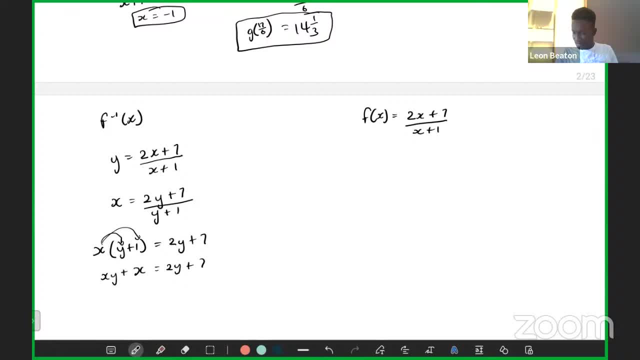 Take over the two y and the x. All right, So take over the two y and the x. So we put it. we put it all the terms y, we put them together, right, So we'll have x- y and this is plus two y. 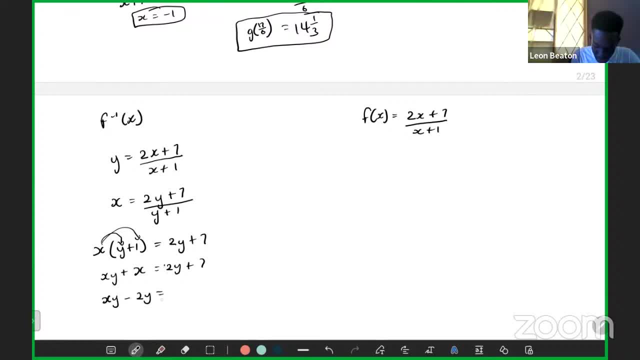 So we take the, we go minus two. y is equal to- and we can carry over this- this plus x, So this will be seven minus x. So we have x y and we have two y. We got two y, but how can we turn these? 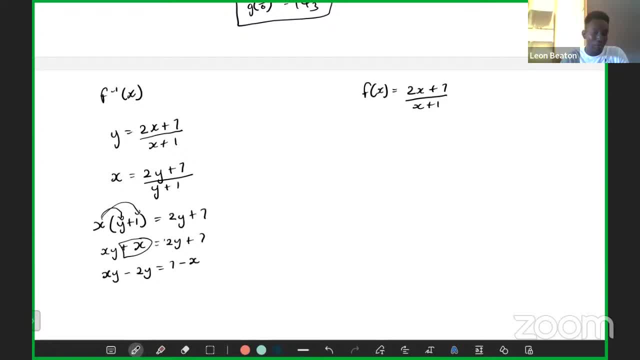 these two y's that we have here into into one y. We can. we cannot make two y the subject. We have a y here, we have another y here. We can't. we can't deal with them two y's. 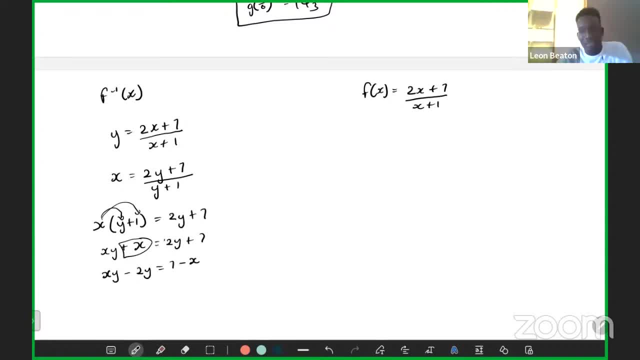 You got to turn that into one y. So what can we do? What taking mathematics can we do to make? what can we do? Make those two y's into one y, Anybody? So we factorize, Yeah, yeah, yeah. 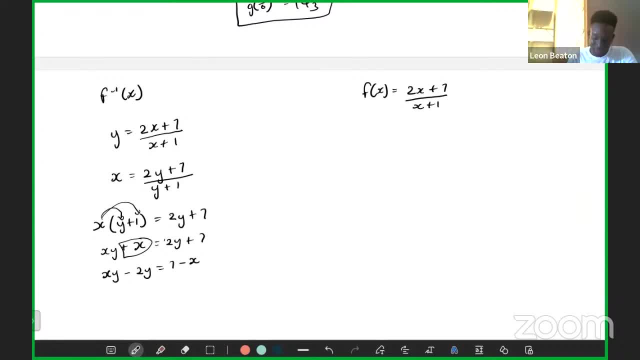 Factor out the y. right, We factor out the y from the two terms. So we have y here, we have y here. so we factor out the y. So we factor out the y. we'll be left with x minus 2 is equal to 7 minus x. 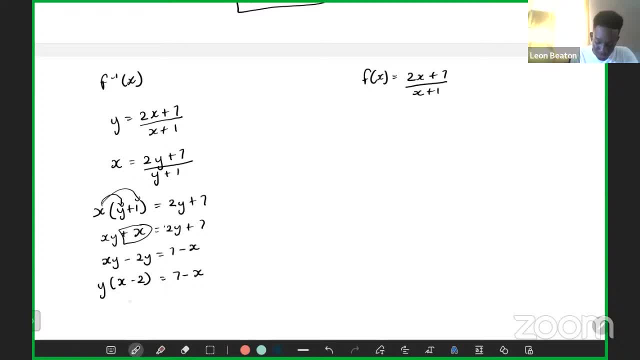 So now we can make y the subject by taking over this x minus 2.. So this will be: y is equal to this. x minus 2 is multiplying the y. So we take the real divides, We'll have 7 minus x, all divided by x minus 2.. 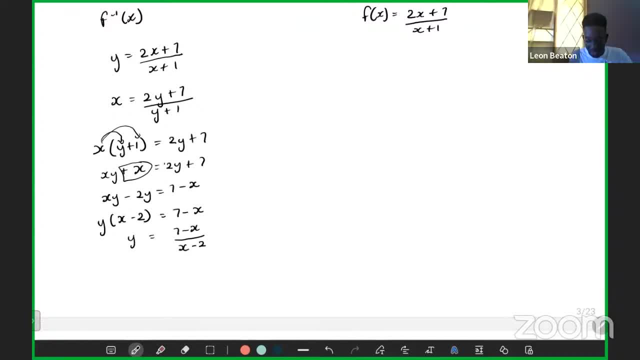 And then the last but not least, the easy step: we change y to f inverse of x, And that is what we wanted to find. So f inverse of x is equal to 7 minus x, all divided by x minus 2.. And there you have it, your three marks right. 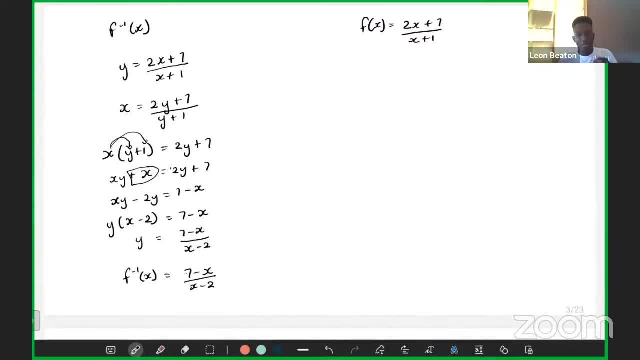 Three marks, All right. So, as I said, there's a direct correlation between the amount of marks that the question is worth and the amount of work that you've got to put into the question. So you want to keep that to the back of your mind when you're working on these questions. 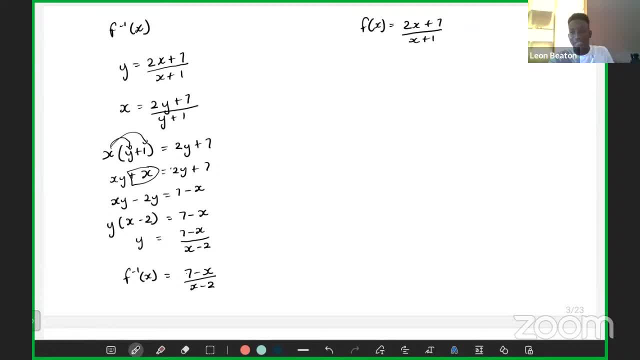 If you see a question with three, four marks, you can't get two lines, You can't get one line Unless CX. you know CX decides to be real timed and you know: All right, everybody go there. Yes, sir. 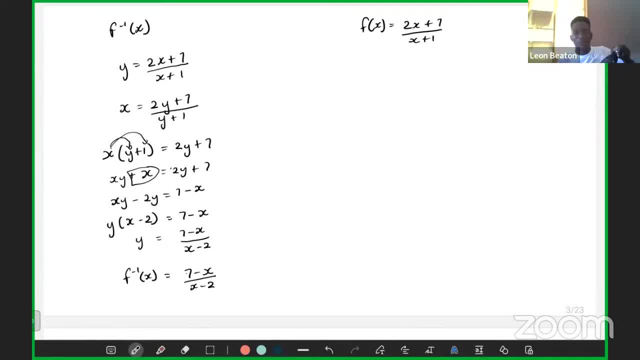 Yes, sir, For those of you now joining, I have a few of my students on the live, because we've been going for a while And I don't want to speak to myself for so long. I have some of my brave students here joining me for some questions with me as well. 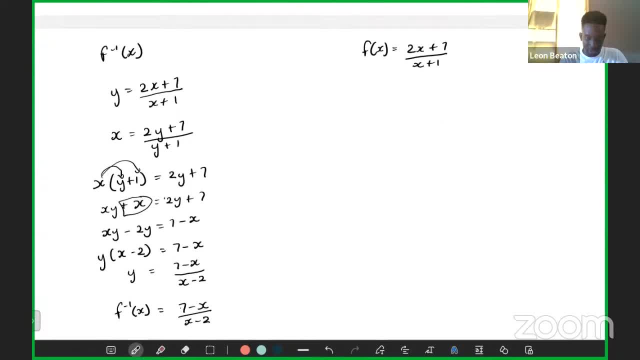 All right. So that was functions. This is probably one of the challenging ones for functions. Sometimes you may come across a simple function like f of r, Let me not use. Let me use: g of x is equal to, let's say, 5x minus 3.. 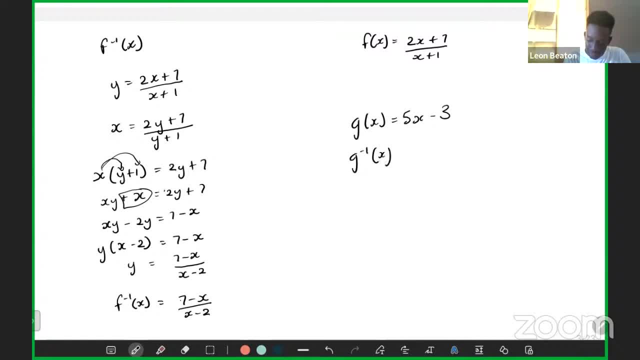 And I want you to find g inverse of x. This is a bit more. This is a bit easier than the one that we just did. We follow the same steps, but it would be easier. So, step one, we change g of x to y. 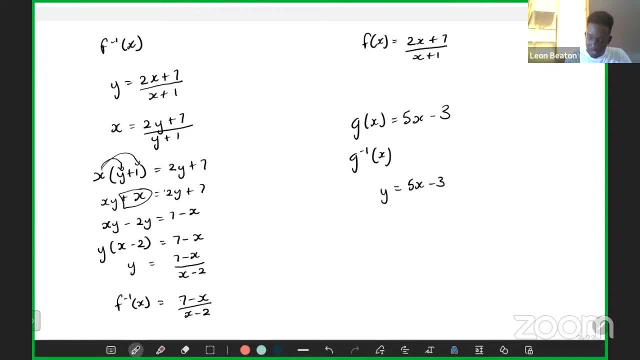 So we'll have: y is equal to 5x minus 3.. And then we interchange the x and the y, So we'll have x is equal to 5y minus And then, just like just now, we make y the subject. 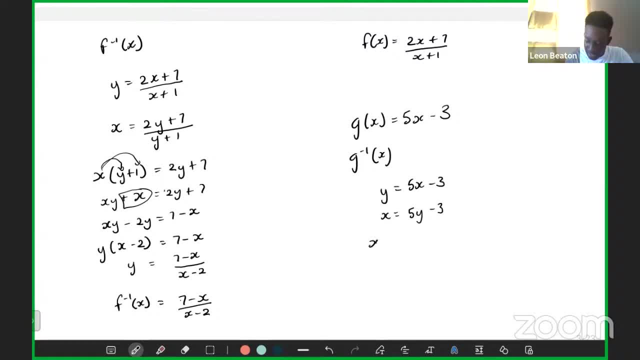 But this is a bit more easier to make y the subject. So we'll have x, The 3 is minus n. We take the over the other. So x plus 3 is equal to 5y And the 5 is multiplying the y. 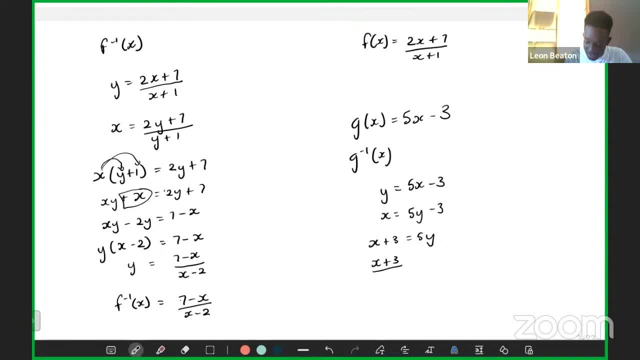 We take it over to divide, So x plus 3 all divided by 5 is equal to y. And then, last but not least, we change y to g, inverse of x in this case, So we can switch it around. So this would be: y is equal to x plus 3 all divided by 5.. 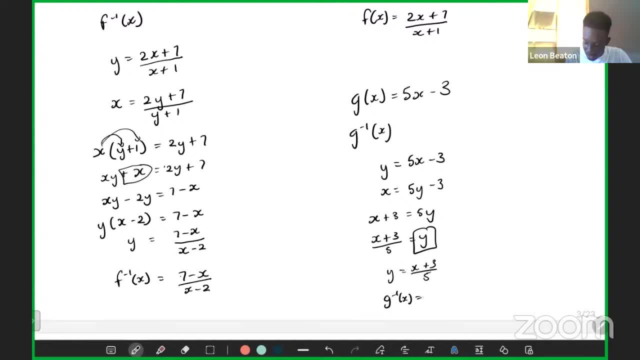 So we'll have g. inverse of x is equal to x plus 3 all divided by 5.. This is an easier version of this one that they can bring, And this will probably be worth two marks or so. So this is an easier version of this here. 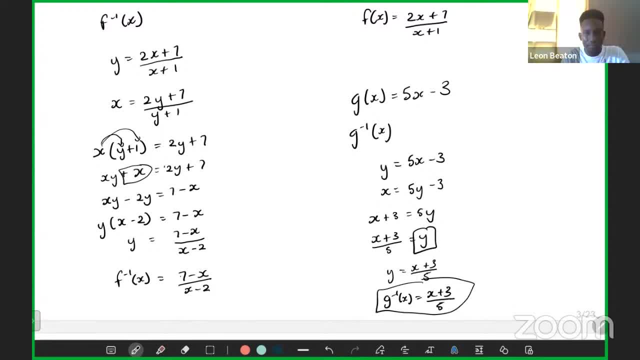 So if you come across one with a fractional function, you know you got to put in some work, You got to do some factorizing, some part of the other, And then from here they can also ask you to find g inverse. So let's say, let's say 7g inverse of 7.. 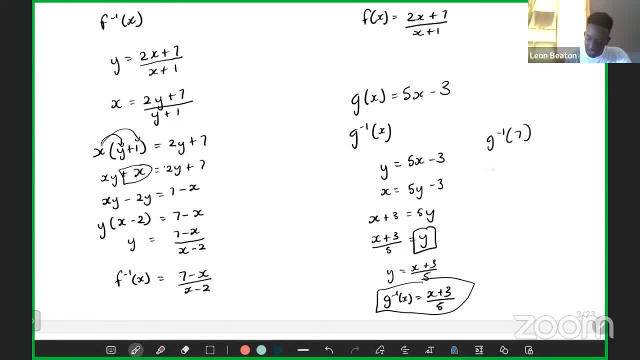 So you're taking this 7 and you're putting it inside of the inverse function that you found here. So this will be g. So this will be g. inverse of 7 will be equal to. we put in 7 inside of this function. 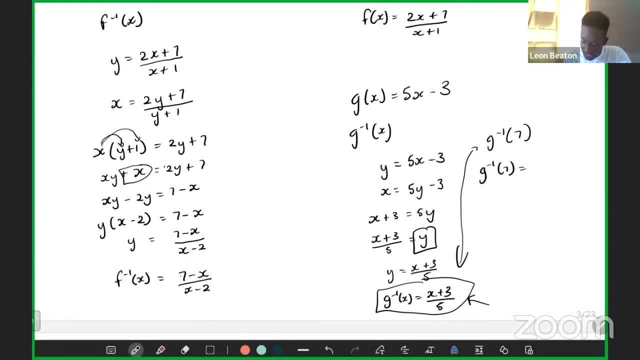 This will be x plus 3 all divided by 5.. So instead of x, can we replace x with the 7?? We got to do the same thing. So this will be 7 plus 3 all divided by 5.. And 7 plus 3 is 10. divided by 5 is equal to 2.. 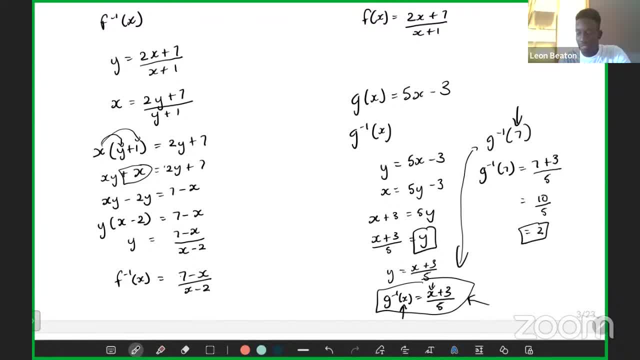 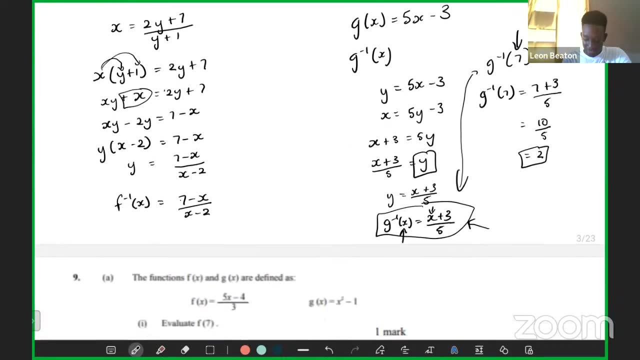 That is how you can find g inverse of whatever thing you want to find. All right, All right. So that was it for that part of functions, Let me see. Let's see what else I have here. I have another set of functions. 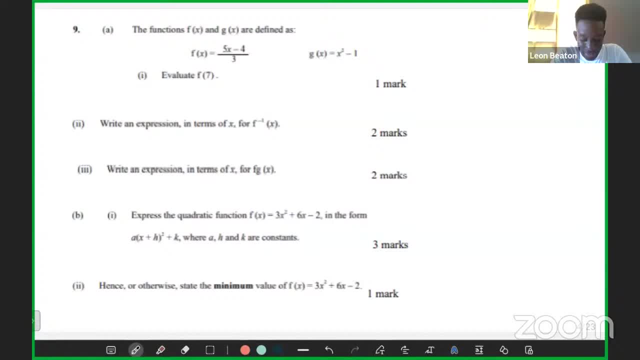 So we have the functions. f of x and g of x are defined as: f of x is equal to 5x minus 4 all divided by 3. g of x is equal to x squared minus 1.. So I want to evaluate f of 7.. 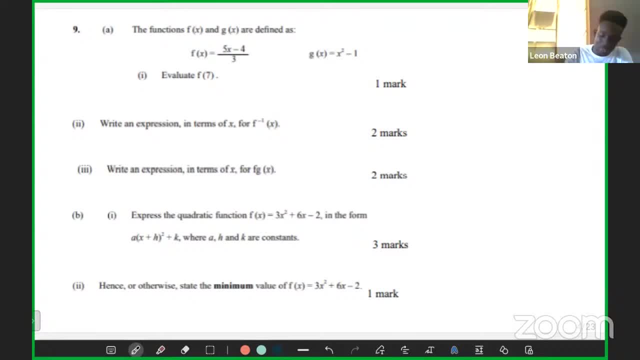 So f of 7 is simple, So let me work with that one. So we want to find f of 7.. So once again we put in the 7 inside the function f. So f of 7 would be equal to: instead of 5 times x, is to be 5 times 7 minus 4 all divided by 3.. 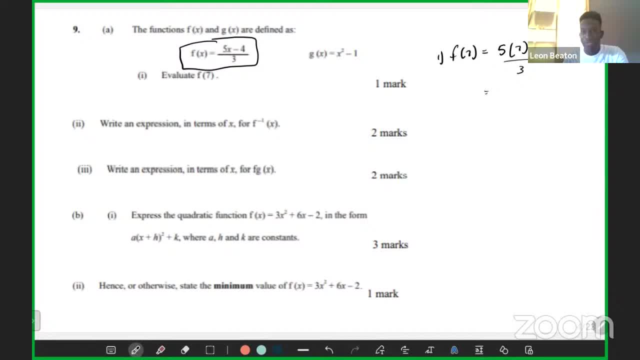 5 times 7 would be what? 5- 7s Young brains, 5- 7s, Sorry to fight. Sorry to fight. See, I'm brain young and I'm my own, All right, I mean it is 5 star to 5 minus 4. all divided by 3 star to 5 minus 4 should give me what. 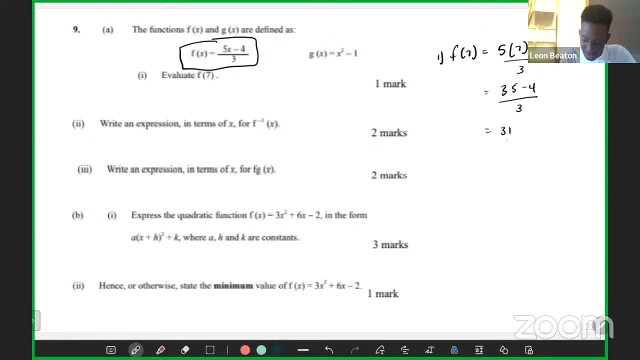 Star to 5 minus 4 would give me star to 1.. Correct Star to 1.. Star to 1 divided by 3.. Star to 1 divided by 3.. We can break this down So 3.. We can go into star to 1 10 times and we'll have back with 1 over 3.. 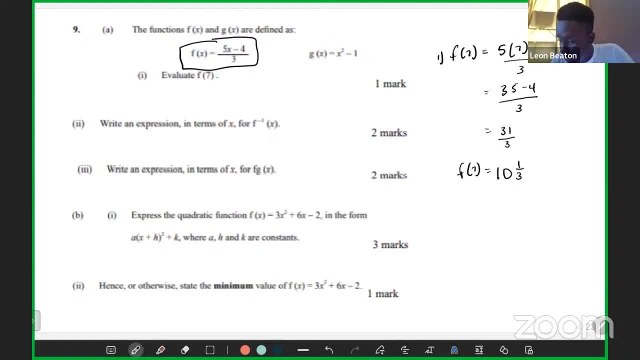 So f of 7 is equal to 1 over 3.. 10 and 1 over 3.. All right, That was simple. We're at one mark. One mark for that, So the next one. Write an expression in terms of x for f inverse. 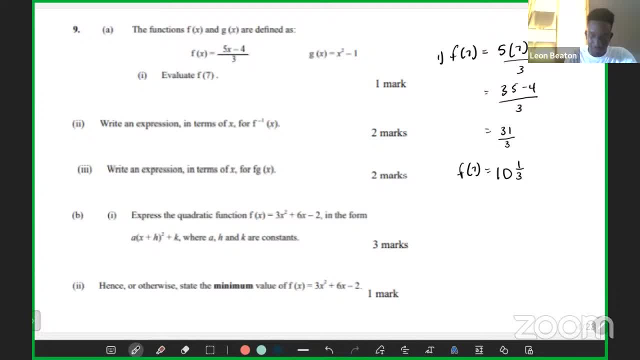 So you want to find f inverse of x. And since we did this one just now, let me hear, Let me get, Let me hear somebody, Somebody work this one out for me. So let me hear f inverse of x. So somebody work that one out for me. 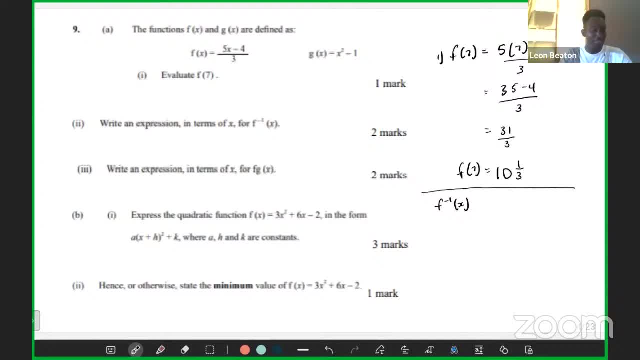 Take us through, Lead the way, Take over the class F- inverse of x, F- inverse of x- 公式, These functions we're using, Huh, Either way, that may be actually a really good method. Oh, Just trying to get to a really control, nope. 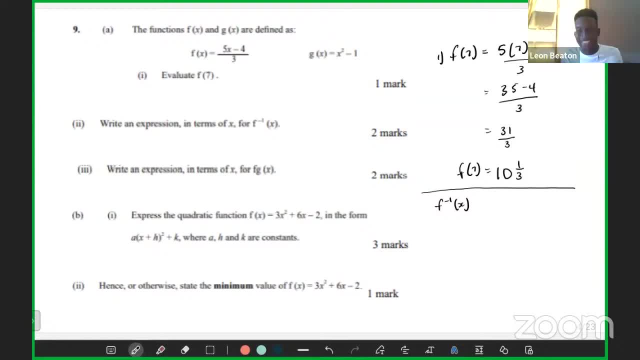 Nope, no, Okay, Move the thing showing f. Here we are, Be careful, There's no, Not this, No, All right. so we're basically finding the inverse function right. So that's when I say: write an expression in terms of x or inverse of x. 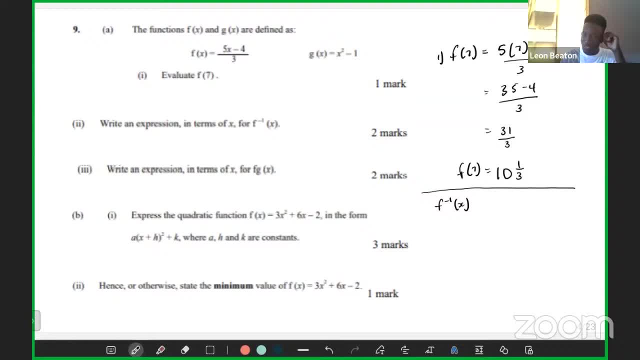 We're basically finding the inverse function. We're not doing anything fancy, So somebody find the inverse function for me. All right, so we have to find – if we don't like what we did just now, this is the function that we're using. 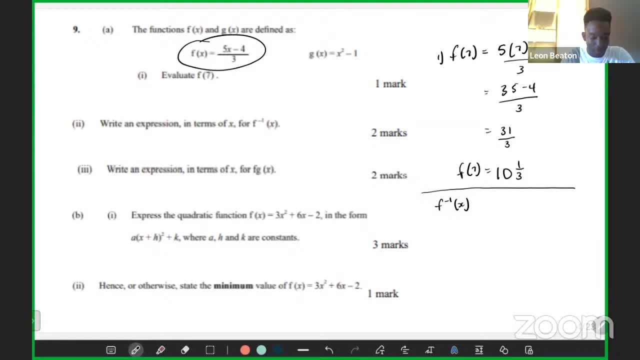 So once again, forcibly replace – what are we? – what's the fourth step? Replace f inverse with y, All right, replace f of x with y, right F of x with y, So we'll have: y is equal to – 5x minus 4, all divided by 3.. 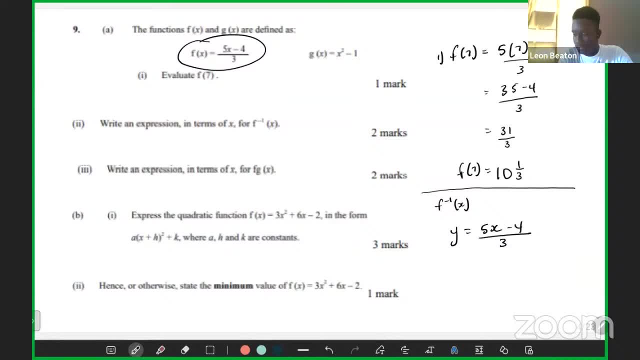 And what next? Next step? Yeah, Go ahead, Singh So – Finish it Singh. x equals 5.. All right, so we interchange x and y, So this will be: x is equal to 5.. y minus 4, all divided by 3.. 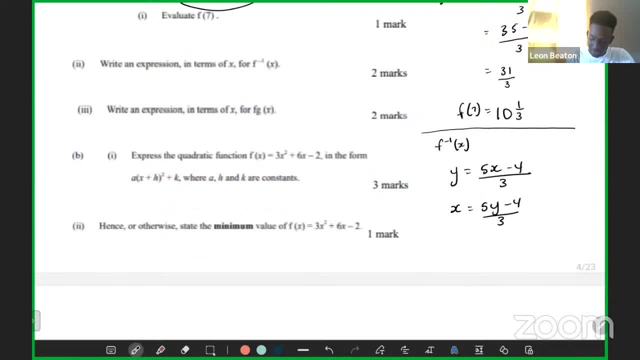 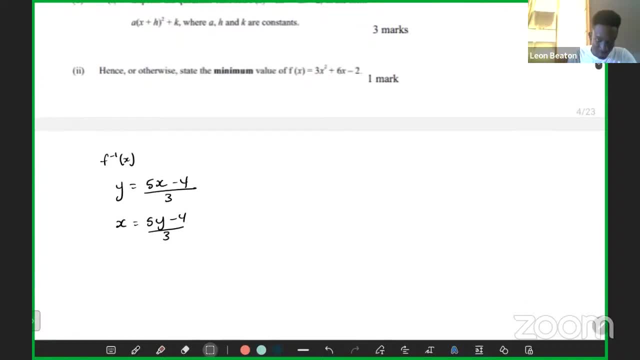 And then we simply make y the subject, right. All right, so I have to bring this down. So we simply make y the subject level. So this would be: 3 is divided, And we take the word multiply, So we'll have 3.. 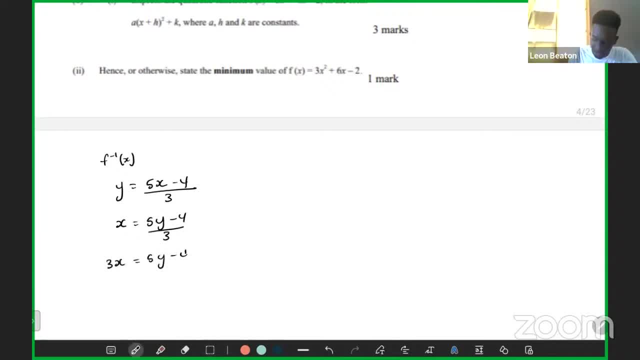 3 times x will be: 3x is equal to 5y minus 4.. And then we make y the subject from here. So this would be this: 4 subtracting, Take the word add, We'll have: 3x plus 4 is equal to 5y. 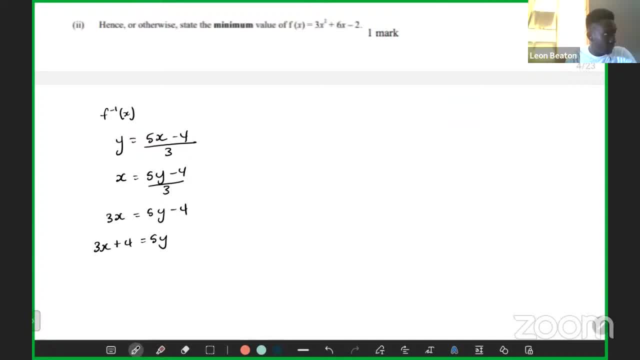 And the 5 is multiplying the y. So when we take that over it will divide. So we'll have 3x plus 4. all divided by 5 is equal to y. And last but not least, we replace the y with the f inverse. 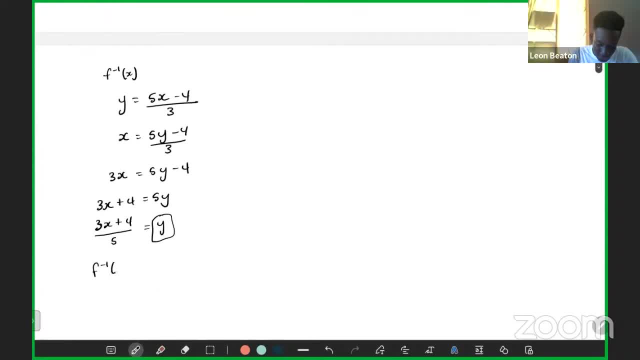 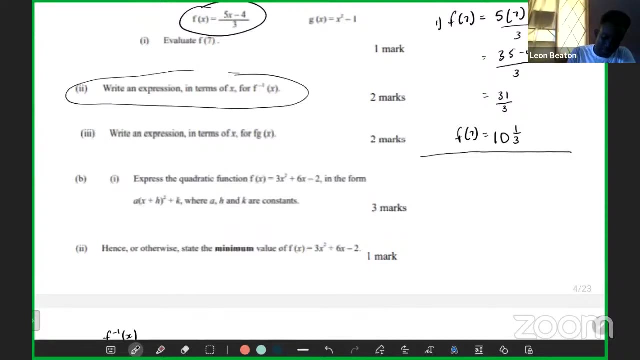 It's f inverse of x. So f inverse of x is equal to 3x plus 4. All divided by 2.. And that is how you write an expression in terms of x for f inverse of x. It's simply just another way of saying: find the inverse of f of x, right. 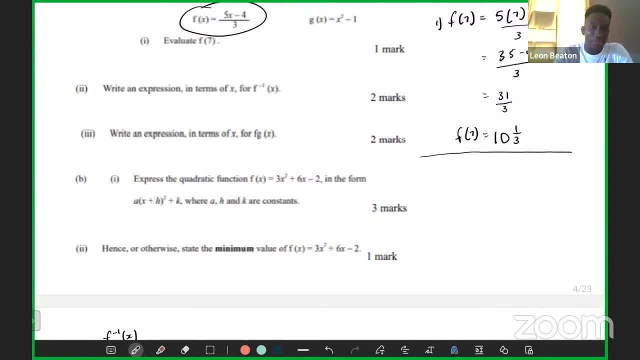 So look also for questions like that. They may tell you: write an expression in terms of x for whatever, but it's simply finding whatever they give you here, right. f, inverse of x, And the same thing here. Write an expression. Write an expression in terms of x for fg of x, right. 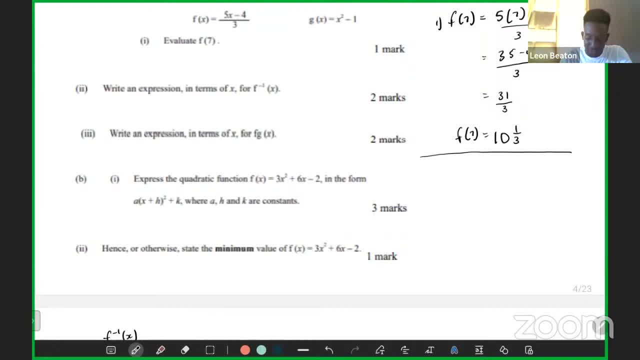 So fg of x? What are we doing exactly for fg of x? This is a composite function. What are we putting here, Anybody? what are we putting? What do you mean? g into f? Sorry, put in g times. We're putting the function g into the function f, right? 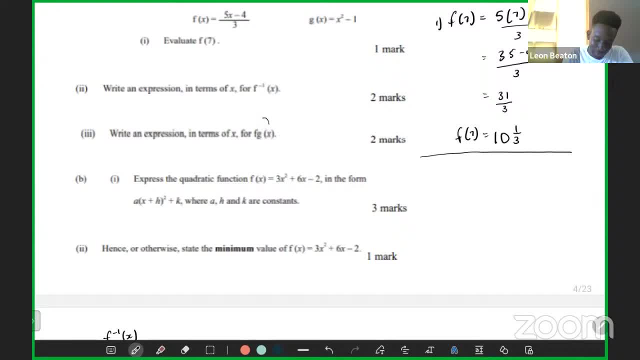 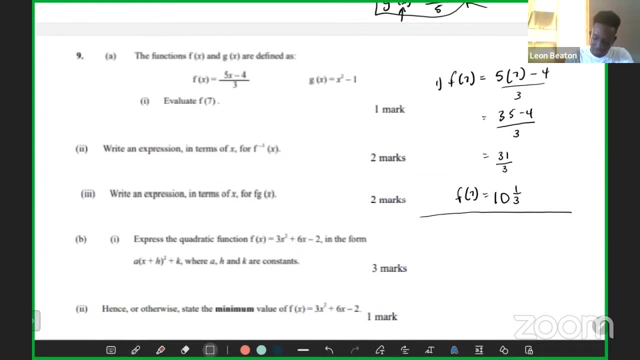 Right, Right, Right, Right, Right, Right, One on the outside. We're putting it on the inside right. We're putting g of x into f, right. So let me pull this down a bit so I can work on it. 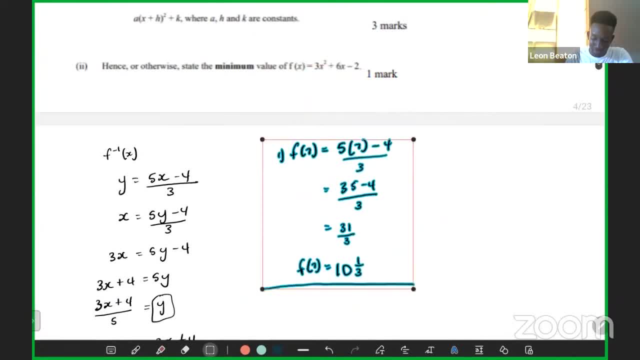 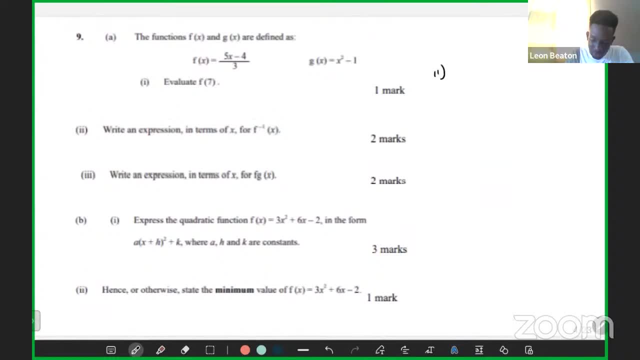 so we can see the equation that we're working. So we'll put this down on the bottom here. Number one, number two, Let's go Number three. So we put in the function g, So we take g, so fg of x is equal to. we're taking the function g, we're putting it, we're. 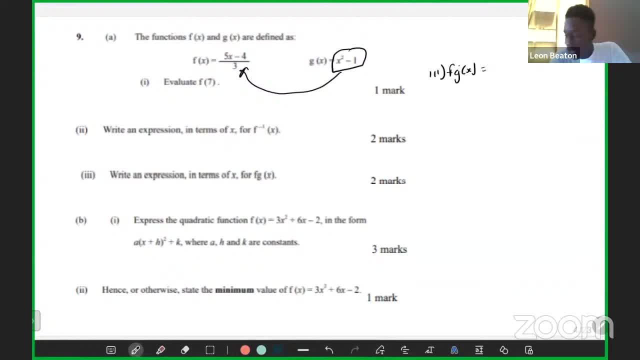 taking this function and we're putting it inside of this function. And how are we putting it? We're simply, you know how are we putting it. We're simply putting the function and we have to see x, we replace it and I put in: 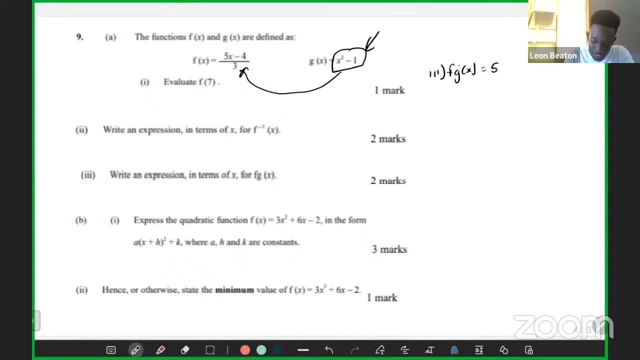 this function. All right, So this is the function. This will be 5 times x, 5x, But instead of x we're putting the function x squared minus 1.. So 5 times x, squared minus 1 minus 4, all divided by 3.. 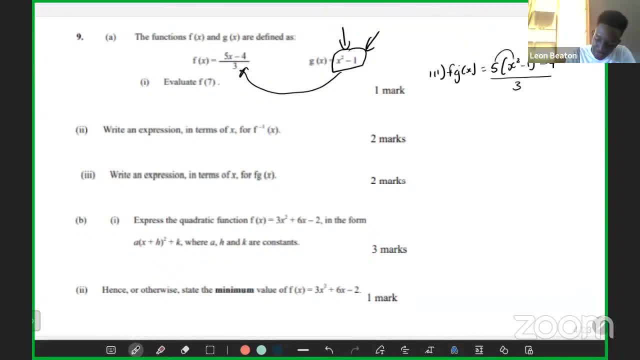 And then we do some simplification. This will be 5 times x squared 5 times 1.. So 5 times x squared is 5x squared minus 5 times 1 would be 5 minus 4, all divided by 4.. 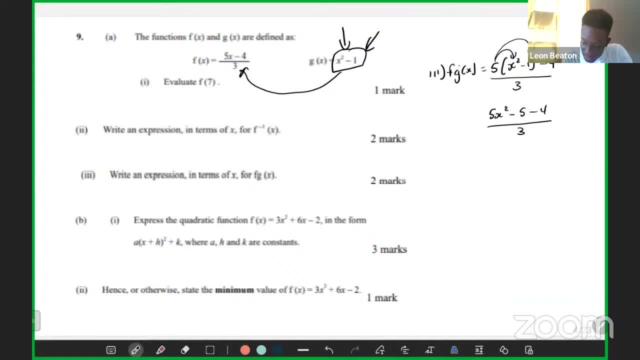 And then we do some simplification. So 5 times x, squared minus 1 minus 4, all divided by 3. And then this would be 5x squared minus negative 5 minus 4. That would be negative 9.. 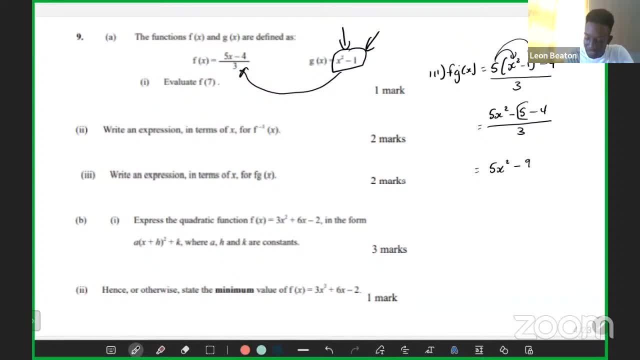 And we've got to be careful with this. Some students tend to make the mistake of minusing 5 times 4.. But remember, you've got to take into consideration the sign in front of the term, right, The sign in front of the term. that is the sign that is governing the term. 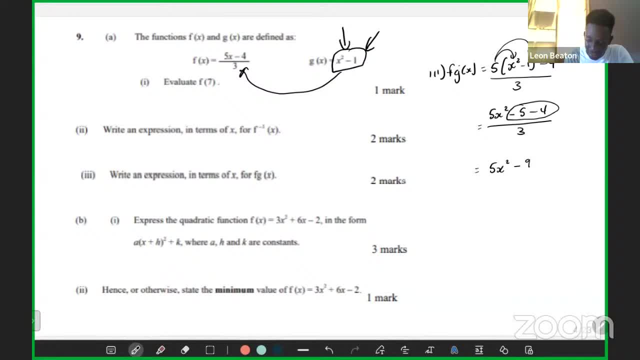 All right, So this is like. this is like I have negative 5 minus 4.. And then, alright, So this is like. this is like I have negative 5 minus 4.. divided by three, and that would be f, g of x is equal to that, so that is the. 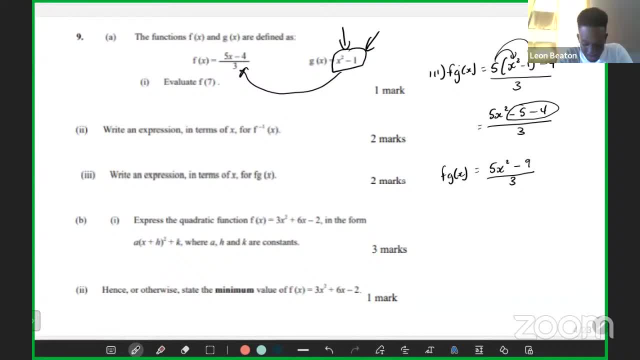 that is how you write an expression in terms of x for f, g of x. anybody go there? yes, sir, all right, so we're going into a big question. let me see who can remember this one. so express the quadratic, express the quadratic function: g, x, square plus 6x minus 2 in the form: 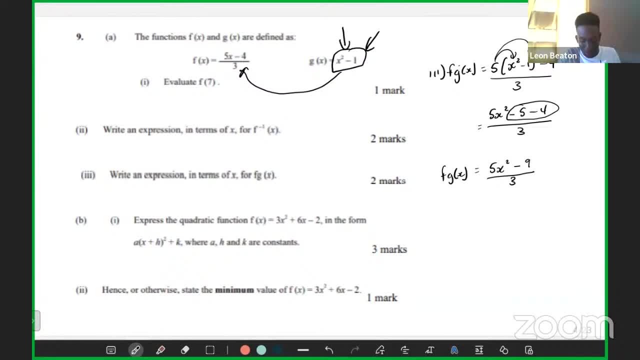 a plus h, square plus k, where a, h and k are constant, three marks i. i don't want to, i don't want to give. I want somebody to tell me this here: man, Let's see who would have gotten these three marks. Who would have gotten these three marks? 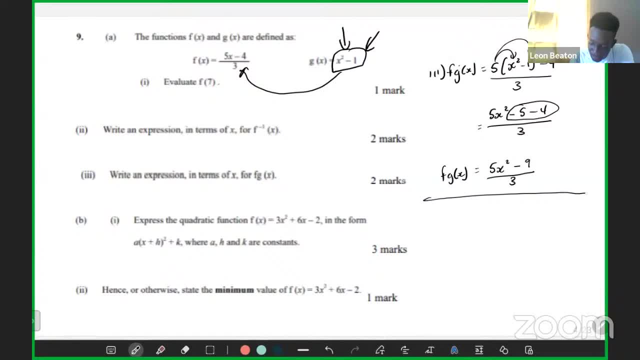 So let me write it over. What kind of function is this again? What kind of function this is Anybody? what kind of function did they say? it is 3x squared plus 6x. It's a quadratic function, right. 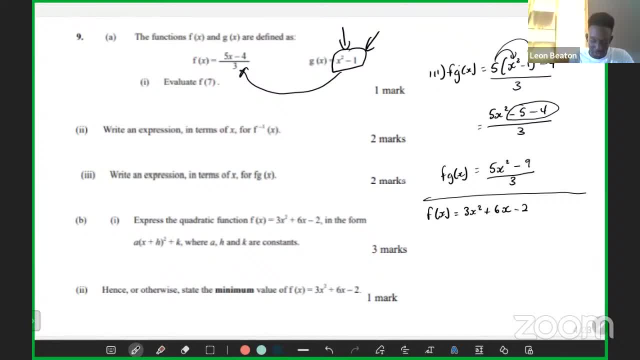 It's a quadratic function, So we want to write this quadratic function in this form. So let me hear where I think we should go. first. Big question: Big marks. Sorry, I think we have to find for k and h. Yeah, find for k and h. 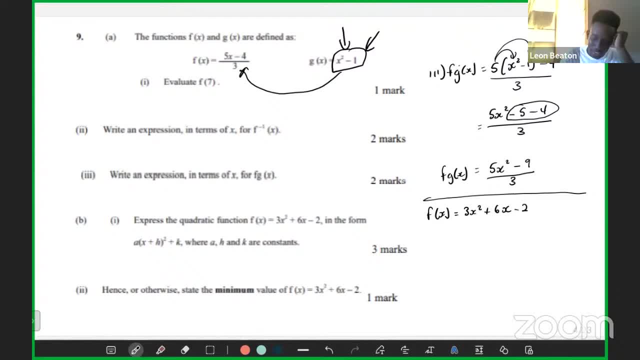 Yes, sir, Yes. So there are two ways you can do this right. We can either complete the sphere or we can use the formula. So, yeah, I can remember the formula. Yes, Anybody remember. Yeah, you can remember the formula. 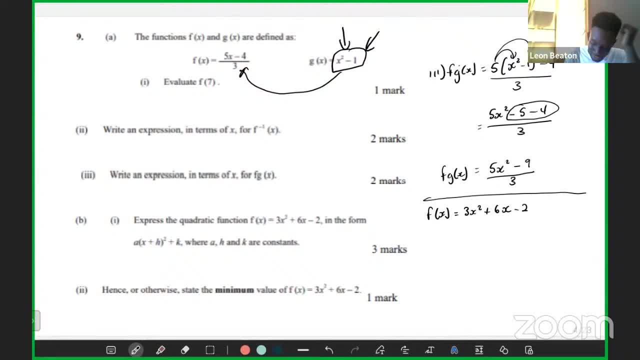 Yes, Yeah. So the thing is, first of all, what is a? A is three, right, So this here. So a is three. What about h? What is h? How do we find a? First of all, before that, let me identify. 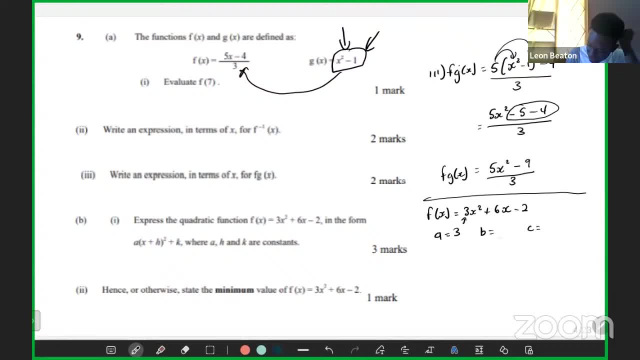 What is b as well? What is c? b is six and three, c is negative two, sir, c is negative two. Good, So we know a, b and c. Now we want to find h and k, right? 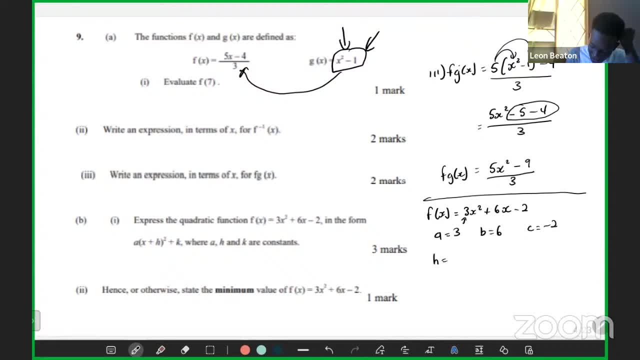 So how do we find h, b over 2a, b over 2a? All right, So it's b over 2a. So we know b is six. So we know b is six over 2 times a, which is three. 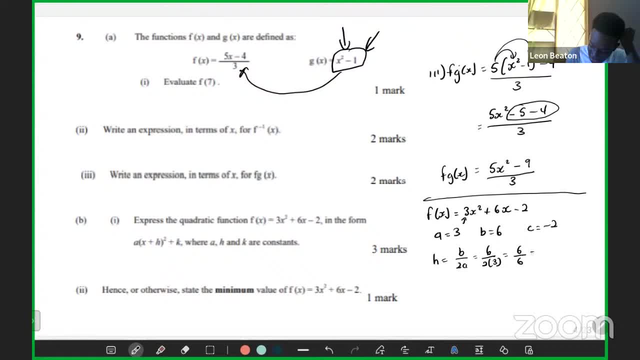 So six divided by two times three is six. So six divided by six is one. So h is one. right Next thing: what is? how do we find k again, Sir? 4ac minus b, squared divided by 4a. 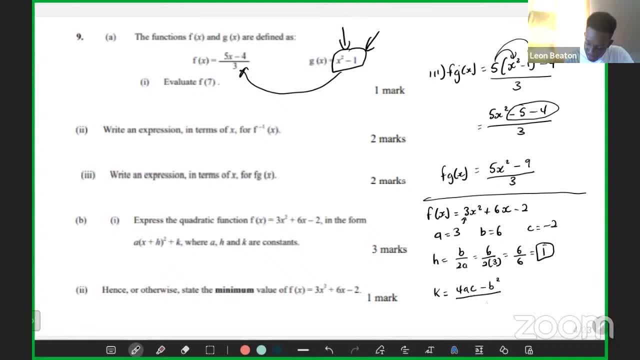 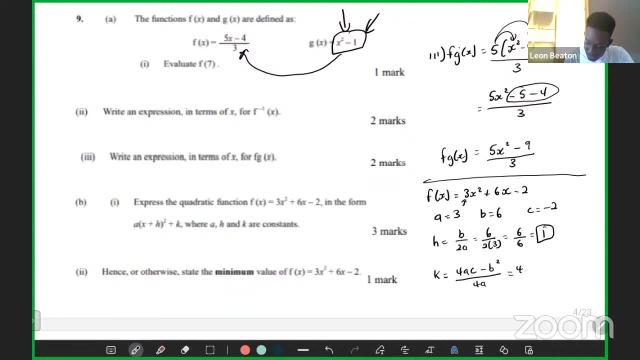 4ac minus b, squared divided by 4a. 4a. Like this here, Exactly like this. Yes sir, All right, Another form we can use as well, But nevertheless, let's go. So it's four. 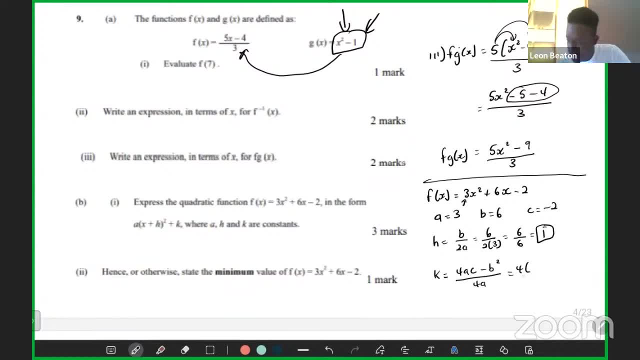 So we just substitute in the value of a, b and c. So it's four times a, which is three, times c, which is negative. two subtract b squared, which is six squared, All divided by Four times a, which is three. 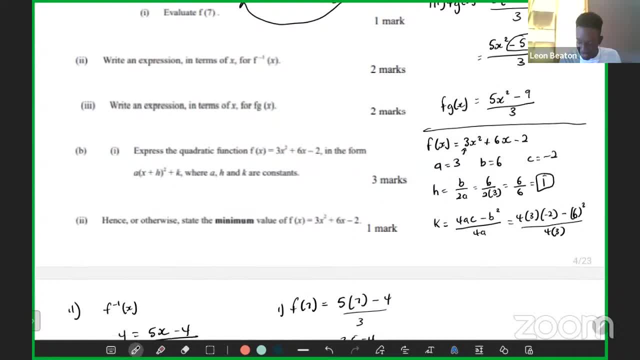 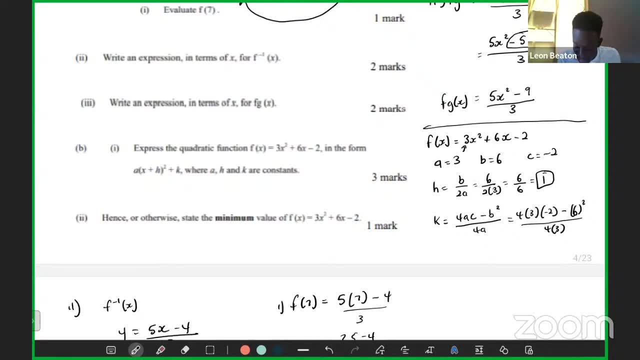 So this is a lengthy formula. Can anybody remember the other formula? I mean it's similar to this, It's the same thing, but, Sir, c minus b squared divided by 4a. c minus b squared divided by 4a right. 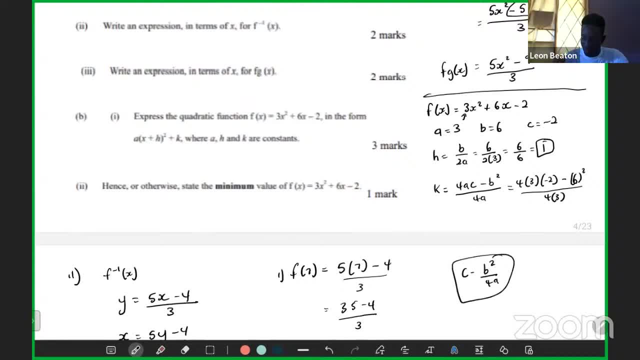 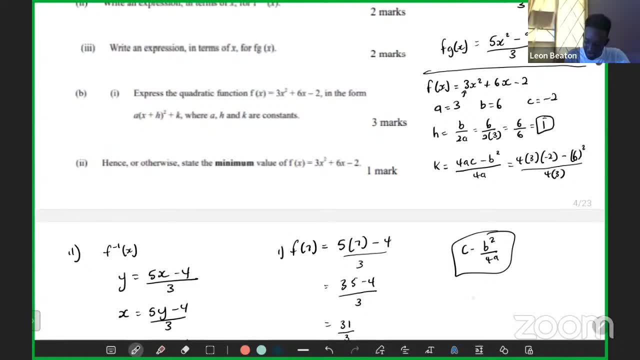 Yeah, this is another formula. This is another formula, Can you? They both are the same thing, but it's just that with this formula, what they did, they kind of simplified. They put 4a as the LCM and 4a. 1 divided by 4a is 4a. 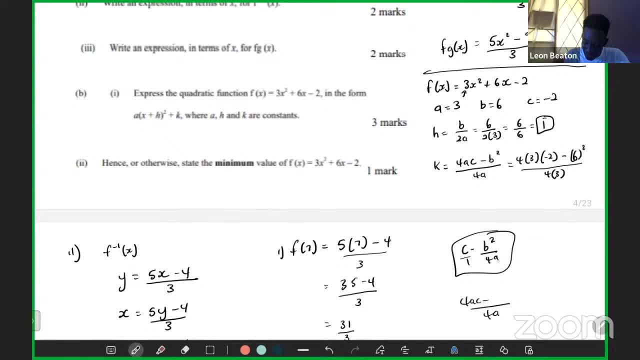 4a times c will be 4ac minus 4a, divided by 4a is 1.. 1 times b squared will be b squared. So it's the same formula, right? But you know, whichever one you feel comfortable with, it's up to you to get the same answer. 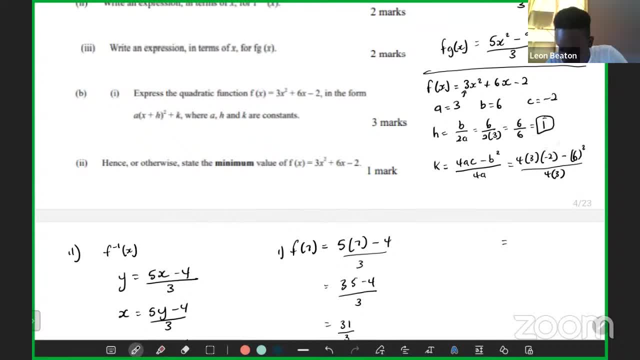 Anyway. so let's simplify. So it's 4 times 3 times negative, 2.. 4 times 3 is 12.. 12 times negative 2 would be negative. 24 minus 6 squared would be 6 times 6 would be 36.. 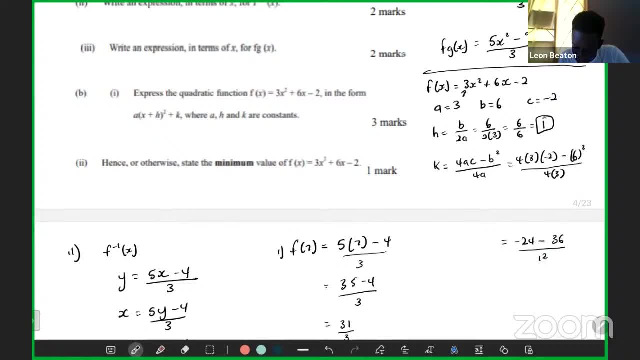 All divided by 4 times 3,, which is 12.. Somebody said the answer is negative 5.. All right, let's see So: negative: 24 minus 36.. All right. Negative 6.. Negative: 60.. Negative: 60 divided by 12.. 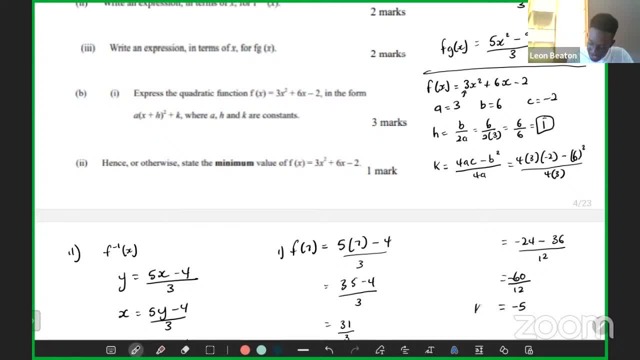 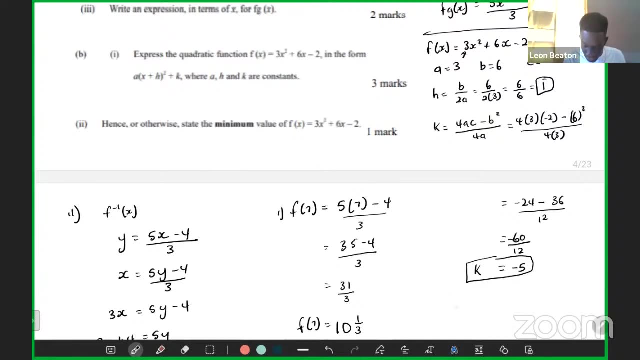 Negative, 5. Negative, 5.. So k is equal to negative 5.. So we got a value for k, We got a value for h And we got a value for a. Now it's just a simple way of putting that into this general form, which is a open bracket: x plus h. 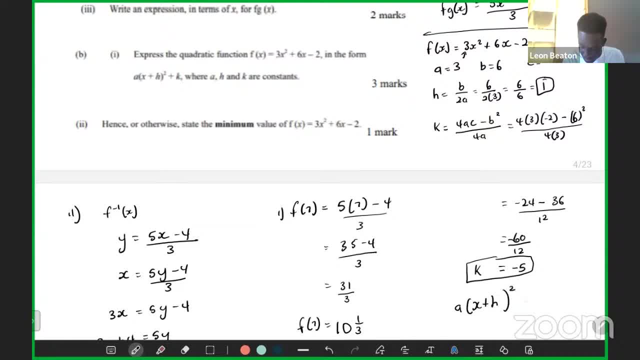 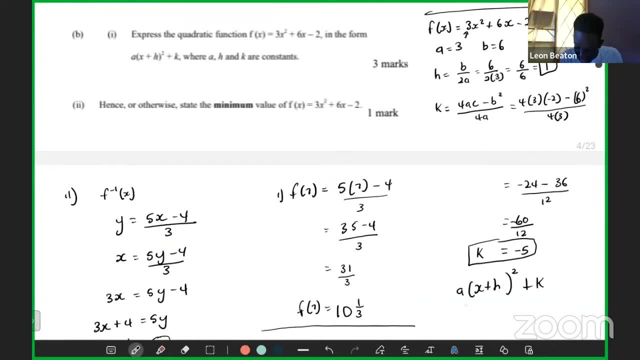 X plus h, squared plus k, So it's just simple to put in those things right. So we know the value of a is 3.. This would be 3, open bracket. We're not changing x. x is x, So this would be x. 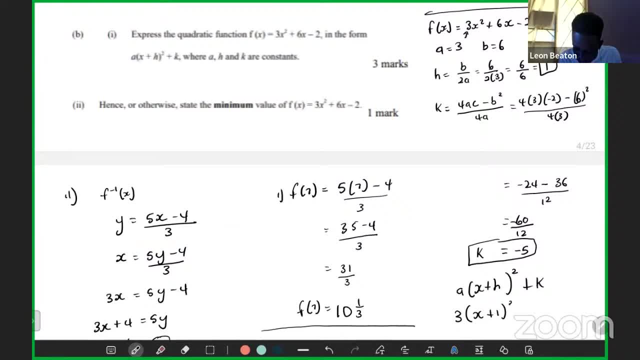 h is 1.. So x plus 1 squared And plus k, which is negative 5.. So plus negative 5. And we know these two signs will cancel out and give you a 5. Plus and a minus will cancel. 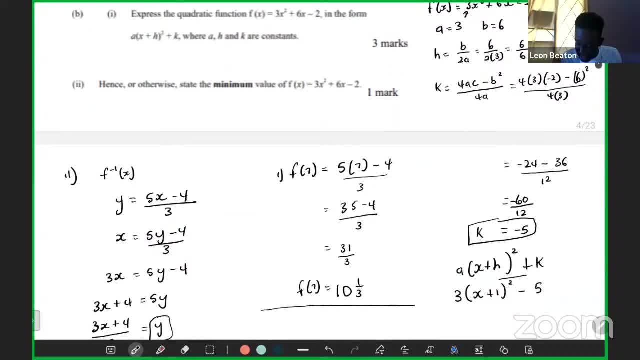 So it'll just give you a minus. So minus 5.. And this is our answer in that form. All right, So it's just a matter of remembering. I'm not a big fan of remembering formulas, That is what you know. for completing the squares, it's a good thing to remember formulas. 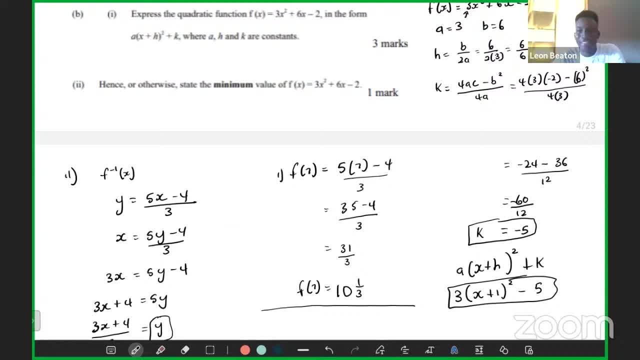 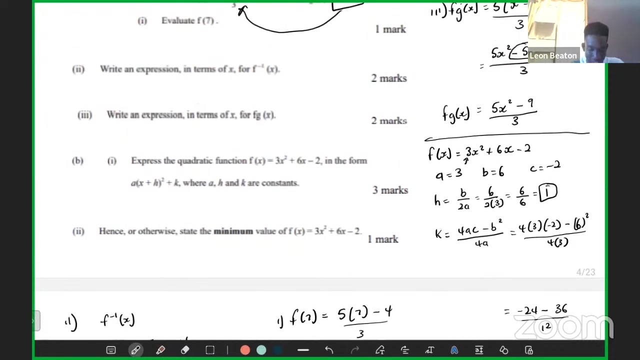 So write it down somewhere, Commit it to memory, Because I don't think this will be given in the exam. All right, So everybody go there, All right, Last but not least. Last but not least, The other question says: hence or otherwise, calculate the value. 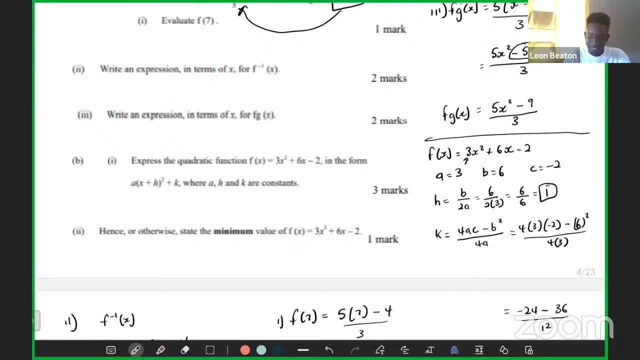 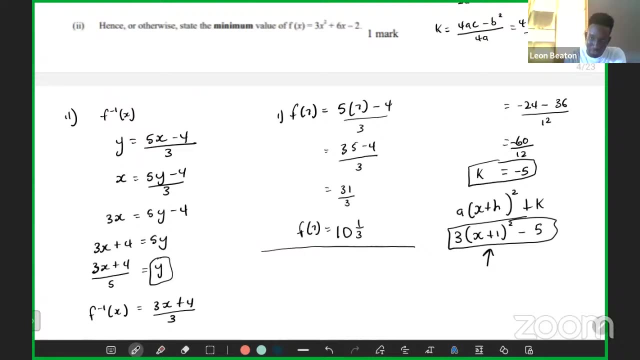 Say the minimum value of the function. Say the minimum Minimum value of the function f of x is equal to 3x squared plus 6x minus 2.. Say the minimum value of this function. So we have, we already have, the function in the form completing the square form. 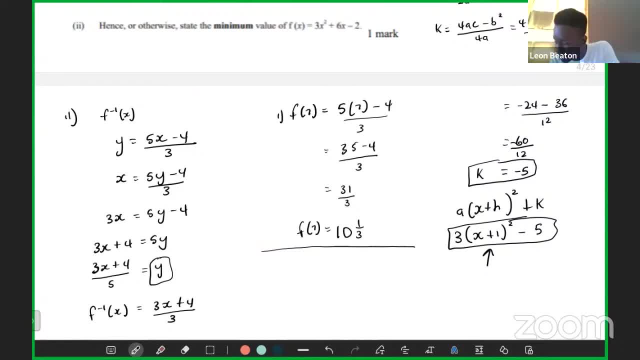 So how can we find the minimum value Anybody? how can we find the minimum value? Anybody remember? Sorry, the minimum value would be k, which would be negative, 5.. Negative, 5., Negative, 5.. So the minimum value would be k, which is negative, 5, right. 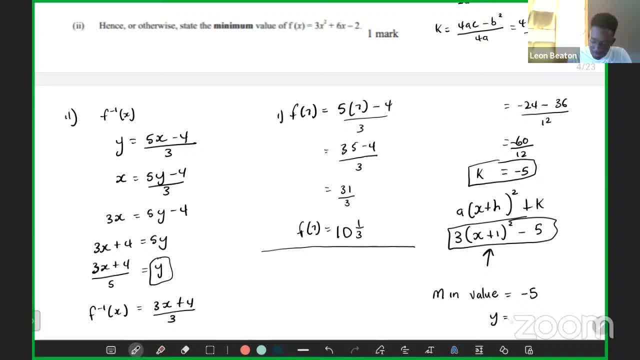 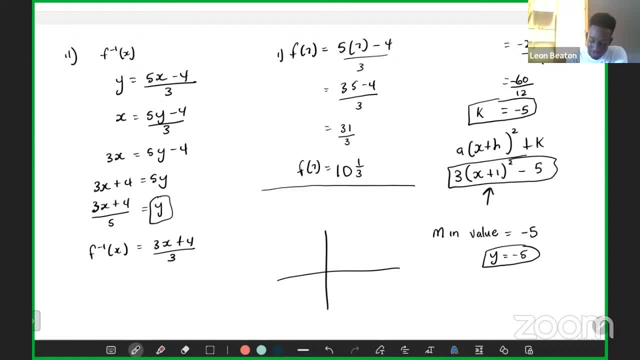 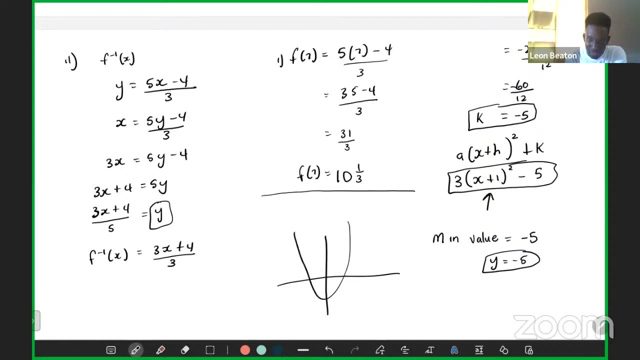 So this would be: y is equal to negative 5. That is the minimum value. Minimum value means when you have a quadratic function. So we know a is positive, So that means the quadratic will come something like this: So the minimum value is basically telling you. 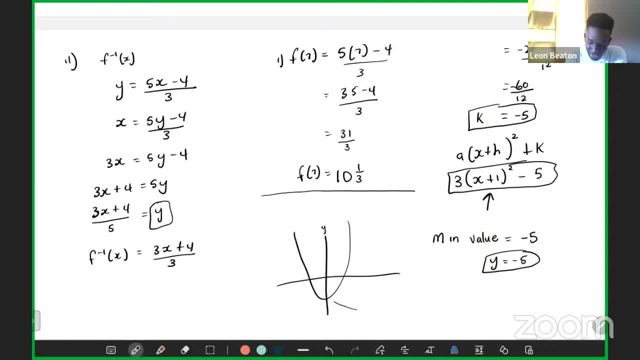 The lowest part on the graph. so this is the y-axis, this is the x-axis. So the minimum value is telling you the lowest part on the quadratic. So, and that is what that is why we have, y is equal to negative 5.. 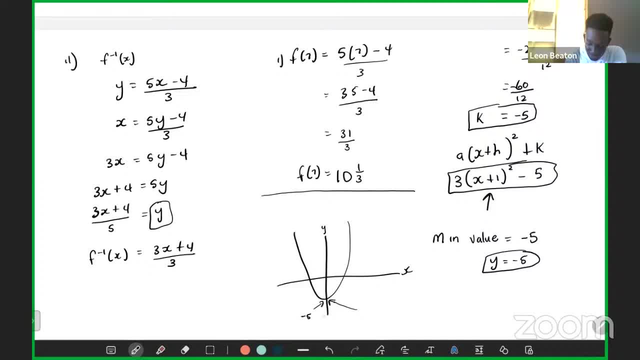 Because that is the lowest part on the graph right, Which is negative 5, right. So that is how we have y equal negative 5.. Everybody go there? Yes, sir, Let me see. Let me check out the Facebook. 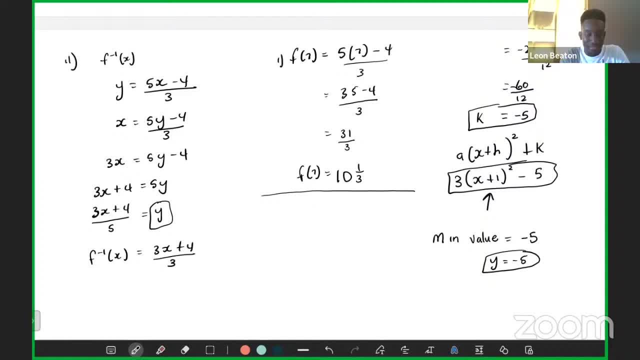 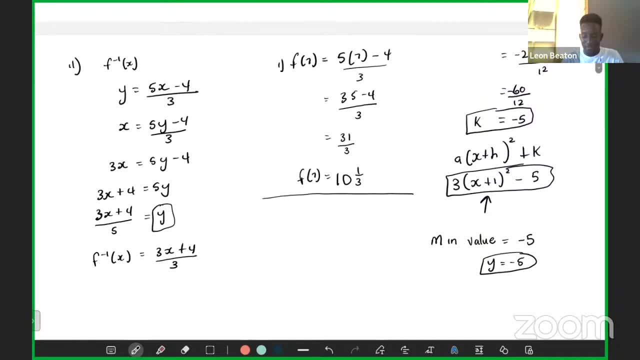 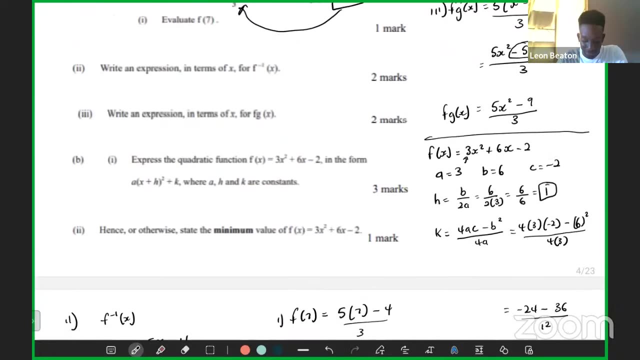 Let me check out the Facebook comments. Somebody said da da da And SQL, all right Anyways. so that is it for that one. Those questions can be challenging, right, And you have to write it in this form. 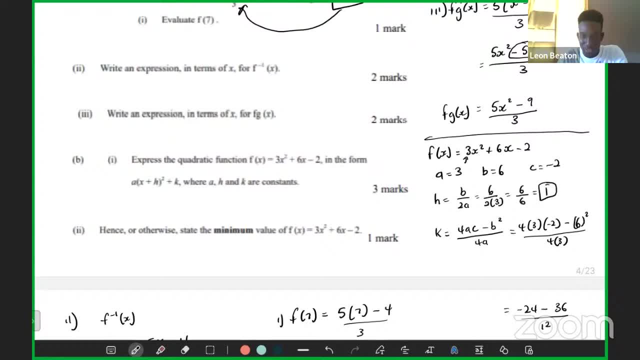 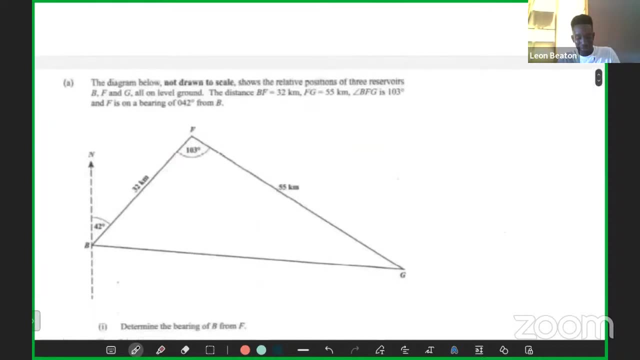 It could be challenging. I know, when I was in school I was afraid of these kind of questions, right? But you shouldn't be afraid. Very simple, right. Very simple, All right. So that was it for that one. So we're coming now from functions and quadratic functions. 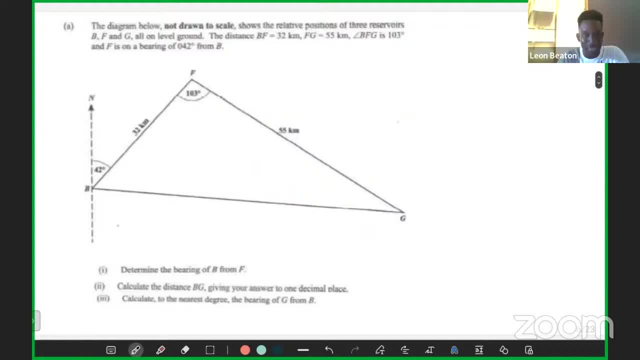 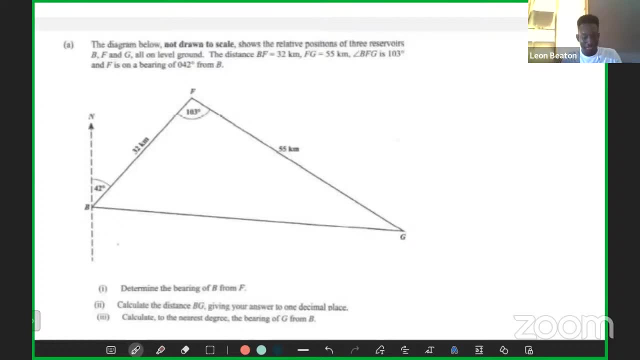 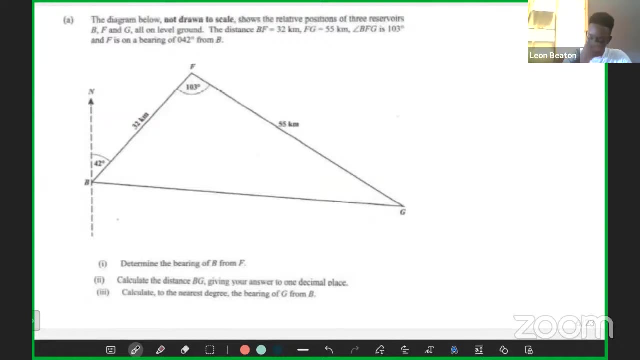 And we're heading into some, some, some, some, some bearings. How good are the bearings? Everybody solid with the bearings. All right, All right, let's go. So I I've been talking all the time, So let me get somebody to read the instructions here. 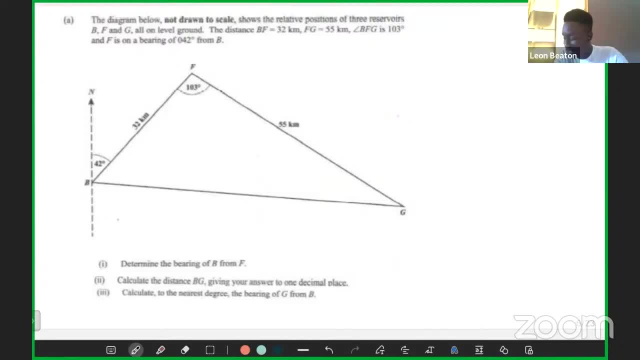 My throat is working. I have a few of my students on the live, So they will be working it along with me, because it will be a lengthy life And it will be very challenging to do it by myself. So I have my students here to keep me. keep me at it. 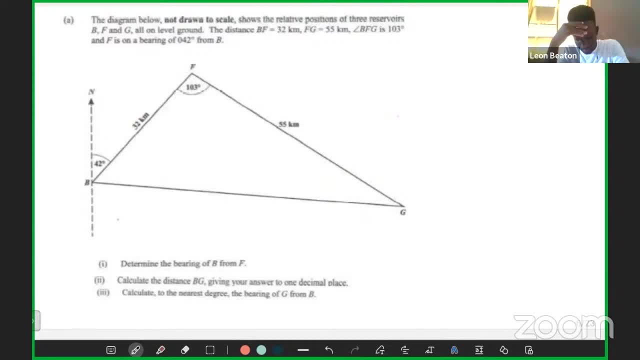 Anyway. so yeah, somebody read it for me. I'll go, sir. Yeah, go ahead. Okay, All right, I need some more, let me sleep a bit. So yeah, we have a few more. So I have a few more over here. 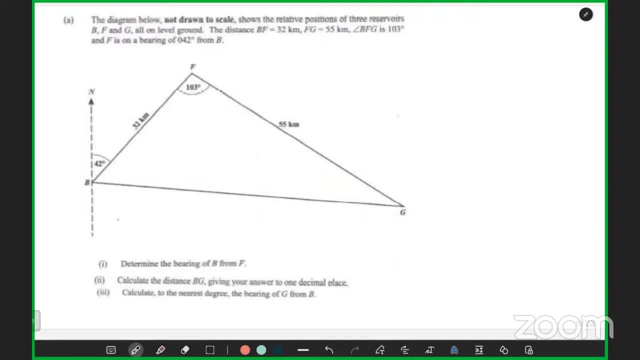 I also have a few questions for you, So let me talk about this one. So I have a question for you. So I'm going to do the math, maybe like an E and a business class, What do you do? So I'm going to take the math quiz and run. 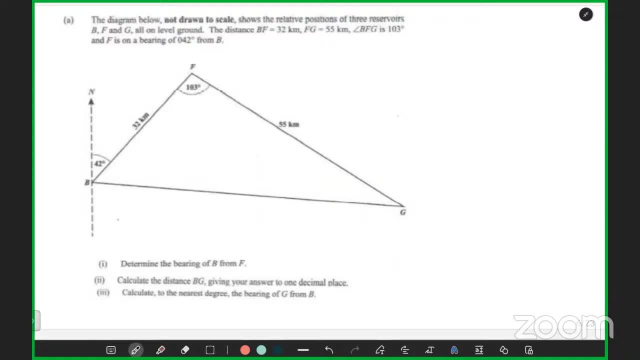 I'm going to run it by using the time and distance to see the Chloe and the other questions, And then I am going to take the math quiz. I will take the math quiz And then I'll show you how to do that And it will be the math quiz and you will be the expert. 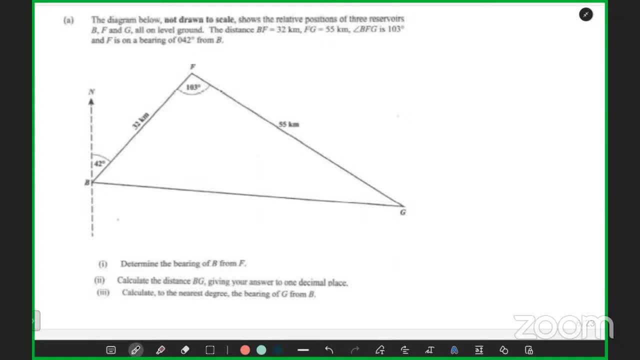 So I'm just going to take the math quiz. I will do it by using the time and the distance: three degrees, and f is on the bearing of zero. 42 degrees from b. excellent, all right, thank you very much. good, so it's basically explaining. i want to read these kind of instructions carefully. 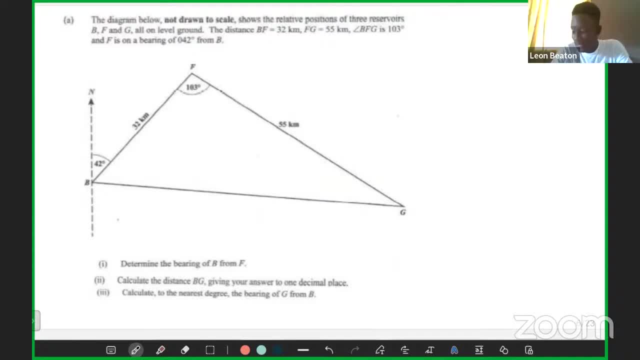 read it twice and understand what is going on in the diagram. a big misconception that many students uh make is to just browse through the instruction, the instructions. they are not there to you know, as the operation on the page right. we're actually there to guide you, um, to get your answer and 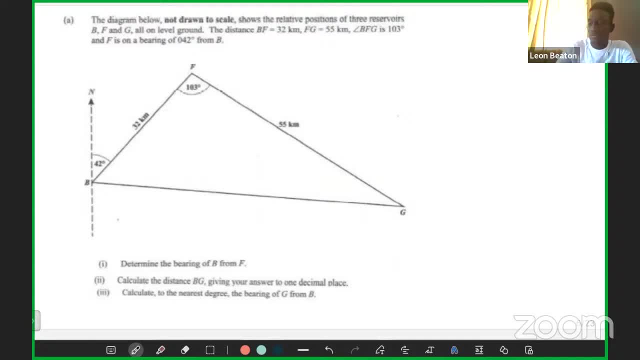 you know any question that cx said they will not leave you to make any assumptions. any assumptions that you got to make wouldn't be assumptions, would be things that are proven, so you should not be looking at that. oh, this angle look like this here. all right, so this got b. this angle look like 32. 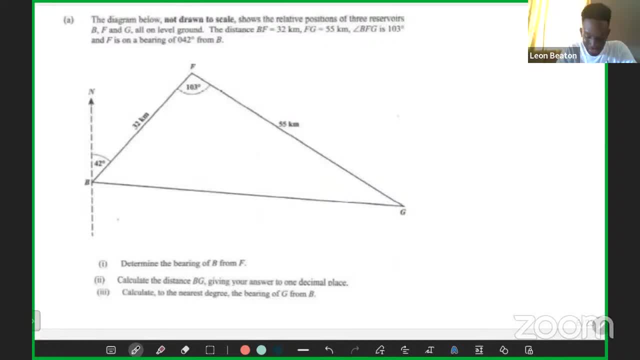 so you'll be 32.. i know they will tell you everything that is going on in the diagram anyway. so determine the bearing of b from f. so you want to determine the bearing of b, which is here, from the point f, so from this point. uh, anybody could tell me what is the important thing when you're dealing with? 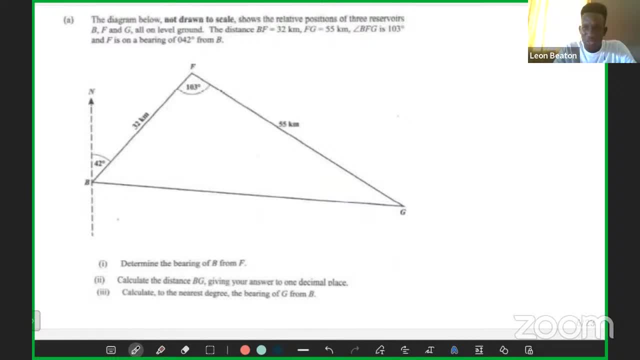 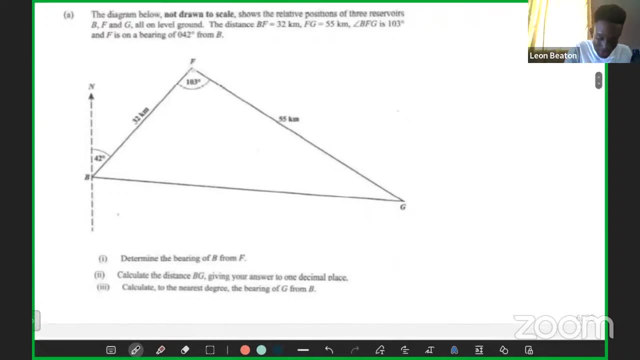 uh, appearance. what's the first thing you want to do when you want to take a bearing of an object? what line is important? an art line, right. the first thing i gotta do is get in art line excellent. so we gotta draw in an art line from f. 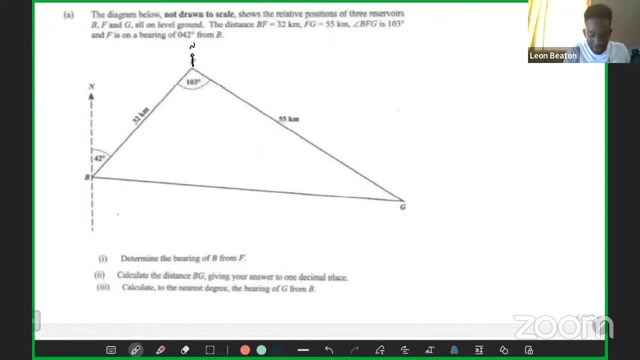 we draw an outline from f and then we want to take the bearing from here. we go all the way around to the b, which is here all right. so how can we find that bearing? how we use? what mathematical relationships can we use to help us to find that bearing? 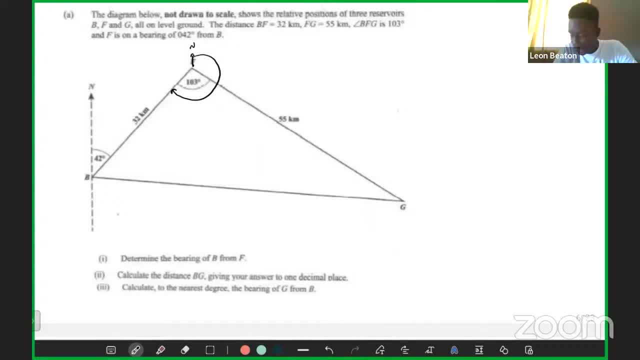 by the way you go, clockwise or counterclockwise. i read clockwise. what mathematical relation can we do to find that bearing? nobody could remember. so yeah, we find for f by um minus 1, 42 from 180.. you're correct. excellent, that will give us this pc, right. what is the relation between those? 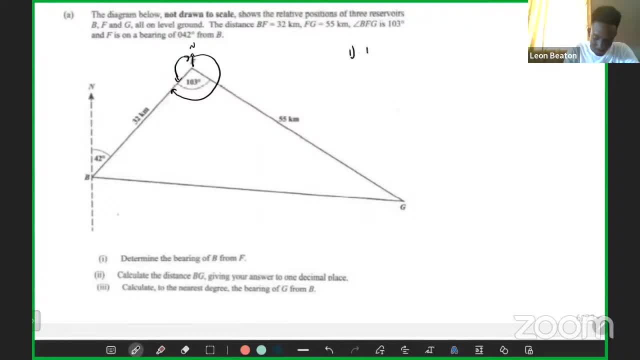 two. there are two. um yeah, go ahead, um sure, because it's a quarantine angle and quarantine is equal to 180 degrees. yeah, they're supplementary, right, so it's 180, okay, subtract 42 degrees. 180 subtract 42 would give us what 138, 138 degrees 138 is from here to here, and we know from here to here is 103. 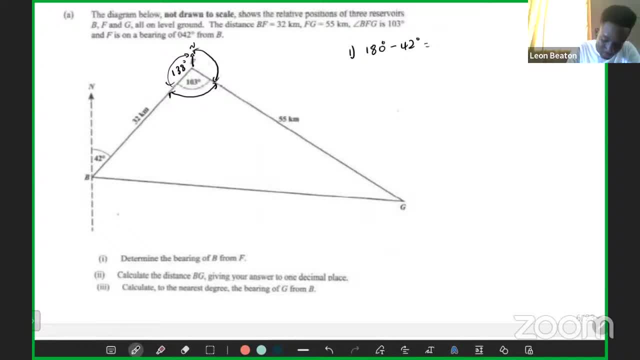 so what else can we do to find from here to here, sir? 360 minus 138 plus 103.. so 360 minus one, or why are you always 360, though? how do you know it's 360.. why am i just in 360.? 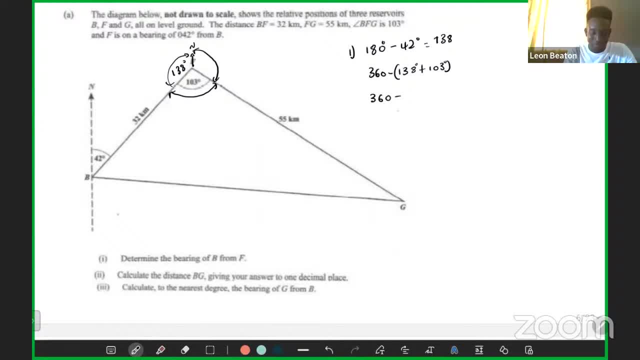 you're correct, right? anybody? great, why do you mind that's 360.. sorry, because the circle is equal to 360 degrees. yeah, it's a circular form. they're right the way around. yeah, somebody's saying anything about the circle, right? so 138 plus 138 plus, uh, 103 would give us. 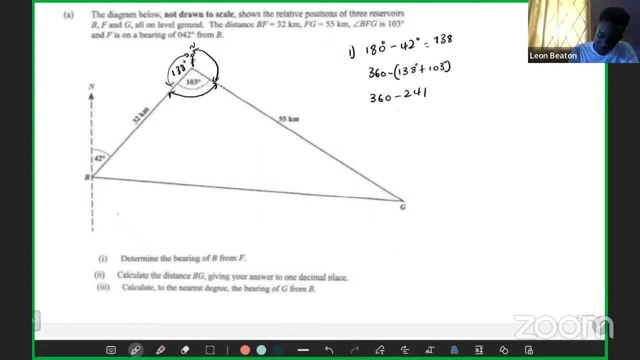 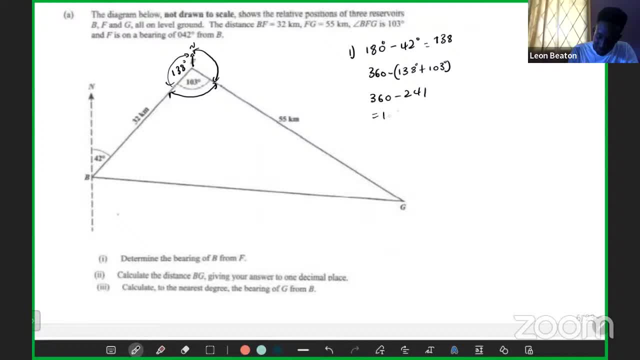 give us a value of 100, 119 degrees, so 119 degrees. 119 degrees, so the 119 degrees. um, that is from here to here. so the beer not to be the bearing, so we can say so. how can we say the bearing of? so, how can we say the bearing of? 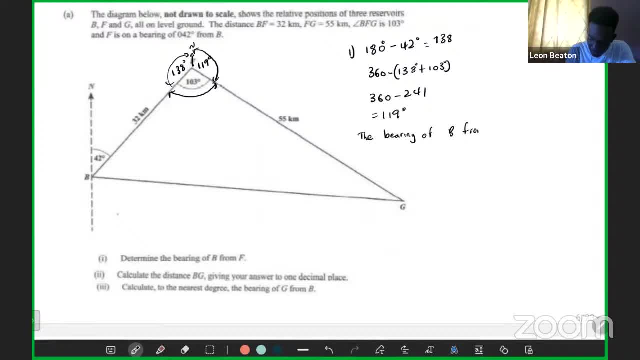 if we're achieving all of this shall be granted. then a Self one 19 plus one or three, one 19 plus one or three that we want all the way around here. so one 19 plus 103 and that would give us a value of 222, 222 degrees. all right, this went for about一個. 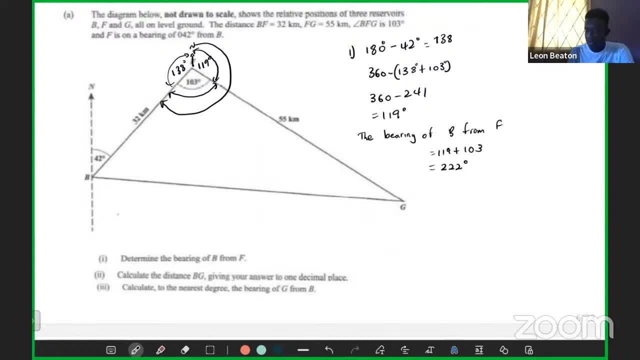 hundred and twenty-two dollars for about, I think, three marks. so, parents, you start from the north line and you go all the way around to the line that you are fine, right, and a bearing of something from, something from where you want to measure from, that is really. 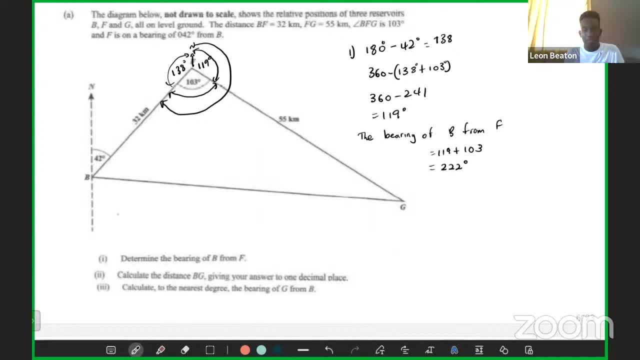 under has to be from something you go all the way from right. so the bearing of B from F, you gotta start from it. all right, good, so that was number one. number two: calculate the distance. so let me erase all this one. so calculate the distance: BG. given your answer to one decimal, please. so you want to find G, BG. 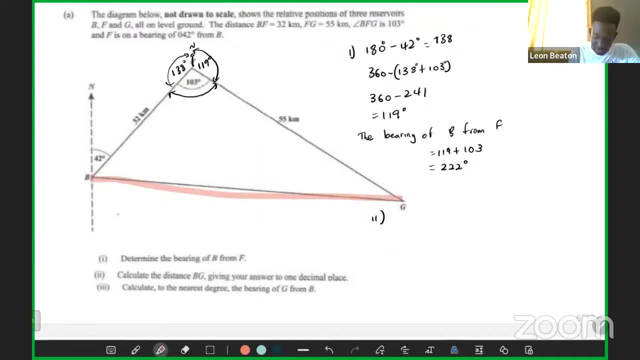 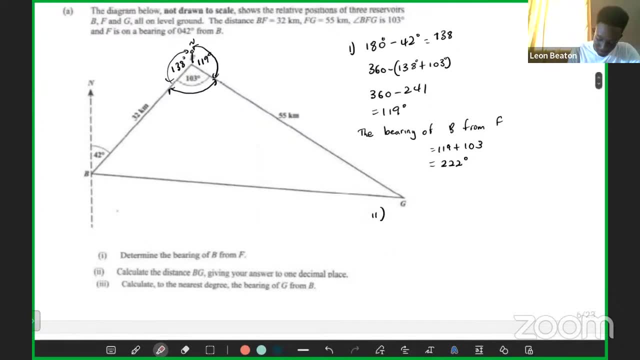 BG, which would be this line here, right to one decimal place. so what can we do there? what can we use? BG, which would be this line here, right to one decimal place. so what can we do? BG, so I could use the. on the cosine. cosine rule was the cosine rule by the. 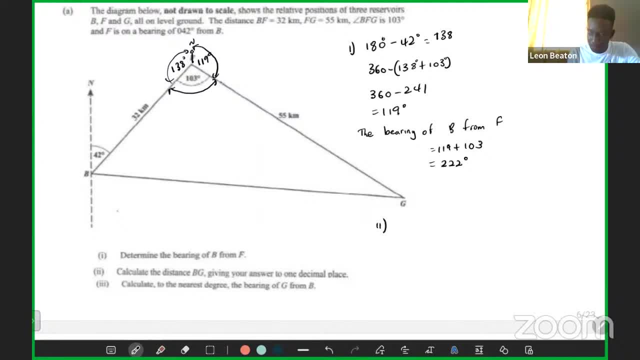 will give me cosine rule is the cosine rule, sir. a square is equal to B square plus C square minus 2 PC. cause a. it's crazy what. the B square minus 2, 2 BC times, cos times, cos you know, the side is a. now, this is this, is a, this is a form that I would give. 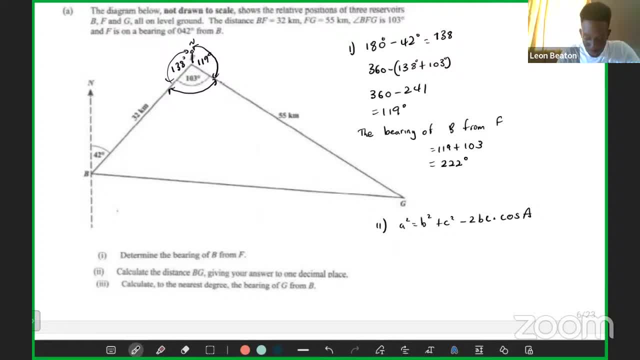 you. they will give you any existe right, but we must understand what is forming it. seeing, of course, you don't have B and a, B and C s. well, you have B, f and G, so let's try to use the letters that we are given here to put in the form: a creator. 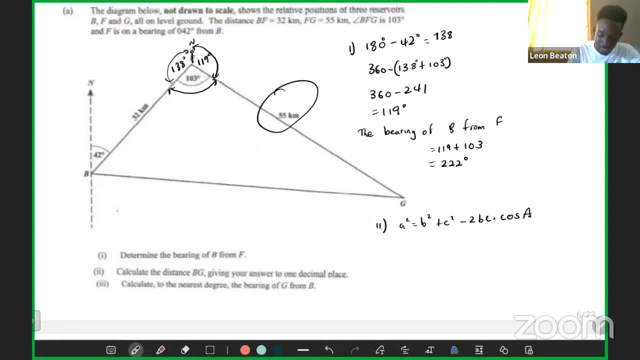 Say: what would be this? sorry that angle here. So what would be this side here, Common B, Common B And what would be this side here, Common G, Common G, And what would be this side here, Common F. 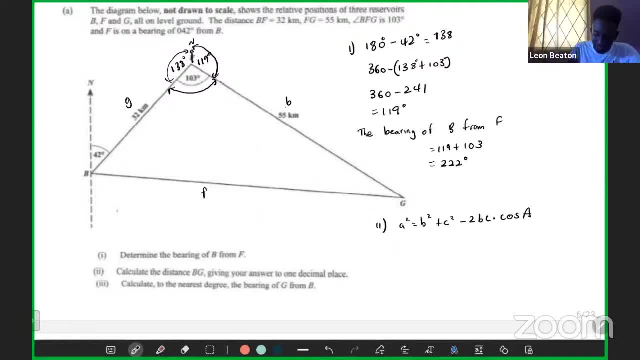 Common F. So you want to find the side F and you're given the angle F as well. So we can say: instead of A square you can say F square is equal to and the other two sides, which would be B square plus G square minus two. 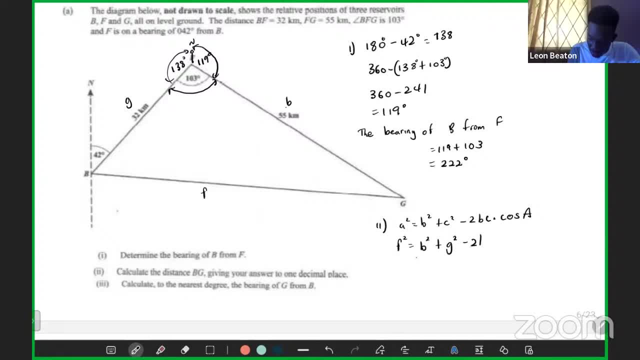 these two same letters to BG multiplied by cos, the angle, cos F. All right, Whatever is the side here, you got to get the correspondent angle to that. Now we can do some substitution So you can have: F square is equal to B square. 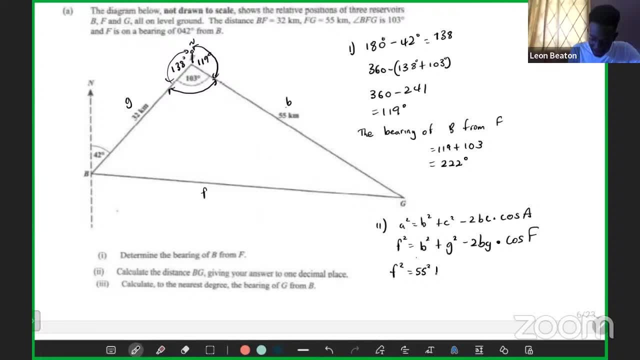 which would be 15.. So 15 to 5 squared plus G squared, which is 32.. 32 squared minus 2 times B, which is 55, multiplied by G, which is 32, multiplied by cos F, which is cos 103.. 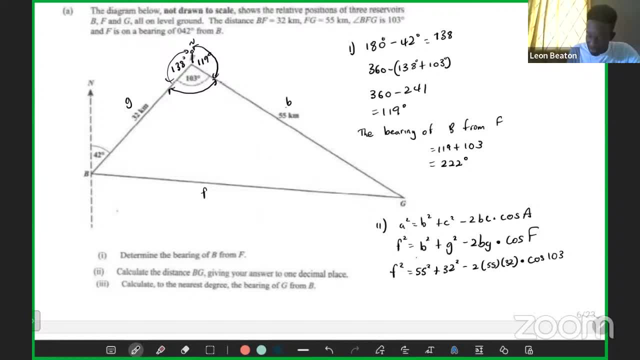 And now it's just a matter of doing some simplification. This would be: F square is equal to, so work with this piece of me. F square is equal to B square plus 32 squared 4,049.. Can you work with this entire thing? 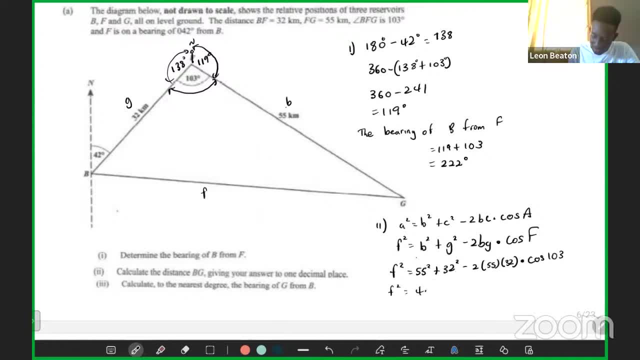 Yes, sir, All right, So 4,049.. 4 to 9.. 4 to 9.. All right, Minus, let's multiply 2 times 55 times 32.. 4 to 9.. 2 to 12,, 2 times 55 times 32.. 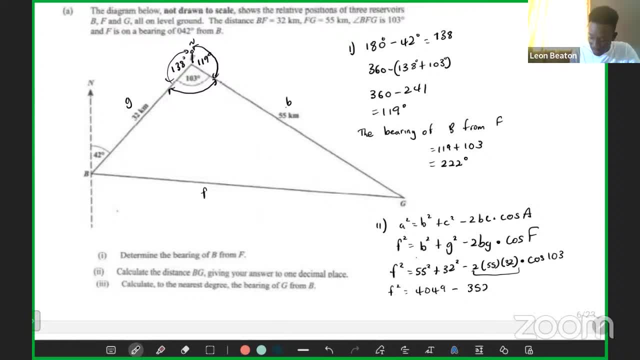 Well, that give us 3,520. 3,520. 3,520. Multiplied by cos 103.. So let's multiply our answer by cos 103.. So 3,520 multiplied by cos 103.. So by cos 103.. So we have 50,000.. Well, 3,520 times cost 103.. So that does that. that number which you have, yeah, easily죽ila 전onner Voronkingi- is 1%. 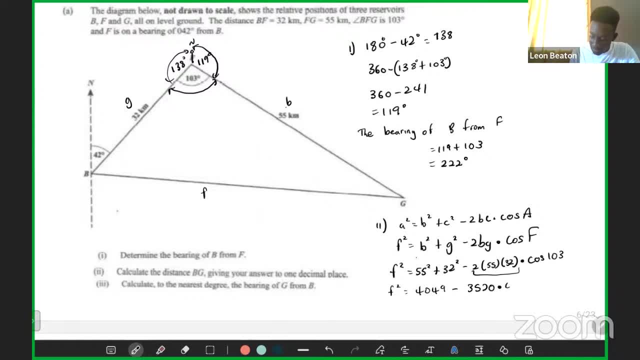 At the same time you should do multiple Ryerson addition of Afriendly Stewart, addition to your, across all the original numbers and that should give us, that should give us 4,049. subtract and multiply this piece here by cos 103, we should get. 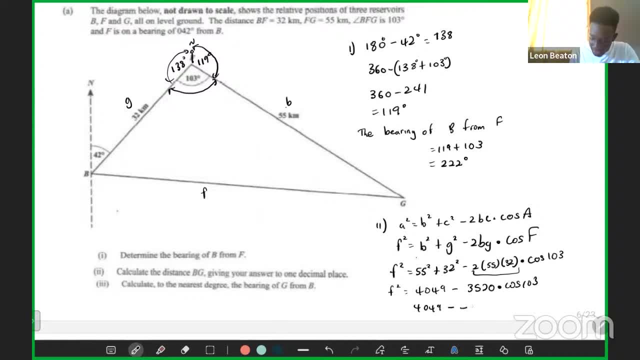 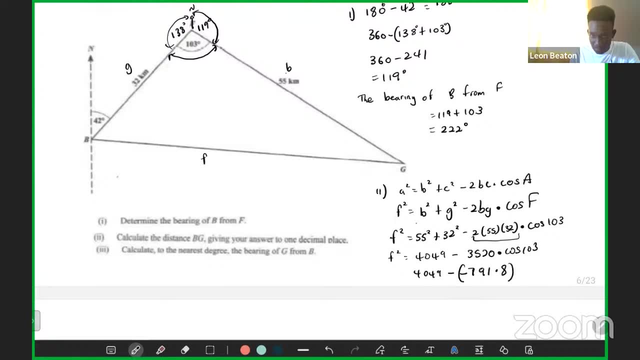 negative 791.8. you all got it. yes, sir, this is equal to F square. so F square would be equal to to the minus and the minus that would become plus. so we have 4,049 plus 709 to 1.8. how does that give us? 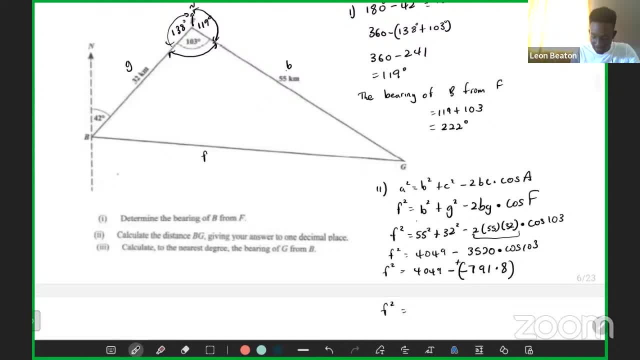 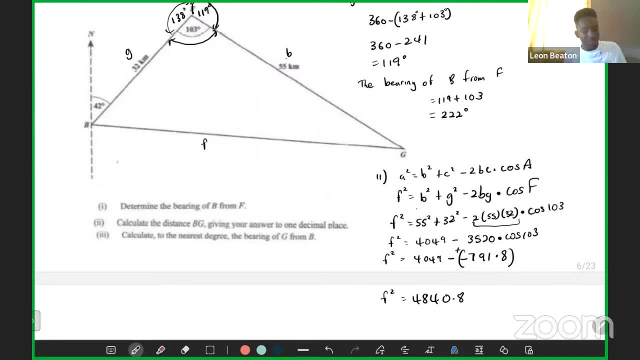 that should give us a value of 4,840.8, 4,840.8, alright. and of course we're not done there. we don't want to find the value of F square, we want to find the value of F, so we gotta take over the square. 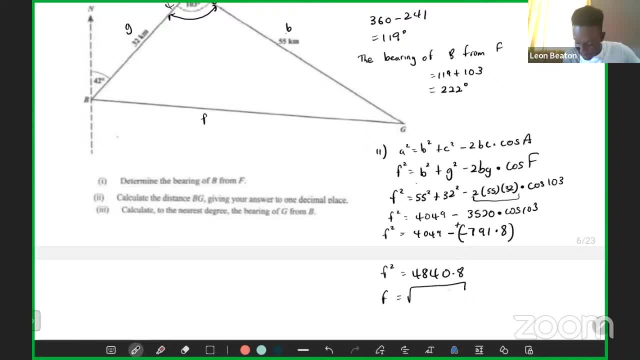 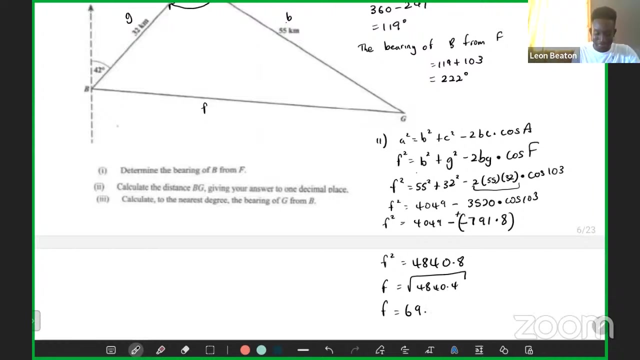 so this will become: F is equal to the square root of 4,840.4, the square root of that. so we take the square root of that, we'll get the value of- sorry, 69.5, 69.5, you sure 69.6. 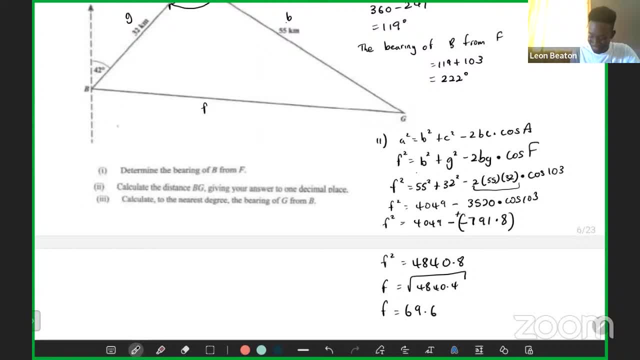 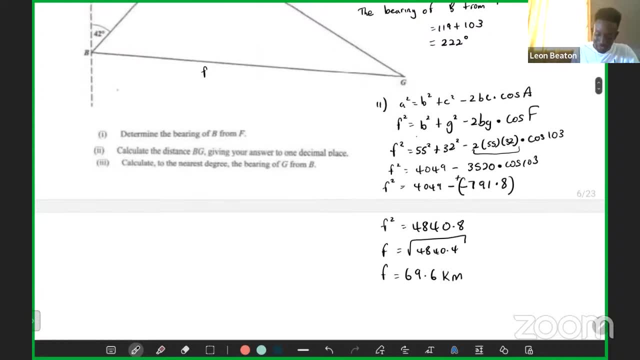 alright, 69.6, so 69.6 KM. alright, and that is the distance. so again the thing is, they told us to find BG, right? I mean, we know F is BG, so let's just leave anything for granted so we can say BG is equal to. 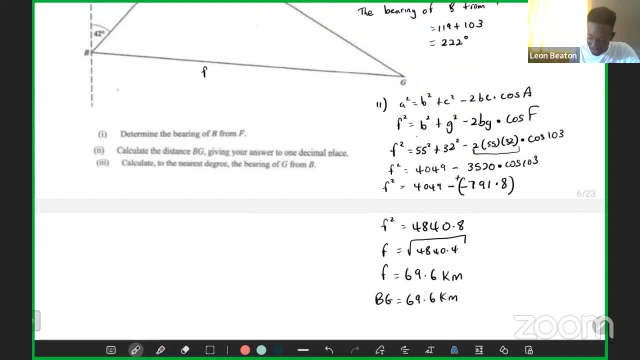 69.6 KM. right, and we leave that as our answer. let's see what's going on. everybody got there. let's see what's going on. let's see what's going on. yeah, so it's just a matter of substitution. now the thing about the 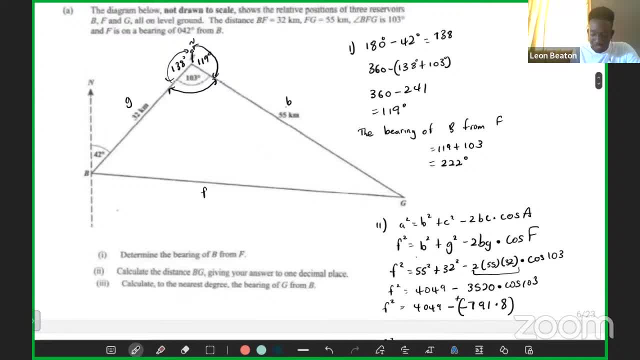 the cos, the cosine rule, um. use the cosine rule when you're given two sides and an angle right, and it depends on which two sides and which angle you're giving. if the side that you want to find, in this case here, and you're giving the 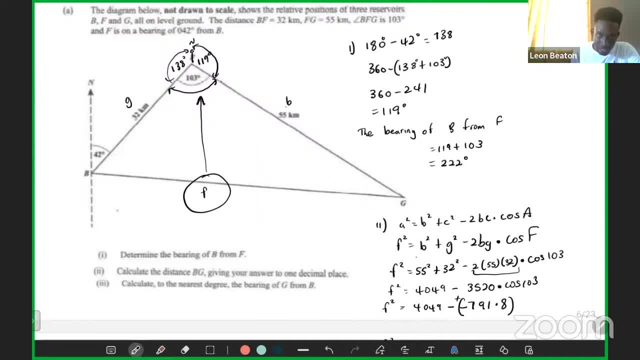 corresponding angle to that, the opposite angle, and you're giving it two sides here. that's where you can use the cosine rule. we use the sine rule now when, um, you're not. you're given similar things, but not in that order. right, in order to use the cosine rule. 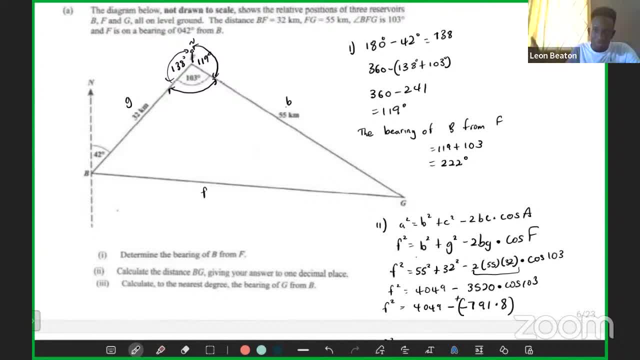 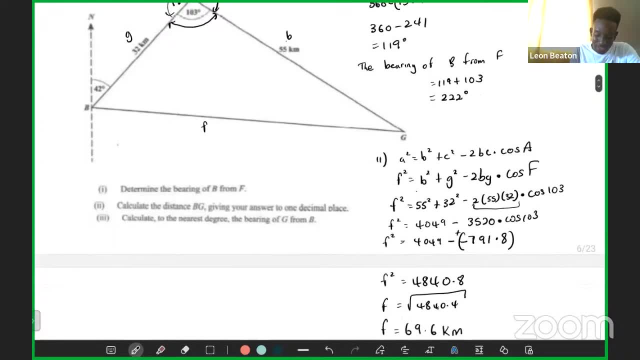 you must be given three out of the four things. because you want to find for one right, you must be given three out of the four things. and in algebra, in maths and so on, any formula that you're given, uh, whatever, whatever are the the values that you gotta? 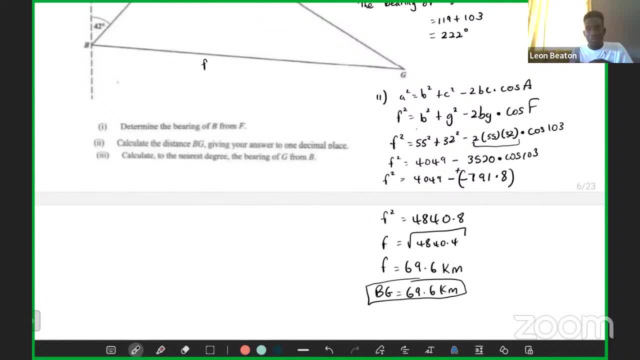 substitute in the formula you must be given. only one thing must be missing from the formula, and you can find that one thing. it doesn't matter the order of the formula. as long as one, one part of the formula is missing, you can use that formula to find for it. 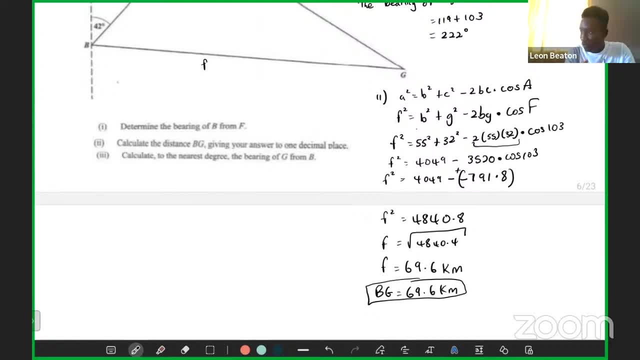 right, that is the key. you can't have two things missing and use the formula to find for those two things unless the two things got the same value. but yeah, so you know that's what you gotta be on the lookout for. you must be given. only one thing must be missing. 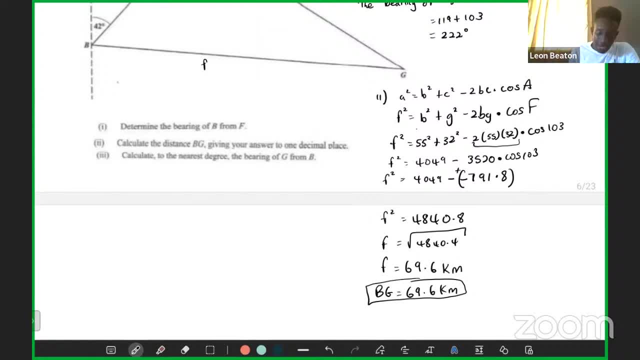 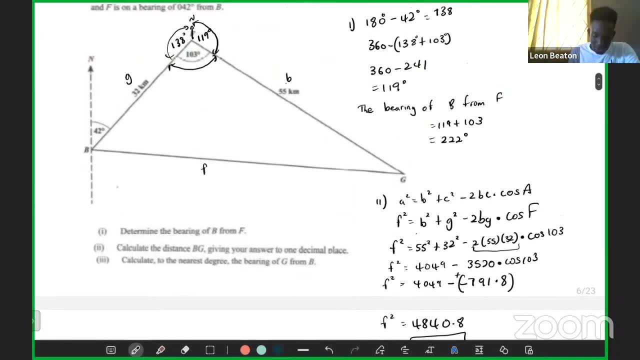 from the formula or any formula that you want to use. all right, so the next one: calculate to the nearest degree the bearing of g from b. the bearing of g from b. so the bearing of g. now, this is a part that many students mix up: the bearing of g. 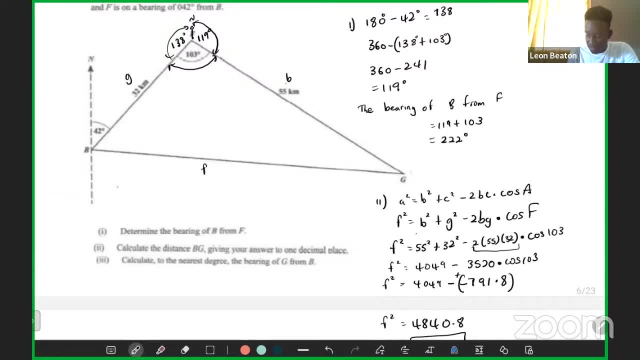 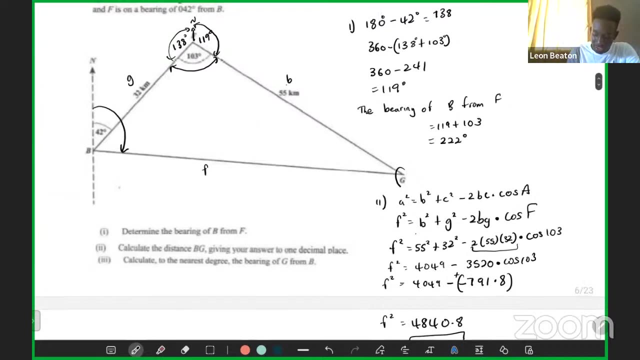 from b. so from b would be here. so you want to find this bearing. many students would go and they would do this, so from b would be here. you go and draw the north line here and then they go all the way wrong. that's why no. the bearing of g. 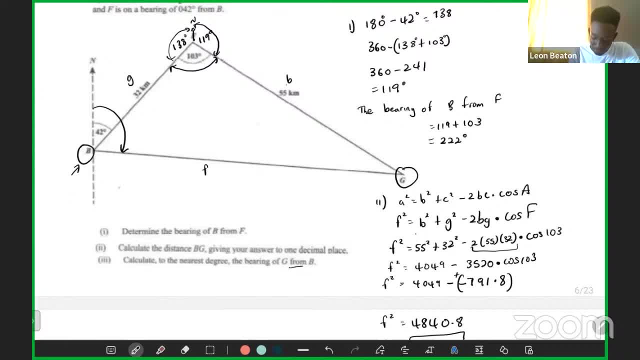 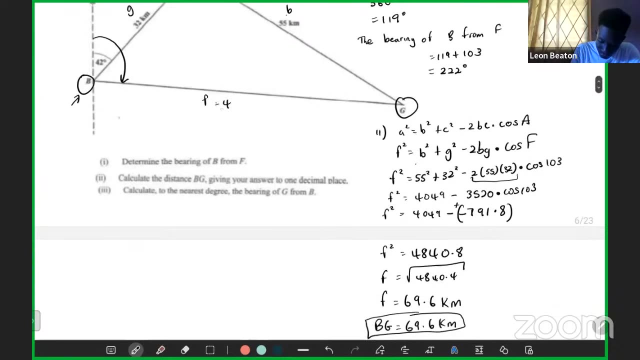 from. b right keyword there is from. from is where you're measuring the angle from. so what can we do to find that bearing? so let me write on this side. this side is equal to 69.6 km. you can use the cosine rule again. use the cosine rule. 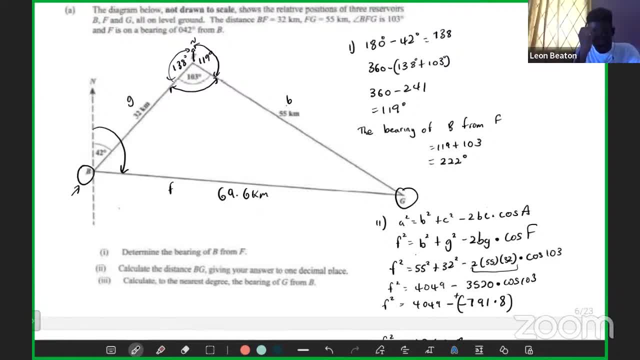 you want to use the cosine rule. any other easy rule you could use. make one, any other rule. start a sign. you can use a sign as well, because we're given three sides and an angle that we want to find. we're given all three sides of the triangle. 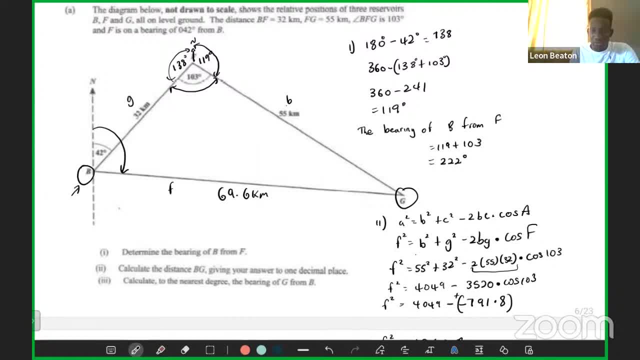 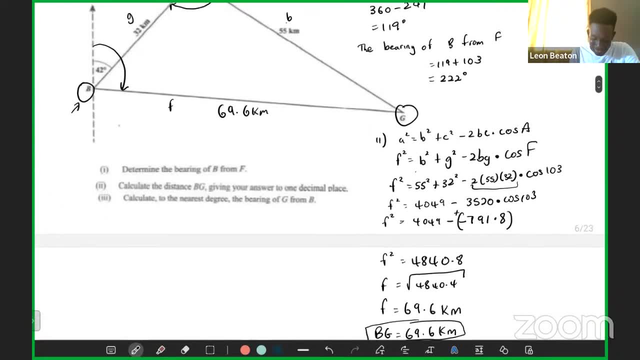 and an angle and we want to find an angle. so we can use, or you can use, a. I think I can use the cosine rule as well, but the cosine will be a bit longer, right, so the sine rule is shorter easier, so let's use the sine rule. 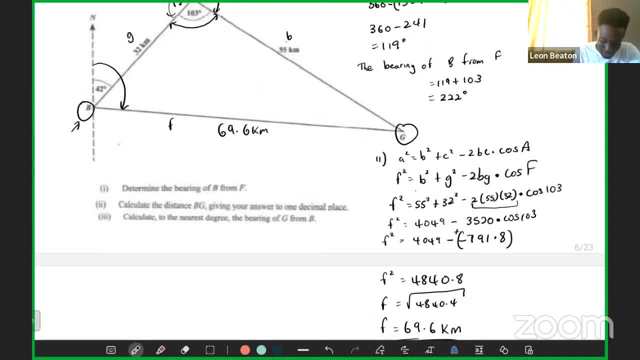 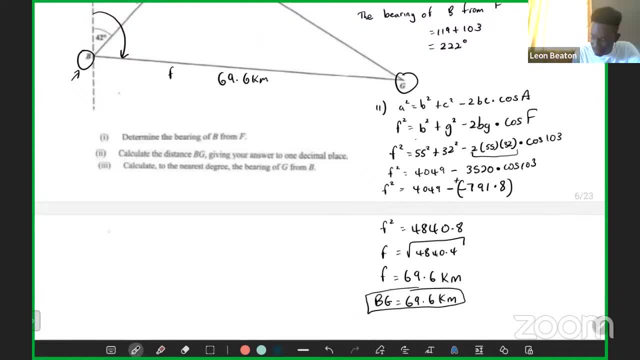 so you want to find angle b. so what is the cosine rule? what is the sine rule? again, what is the sine rule? I can't remember. help me out. start. a: divided by sine, a is equal to b. divided by sine, b is equal to c divided by. 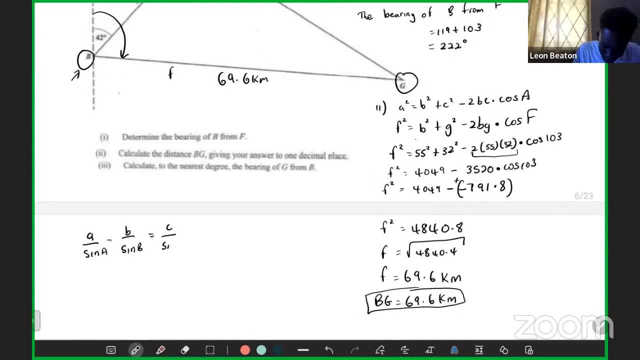 sine c. yeah, a divided by sine a, sine a would be the angle, so that would be the big a and b divided by sine b, angle, again at the bottom, and c divided by sine c, right, so yeah, but of course this is it in its general form. 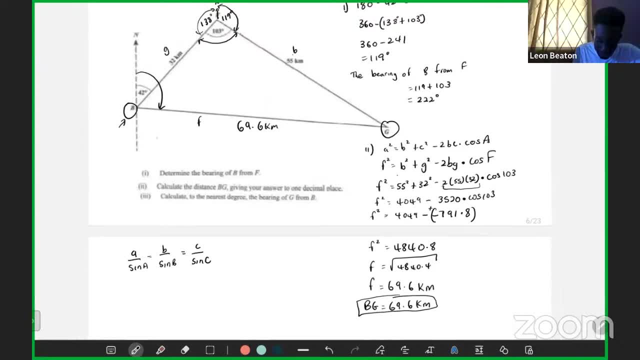 we can use the letters that we are given angle b. so let's say b divided by sine b is equal to. we can use any, any pair, any combination, any pair of the equation. we can use these two. we can use these two. we can use these two. 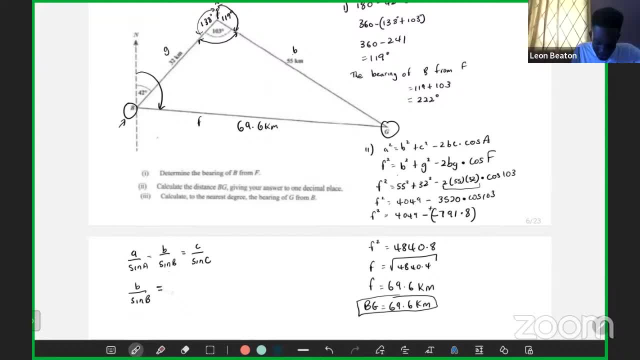 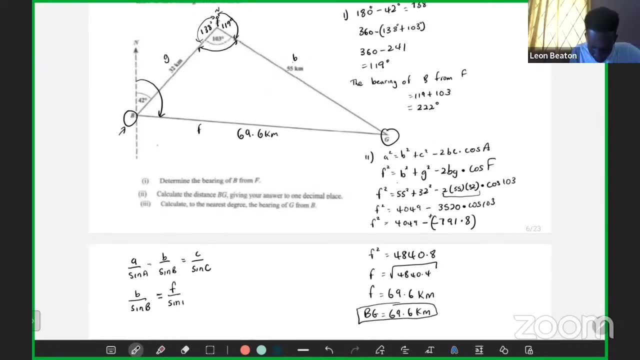 it doesn't matter. so b sine b is equal to. let's see, since we are given f, so we will do f over sine f, right? this is the angle f, and we are so the side f. now, this is the side f and this is the angle. 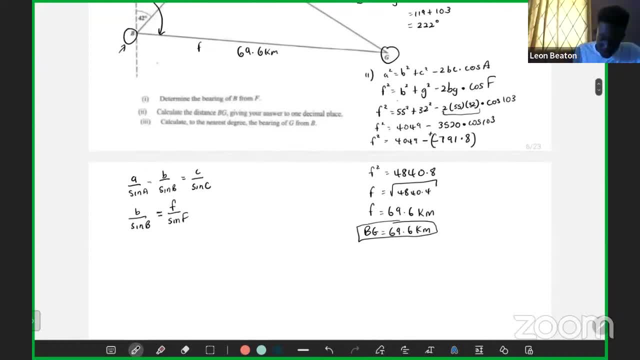 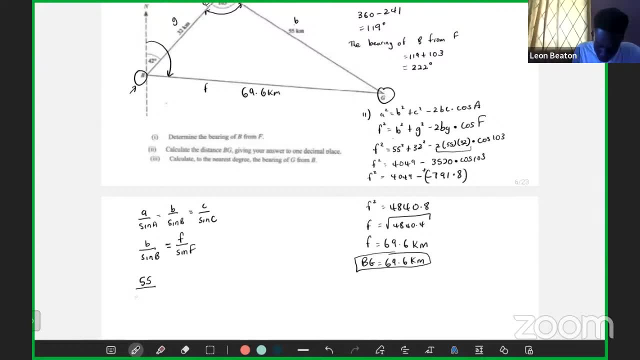 f. so we gotta use those two combinations. so b would be- let me zoom out- so b would be side b. side b would be 5 over sine b would be the angle that we want to find. so sine b, which is this angle here, this angle we find it. 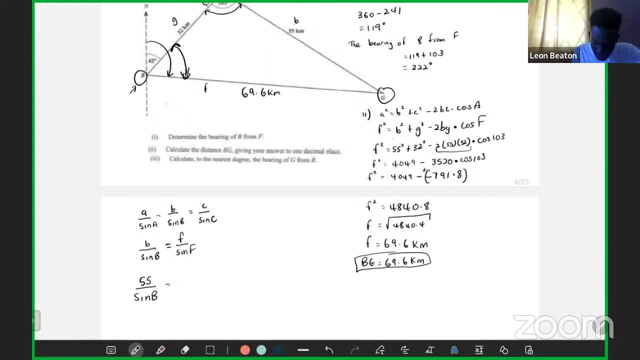 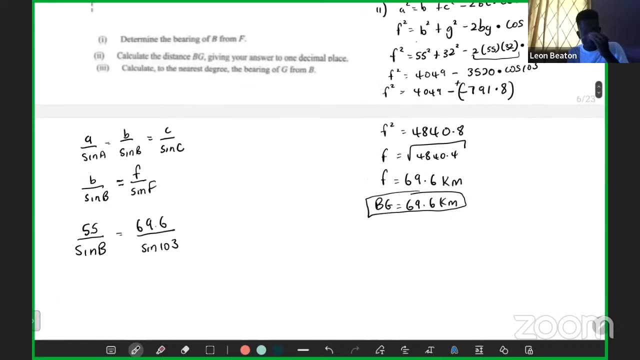 by the way, right side, this is angle b, so f. so f would be 69.6 divided by sine f, which is 103. and then we know. let me ask what? what can we do here to help us to find for angle b, as you can see, 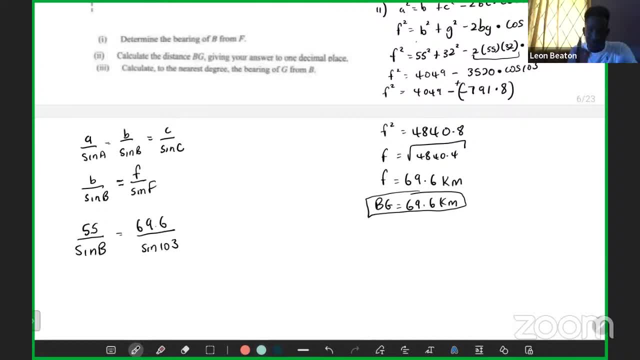 we just have one unknown, right. so that is what that is what you want to look for in the. that is what I want: to make sure you have one unknown alone. you can't just be one unknown only. so what can we do? so we cross multiply. yeah, we cross multiply. 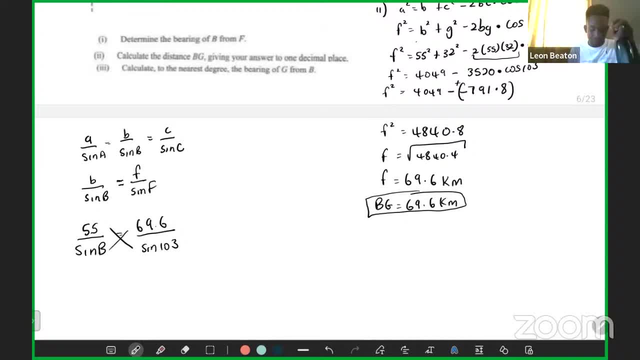 you cross multiply to help us find for b. so we cross multiply so we can have 69.6 multiplied by sine. b is equal to 55 multiplied by find, 103. and since we want to find for b, this 69, this 69, this 69. 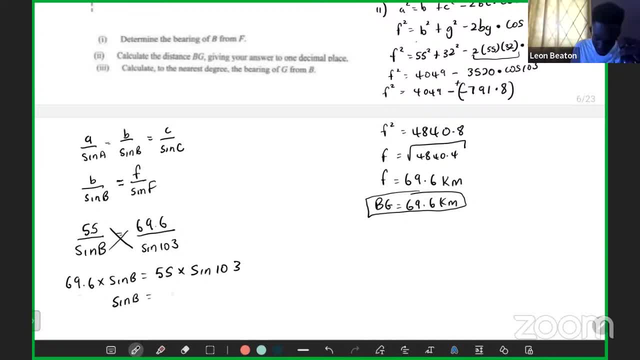 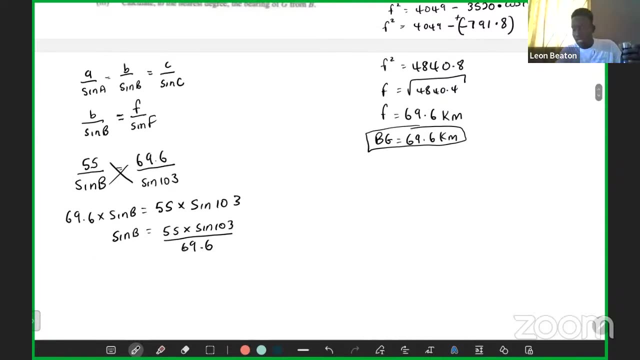 when we take it over to divide, we'll have: sine b is equal to 55 multiplied by sine 103, all divided by 69.6. and we use our calculators to simplify this. use our calculators to simplify this. to simplify this, We'll take this: 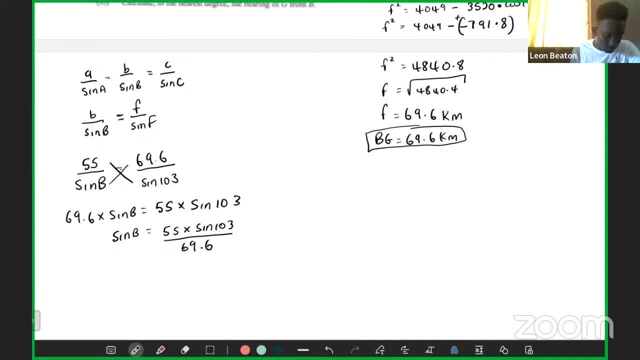 and then we take the. let's use four. zero point, zero, six. you sure, zero point, zero point, zero point, zero, six, you're sure, sir, zero point seven, six, nine, but i think i'll be zero point seven. all right, let's use five decimal, please. let's use five. let's use five. zero point seven, six, nine, zero point seven, six, nine, nine, seven. 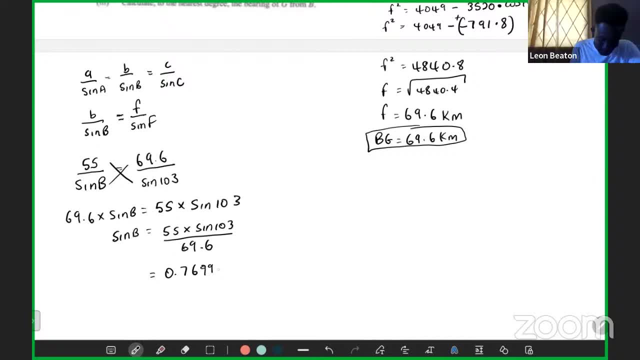 nine, nine, seven. you shouldn't be seven, nine, nine, eight, good, excellent, um. check this. make sure your cathlete is in degree right. make sure your cathlete is in degree. if it's in radiance you you will get um some issues there towards somebody, god, just now. so make sure you can't lose the degree. check. see my degree. 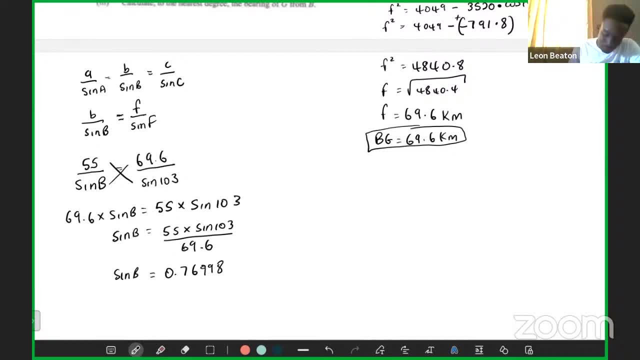 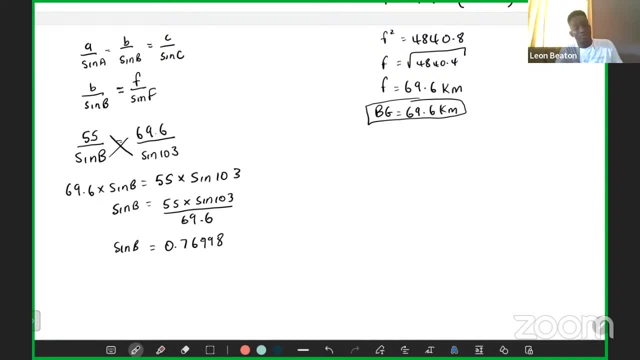 and you can't plus and them things in this. so it's a degree and sure you got this. in degree you will get something different right? so make sure before you go exam, make sure you, you know you take a point or you, or your pencil and you. 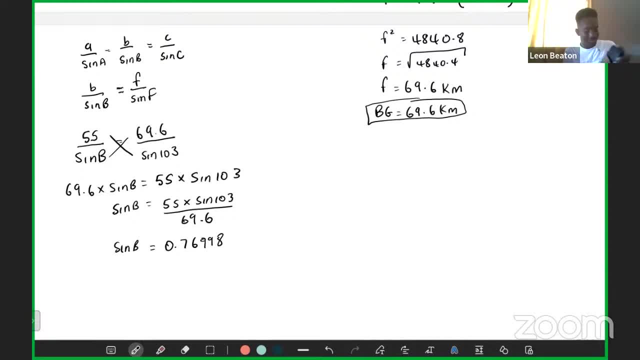 click that reset button because you don't want to lose marks, because or or you're, you're working and typing and checking and you realize at the end of have five minutes remaining to realize a calculator was in radiance. it'll be a terrible situation to be in. 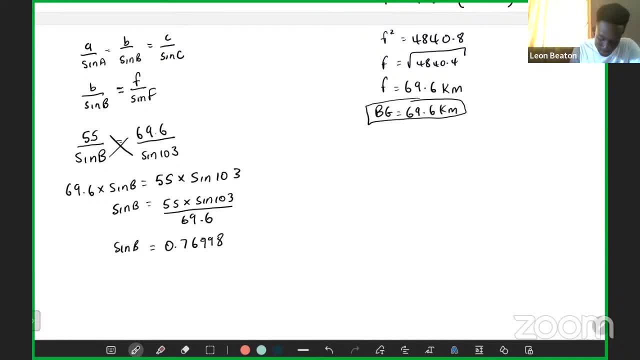 so to find for um b. now we say b is equal to- let me take over side- it becomes sine inverse of 0.76998 and so b would be equal to. i take sign inverse of this. what do we get? so b, there's zero. so um b thing. 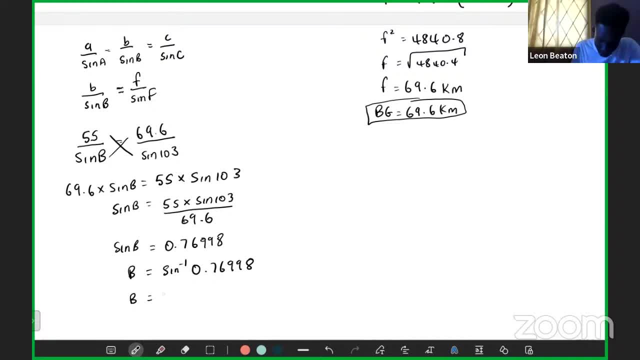 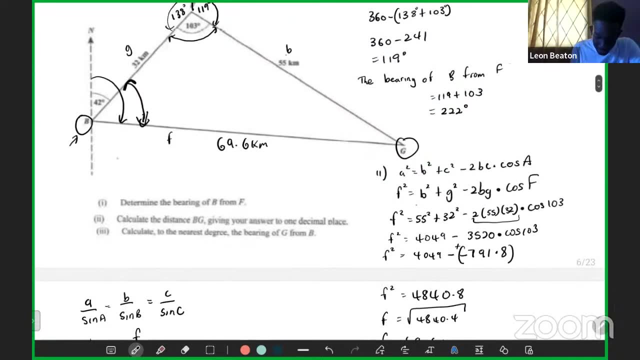 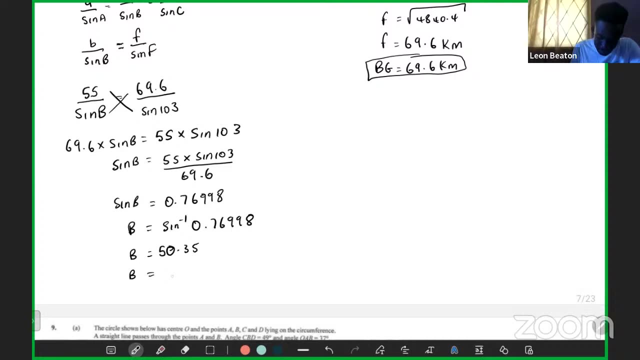 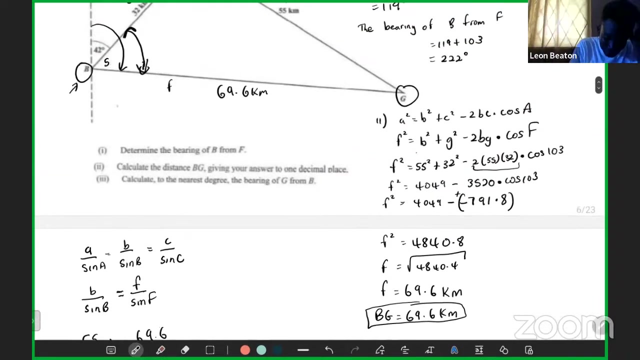 b here, b we're called. every stay fight t, t during the of f, f constitution, b, ft, a, c, d, etc. l to c, e, n, f, n, d degrees. so B is equal to 50 degrees. so you know B is equal to 50 degrees. so 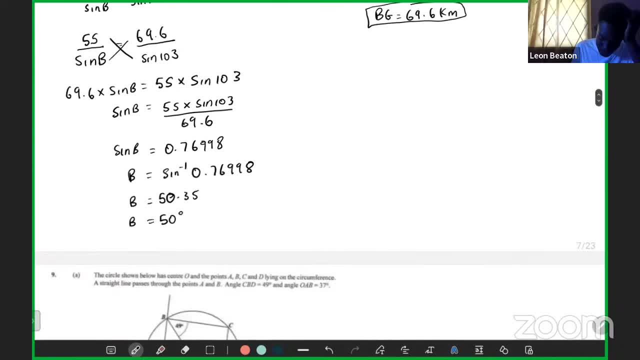 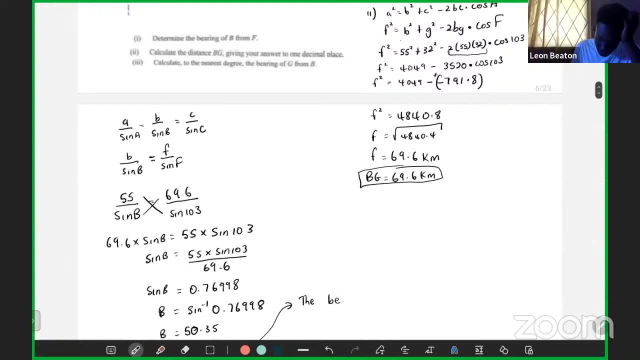 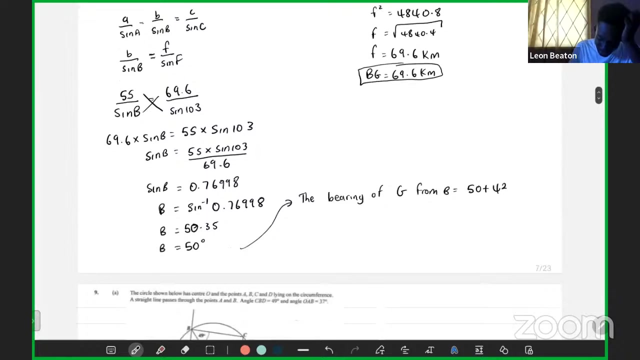 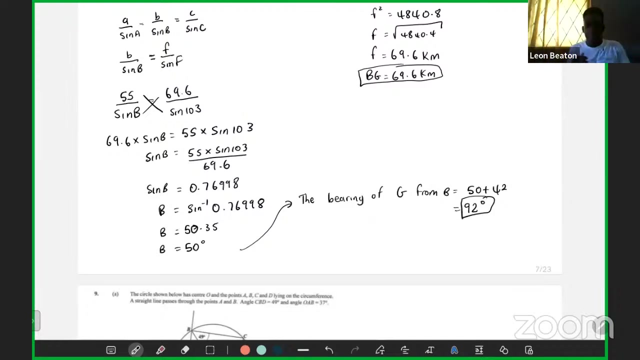 what would be the bearing of G from B? so we gotta add these two, right. add the 42 and the 50. it'll be 50 plus 42. the 92 degrees: all right, 92 degrees, easy marks, right. let me see what's going on. that's. this is on Parsons commenting. 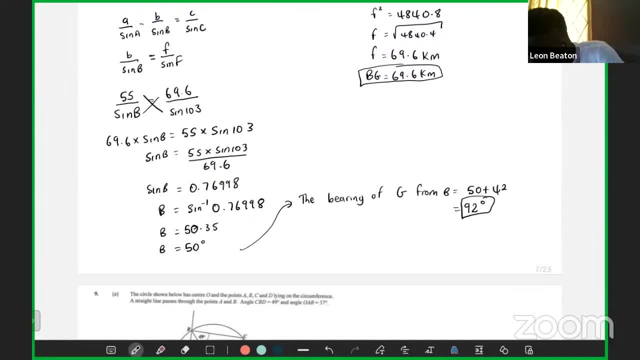 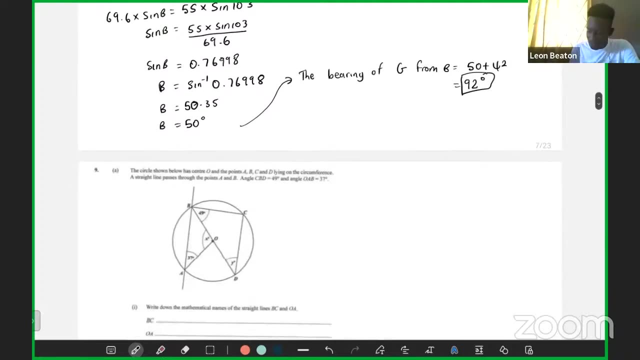 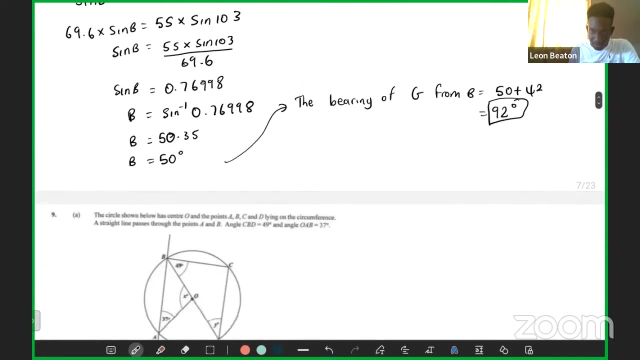 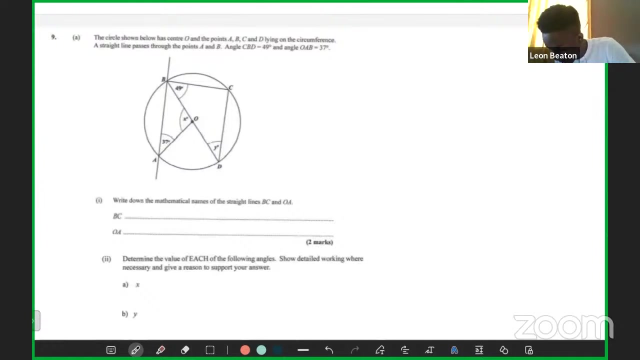 yes, AC Clarke, Nicola Bell, Emanuel Heels. all right, so that was some bearings, that was bearings, right, everybody good there. so as you come in, you can share the live. share the live, and, uh, you know, target CXC students. so my watch has saved me. live for one hour, is that? so it's been one hour already, students. 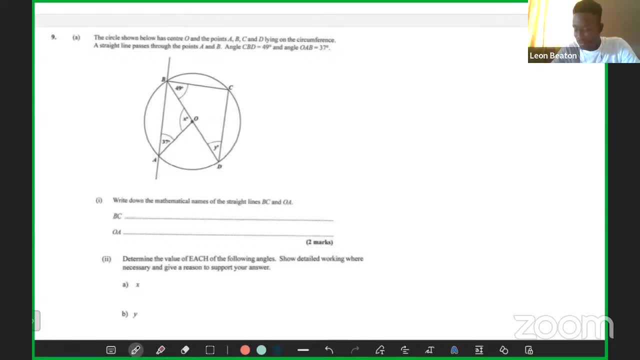 has it been one hour? you are you all in check-in? anybody check-in? it's been one hour. yeah, it's been one hour. it didn't even seem like one hour. feel like five minutes? right, don't take five minutes for anybody, okay? yes, case you. 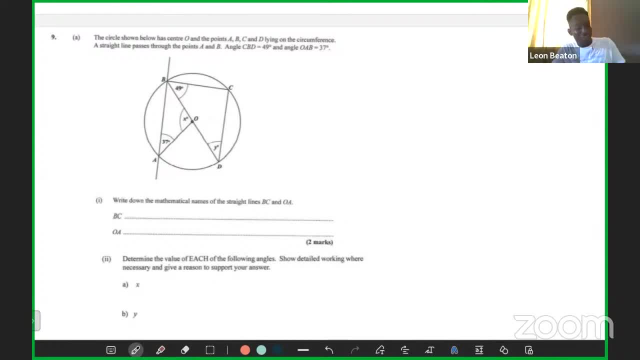 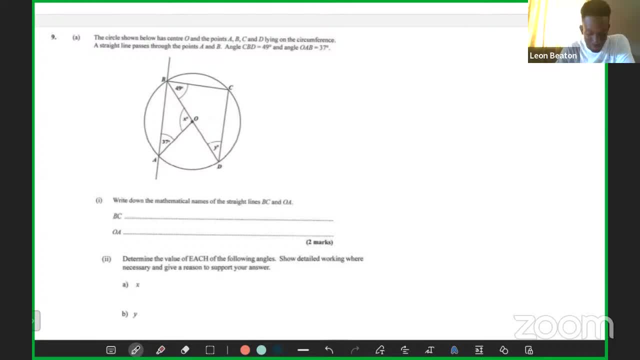 lying on the circumference has center O and the points A, B and C lying on the circumference. straight line pass is through points A and B. angle C, B, D is equal to four out of nine. an angle a o- sorry o- a, b is equal to 37 degrees. 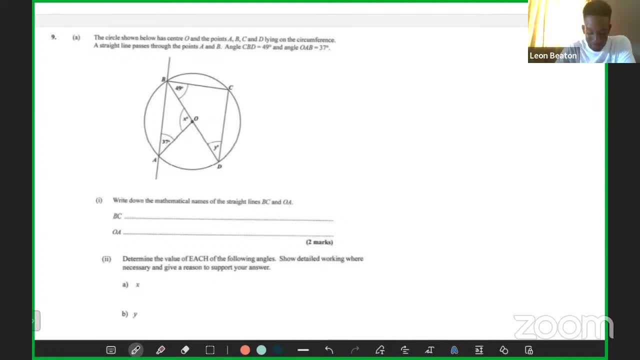 So the first one write down the mathematical names of the straight line b c and o a. So what is the mathematical name given to b c? Anybody b c. This is my mathematical name given to b c. 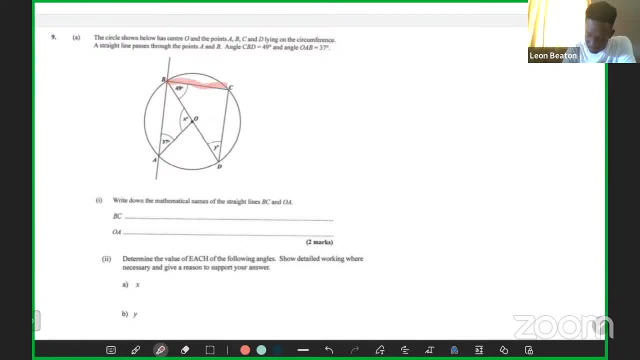 b, c would be here. Let's see if anybody will get it in the chat or I will get it here for us. We're also live on YouTube. I don't see what's going on over on YouTube. Oh, we have 4,000 YouTube as well. 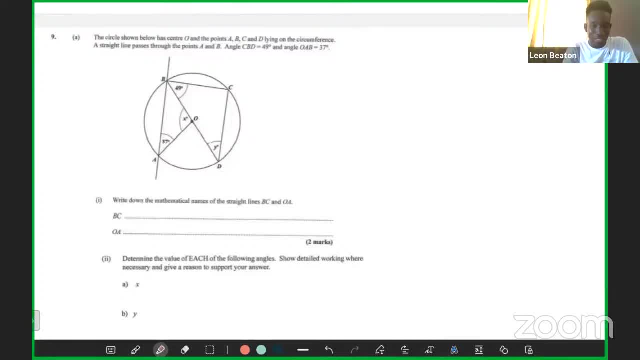 Somebody's saying they're listening. Yeah, anybody. Yeah, go ahead. It's a chord, sir, It's a chord. Yeah, it's a chord, It's a chord. So b c is a chord, b c is a chord. 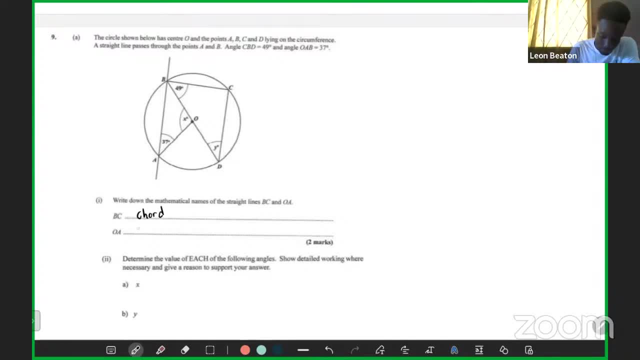 And what is o, a Radius, Radius, Radius, Two easy marks here. Yeah, so b, c is a chord, o, a is a radius, Two easy marks. Let's see. Yeah, So next one. determine the value of each of the following angles: 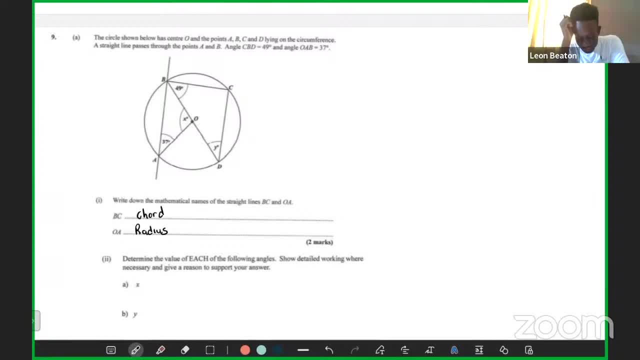 Show detailed workings where necessary And give a reason, A reason to support her. And so so we want to find the value of angle x. So we have angle x, which is this angle here. So let me a angle x. 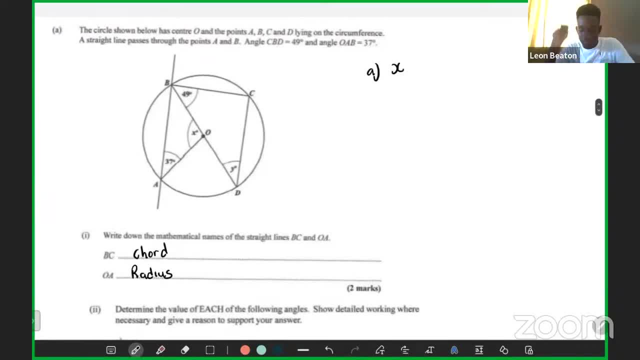 Anybody what's the value of x And how can we find that value? So let me zoom out. Sorry, Sorry. This is an isosceles. So we know that is a isosceles triangle. It's an isosceles. 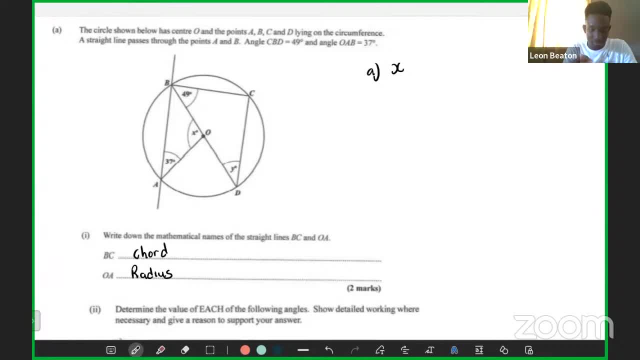 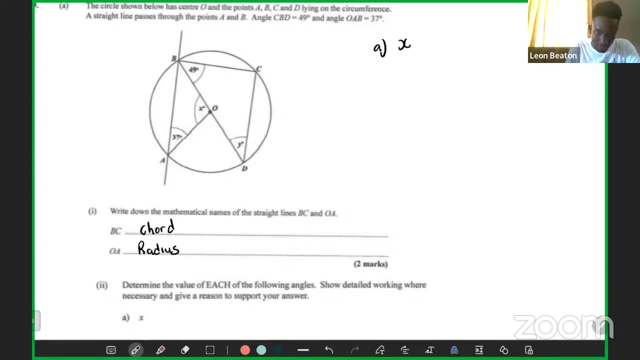 How, how do you? how the? So because, um, the, the point in the middle, Mm-hmm, And it touches the right. Yeah, So it's a isosceles triangle. two lines are equal. and also, in addition to those two lines being equal, um, what else do we know? 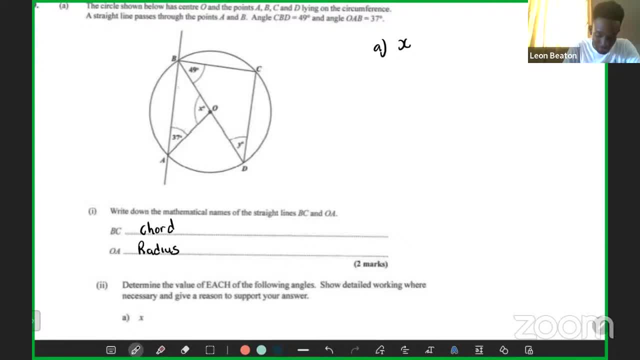 again, if here is 37, here would be what 37, 37, excellent. so if there is 37, there is 37. so we can say x would be equal to 180 subtract 37 plus 37.. it'll be 180 subtract or 737. 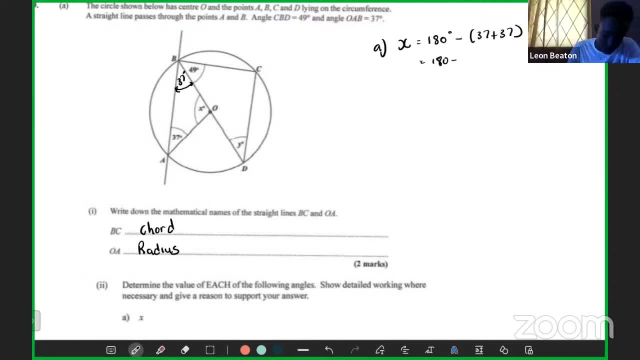 74, 74, 74 and 180 minus 74 give you 106. so we can see what would our reason be, what would our our reason be, what would the reason be? so you can say: because it's an isosceles triangle, right? so you can say oh, so you can say a, b o. 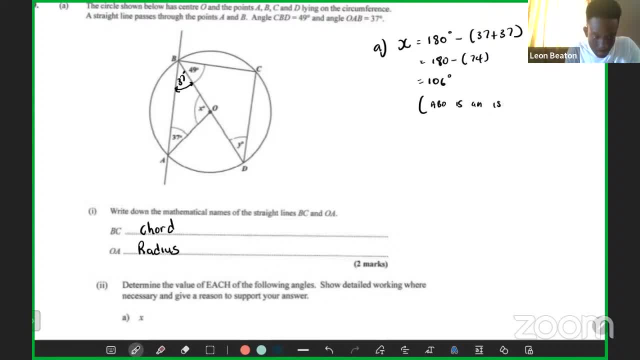 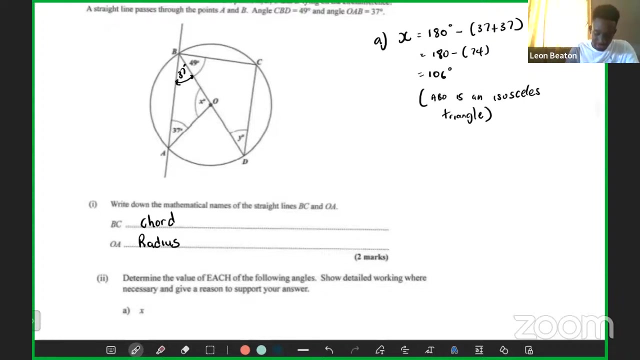 is an isosceles triangle. all right, that would be a reason. so, like socialis are, angle meaning the two angles are equal and so on. all right, so i said for that one. so the next one, um, calculates. well, we got to find the value of y, so we know, here is um. 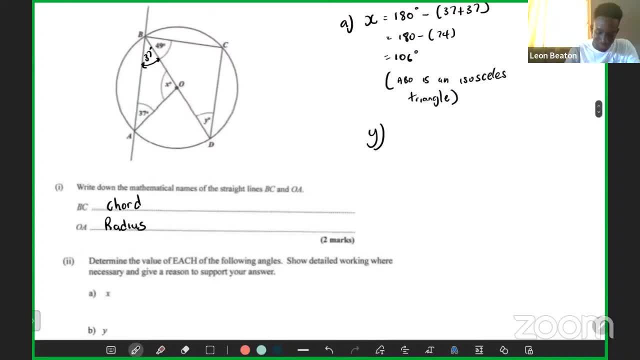 106.. What would be the value of Y? It's nice and easy: 37.. 37? Why, Careful, Don't assume right. Why? What would be the value of Y? We know it's a triangle and it's at a certain location. 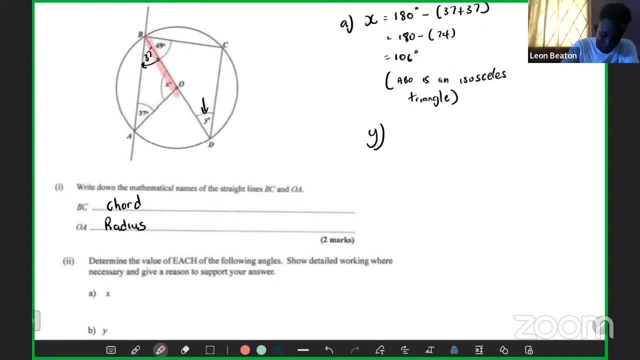 Let me outline the triangle for you. Somebody is saying it's at 37 because I was there. I guess you're talking about dead angle, Right? In order for you to have a dead angle, you must have two parallel lines, right? 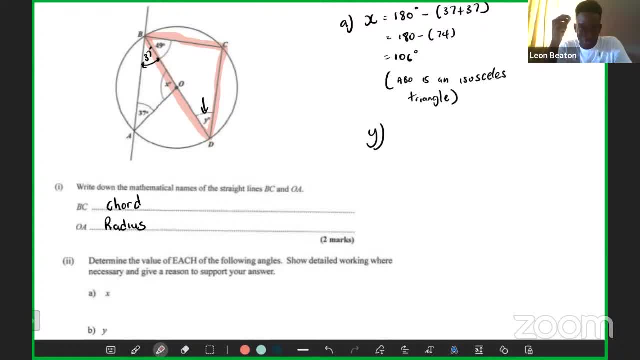 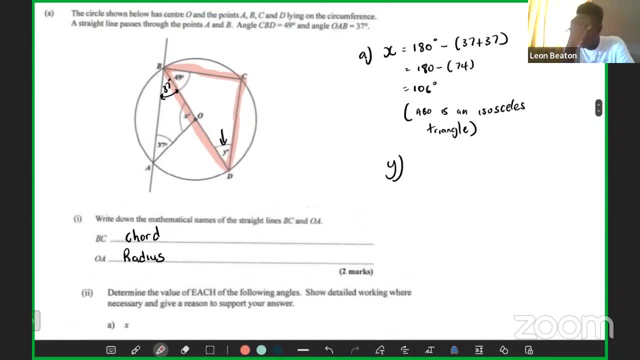 And I don't think in the instruction I read anything about two parallel lines. Did I miss it? No, No, they didn't say anything about parallel lines. So it can't be dead because you don't have a parallel line. Now look at it. Look at the triangle. 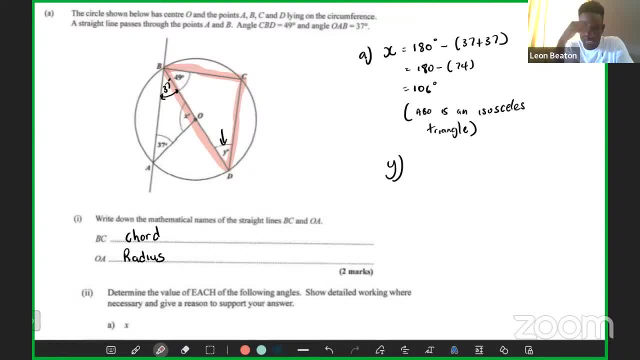 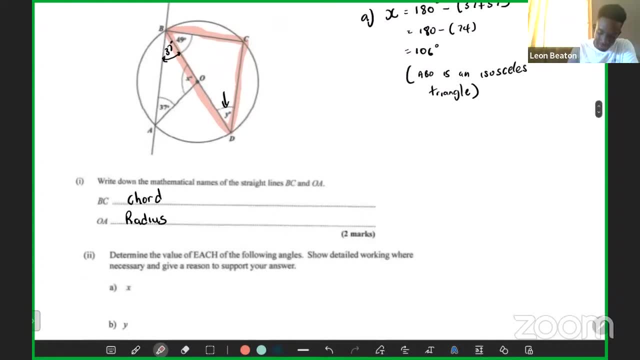 good. Where is that triangle located, Sir? in a sense in a semicircle, In a semicircle, Excellent. So it's located in a semicircle. So it's located in a semicircle. So how can that help us to find for Y? 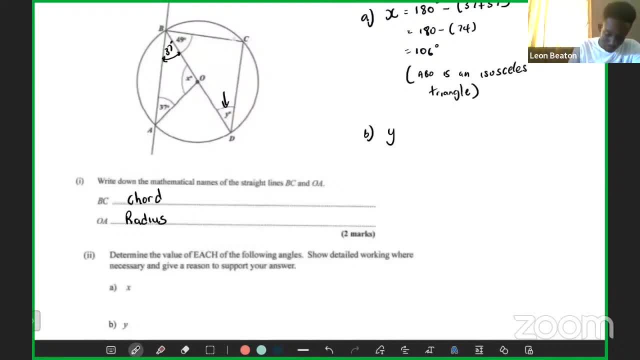 Sir, it will form a right angle. So you know, here would be a right angle, right, So here would be a right angle. So we know two angles. We know this angle here and we know this angle. So now we can find for Y simply by subtracting. 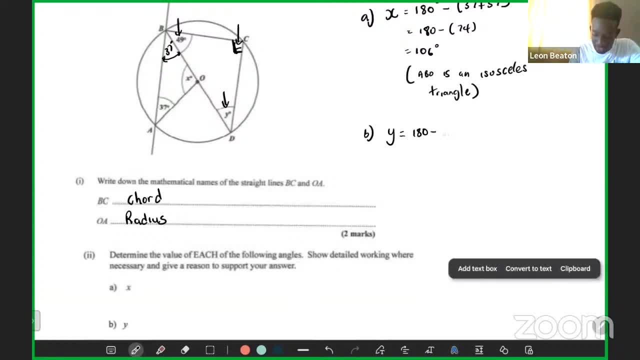 So you can say Y is equal to 1.. 180 subtract 180 subtract Part of 9 plus 90,. right? So this would be 180 subtract part of 9 plus 90.. 139.. 139.. So we want 80 subtract 139. 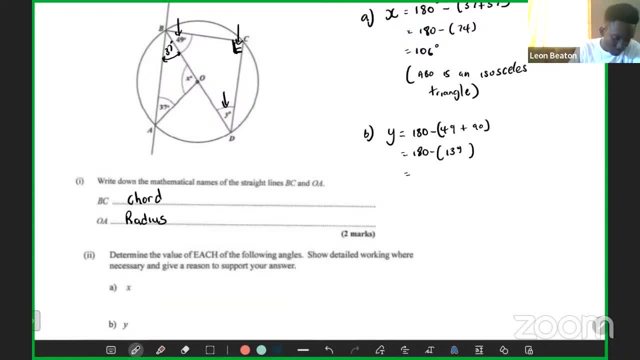 And then we give us a value of 4 to 1.. 4 to 1 degrees And our reason would be, Our reason would be: angle in the semicircle is a right angle or 90 degrees, All right, The angle in the semicircle is a right angle. 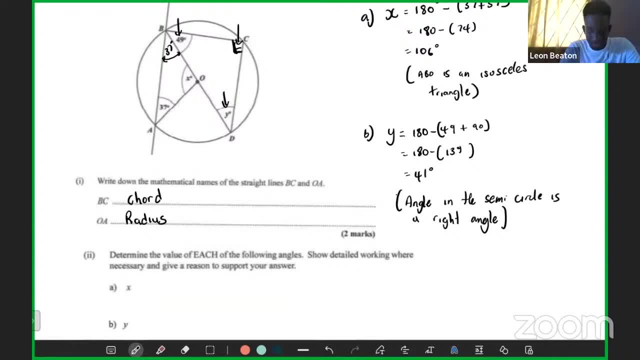 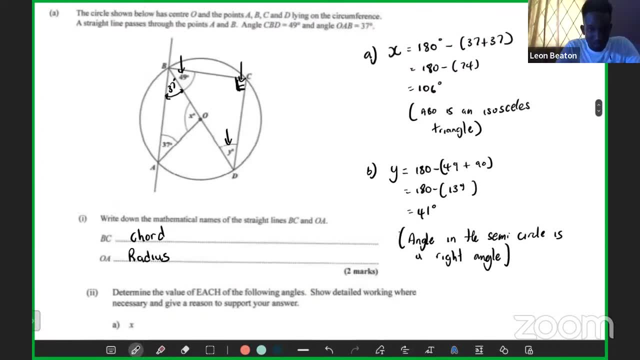 Yes, Casey Clark, And that is Y All right. So now we are going to work on our right angle, right angle. So we have one angle and one right angle. Alright, Everybody good here. So we use some sort of theorem and we use some knowledge of triangles to answer this question. 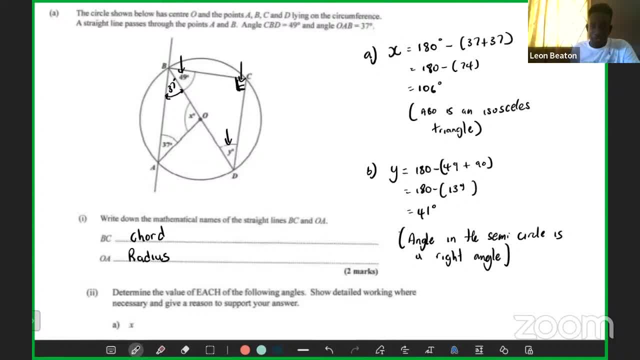 Alright. So sometimes you will have to do a mixture of the two. You're got to know what your triangles, Type of triangles. You have to know about angles. Sometimes you'll have a Z angle, Sometimes you will have an interior angle and sometimes you will have to use theorems. 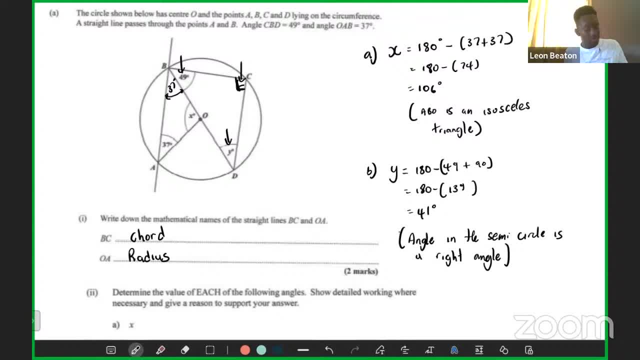 Right, Or sometimes you know you can use any one. all right, so you're not limited to just the circle theorems. all right, you're not just limited to the circle theorems, to be any combination of any theorems or anything that you know that can help. 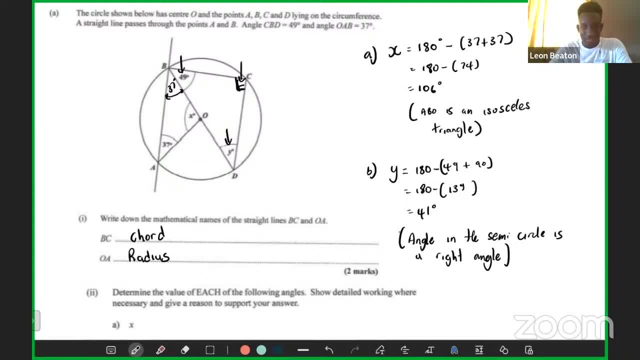 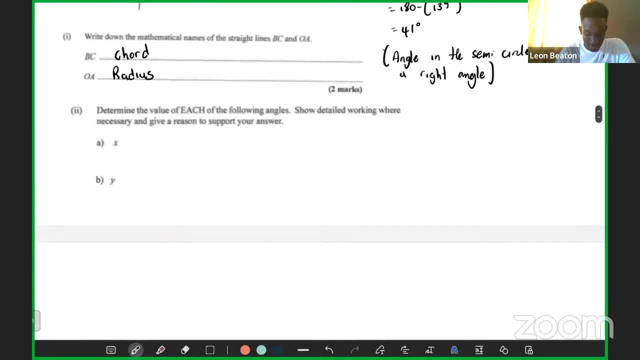 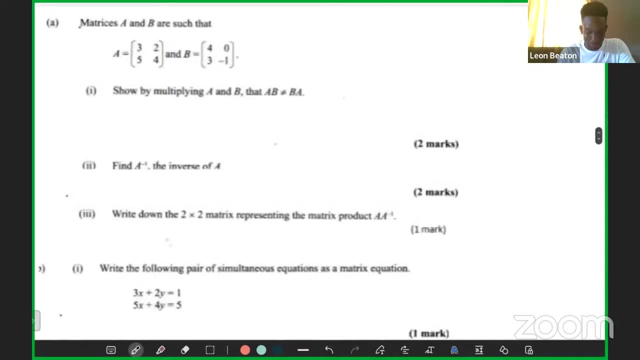 you all right. so that is that. so let's see what else we have here. ah, so we're moving to some matrices now. oh yeah, how good they are good with matrices. is my friend leno there? yes, all right, leno. leno should be leading here with matrices. 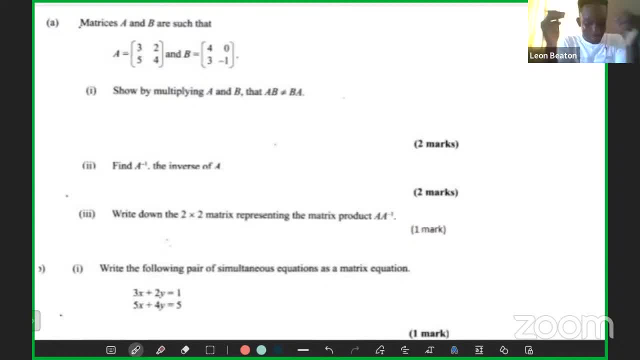 he knows why, anyways. so, um, so, let's go, let's go, let's go. so the matrix a, b and c are such that a is equal to three, two, five, four and b is equal to four, zero, three, negative one to show why, multiplying a and b, that a, b is not equal to b, c. 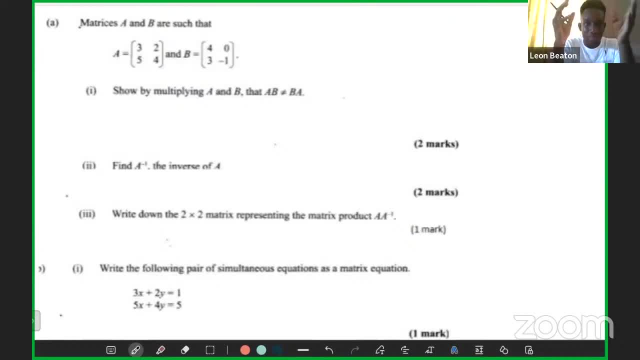 so this is telling you that they want to multiply a- b and they want you to multiply b, c and after you finish multiplying, those two matrices should not be equal. all right, they want you to show, by multiplying a and b, a, b and c. b is not equal to b? c. 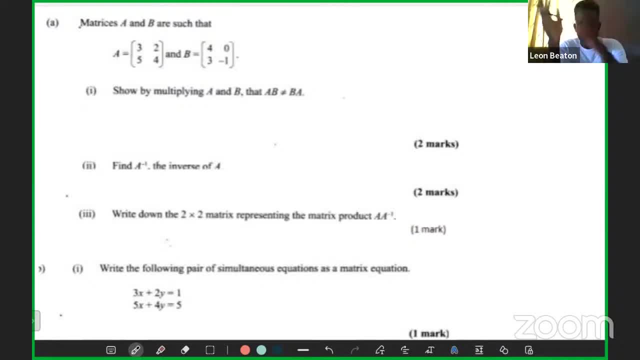 so the first thing you gotta do, you gotta find, um, you gotta find for a, b and then you're fine for b, a. ah, can anybody remember how come, how we can multiply uh matrices row by columns or row by column, row by column, right row by column? 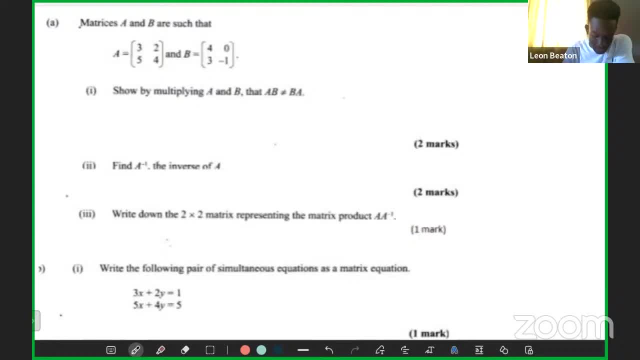 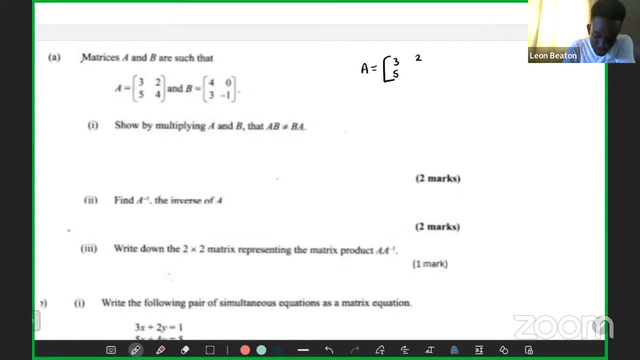 so let's multiply the rows by column. so let me see if i can work with. all right, let me let me write down the matrix. so we have: matrix a is equal to three, two, five for a. matrix B is equal to 4, 0, 3 negative, 1. yes, Casey Clark's go by. 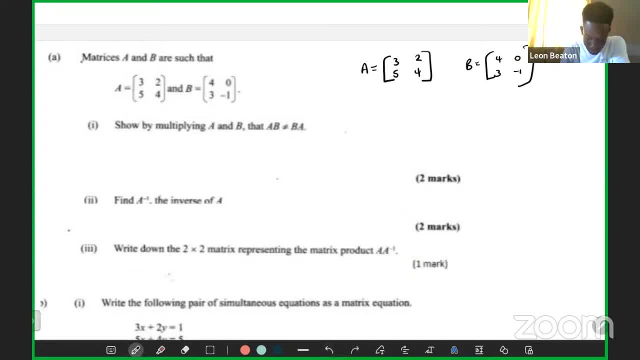 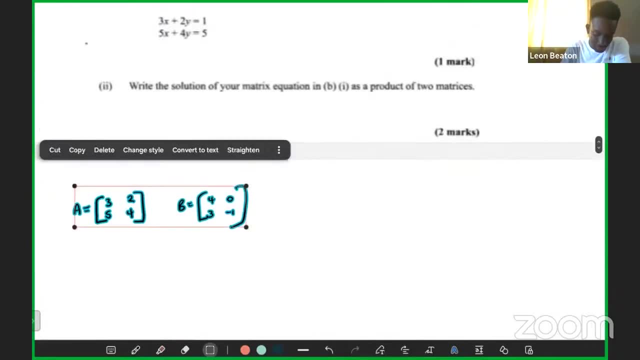 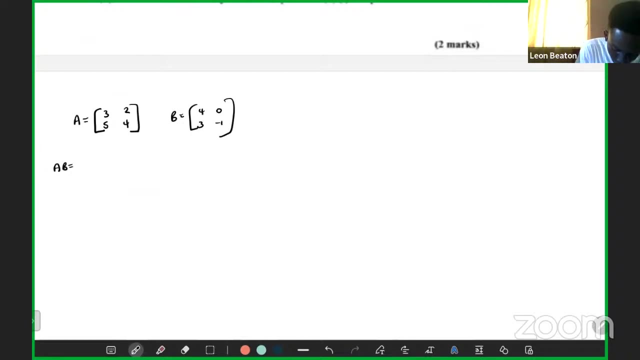 column. oh, let me draw example- is at the bottom. so let's find for um, let's find for a B. so what is my for a B and B C. so let's find for a B force. so a B is equal to 3, 2, 5, 4 x, 4, 0, 3, negative 1. so row by column, so it's row by column. so row by. 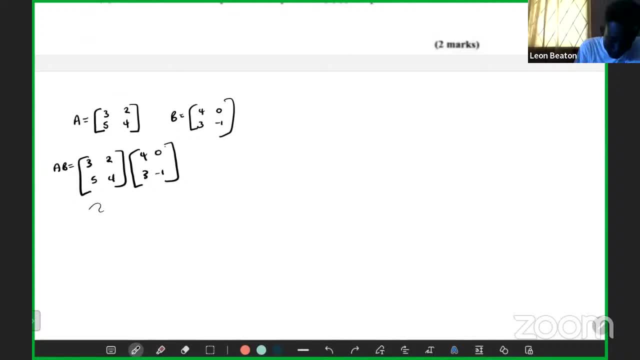 column would be somebody out. there will be um 3 times 4 plus 2 times 3, two, three times four plus two times three, two times three. good, I'll be for the fourth one, and then we go row by column for the second one, else would be three times zero plus two times negative. one would. 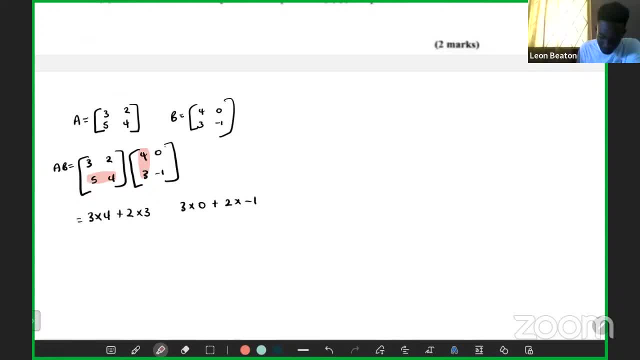 and I sort of force, or that will be Israel, by this column: five times four plus four times three, mm-hmm. last but not least, these five, five times zero, zero plus four times negative one. good, so let me access now. um, you know this, this part here can be a bit confusing for forces. what is a good indication to what? 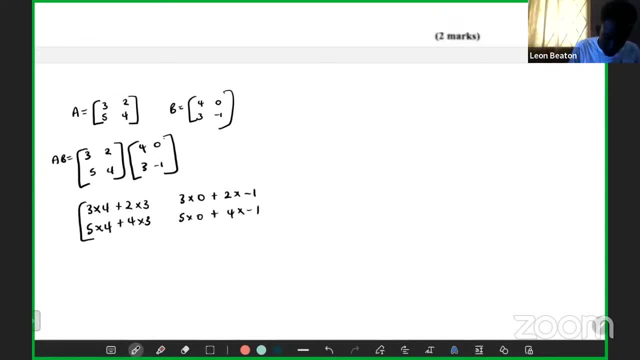 is a good indication to check for when you're multiplying, to know that you're, you know you're correct. what is one thing you can look for? a trick or you know they can look when, when you finish setting up this part here, what is one thing you can look for? third arm, the last number in the 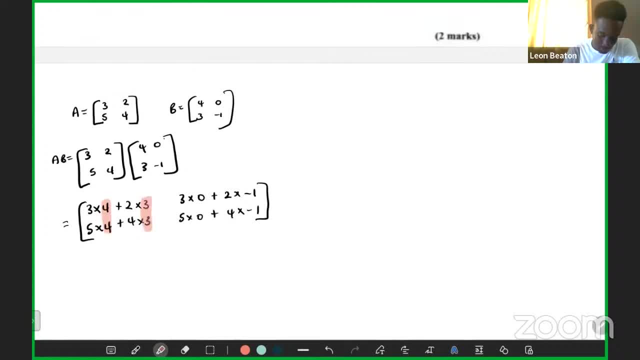 in both um rows should be equal, so these two elements should be the same right. so there's one thing you could check for if those are. if those are not the same, that means you did something incorrect. i want to go, and you know, check back to see where you made the error, or 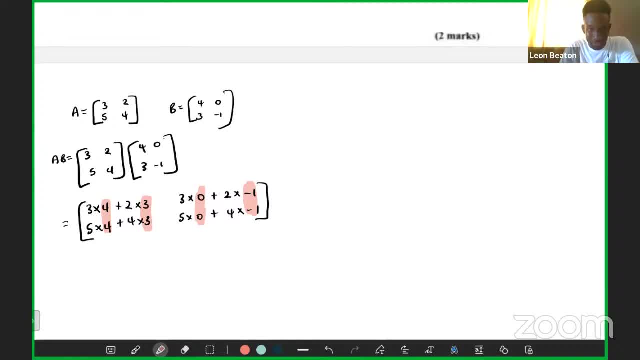 the mistake right. so be on the lookout for that, because you know it can get a bit confusing when you're at this piece, especially after matrices, would be the last set of things on the paper. you know you're tired from the exam, so look out, be on the lookout for that. 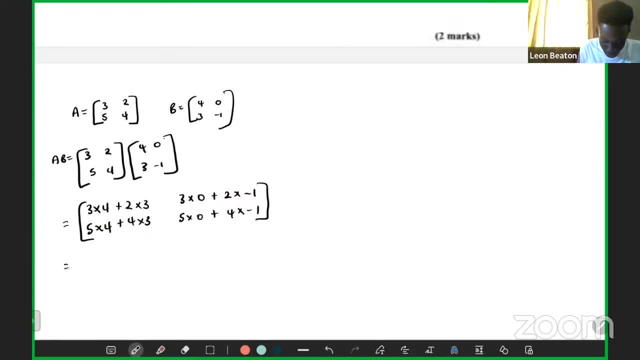 so that would be that. um, so then we know, we just do some simply simple computation. so this would be: three times four would be twelve plus, uh, two times three would be six. five times four would be twenty plus four times three would be twelve. and three times zero would be zero. plus two times negative one would be negative two. 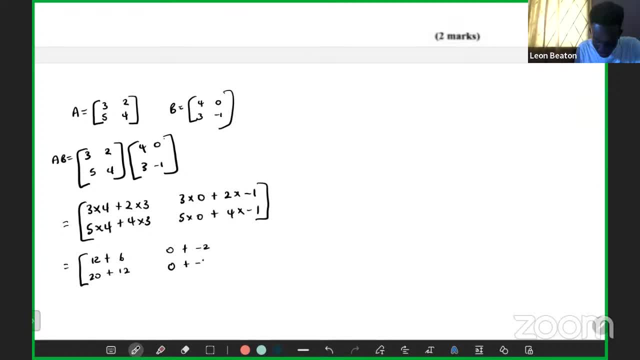 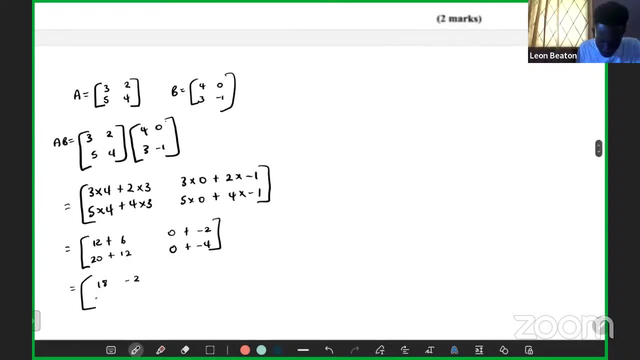 five times zero would be zero plus four times negative one would be negative four. all right, so now we have: twelve plus six would be eighteen. zero plus negative two would be negative two. twenty plus twelve would be thirty two and zero plus four would be zero. plus negative four would be negative four. so there's our answer. 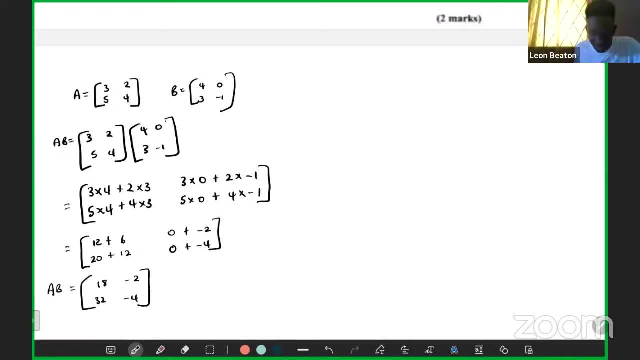 for a b. All right. so the question said to show that A B show I'm multiplying. A B and B C are not the same. So the next thing we got to do we got to find for B C. 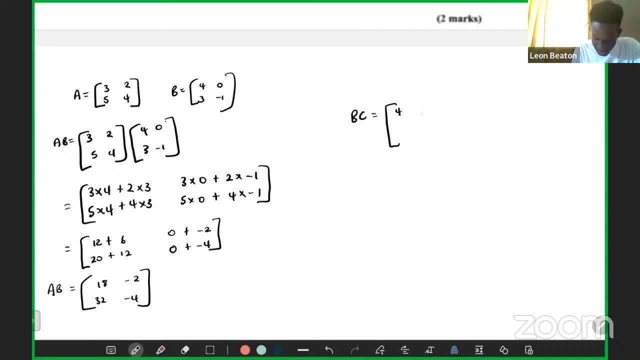 All right, so B C would be 4,, 0,, 3, negative 1.. And then we do anything reverse: 3,, 2,, 5,, 4.. So we do the same thing, like what we did, row by column. 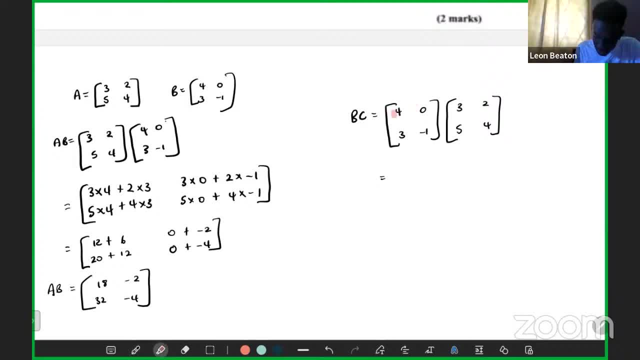 So this would be row by column, row by column. So this would be 4 times 3 plus 0 times 5.. And then this would be 4 times this here, by this here now, 4 times 2 plus 0 times 4.. 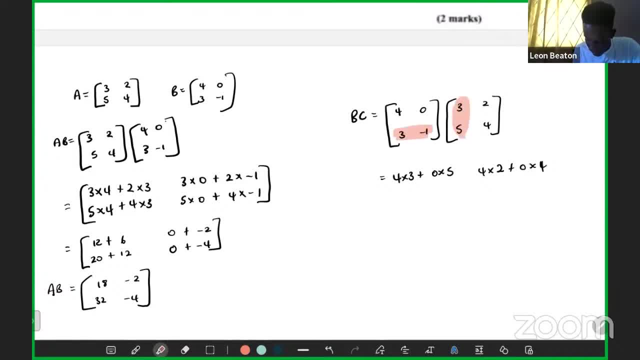 And then we go this here by this here now, And this would be 3 times 3 plus negative 1 times 5.. And then the same thing, this here, by this now, And then this would be 3 times 2 plus negative 1 times 4.. 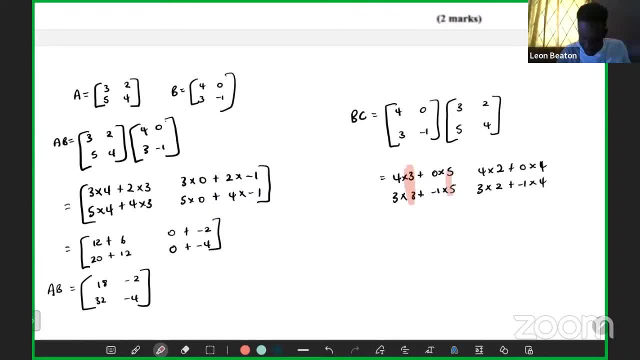 And once again, you want to check to see if you know these two are corresponding. And if those two are not corresponding, it means that you made some error. All right, so row by column, And then we do some simple computation. 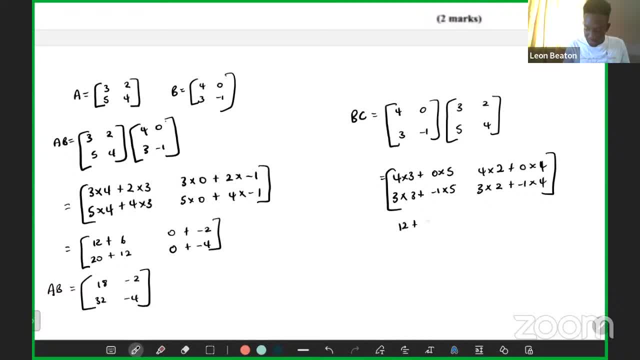 It would be: 4 times 3 would be 12 plus 0 times 5 would be 0.. 4 times 2 would be 8 plus 0 times 4 would be 0.. And 3 times 3 would be 9 plus negative 1 times 5 would be negative 5.. 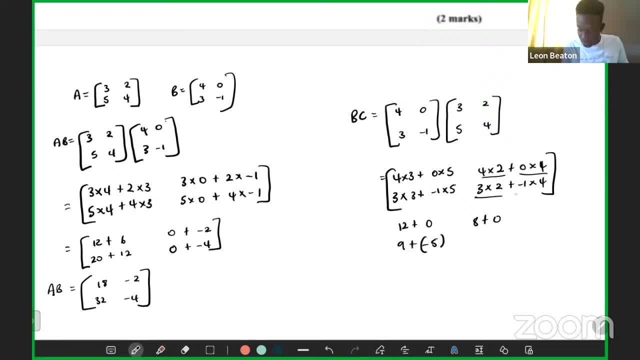 And 3 times 2. Would be 6 plus negative. 1 times 4 would be negative 4.. All right, And then we simplify: 12 plus 0 would be 12.. 8 plus 0 would be 8.. 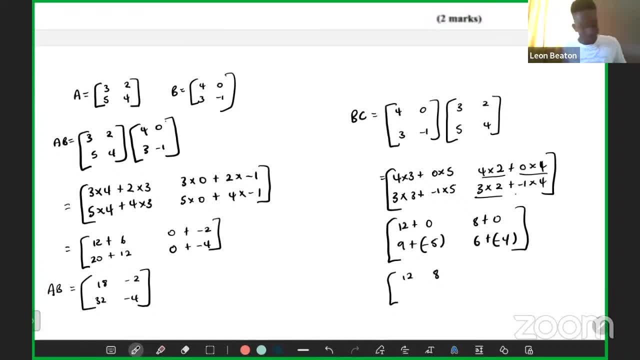 9 plus negative 5.. Let me show this out: 9 plus negative, 5. Positive, 4. Positive, 4.. That is 2 divided by 2 and negative. 9 minus 4 would be. 9 minus 5 would be 4.. 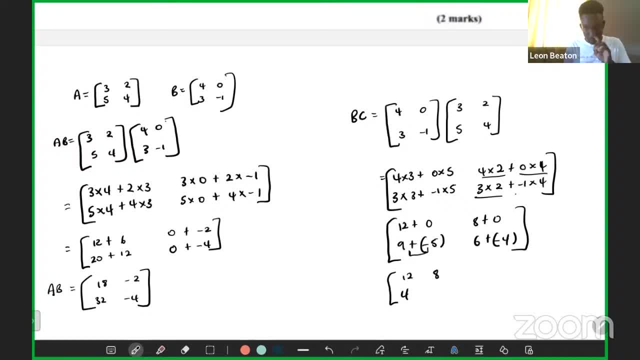 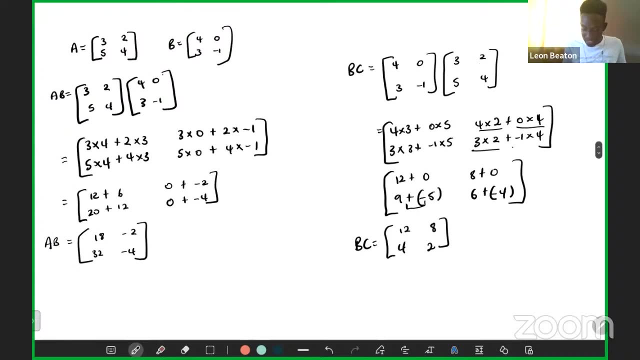 6 plus negative, 4. 6 plus negative, 4. Positive, 2. Positive, 2. Excellent. So this would be BC. So you can clearly see that AB and BC they're not equal right. So that is what the question asks us to show. 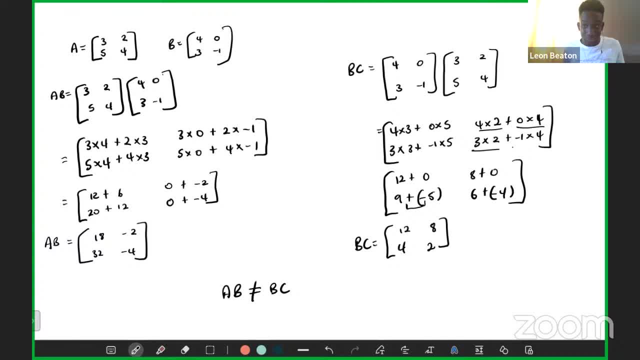 So we can clearly see that those two are definitely not equal. So it's BA, sir, Oh BA. So it's BA sir. So it's BA instead of BC, right, Yeah, All right. So, unlike matrices, if you have two normal numbers, 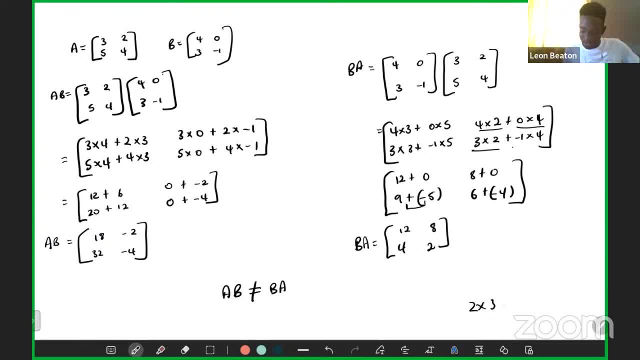 you know, if you got 2 times 3 is 6,, 3 times 2 will also be 6.. So this doesn't hold for matrices, right? The order of the multiplication it matters, All right, So that's what they wanted you to show. 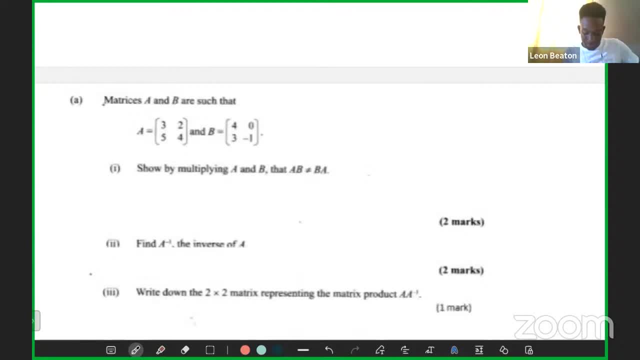 So the next, they want us to find the inverse of matrix A, The inverse of matrix A. So you have matrix A here And they want you to find the inverse of that matrix. Inverse of matrix A. So let me work it right here. 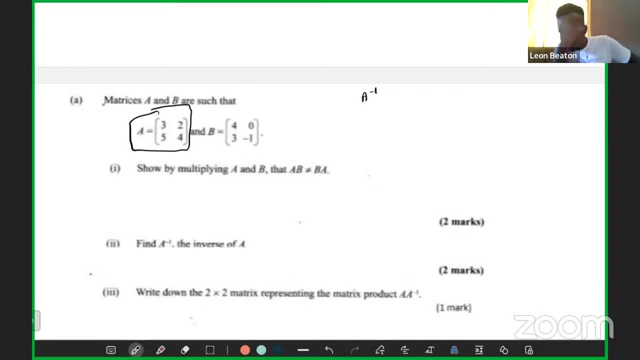 Anybody can remember how we find the inverse of a matrix. There are 1 divided by the determinant times, the adjoint, 1 divided by the determinant multiplied by the adjunct, 1 divided by the determinant multiplied by the adjunct. So we can find the determinant separately and the adjoint separately. 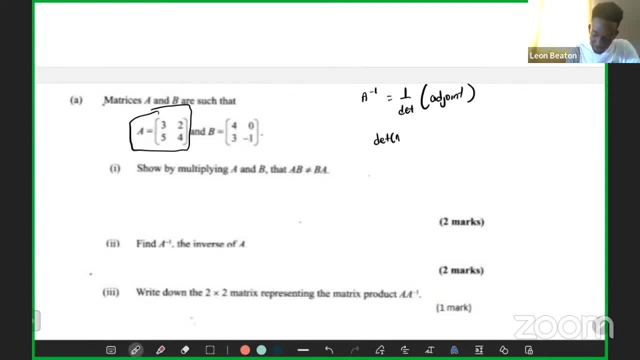 So let's find the determinant of A for us. So the determinant of A would be: Can you remember the formula to find the determinant Ad minus bc. Ad minus bc. So we're using matrix A, right? So we know the force element is A. 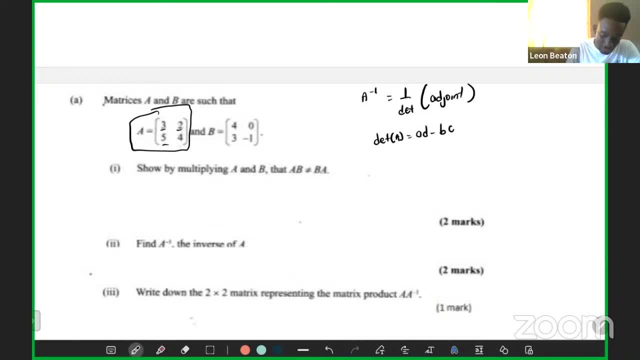 The second element is B, This is A, This is B, This is C, This is D. right. So A, B, C, D, right, It's A times D. So we know A is 3 times D, which is 4.. 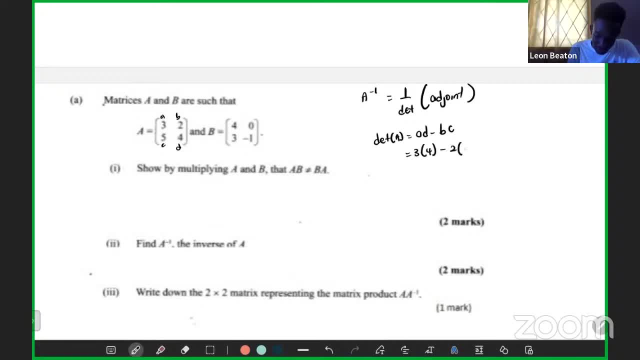 Subtract B times C, which is 2, multiplied by C, which is 5.. So 3, 4s 12 minus 2, 5s 10.. So the determinant of A would be 12 minus 10 would be 2.. 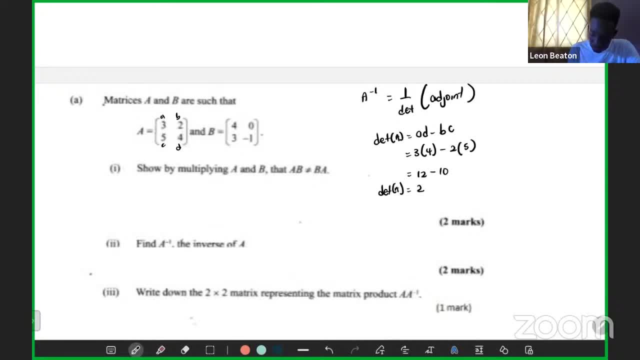 So the determinant of A would be 2. All right. Next, we want to find the adjoint. The adjoint is a nice thing to find, So you want to find the adjoint of: all right, let me write back this thing. 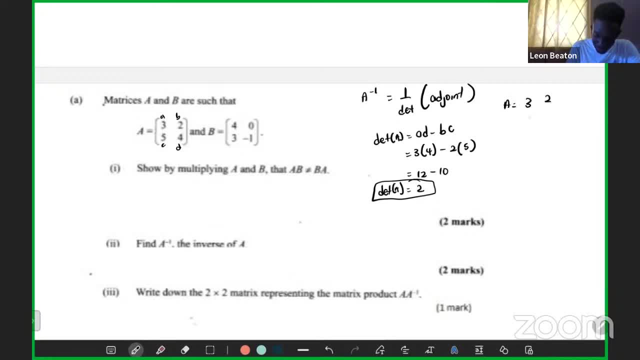 So matrix is 3, 2, 5, 4.. You want to find the adjoint of this, So the adjoint. how can we find the adjoint again? It's a nice thing. D negative, B negative, C A. 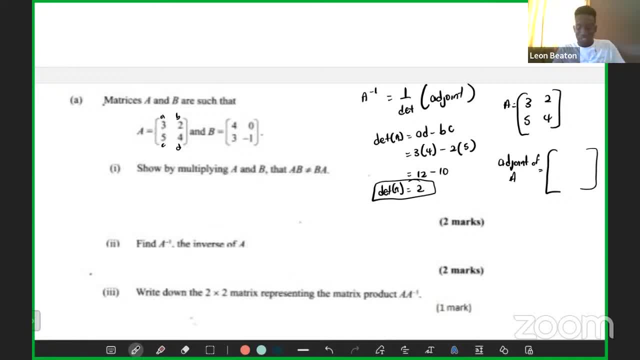 It's a lot of fancy, All right, So we switch. we switch these two, right. We switch these two. We interchange those two. We interchange the 3 and the 4.. So where is the 3?? We put 4.. 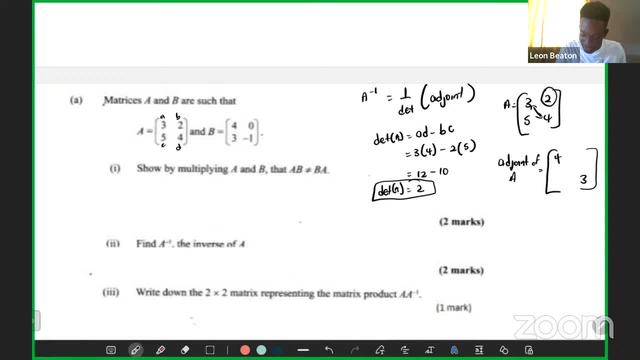 And where is the 4?? We put 3. And then we flip the signs of these two. So this would be negative 2, negative 5.. That is the adjoint. You switch and you flip. You switch these two and you flip the sign. 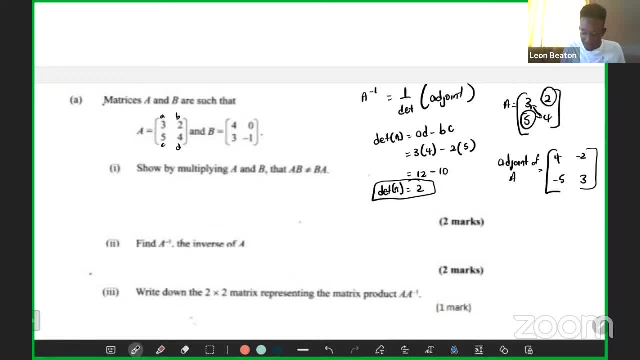 So if this was a negative, we're going to pass this. So that is the adjoint of A. So we have the adjoint of A And we have the determinant of B. So next is 1 over the determinant times, the adjoint. 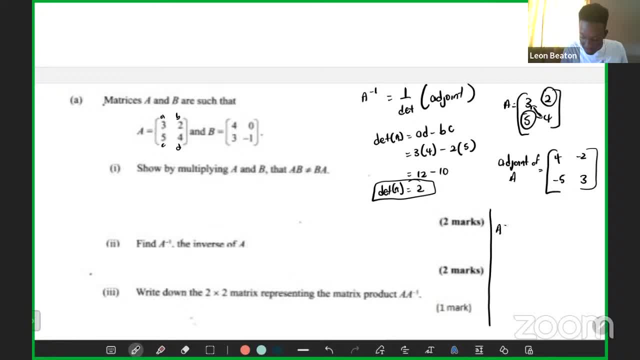 So let me work this right in the car in here. So A inverse would be 1 over the determinant times the adjoint. So it would be 1 over the determinant which is 2, multiplied by the adjoint which is 4, negative 2, negative 5, and 3.. 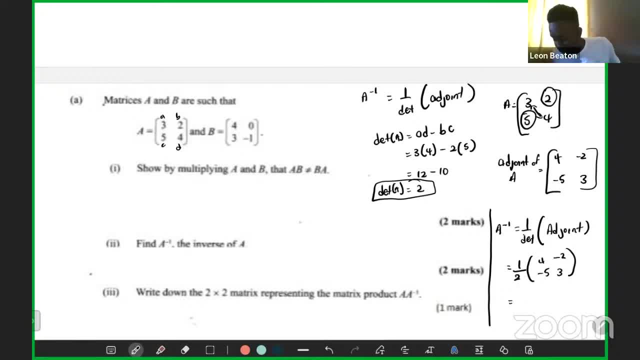 So we multiply, We do some scalar multiplication, meaning the thing directly outside, and multiply it by all the elements in the matrix. So this would be 1 half times 4 would be 4 over 2.. 1 half times negative 2 would be negative 2 over 2.. 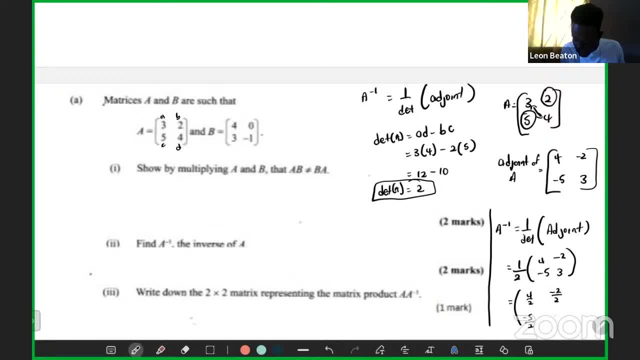 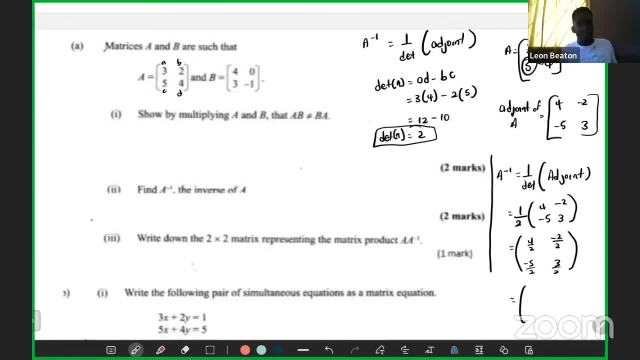 1 half times negative, 5 would be negative, 5 over 2.. 1 half times 3 would be 3 over 2.. And then we just simply simplify it. Simply simplify it Anyway. so we simplify it. So it would be: 4 divided by 2 would be 2.. 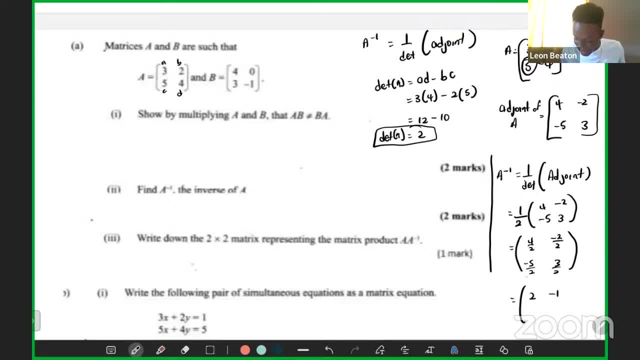 Negative 2 divided by 2 would be negative 1.. Negative 5 divided by 2 would be negative 2.5.. And 3 divided by 2 would be 1.5.. All right, And that is it for that. 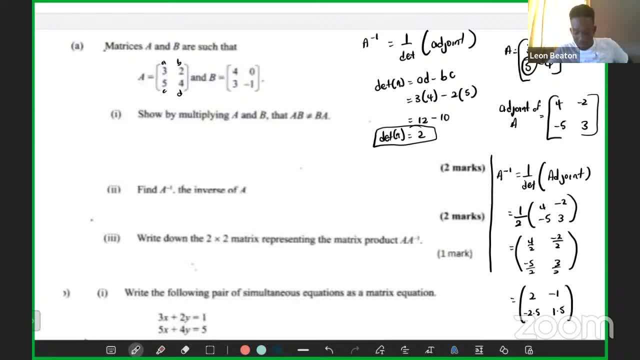 That is it for the inverse of that matrix. It's 1 over the determinant times, the adjoint, And that is how you can gain your full marks for that question. And, as you can see, this question went for two marks. Anybody got there. 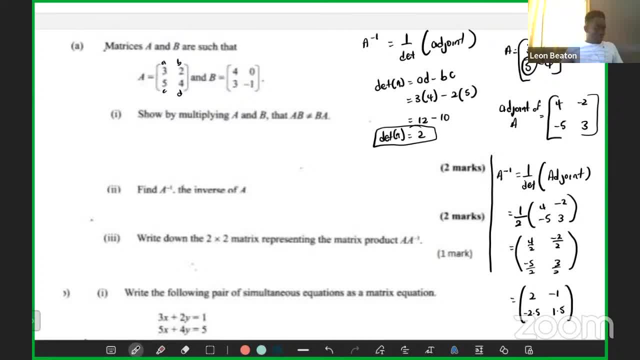 Yes, sir, Yes sir, All right. So for those who are now joining: normally I would go live by myself, but today I have a few students joining me. They said they were willing and excited, as I am, to come, and you know. 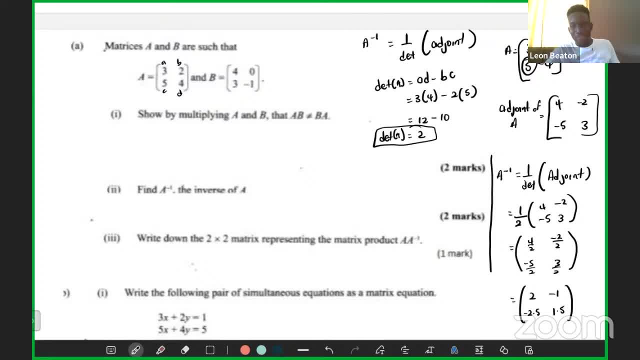 work some mathematics and help everybody prepare for the exams, All right, So that is all we're doing. I have some students along with myself. We're going through them together, All right. So these are some random questions that we took, random past people questions. 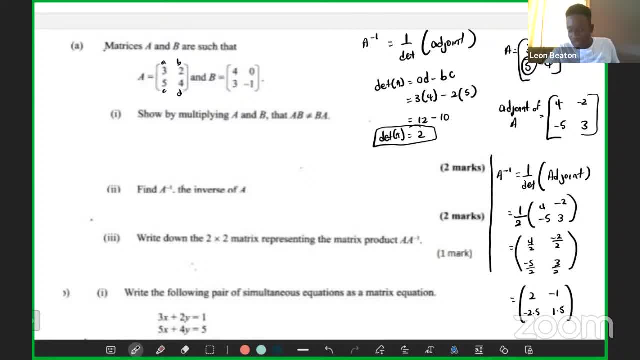 that we are working. try to mix and match as many concepts as possible, you know, to see how this can help students in the exam. All right, So the next one. Write down 2 by 2 matrix representing the matrix, The matrix brought up A times. write down the 2 by 2 matrix representing the matrix brought up. 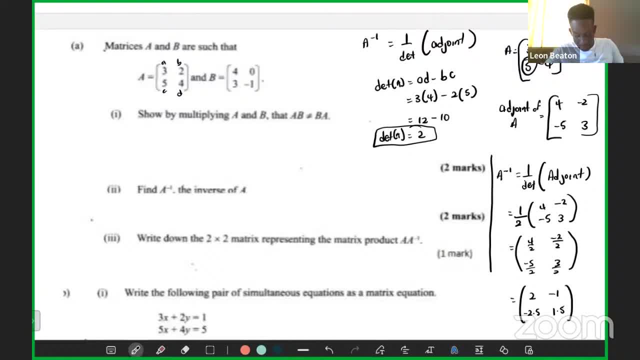 A times A inverse. Anybody 2 by 2 matrix representing not Anybody, could tell me what this is asking us to find. So is it the identity matrix? Yeah, Yeah, Yeah, they're asking to find the identity matrix, the 2 by 2 identity matrix. 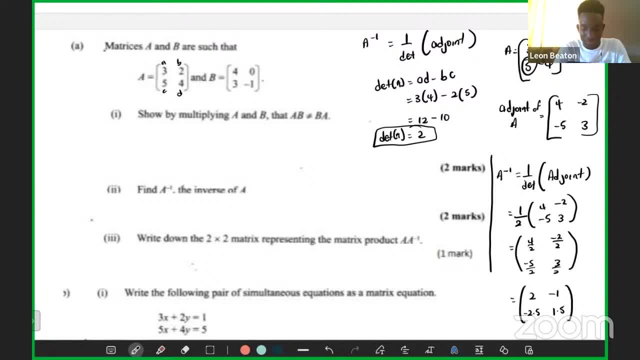 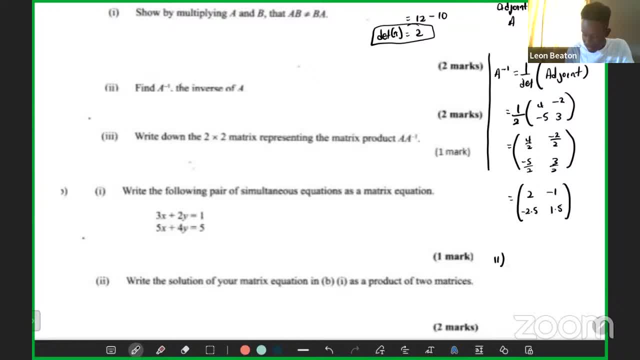 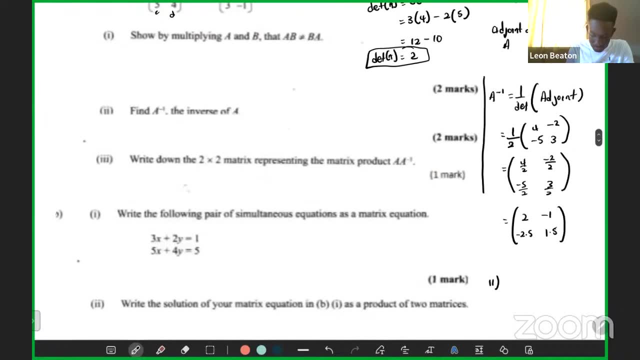 1, 0, 0, 1.. All right, Is that what you said, Russell? So 1, 0, 0, 1.. Good. Next one: Write the following pair of simultaneous: write the following pair of simultaneous equations: 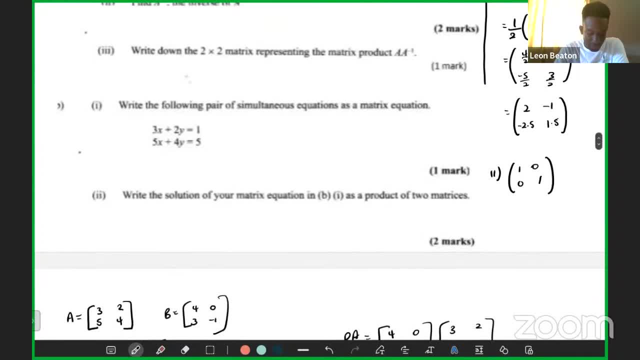 as a matrix equation. So we have the simultaneous equation 3x plus 1.. 3x plus 2y is equal to 1.. 5x plus 4y is equal to 5.. 5x plus 4y is equal to 5.. 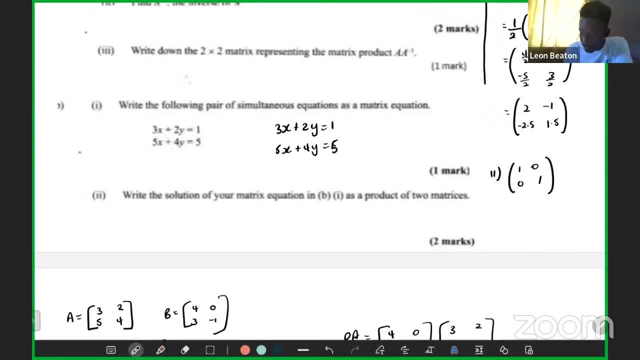 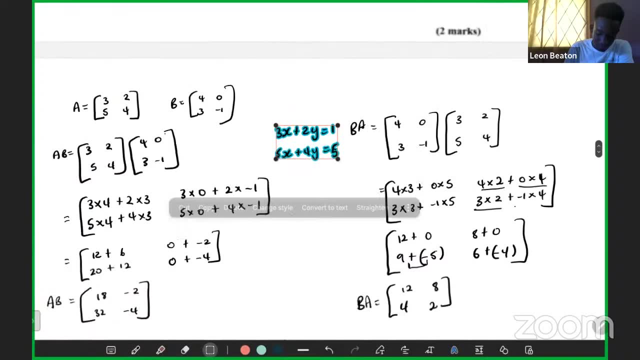 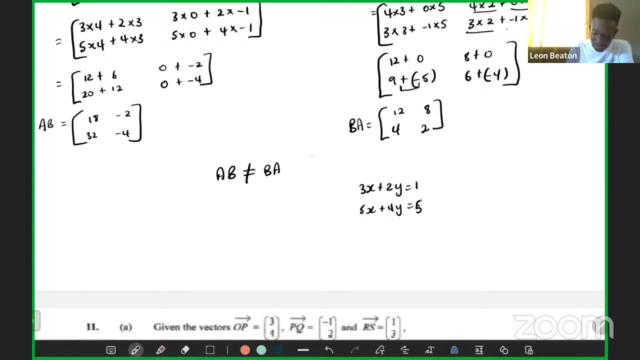 So let me drag this down and put this at the bottom, All right, So I got to look for some space. All right, So let me, So, let's go. So you want to write this in a matrix? 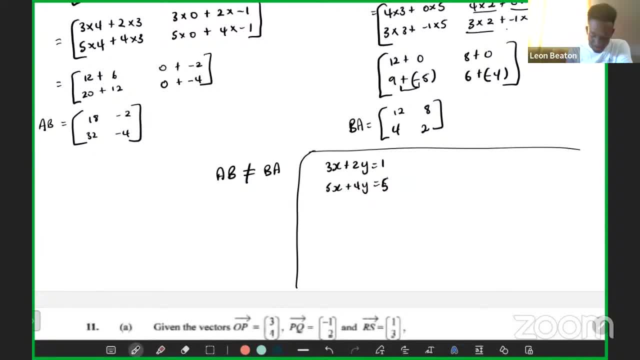 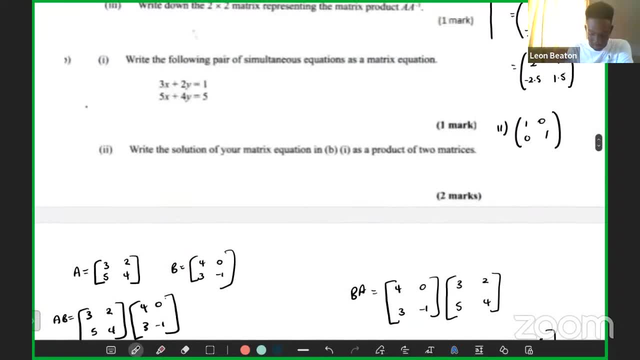 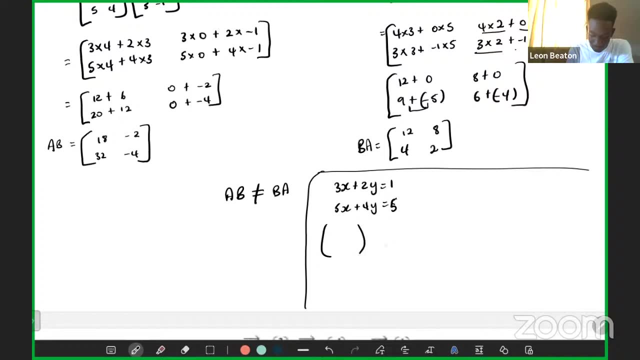 form. um, what would that? be very simple. they want. they want us to write the following periods of time as a simultaneous equation, as a matrix equation. what would this? be fairly simple. go ahead, sir. in the first one you'll get three, two, five, four, all right, plus three, two, five, four. 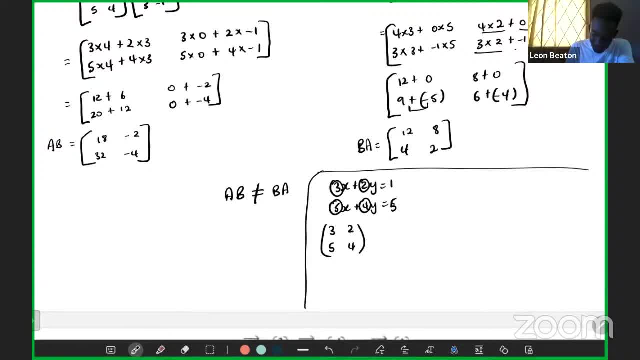 so just taking a number, the coefficients of these here, three, two, five, four, and then the other arm bracket, you'll get x and y. so you multiply by x and y, which would be two variables, is equal to one and five. one five, all right, yeah, all right, yeah. so, yes, you can see claxon and yeah, that's, that's, that's correct. so you take. 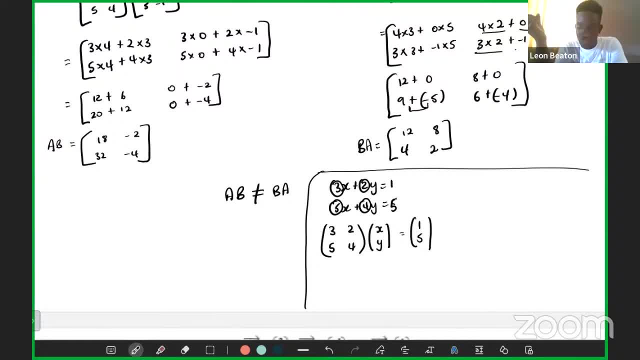 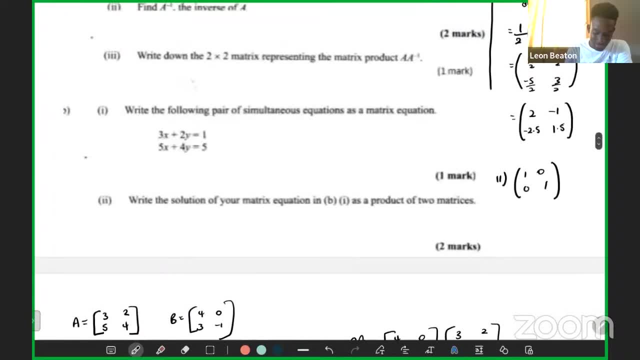 the coefficients you put in one dresser track. if you multiply it by x and y, which would be two variables, and you equate it to, you know the answer, and then it's just a matter of well, did they say, to solve it? yeah, so that would. we had one mark to write it in the matrix form and the next one the access to. 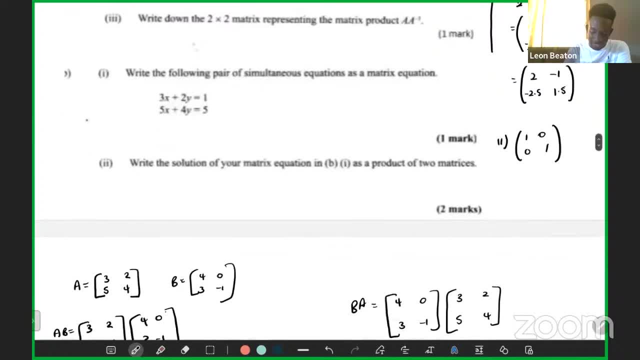 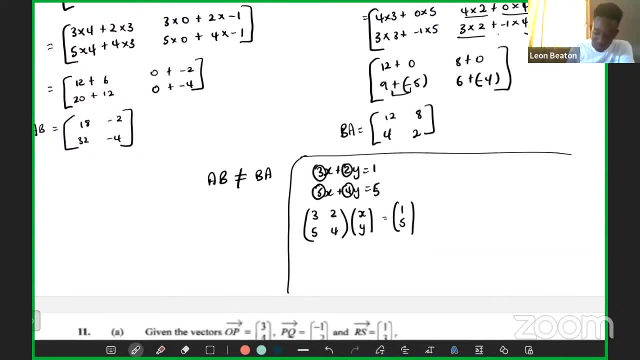 solve it. so write a solution of your matrix as a product of two matrices. so what we have to do- let's see if we get some space to work it out. so we have to do: we have to solve for x and y. So by solving for x and y, we have to take this over the equal sign and put it right there. 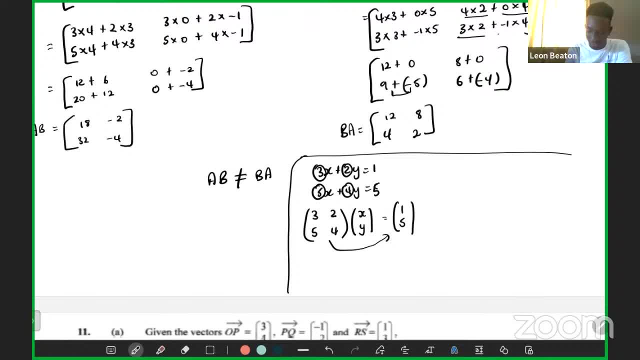 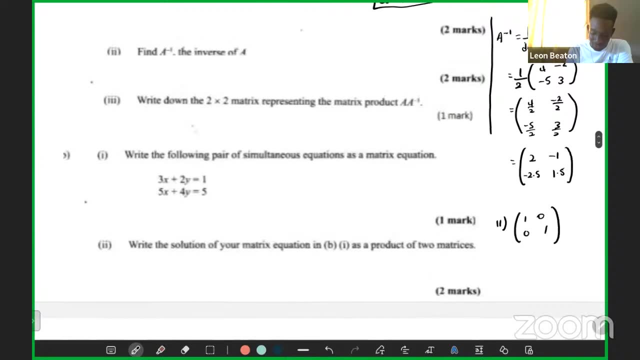 So when we take this matrix over, this equal sign, what will happen? It'll be inversed. Yeah, the inverse, right. So when we take this matrix over, it will become the inverse of that matrix. So the inverse of that matrix. I think we found the inverse of that matrix early on. 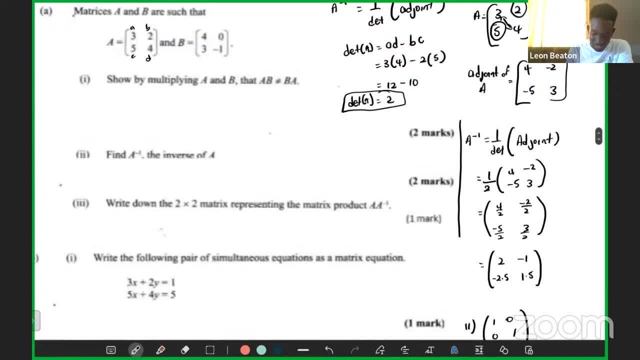 Let me see if CXC- yes, Yes, You see, we found the inverse here, This one, the inverse of A. So that is one thing that CXC do You know, they would bring whatever you found at the top to help you to solve for the one at the bottom. 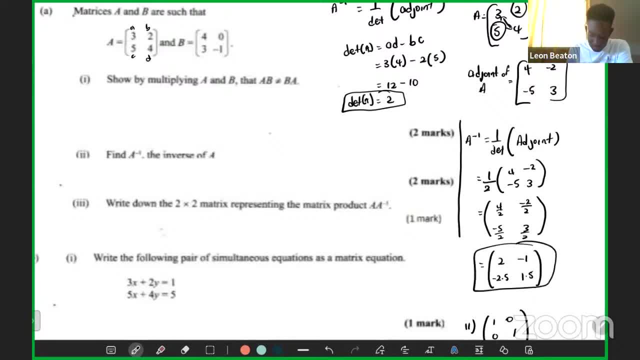 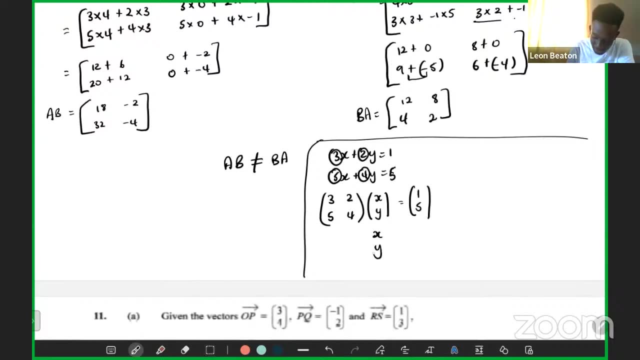 So you already found the inverse here, So let me copy that. You already found the inverse here, So this is the inverse, So there's no need to Redo the entire thing. right, You already found the inverse. So this will become: XY is equal to. 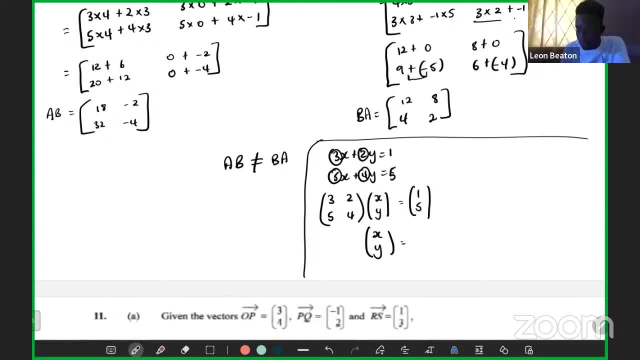 Now, where do we put this? Where do we put the inverse? At the front or at the back? Do we put it in front here? Do we say in front: Let's see, Let's put it in front and see. So do you put it in front and say that multiplied by one? 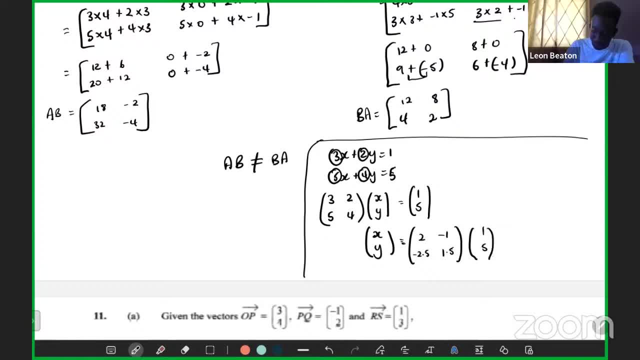 Sorry, One, five. Or do you put one, One five multiplied by that, This is a one, This is one by the inverse of it. Why, Why do, Why, Why? So there are two by one matrix and this is a two by two. 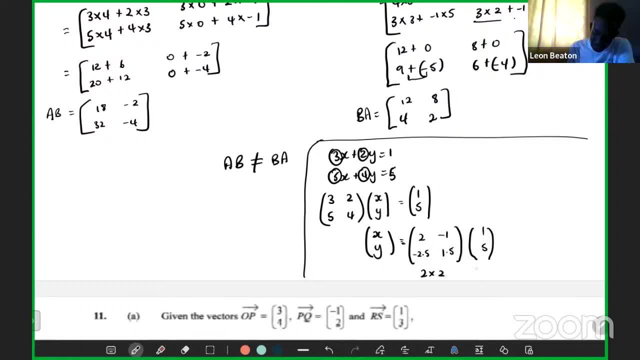 So this is a. this is a two by two matrix, And this is what This one is, what A two by one, Two by one, Two By one And good. How would that help us to determine where to put it? 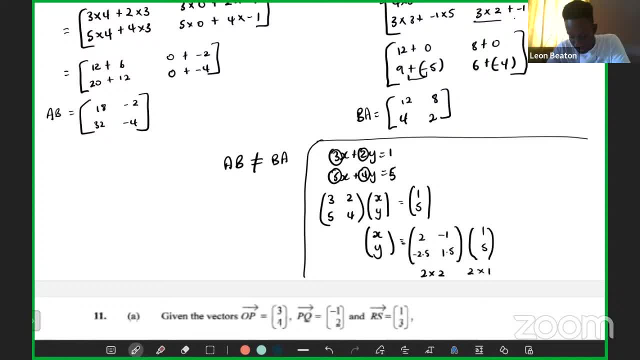 It has to be what the two matrix got to be. what for one? Pick me, John. Yeah, it must be compatible. And how can you tell if two matrices are compatible When you put it together? the inner, the inner arm number should be equal. 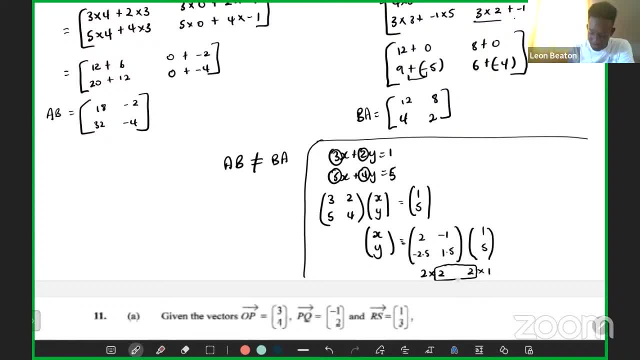 So those numbers got to be equal, right, Those two numbers got to be equal. There's got to be equal to this, And if we, if we had set up the other way, it would have been a two by one multiplied by a two by two, and a two by one multiply by a two by two. 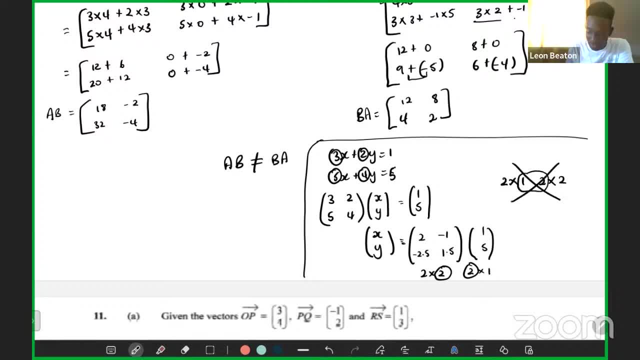 You see, the inner numbers are not equal. That means they are not compatible for multiplication. All right, So they must be compatible for multiplication. That is why you put it in front and not at the bottom, All right, So the R in this case will matter how you put, because if, if you put it behind, 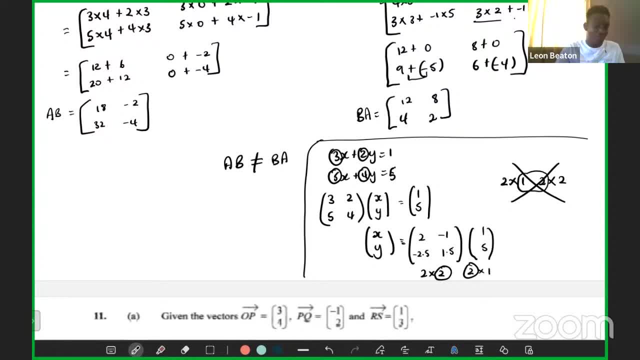 you as your work and you- you know you want to- why you're getting the and so on. you know you get frustrated and so on, so they must be compatible. So you put it at The front: uh, so you're running out of space. 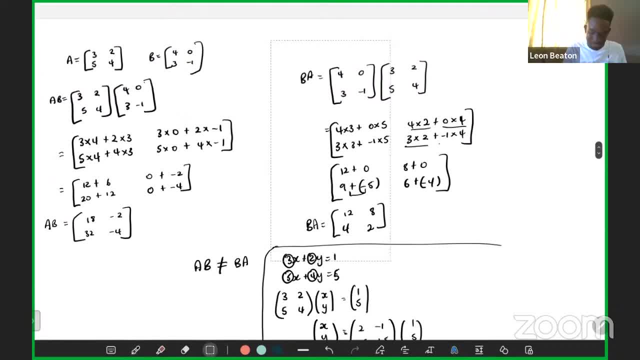 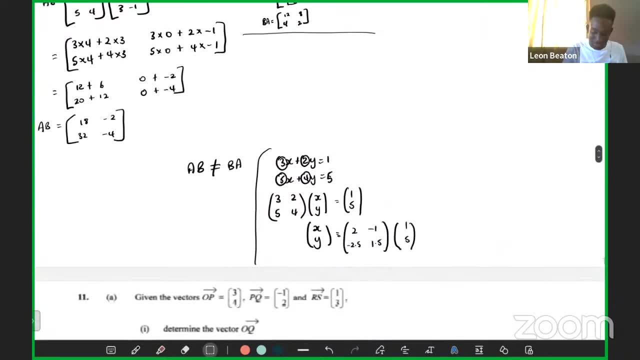 So let me see how I can create some space. So I'll do. we make this a bit smaller, make it a bit smaller And let me- here is this part- and make this a bit. let me drag this up. We drag it up a little bit here. 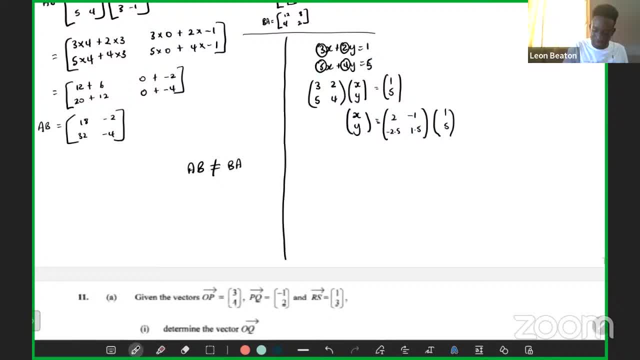 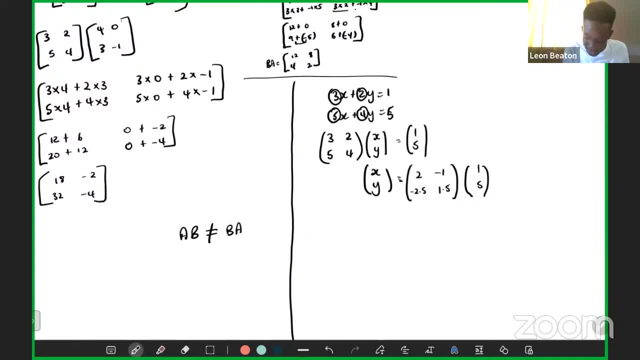 All right, Let me do some separation. Yeah, I know, we Multiply, So our next thing to our next thing. Um so we have a two by two and we have a one, um a two by one, right? Two rows, one column right. 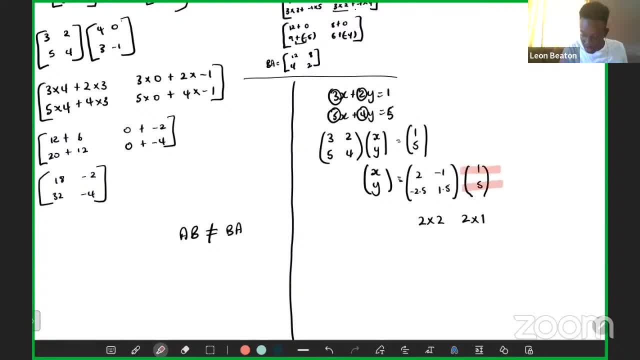 That's how we get two by one, two rows, one, two and one column. That's why it's a two by one matrix. So we have a two by two matrix. We know these two matrices are compatible. but the next thing, um our next problem. 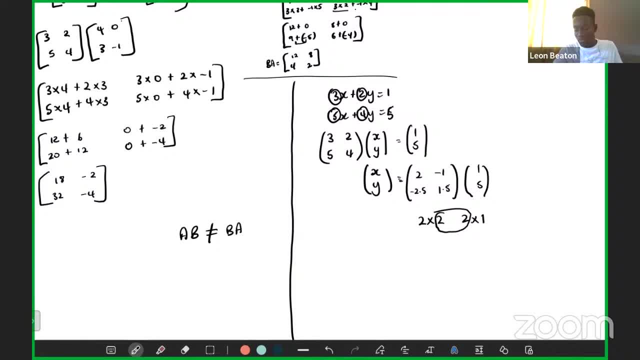 that many students may um reach up in. you want to know. okay, when You multiply a two by two and a two by one, what would, what would be the order of the matrix when you multiply them By one? 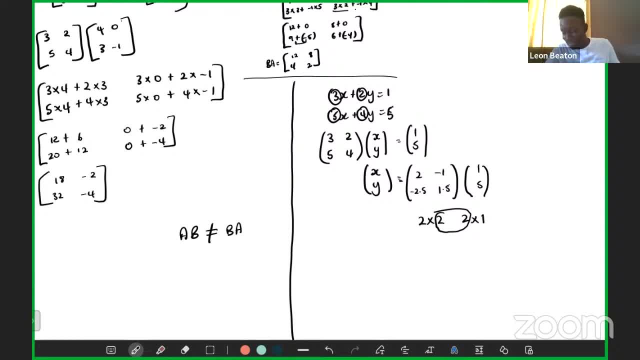 Two by one. How you got a? two by one, You're correct. How do you, how do you know it's two by one? Sorry, because um, the, the outside, um volumes, Yeah, Yeah. So these two here, these two outside matrix, will determine. 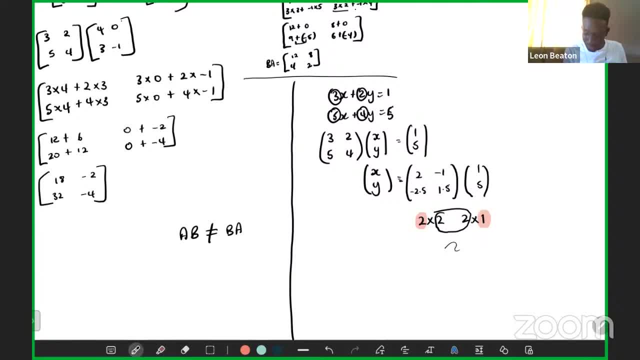 Um, what would be the the? the product of the two matrixes is two by one, So they use this as a guide when you're multiplying. when you multiply two different order of matrix, the outer numbers will dictate what would be the order of the. 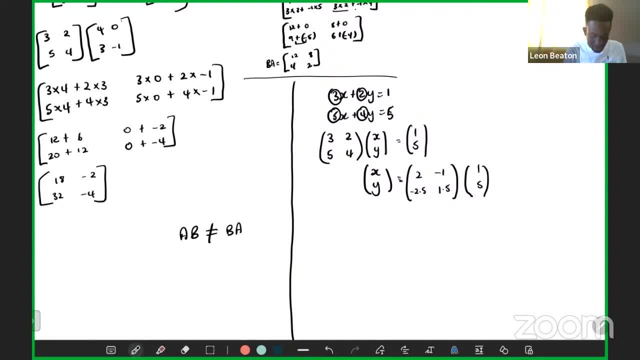 Right, So we'll have a two by one matrix as our answer. So let's work it out now. So this would be two row by column, two multiplied by one plus negative. one multiplied by five tends to be negative: 2.5 multiplied by one plus 1.5 multiplied by five. 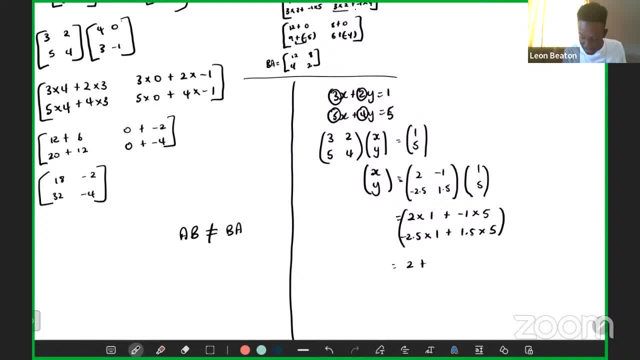 And then we work this out. You'd have: two times one is two plus negative one times five would be negative five and negative 2.5 times one be negative 2.5 plus 1.5 times five. Negative 2.5 plus 1.5 is one. 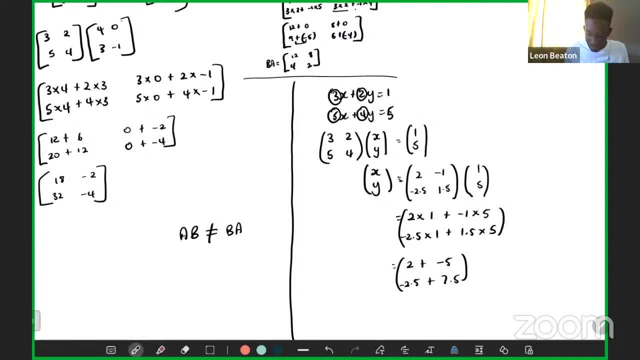 Positive three is negative: two plus 5, 0.5 minus 1, 0.5 minus 7.5, 10.5.. Negative 3 is negative: 2.5 plus 3, 0.5 minus 5, 0.5 minus 7.5.. Negative three is negative: 2.5 plus 4, 0.5 minus 6,, 0.5 minus 6,, 0.5 minus 7,, 1.5 minus 8.. X, X, Y is equal to that. 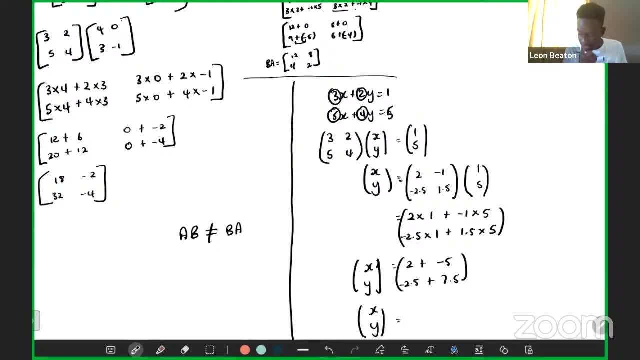 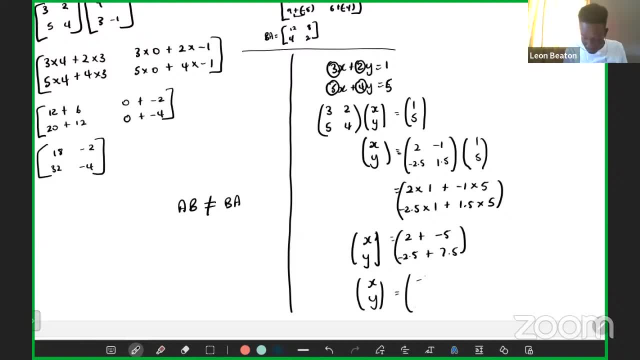 So X, Y would be, uh, two plus negative seven, two plus negative five, Sorry, Negative three, Negative three and negative 2.5 plus 7.5 would give me Five, positive five, Positive five. Okay, Yeah. 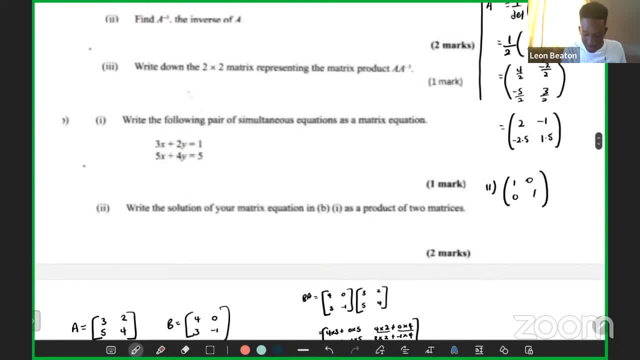 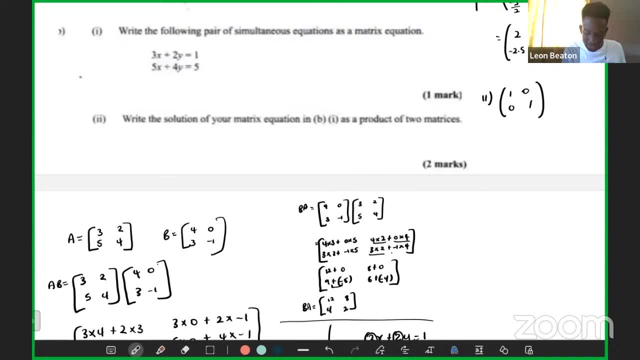 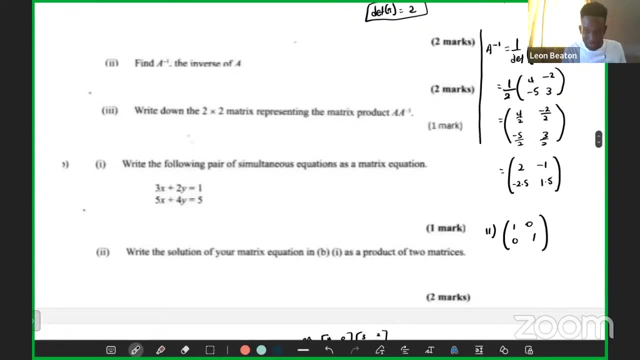 Okay, Okay. so let me see. did you say: write your solution as a product of? yeah, but then again the question said: write your solution as a product of two matrices? did they say to solve it? actually, they did not say to solve it. you know well, we went ahead and and did some extra steps. they said to write it. 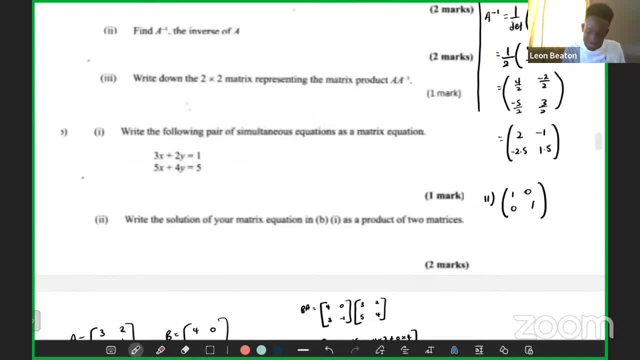 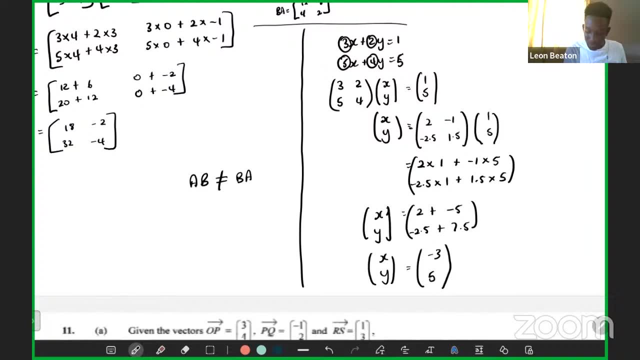 as a product for two matrices. anyway, that's all. it doesn't work. so, yeah, this would be our answer. the question, they really deserve it. i guess we could have probably stopped. um, we could have probably stopped at this step, right, so we'll probably stop at this step here. what are the? 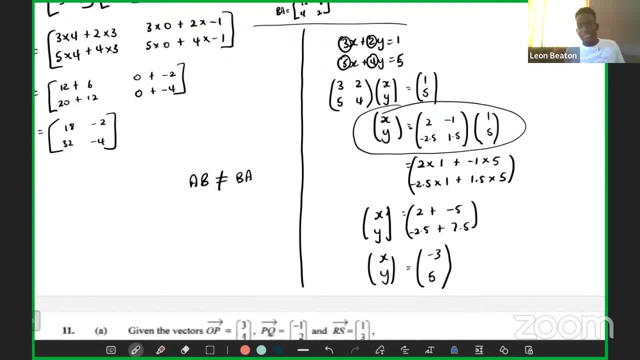 marks based on what the instruction is doing. but, yeah, to be on the same side. you never are. you know we're dealing with. you never know what will come in in this year paper, so this is how you solve it actually, right? so, yeah, but you could have stopped here based on what the question asked. 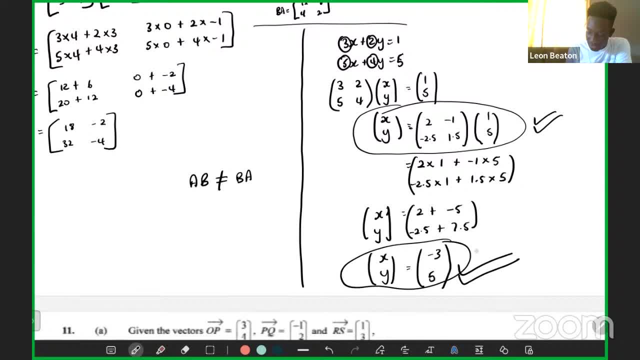 but yeah, this is how you go ahead and solve this and you can put in your answer, you can pull. you can say: x is equal to negative three, y is equal to five. you can say, therefore, x is equal to negative three and y is equal to five. 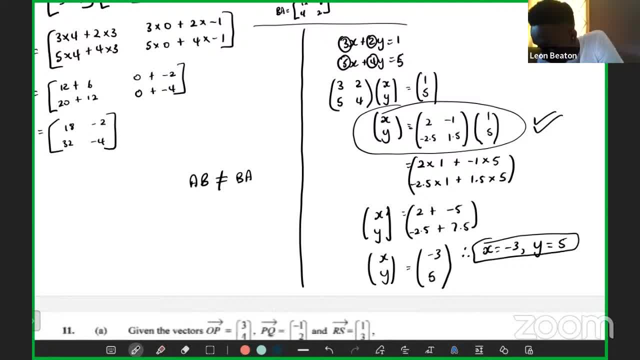 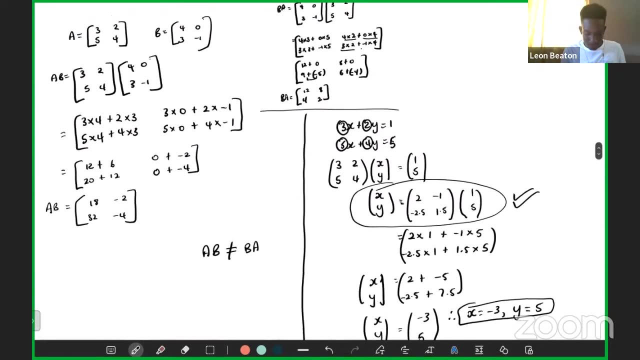 what year paid for? no, i, we don't. we have some random years put together. we- i just pulled some random questions across different topics, so there's no specific year. every person who asks that, all right, so everybody go there and we're going to go through them, and we're going to go through them and we're going to go. 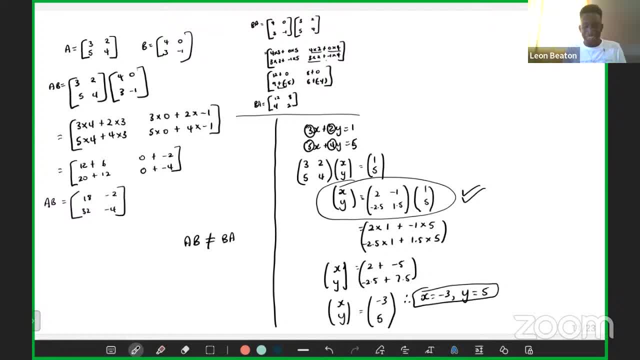 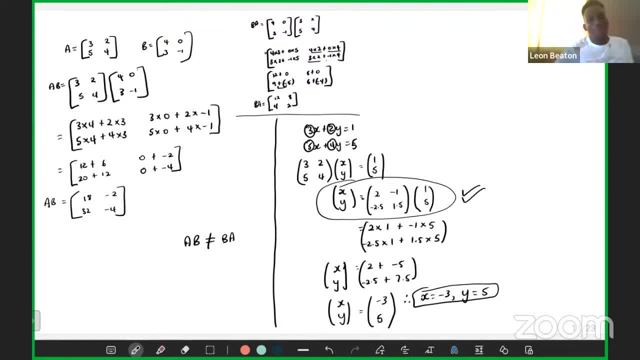 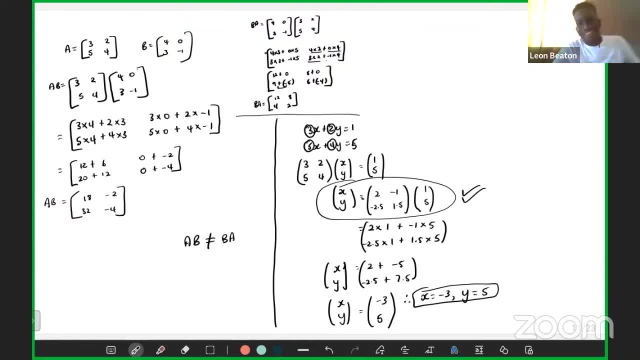 them and we're going to go through them and we're going to go through them and we're going to go through running out of breath. anybody running, anybody blowing hard. what is blowing hard? anybody ready, everybody solid, no thing. you, you're blowing, you're blowing hard. we need some water. 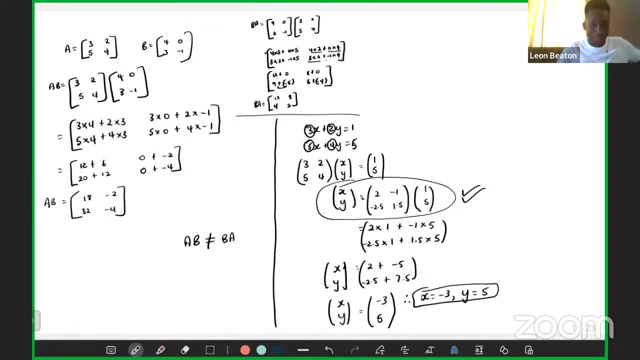 casey clark is running strong. somebody said they are all right. somebody said they are hungry. oh, you are. how you come to run a marathon, eating, eat man, you're gonna get blackouts. you gotta be happy, all right. so when you see, let's see, all right. they see a message wrong, all right. 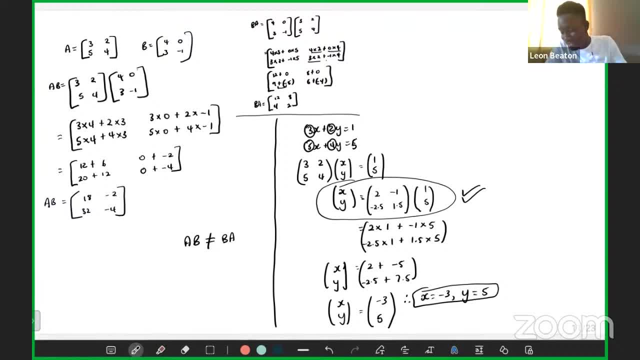 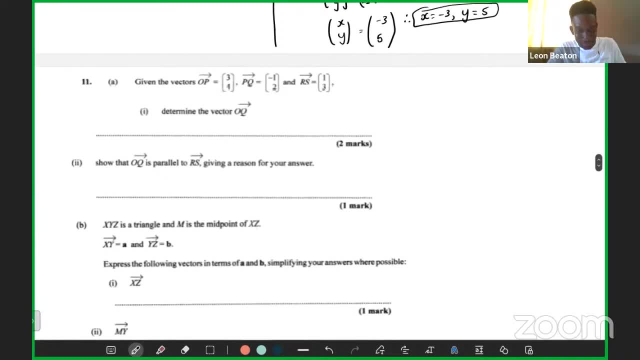 oh, casey clark said it and you know casey clark has been out with us since the beginning. case, the car is going strong, excellent, so let's let's carry on. maybe it's a marathon, right 100? is that 100 meter or a 200 meter? 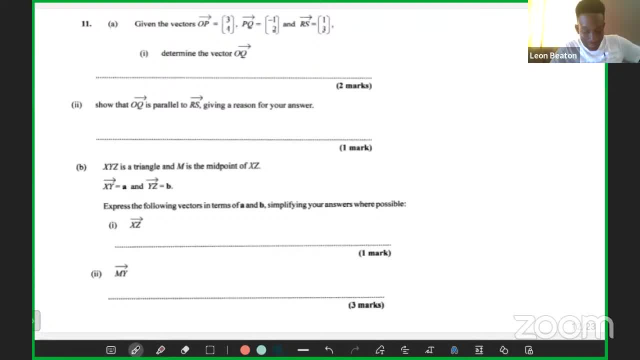 all right, so let's go um. so let's see. given the vectors, op is equal to three, four, and pq is equal to negative. all right, i like you, andra. mia pq is equal to negative one, two and rs is equal to one. determine the vector: o, q, o, q. 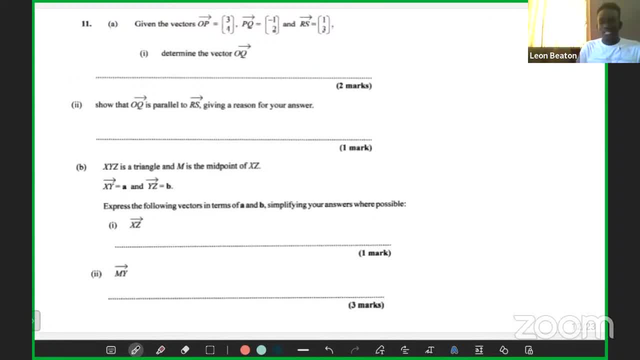 so let's see, we have some vectors. now we move from matrices, the matrices have matrices. vectors and matrices- they're going hand in hand. you know, i think there comes under one topic in the syllabus: vectors, the matrices. so you can't do matrix without some vectors. 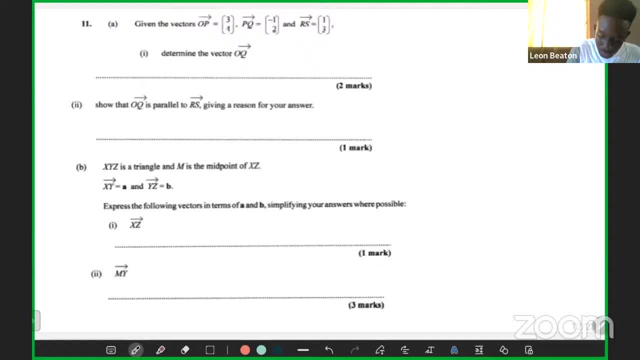 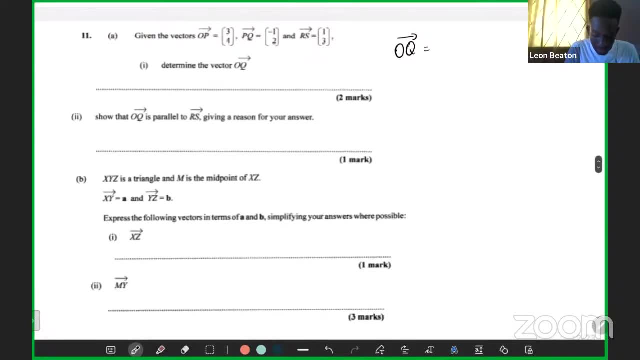 so let's see um determine the vector: o, q, o, q, oq, um. so what would that be? we got a vector op here. we got a vector pq, we got a vector rs. let's see who can remember. how can we find oq, two marks. anybody who's with me here? how can we? how can we find open? 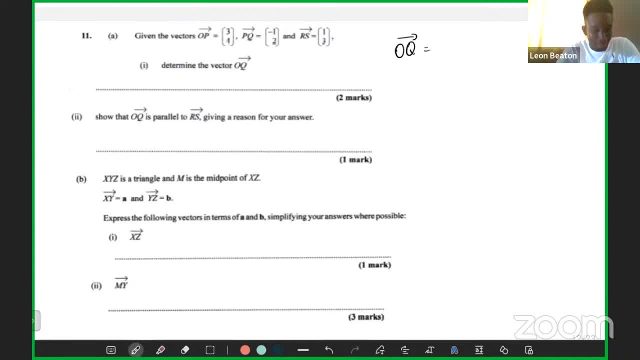 open. ah, ah, all right, let me help you out. remember oq. you gotta move from o to q, so you gotta find a vector, find two vectors that will help you to move from o to q. all right, so let's see, we can start off with op, so we can say: oq is equal to op. 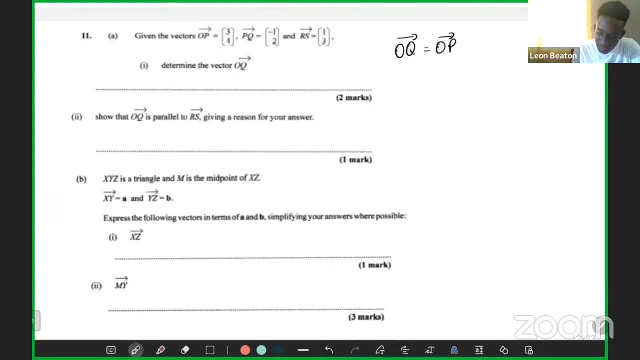 is equal to op to move from o to p and we add that, so we move from o to p and then we can move from p to q, because we gotta start with oh and we gotta end up with p, then you can go from p to q. 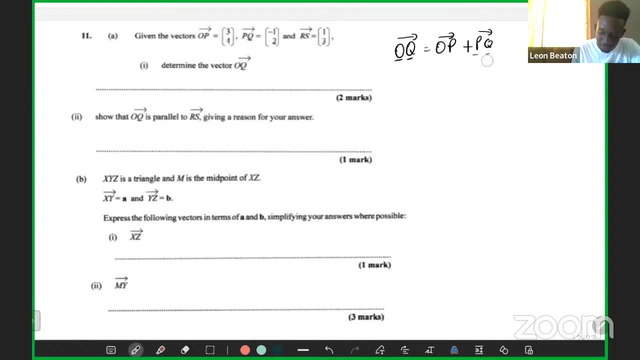 from o to p and then from p to q, and that's how we can find that vector right. you know the force, force and like what can i say or select? the first point in the vector tells you where you start from. the last point tells you where you end up. 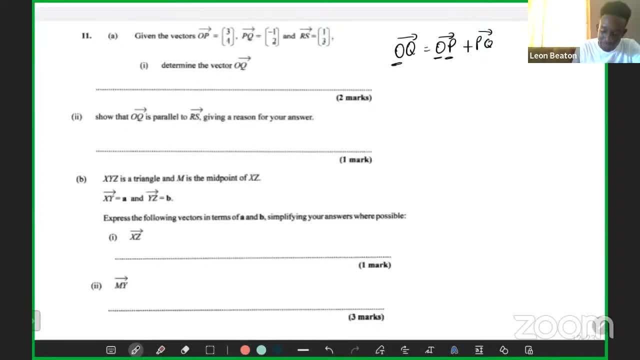 so you can start off with o, so you go o2p, and then from p you go to p to q. all right, these two letters gotta correspond triangular anyways. so that is how you can find that. so we're not working on a specific gear for the course of that. so from o to p, p to q, so we know op. 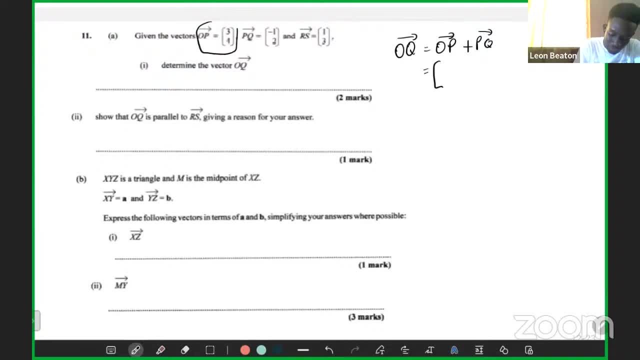 is equal to. they gave us op to be equal to three, four, this would be three, four plus pq. if i'll pq to be negative, one, two, this would be three plus negative one. or four plus two would be three plus negative one would be three plus negative one would be two. or four plus two would be six. 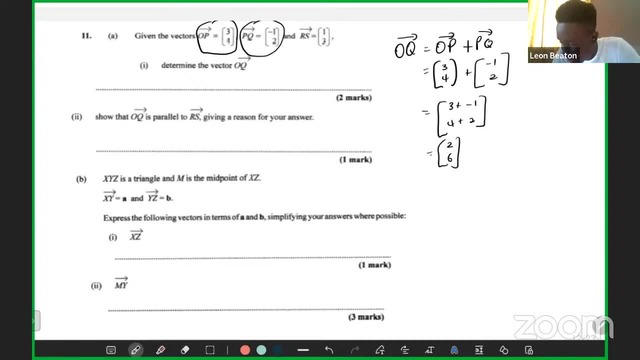 as i see casey clark saying in the chat on facebook. all right, the folks with me here. yes, sir, yes, so that was a refresher, right, that was a refresher for everybody, or it wasn't? yes, sir, oh, i chose that. you are, you have been refreshed and it's it's now. 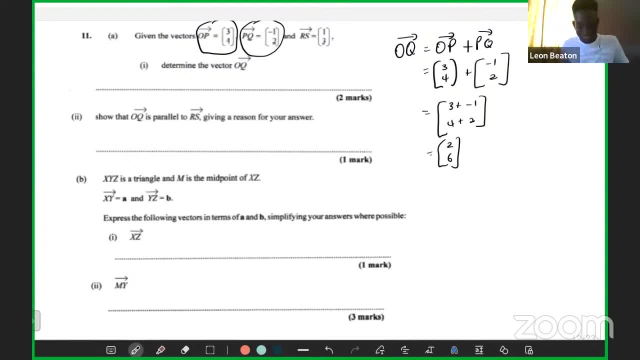 fresh in your head and you stay there, all right. so, yeah, the the points. you use them as a guy. you start from oh, you go from oh to something and then from that something to the last um point in the vector that they ask you to find. all right, so from oh to a point and then from that point. 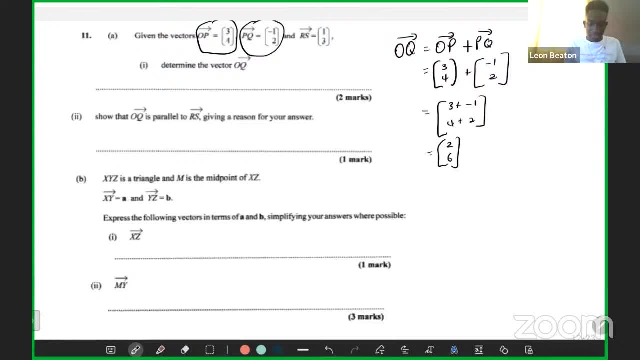 to the vector, to the point that you want to stop at all. right, good, so show that o o q is parallel to r s. so you got oq, so this is oq. this is the vector oq and the vector r s would be one. three. 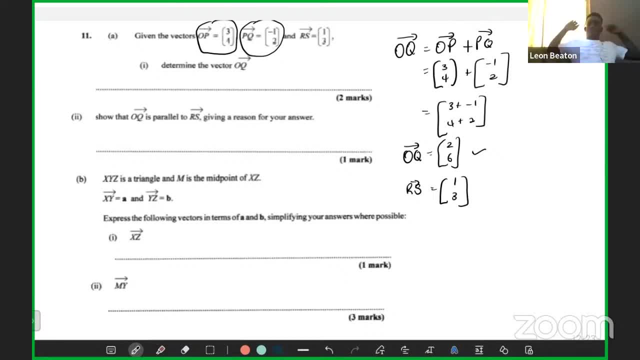 so how can we show that those two vectors are parallel? how can we be sure that those two vectors are parallel? look at them good and think about it: parallel vectors. like i hear the books flipping, i here the pages flipping. let me see if anybody in the chat can give me before somebody. 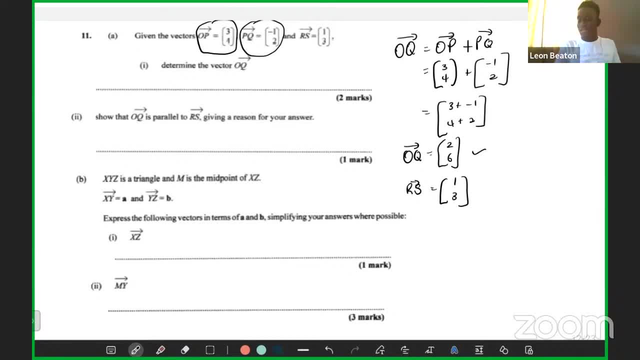 somebody else tells me in in sorry scale or multiple, all right. scale r, multiple, all right. let me see if anybody in the chat can give me, before somebody get somebody else tells me: in this I think we'll scale our multiple, scalar, multiple, so one vector must be a scalar multiple of the other. 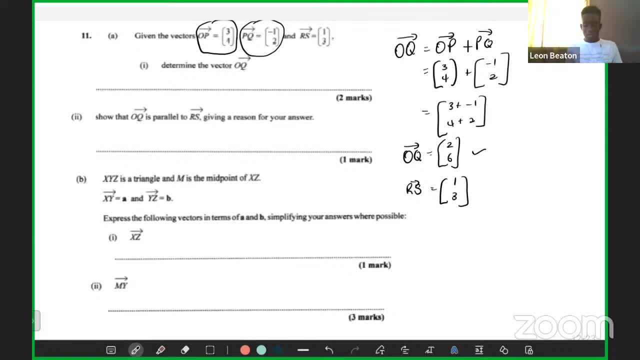 and do we have that in this case? q, q, o, q and rs? yes, so which one is a scalar, multiple of which, and what is the scalar? what is the scalar? we got two, six and one, three. what is the scalar? what is? what is what can be multiplied by what? to give you the artifact, though, 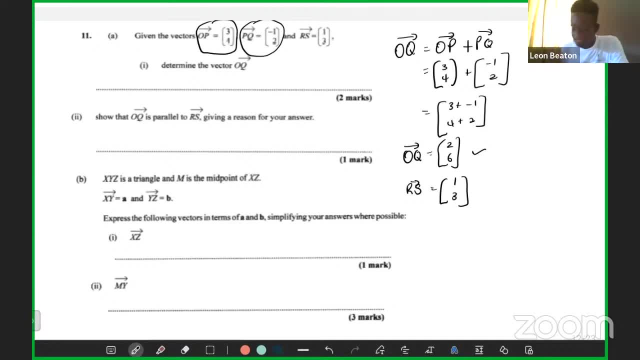 one rs. rs is equal to what? can we multiply by rs to give you: hi, jamal prince, jamal, prince, jamal jamal. why are you not in this class? why are you not in this class in the chat, sorry? no problem, jamal llamas, you're there. yeah, so we can multiply our s by two. 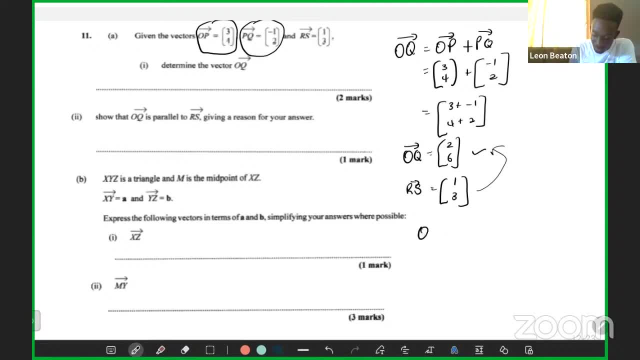 so we can say: uh, you can say: um is equal to two r s, oq is equal to two rs, and that's how you can tell if two vectors are parallel, one must be this: a scalar multiple of the others. all right, one must be the scalar multiple of the other, and that is. 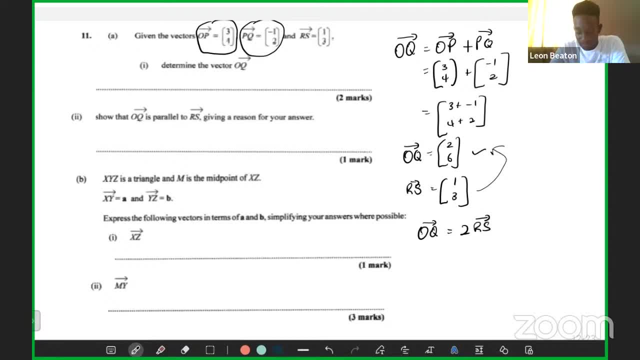 how you can tell if they are here are multiple of each other. and a scalar is just a number and you multiply one vector by a number to give you the other other vector. all right, now you can tell if two vectors are parallel, all right, so one must be a scalar multiple of the other. on the scalar. 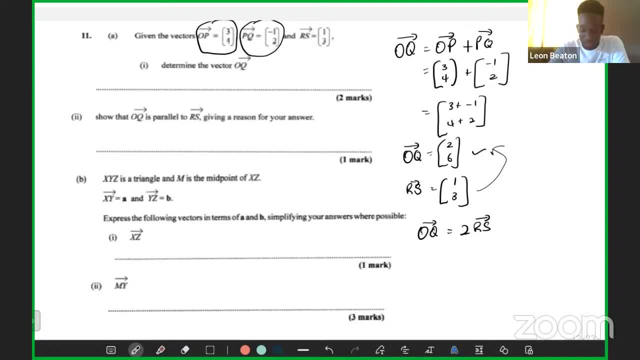 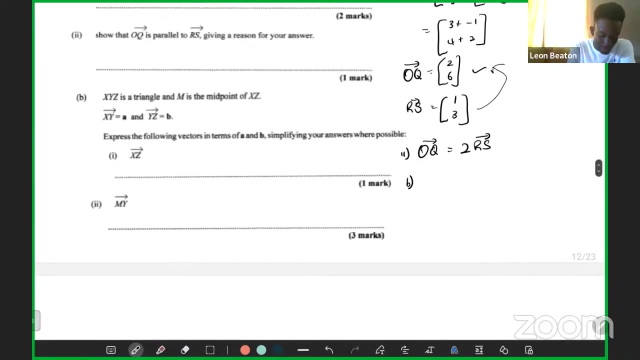 just a number, like you, multiply by the other vector. that you have all right. so that is that. One mark, simple one mark, right? This is I, I, So let's go B. So B says X, Y, Z is a triangle. 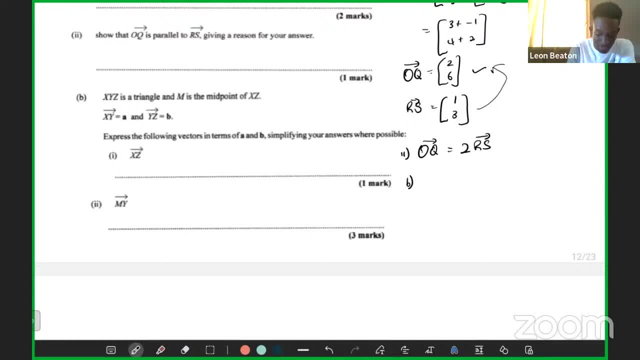 And M is the midpoint of X, Y, M is the midpoint of X, Y, X. Y is equal to A, Y, Z is equal to B. So let me draw the triangle for us about. So we got a triangle. 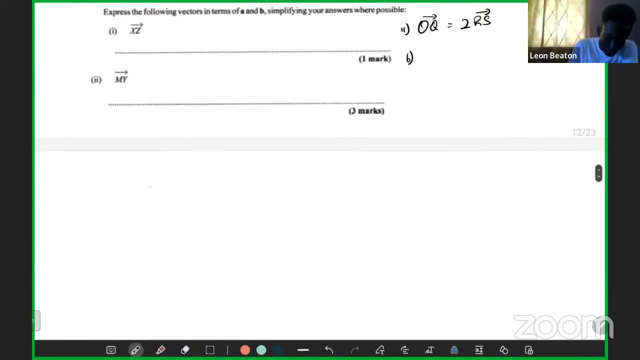 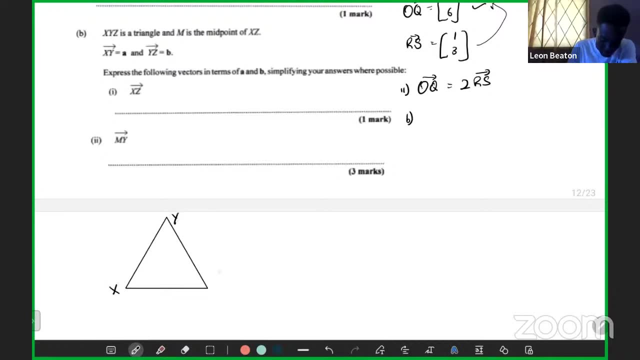 Got a triangle. Let me draw the triangle. Good, So you got a triangle: X, Y, Z. So we said that X- Y is equal to A And Y, Z is equal to B. So they want us now to express the following vectors: 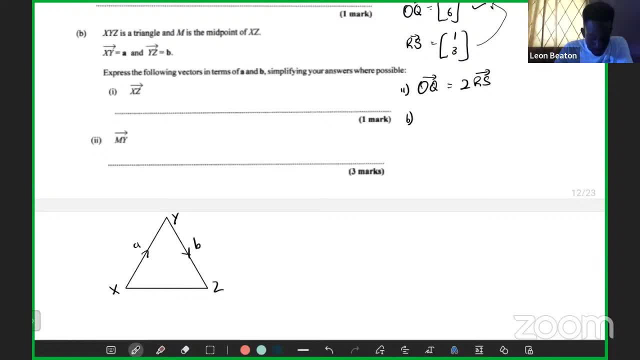 in terms of A and B. simply find your answers where possible. So X, Z. So they also told us that M is the midpoint of X Y. So X Y, M would be here. M is the midpoint, Pardon me. 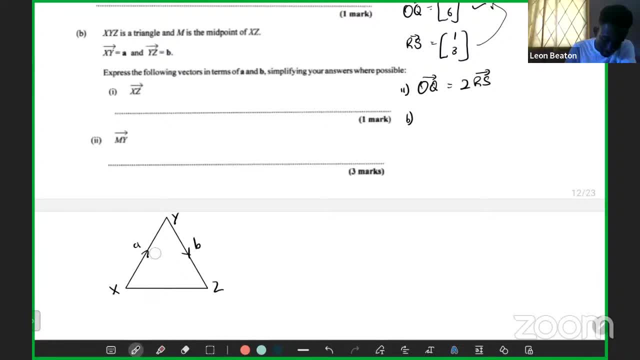 X, Z, midpoint of X, Z. All right, that is what I got out here. So X, Z. So X Z would be the midpoint. There would be M right X Z. Good, Good, So they want us to find X. 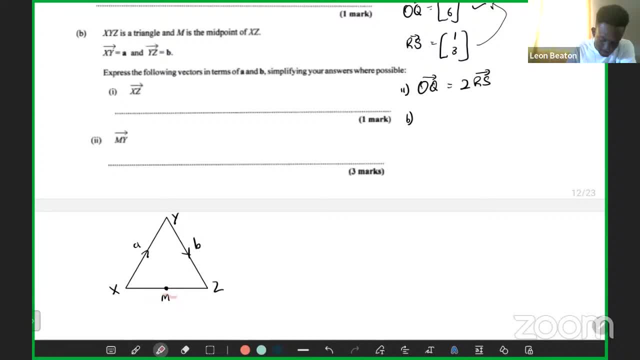 X Z. So X Z or Z X Z would be here. You're going in that direction, All right. So to move from X to Z, we see we can go across The triangle. we complete the triangle. 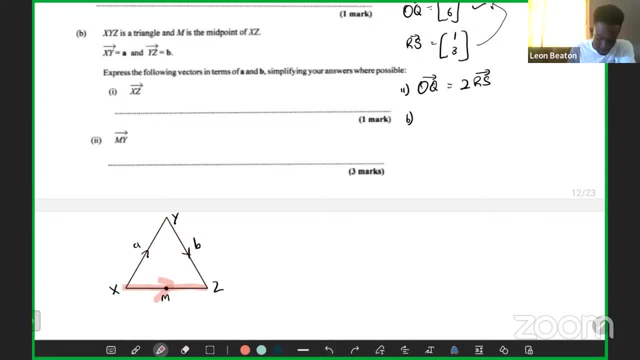 We go from X to Y and then from Y to Z, So X Z would be simply equal to X Z, As it says. one mark would simply be equal to, in terms of A, and B would simply be X. 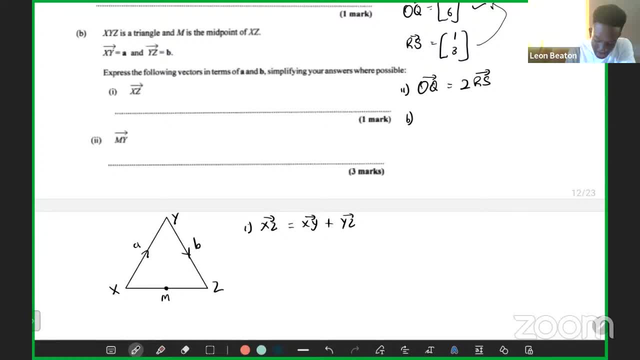 Y plus Y Z and X Y, which is equal to A plus B. All right, That is X Y, That is A plus, That is X Z, A plus B, Simply A plus B. And the last one, we want it by three marks. 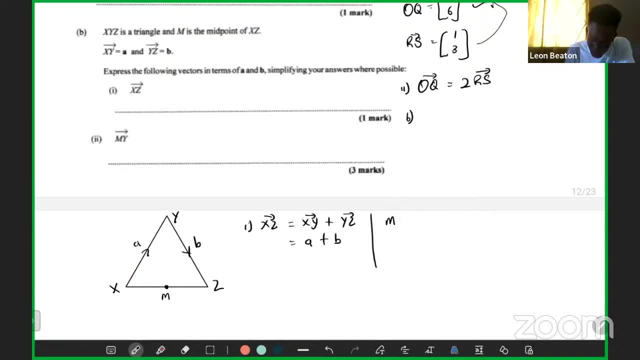 Three marks, Remember I said about three marks earlier. M Y, So you've got to move from M to Y, From M to Y. How can you find for M Y, Where do you move from, From where to where? 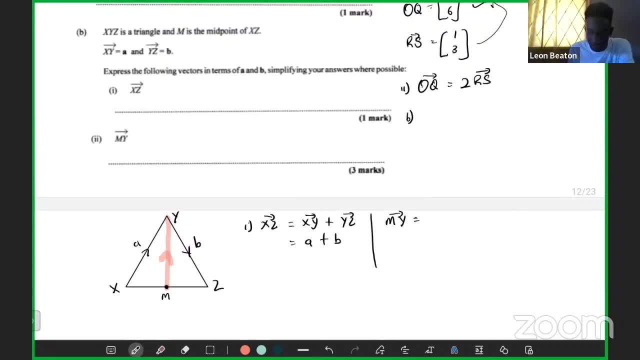 You move from where to where and then from where to where. So we could move M, X and then X, Y, or you can move the other way to M. So yeah, Let's just do it Easier part. 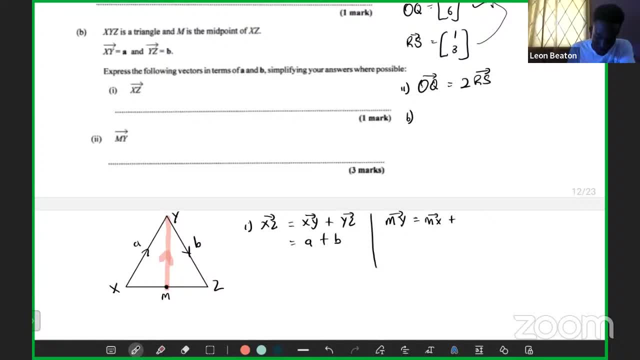 So we can move from M to X and then we can go from X to Y. All right, So we can go from M to X, from X to Y. So the thing about M, X, M is the midpoint of X, Y, right. 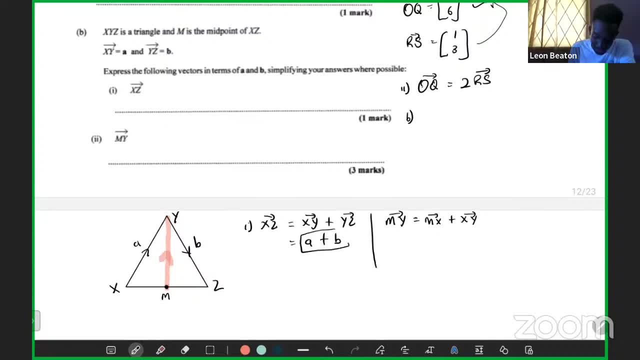 Well, X Z, And we found X Z to be this at the bottom here, right. So if you want to find the midpoint of this, midpoint means halfway. what can we do to A plus B to get half of that? 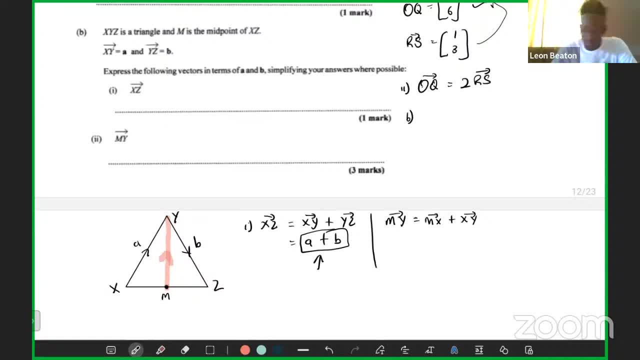 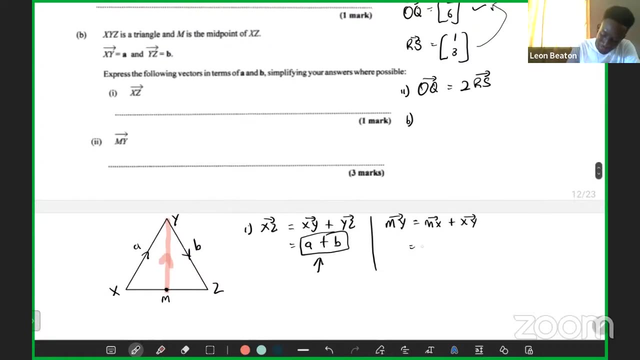 I mean, I kind of gave you the answer in the wording: How can we find half of A plus B, Everybody half of A plus? It'd simply be half A plus B, right? Half A plus B plus Yeah, divide by two. 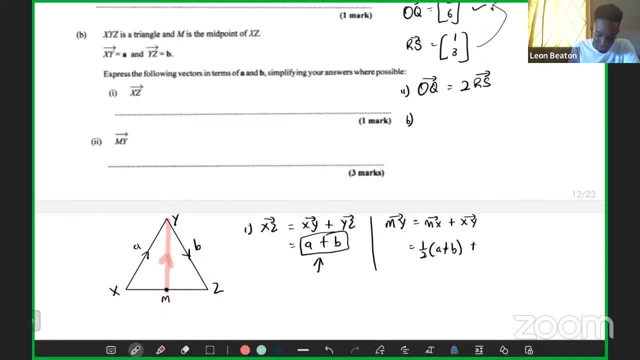 So you have half of A plus B plus X Y, And we know X? Y is simply A. So it says to simplify where possible. so we have to simplify this. So this would be half of A plus B. This half we're going to multiply everything here. 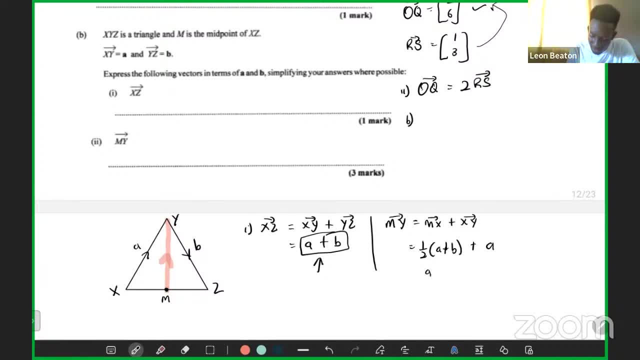 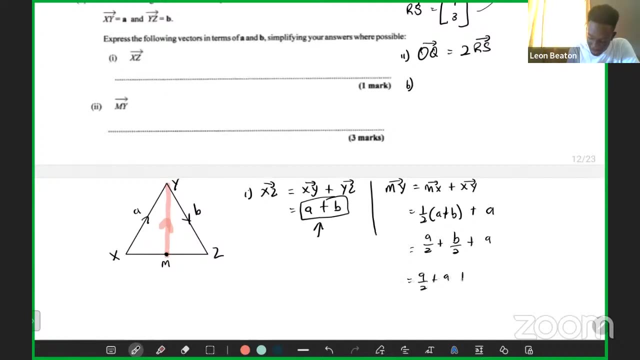 So this would be half times A, would be A over 2, plus half times B, would be B over 2, plus A. So we can put the A's together. This would be A over 2.. A over 2 plus A plus B over 2.. 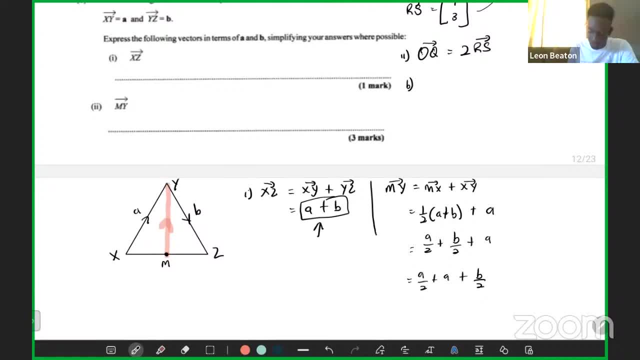 So A plus A over 2 plus A over 2 plus A, That's like half A plus A Right, Half A plus A Right, Thanks Yeah. so a over 2 plus a is like half 2a, sure man. 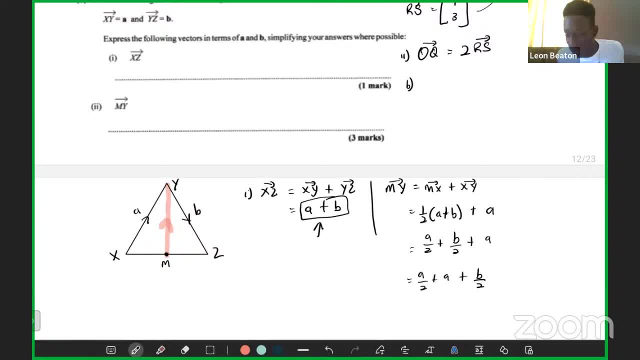 Half plus 1.. Half plus 1 is what He's like. let me write it back. He's like: you got half a and this is half b, right? So half a plus a. If you got half of a cake and then somebody gave you a whole of a cake. 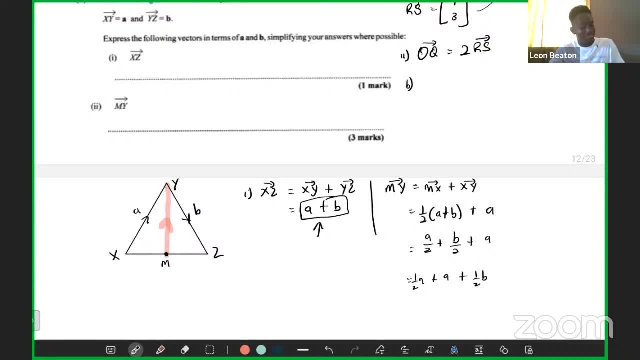 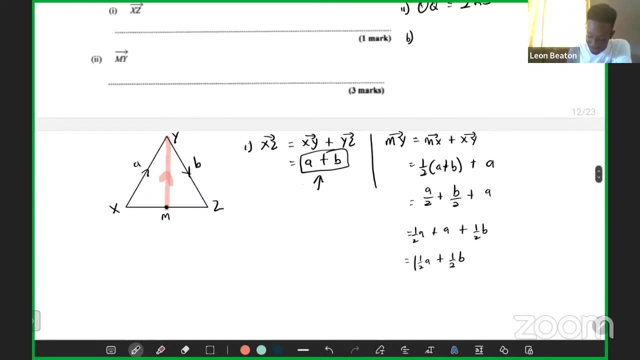 you're going to get half of a cake. Sorry, one and a half, Yeah, one and a half, right. So you can say one and a half a plus half b, right? Or if you want, it can be 3 over 2a plus half b, right. 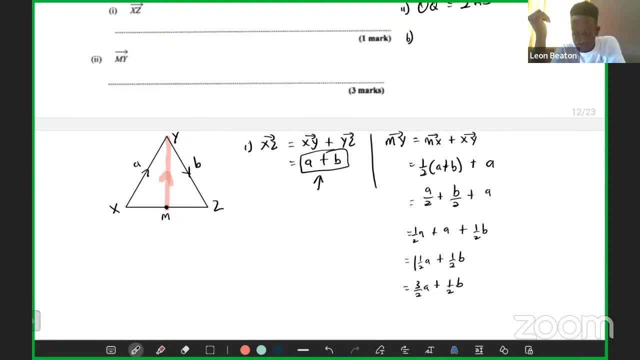 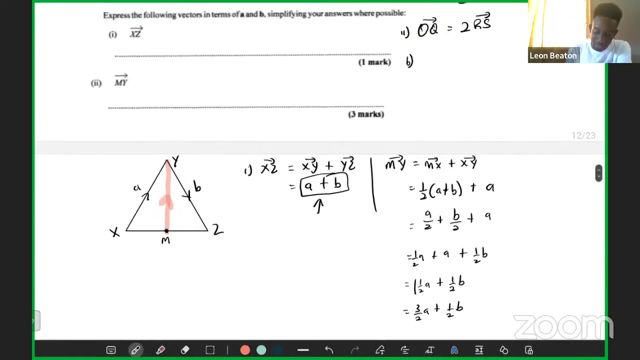 So half plus 1 would simply be one and a half. All right, You might go there. Yes, sir, Yeah, So it's just a simple combination of what we found earlier. You take half of that and you add a to it. 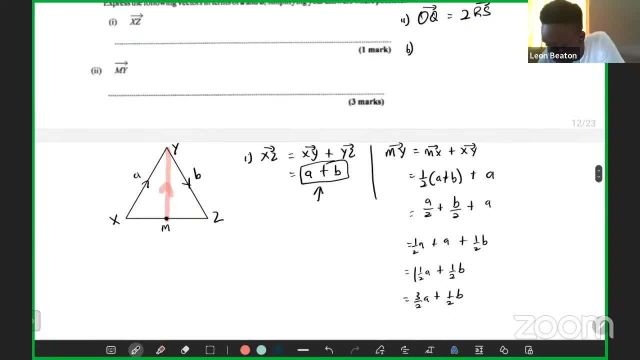 And that's how you find this vector All right. So Casey Clark is saying: you're good One and a half, Julius, Anyways. So that was it for vectors. So this was a nice refresher. Vectors, it's simple, right. 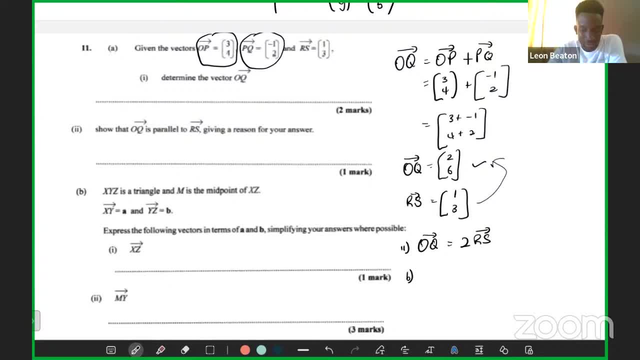 For some reason, students tend to fumble in these kind of questions- Vectors and matrices- But most times these things won't have too much application. You don't have to do too much, It's just a matter of remembering how to work. 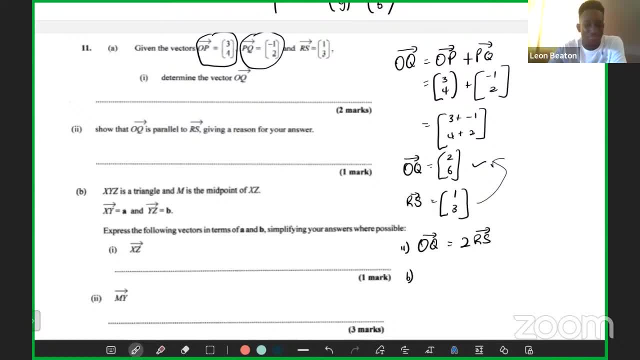 As we list out the other topic areas like measurement and so on. you got to do some amount of application. These kind of vectors and matrices is just a matter of remembering what to do, Some amount of application, as we have to do, But mostly it's kind of remembering and computational knowledge. 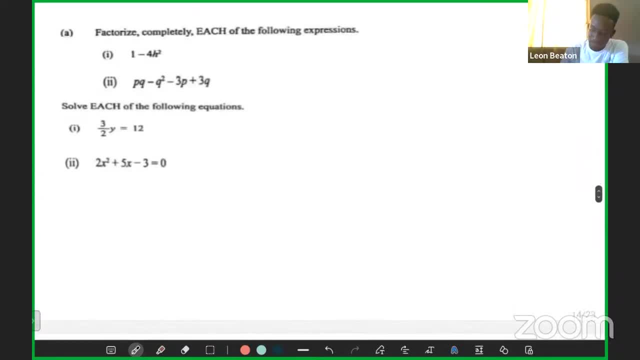 All right, So let's carry on. Let's carry on to some factorization And some solving of some equations. We've been solving equations this morning, but now let's start with some questions directly related to solving equations and factorizing. So we have two nice and easy factorization questions which everybody should finish in under 30 seconds. 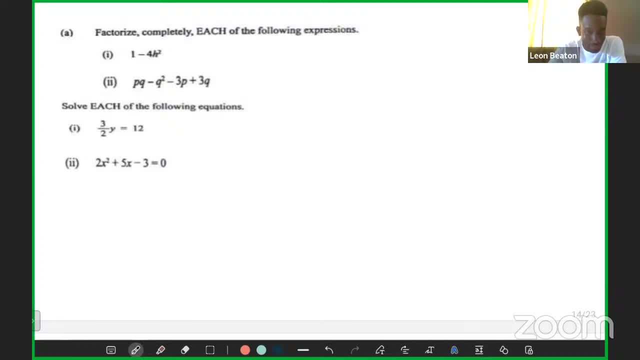 When you see these things, you should start smiling immediately and know that it's free marks. So factorize completely each of the following expression: So you have one minus four h here. So one minus four h And you want to factorize this. 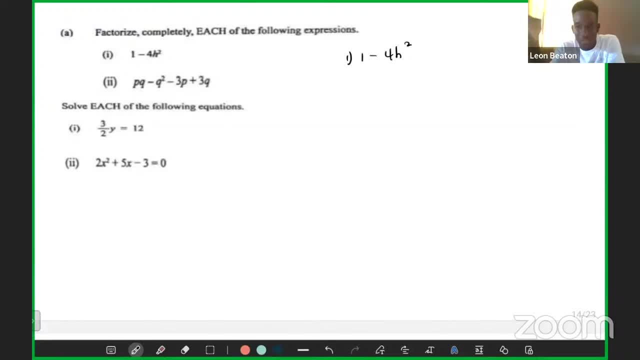 When you think about factorizing. when you think about factorizing, you should be thinking about two factors multiplying to give you the original expression. All right, So how can we factorize this One minus four h squared Using the difference Timeshift two squared? 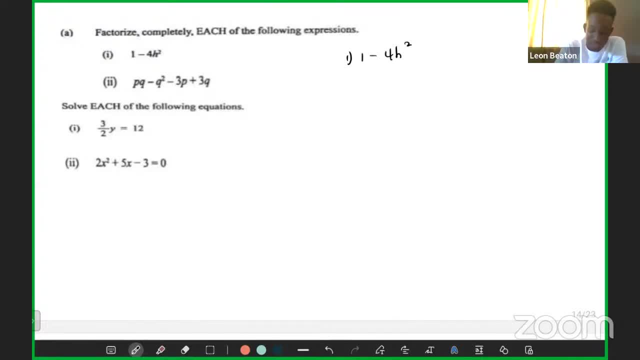 Difference of two squared Right. So difference of two squared. First of all we got the name itself: difference of two squared. Difference meaning two things must be: subtraction, Two meaning you have two terms, And squared meaning you have two squared terms. 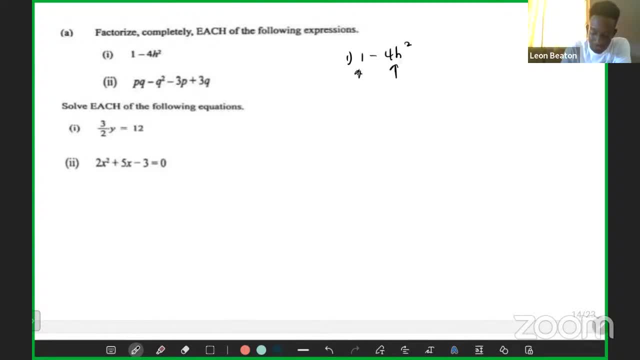 So we have one, We have four h squared. We know we can multiply something by itself to give you one. One by one will give you one. And we know we can multiply two h by two h to give you two h squared. So it's the difference of two squared. 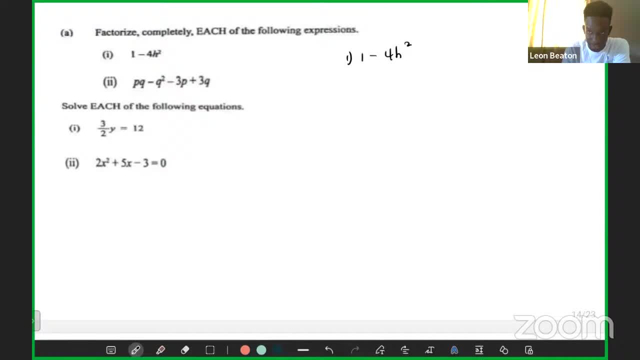 Difference meaning subtracting Two squared, meaning you have two squared terms. All right, That is the name of the topic- is in how you work it and what to look for. So we know these kinds of questions. go for one mark, because it's simply one step. 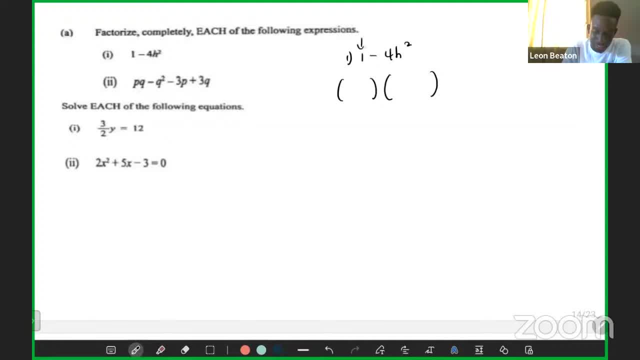 So you can open two brackets and we think to ourselves: what can we multiply by itself to give you one? You know, we can multiply one by one to give you one. So it's one there and put one there, And then we look at the 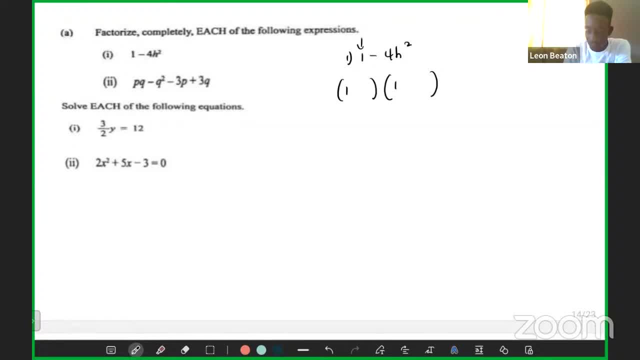 And we look at the four squared term. what can we multiply by itself to give you four squared? You see we can multiply two, sorry, four h squared. So we see we can multiply two h by two h to give you four h squared. 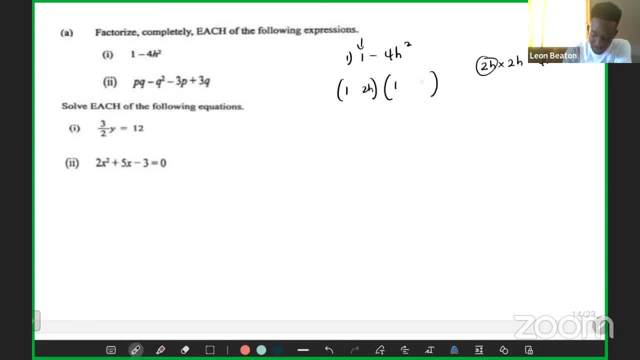 So we take it to h and we put it in here. We put it to h. Here is the one plus two h. one minus two h, one bracket to add in the other one You subtract. All right, So that is it for this question. 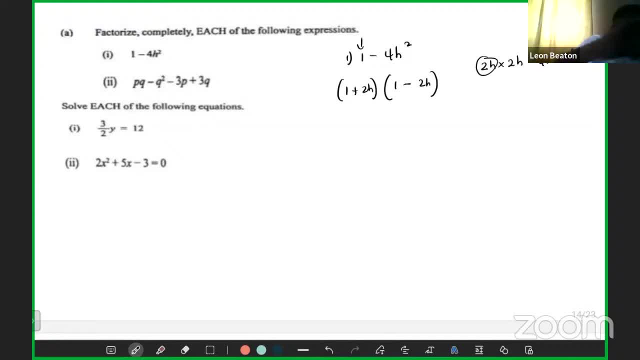 All right, so that is it for that question. For the next one, p q minus q, squared minus three, p plus two, sorry, plus three c. See somebody is saying: if you say is really quick comment, Don Sorry Tonya. 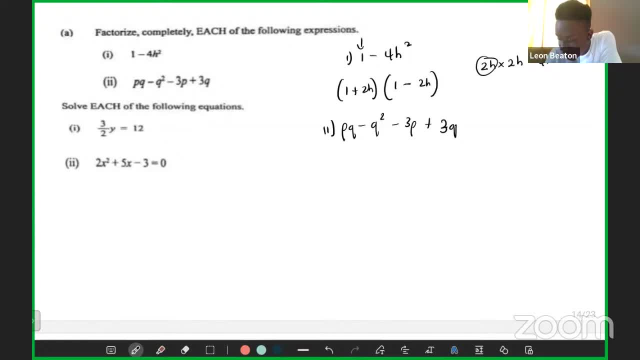 Don Don. All right, so if we want to factor this in p q minus q, squared minus three p plus three q, we have four terms. How can we factor this? Well, how do we factorize four terms? You can group it first. 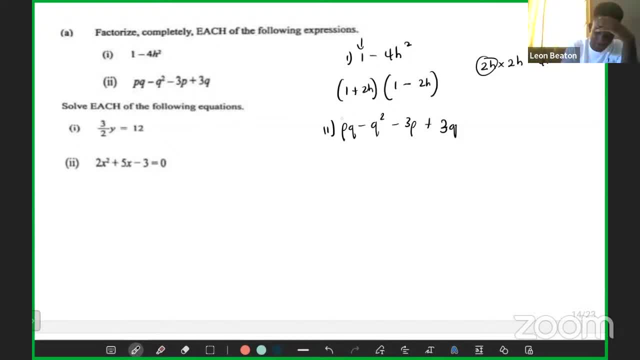 Yeah, we pair up right, We pair up All right. so we pair up And then we factorize the fours back. What is common, What is common in the fours bracket? Q, Q. So we see q is common, so we factor out the q. 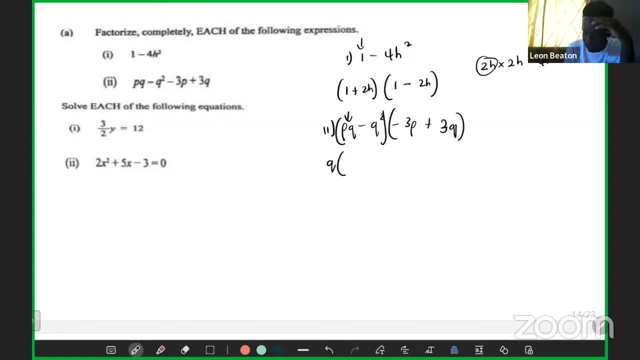 So we factor out the q from the fours term, What is left? p minus q. So we factor out the q from the fours term and left with p minus. we factor out q from q squared. By the way, when you're factoring out, it means you're dividing, right. 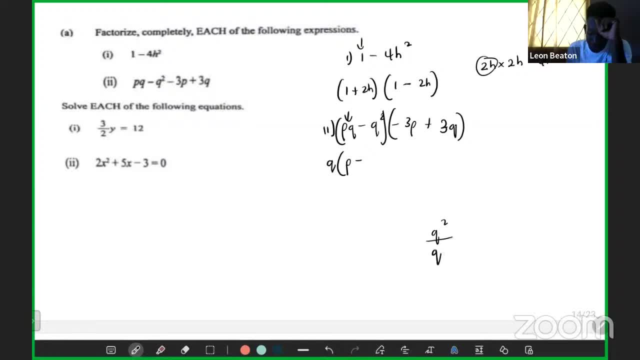 You're dividing the term by the factor. So we divide q by q squared by q. So this q cancels the one in the q. we're just left with q. And then the second bracket. now what is common in the second bracket? 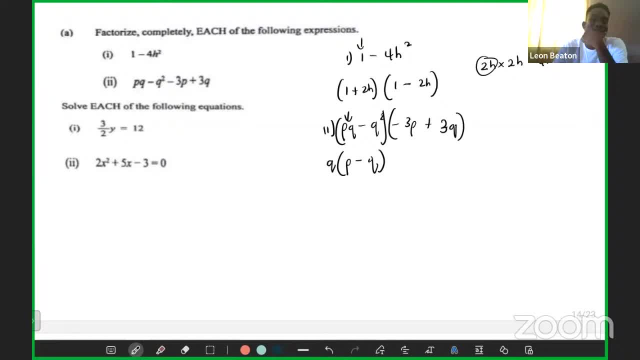 Tree Tree, sir. Hmm, tree alone, Negative tree, Negative tree. Now, a key thing to look for: when you have, when you see a negative, when you see a negative in the term you want to factor out, that negative sign right. 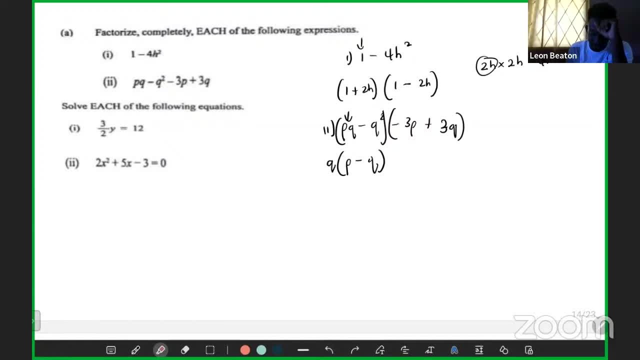 You see this negative here, factor out that negative all the time, right. So you always factor out that negative, So it will be negative. and then we see the common number would be tree, so the negative tree, And we factor out negative tree from this fours term. we see we're simply left with p. 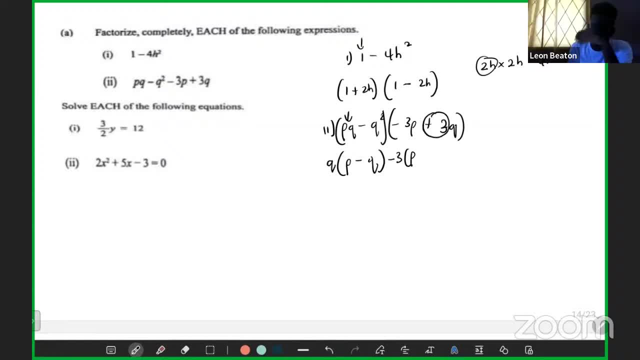 And then we factor out negative tree from this term. we're left with Negative q, Negative q right, Because tree p- Sorry, Tree q- divided by negative tree would be the tree would cancel out, And a positive divided by negative would be a negative. 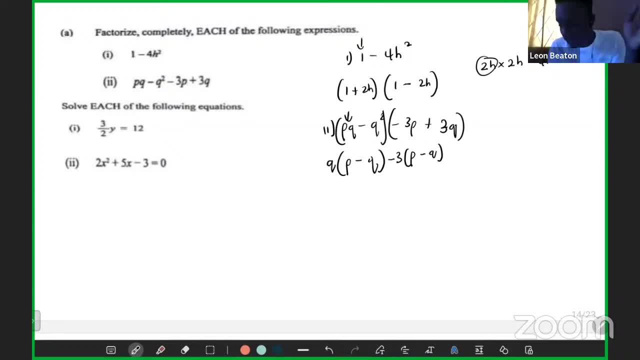 So that we have negative q or minus q. somebody may want to think of it. So the important thing, we see our two brackets are the same. See, we see our two brackets are the same. that means you know you did something correct. 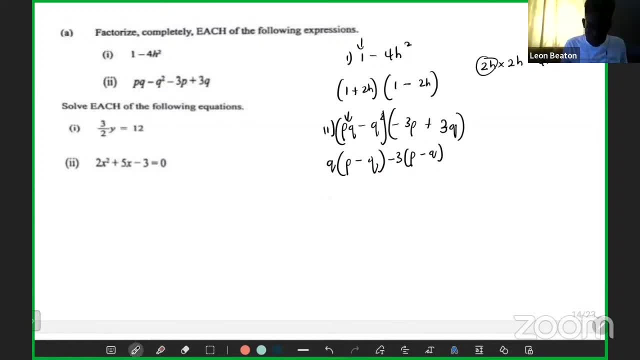 And then the last step is to take what is outside the bracket and put it in a bracket. So you have q minus three in one bracket. And we take what is inside the bracket and we bring it down. So it's going to be p minus q. 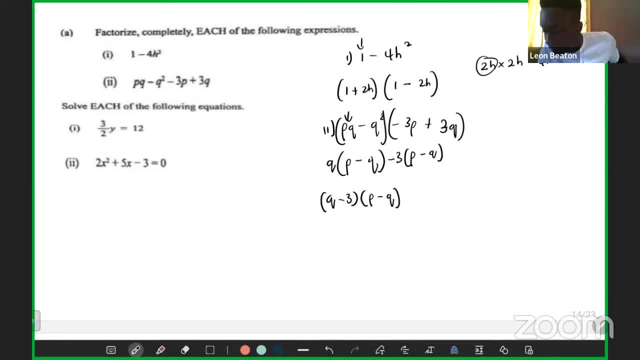 And that's how you get your two marks. All right, Simple as that. Yeah, You want to go there. Yes sir, Yes sir, Oh yeah, We are blowing Anybody. blowing Anybody tired? All right, Mark, we've been at it. for how long do you think we've been at it? 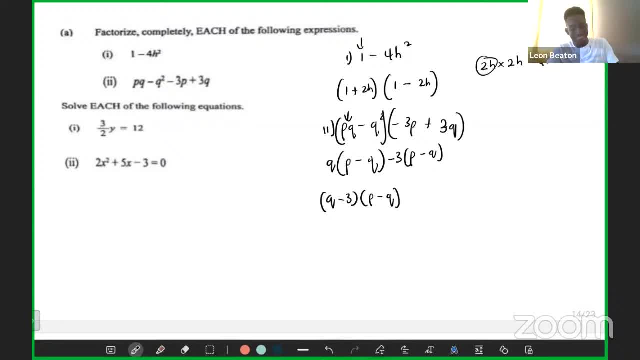 So long, Seven weeks, One hour and a half. How long do you think? we've been at it for? An hour and a half, One hour and a half. Two hours, thirty minutes. Two hours, thirty minutes. Let's see, Much is one. 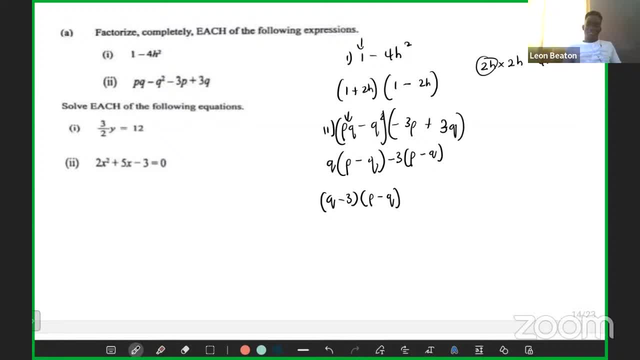 We've been at it for six hours. Six hours, We've been at it for six hours. Anybody believe that? I just look at it. it's not been six hours. Let's try it again. Six hours, Let's try it again. 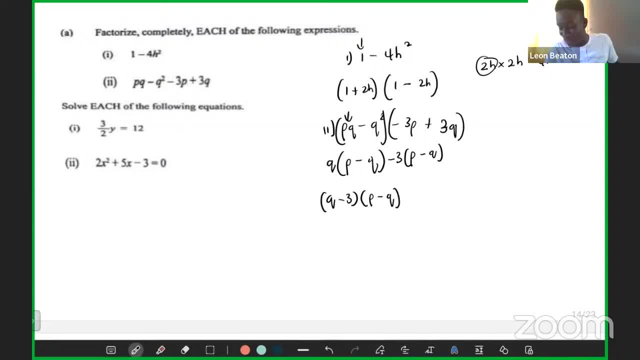 Let's try it again. been two hours? all right, we hit the two hours. mark this, nicola. two hours for me it felt like i, i felt as though we just locked down. i don't know anybody else felt the same. all right, just me alone, me alone. yeah, leave me hanging, okay. no, sorry, me too, all right. 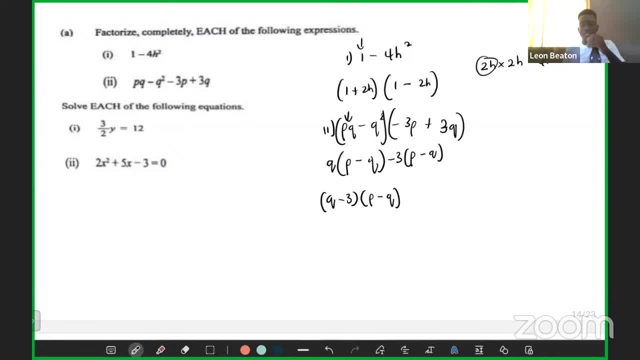 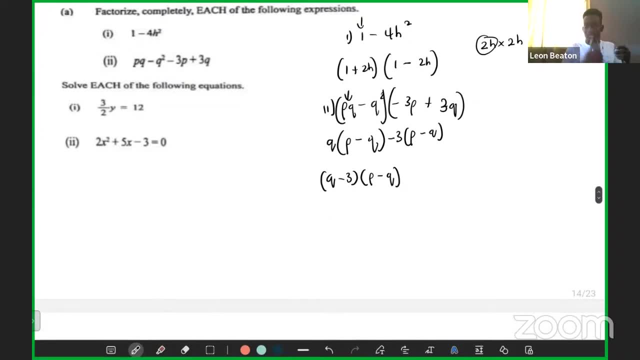 all right. so, yeah, it's been two hours. it's been two hours. i have two good hours, two productive hours. so we, i think we, yeah, we come in, we come into the ending part. i mean it's a marathon. let me call a name. and somebody said to me that um, 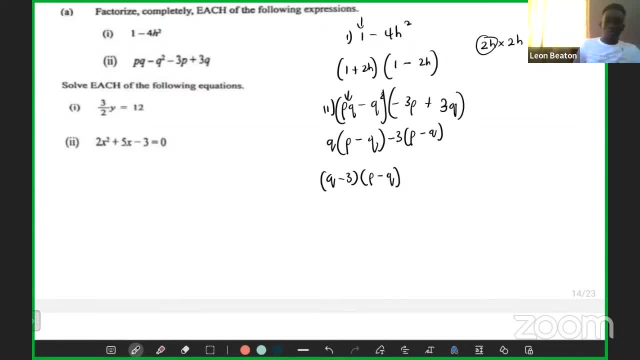 they will stay here for the full thing. that horse is still here. yeah, nicola's in, it's felt, it felt like a 30 minutes, all right. so let's, let's, let's carry on. so we want to solve each other's following equations, so let's see, let me draw down this line. 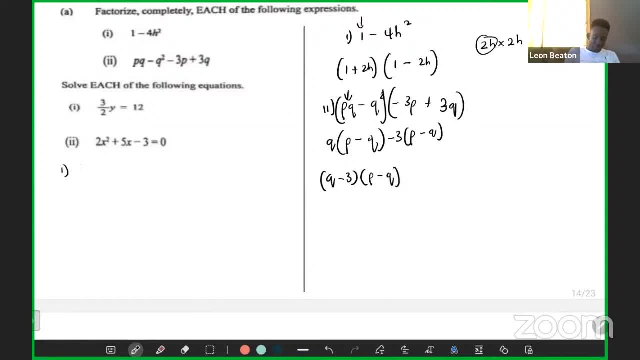 uh, and let's, let's solve the first one. so we have the first one, which is 3 over y, 3 over 2, sorry, 3 over 2 y is equal to 12.. so we want to solve this. so, um, uh, for me, for me i would have, i would have written this: 3 over 2 y. 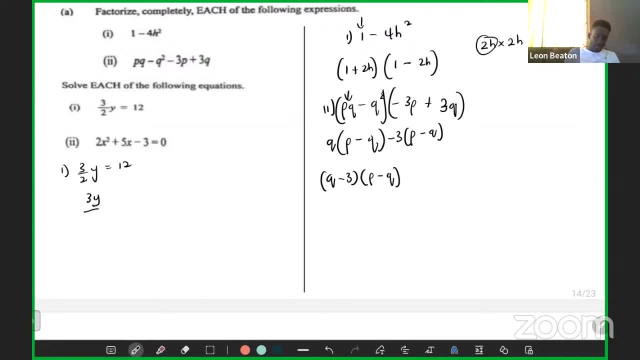 i would have written as: 3 multiplied by y, divided by 2, is equal to 12.. and then this: this is a much more easier it's. it's easier to solve from here. all right, richard, you could have. um, you could have simply multiplied this here by: 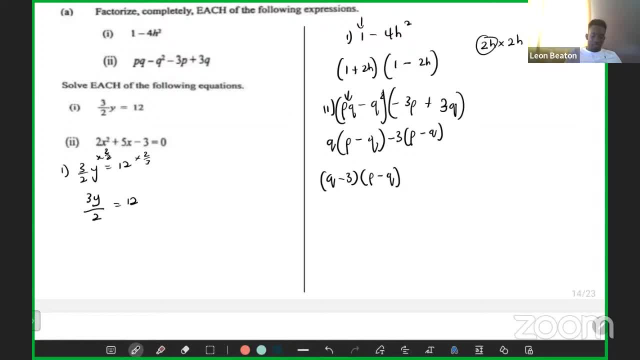 2 over 3 and you multiply this side by 2 over 3. but you know whichever way you want to work it, but i would have simplified it like that. then i noticed 2 is dividing, so i take it over to the to multiply, so we'll have: 3y is equal to 2 times 12 would be 24.. 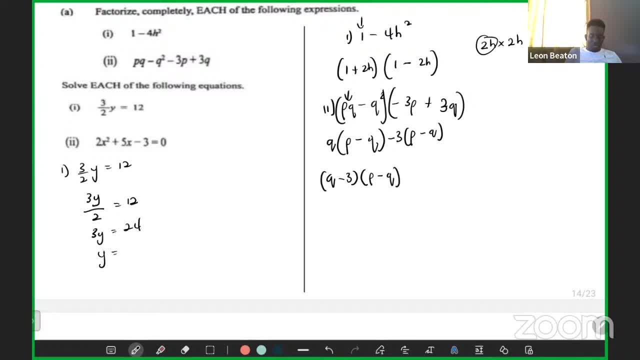 4 and then y would be equal to this. 3 is multiplying the y, so we take that off, it will divide it to be 24 divided by 2. sorry, 3 y will be equal to 24 divided by 3.. so ryan says y is equal to 8. right, that's emmanuel says in the chat as well. 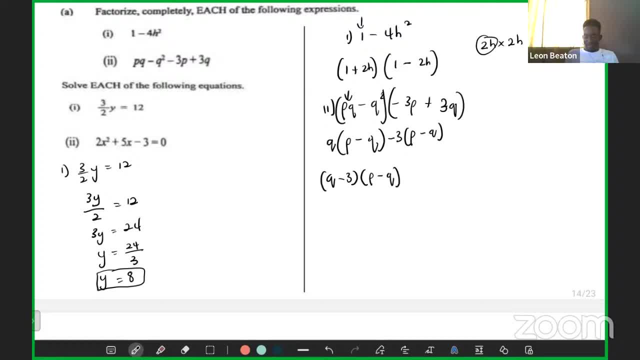 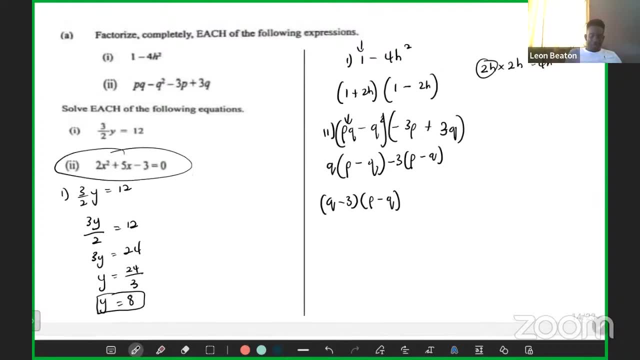 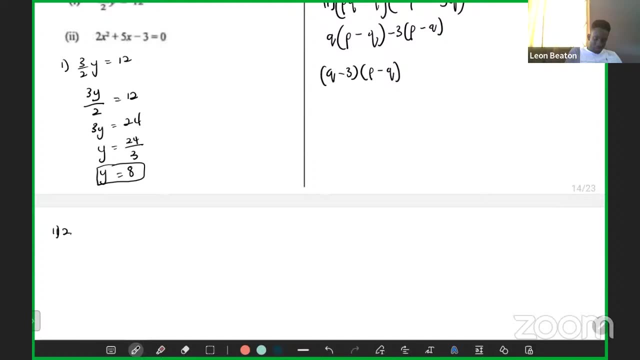 and case clark or cassie clark. okay, so, yeah, so that is this for that one, i think this went for how many marks? one, i guess, and this one probably goes went for two marks or two. so the next one we wanted to solve is: 2x squared plus 5x minus 3 is equal to 0.. what kind of equation is this? 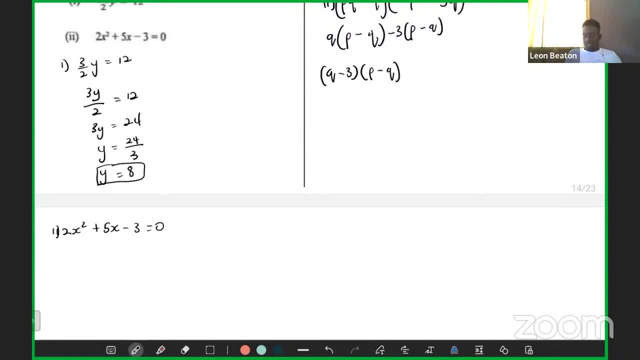 a quadratic equation, a quadratic equation. so how can we solve this? you can use the ac method, we use the ac method. or we can even go and use the quadratic formula. right for me, i know how many. yeah, i like the ac method, so we'll use the ace method. so let's use. well, we 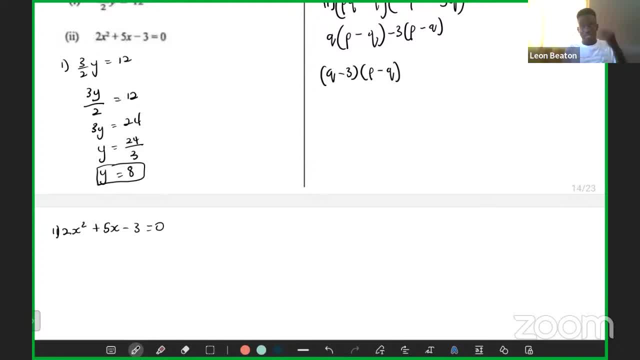 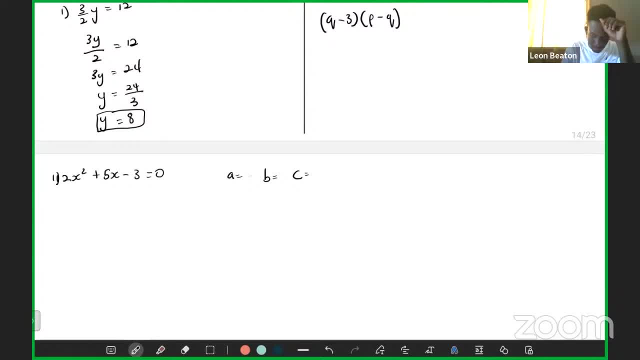 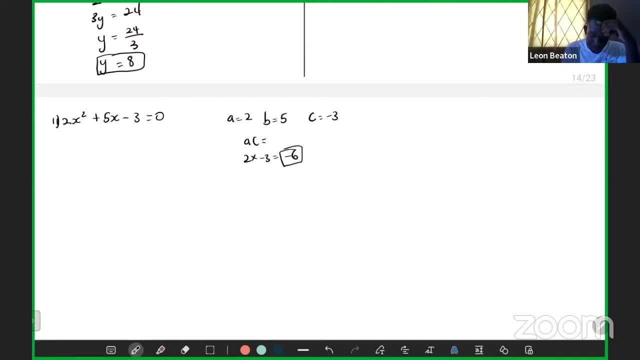 negative six. so ac method- since we're doing a revision ac method, somebody tell me: give me a little. uh, give me a little something on the ac method. what are we looking for? you're looking for two numbers. so when you multiply a and c, um, it must be equal. 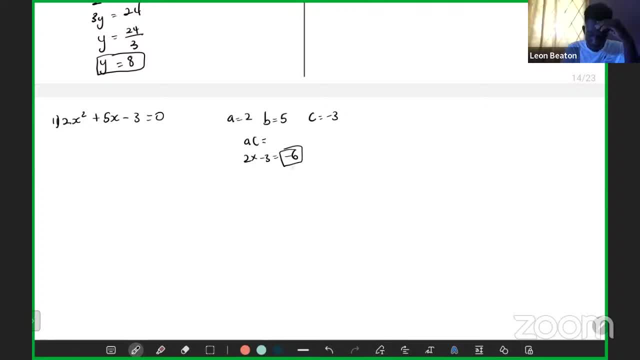 you multiply the two numbers. when you multiply a and c, um, and when you add um and when you add it, you must get b. excellent. so the two important things you want to look at is b and c. so we're looking for two factors, two numbers. when we multiply these two, 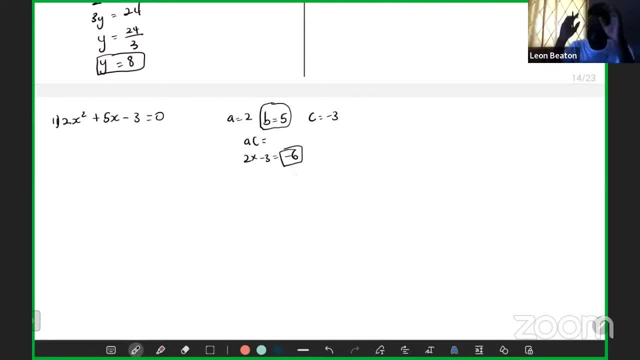 numbers. as i said, we must get negative six and we add these two numbers, we must get five. all right, we must get b. we must multiply them, we get uh, ac. what is the value of ac when we add them? we must get five, so this will be uh. 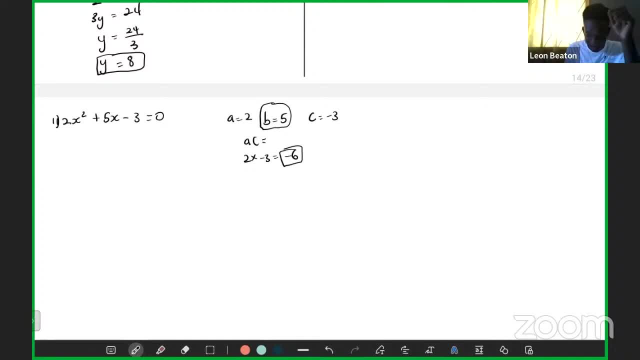 so this would be a times c. so what two numbers you have in mind? six and negative one. all right, let's, let's do, let's switch it wrong, let's do: negative one times six would it indeed give you negative six, and negative one plus six would indeed give you a positive five. so these two are two. 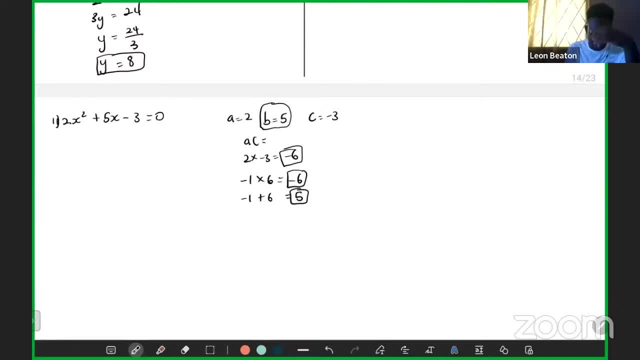 important things we're looking for. so we'll use negative one plus six. so we substituting negative one plus six for this middle term here. all right, so this will be two x squared minus. now we gotta attach to the the one and the six negative one and six. we gotta put x, right. 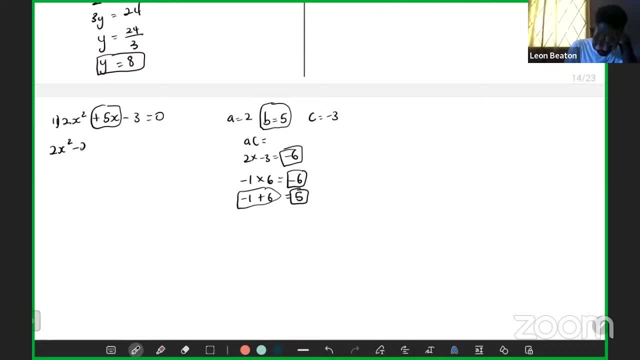 so two minus negative one x, which is the same as negative x plus six. x minus three equals zero. now the whole purpose of of doing that is to find two suitable numbers to replace 5x, and the two suitable numbers must be two numbers. when we put it inside the well, two. 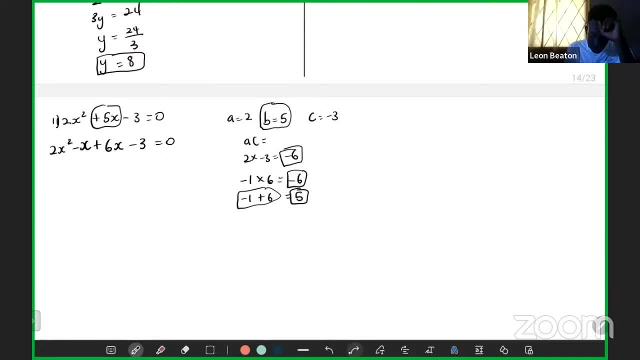 terms. sorry, when we put it inside of the equation it should not change the value of the equation. so we don't want to change it. we just want to expand it into four terms so that we can factorize it like how we we factorize these four terms at the top here. so that is what we're doing, right, that's. 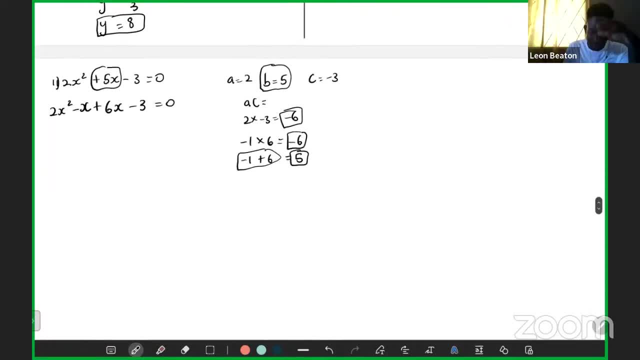 why we do the ac method and we love the a and and c and two suitable factors and so on. all right, other than that we could have put any number, but we want two numbers. when we put it inside the equation, it should not change the value of the equation, because if we change the value of the 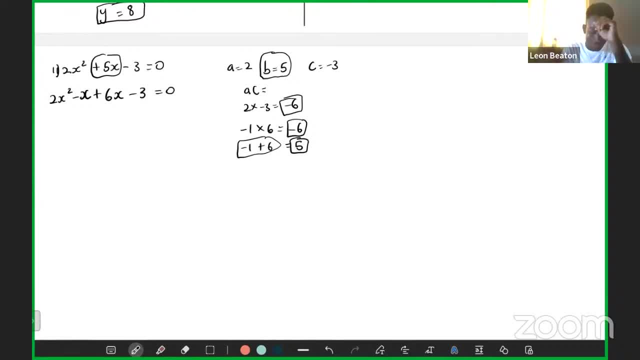 equation. that means you're solving a different equation. anyways, there's just some background as to the two numbers. so next we do like what we do what we did just now, we pair off and then we factorize, so we see 2x squared minus x. we see: 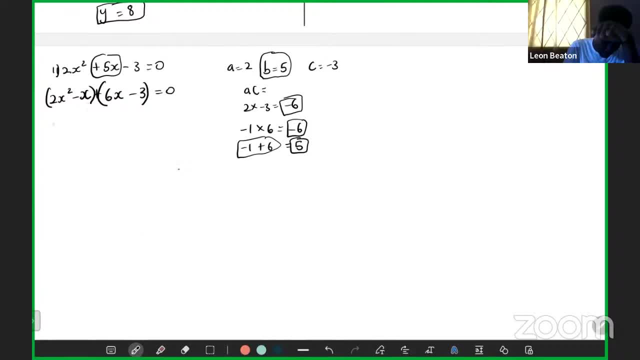 the common factor there. we see the common factor is x and we factor out the x from the 2x squared we left with 2x minus. we factor out the x from the x we just left with. x divided by x is 1 plus you see 6x and minus 3x. we see the common factor there between 6 and 3 would be 3. 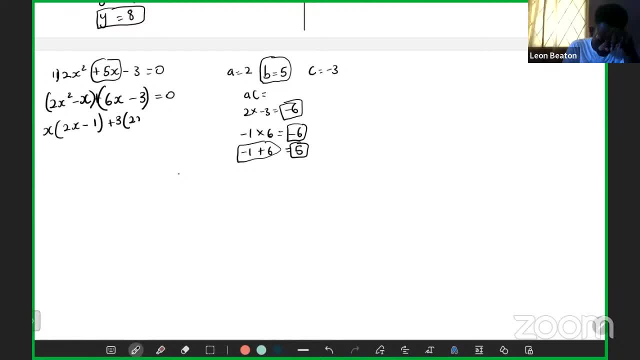 so we factor out the 3 and we're left with 2x minus 3 divided by 3 is 1 and that is equal to 0.. so we take what is outside the bracket we put in the bracket, so we have x plus 3 in a bracket and x minus 1 in a bracket equals 0.. 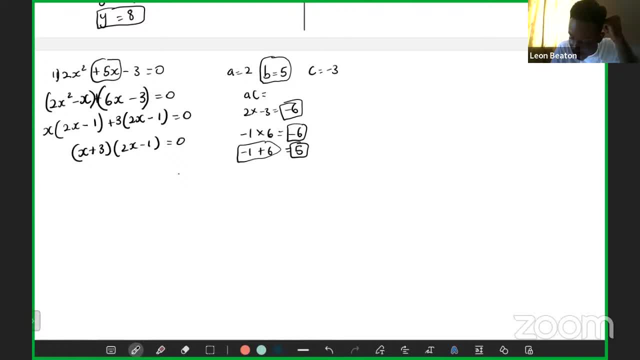 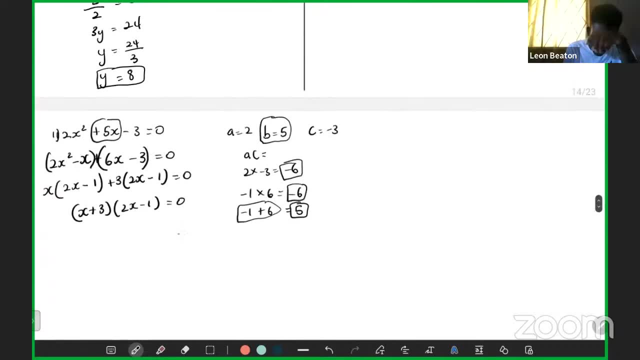 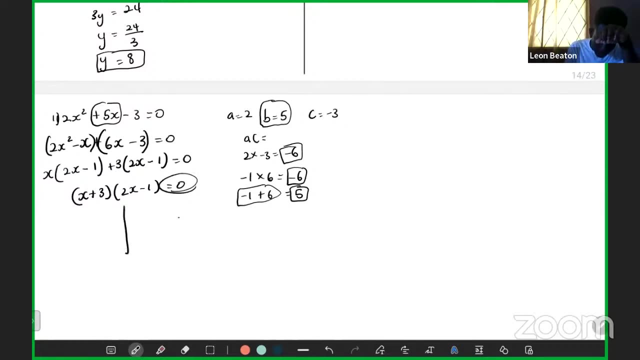 and then the question asks us to solve. so we solve. so they didn't access factors. they said to solve each other right, so we have to solve it. meaning we have to find what is the value of x and y quarter from here. so we equate over bracket to zero. it would be x plus three is equal to zero. 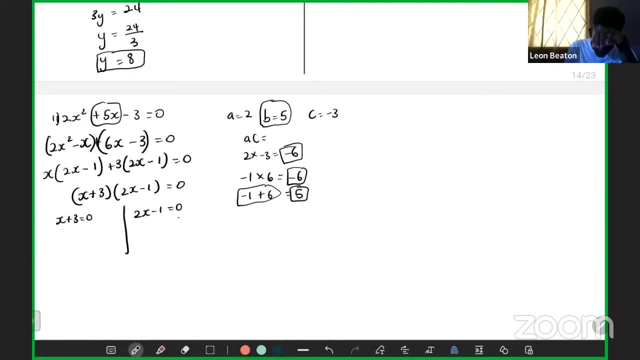 and two x minus one is equal to zero. so x plus three would be equal to. x is equal to negative three and two x minus one, that would be two. x is equal to this. one is subtracted and we take it over to add, so you'll have: one plus zero would be one and x would be equal to the. two is multiplying. 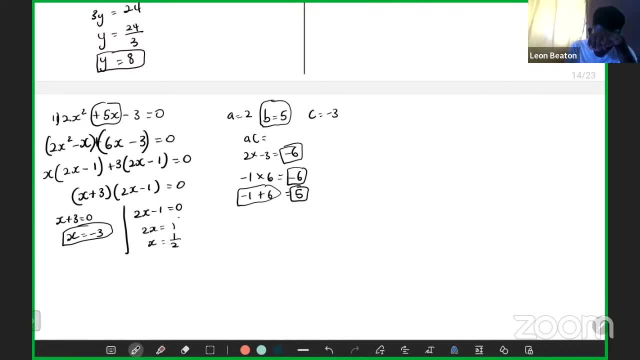 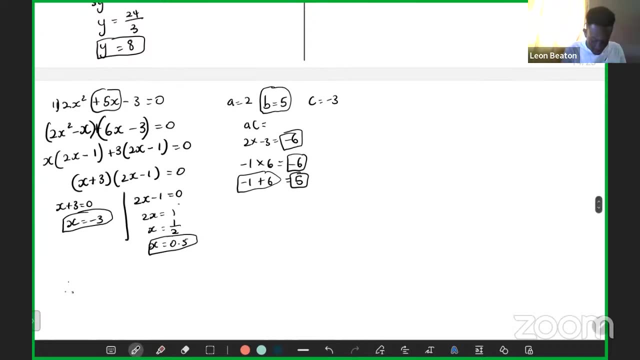 x and we take it over the divides, we'll have one divided by two, which is a half. so x is equal to 0.5, or you can leave it as a half, it doesn't. it doesn't doesn't matter, unless they said to express your answer as a decimal, it doesn't matter. so you can say: therefore: x is equal to negative three. 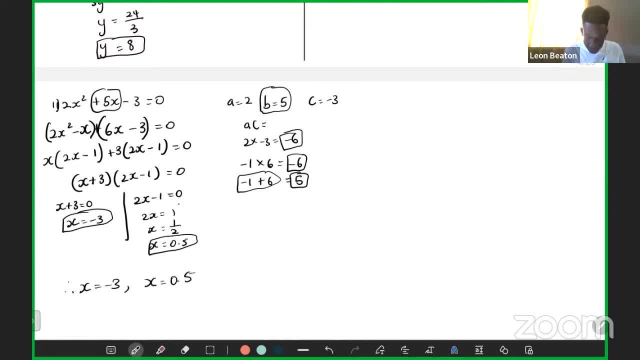 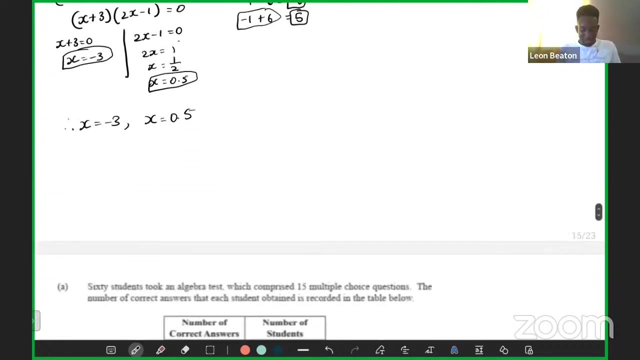 and x is equal to zero point five. all right, let me go there, let me head over to youtube and see what is happening if you have a few courses on youtube. yes, do you two got some fancy names anyways. yeah, so that is it for that. let's see what else we have here. 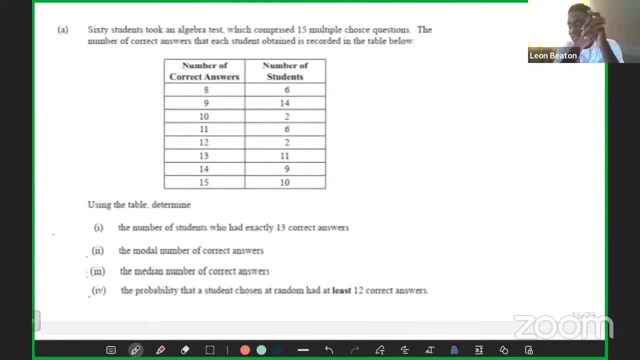 we have some statistics. so we completed uh algebra, we completed trigonometry, we completed um. what else did you want us to do? so let's go on to um functions. yeah, so we do some um satistics, every lap, every, every topic that we've crossed. you call it a lot. it will be done about four laps. 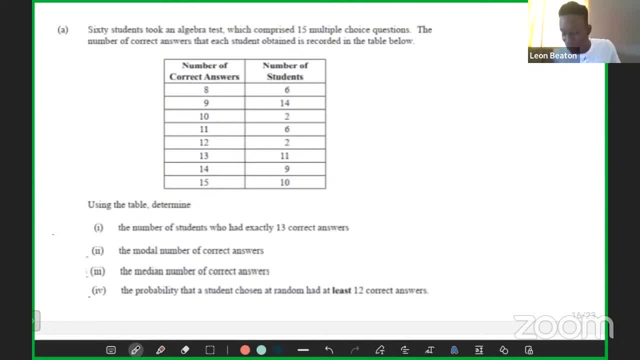 vectors as well. yes, vector to major C with manually. so let's check, so let's see here. okay, we've gotten a very booked long time考ηn. we've, they've, we. you know, we've gone between 18 and full Emil seven ¡» one. okay, now this is a mix between two of those and my elements. you know the problem with counting and yeah. 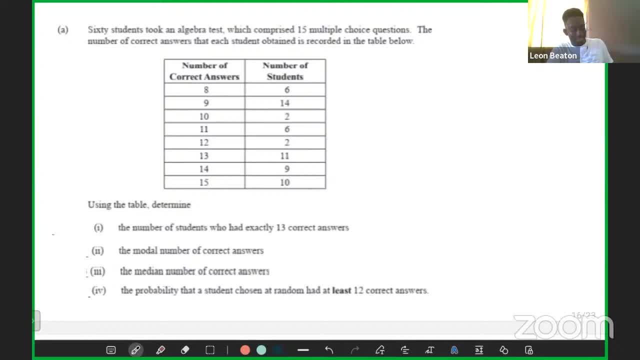 so statistics, statistics is probably um, it's, uh, it's a light part for most students as it's it looks fairly simple, but it can. the simple stuff is what would cause worry, so you don't want to take it for granted. so it says: let me get somebody to read it. i've been talking all the time. somebody 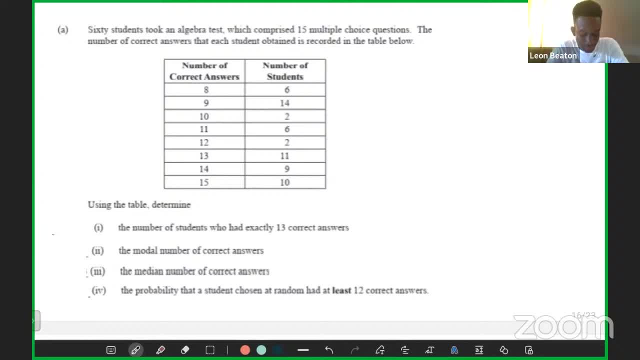 read the the instructions for us: anybody. 60 students took an algebra test test, which comprises 15 multiple choice questions. the number of correct answers that each student obtained is recorded in table view. using- oh sorry, using- the table determine the number of students who had exactly 13 correct answers. 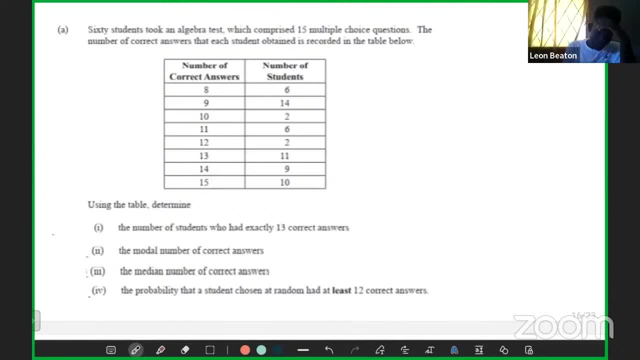 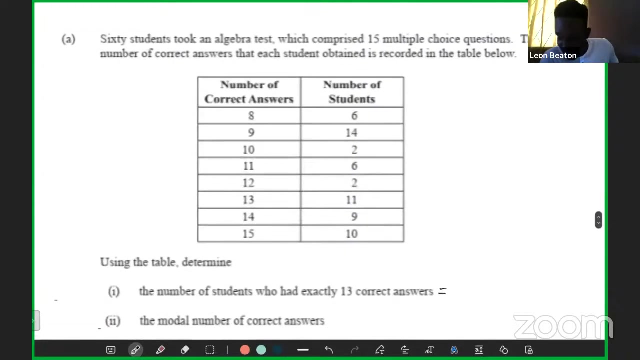 good, so how many students had exactly 14 correct answers exactly? let me ask in um. let me see again- so somebody who's been looking at us from starting- how many students have exactly. let me zoom up 14 correct answers. let me see who can come in here. all right. 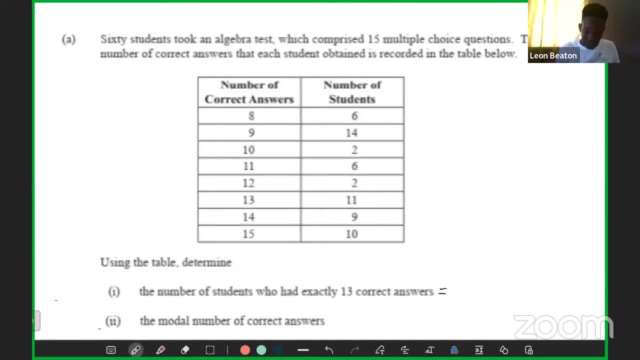 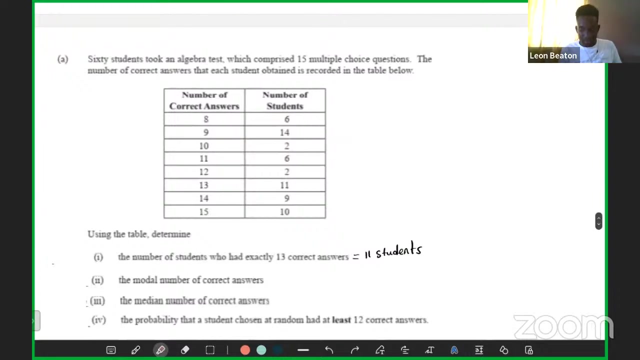 so nicola is saying 11.. yeah, so that's correct, right? 11 students. and you say 11 students, erica. simply correct answers 13.. now for a cancer starting, i will see 11 students. all right, 11, yeah, next one, the model of the correct answers. so what is mode or modal? 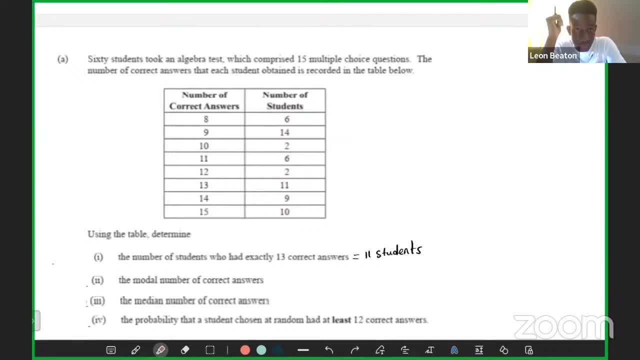 what is mode? again, the one that occurs the most, the one that of course the most the mode right, the one that of course the most highest frequency. so let me see- you can send me the chat again- the people on facebook. there's the mode. in the meantime, let me hear from somebody what is. 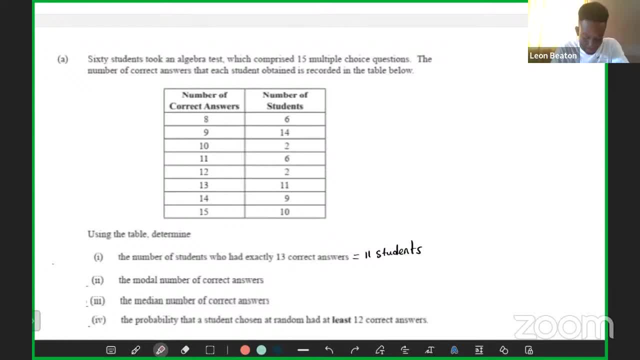 the mode by them. so somebody's saying nine, manuel is saying nine, katrina is saying nine. so let's see, nine has 14 number of core cancers. all right, is there nine? anybody disagree with that? in here are we saying this night: oh yeah, sorry, my bad, my bad. 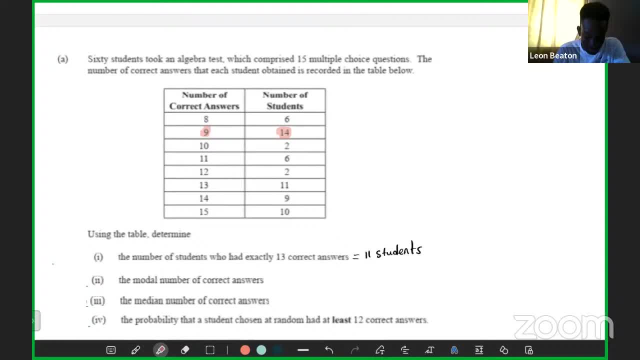 so, yes, nine, so nine students. 14 students got nine, got nine correct answers. so yeah, so we can see nine, it's got 14 students. had you know the most students had nine correct answers. all right, excellent. next one is the median number of correct answers. the median number of correct answers. 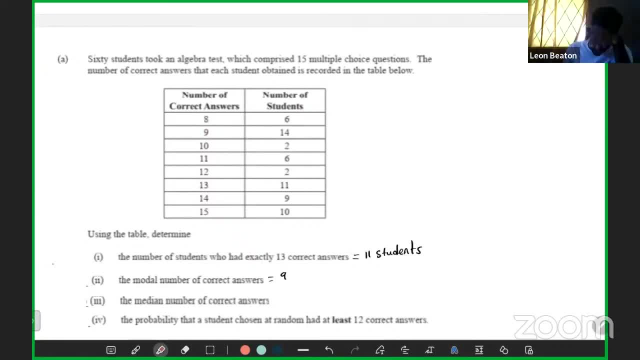 so for our two motor, number of correct answers, we see 14 students got nine correct answers, so 14 would be the most right anyways. so next one, the median number of correct answers. so this one, you got to do some thinking. median number of correct answers- what is median? again? 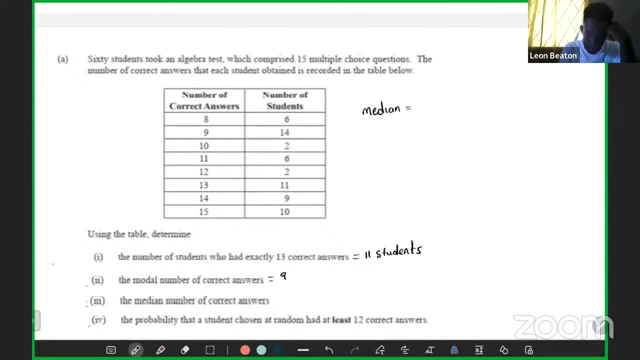 median number of correct answers. what is median again, outside, because inside is too hot. what is median again? anybody middle, manual, say middle, yeah, yeah, the median is the middle number, right? so let's say we had, um, let's say we had two, six, and then median here would simply be six. right, the media would simply be six. so we'll find the. 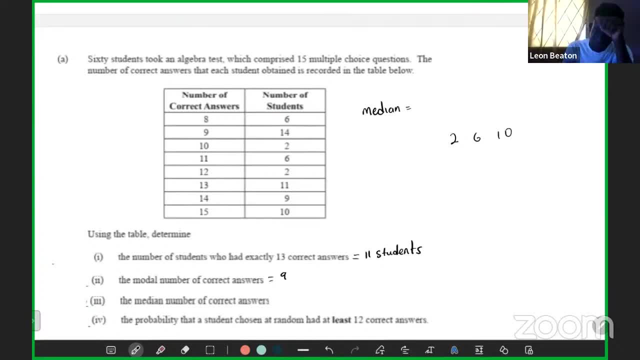 middle numbers, middle number. so the formula we can use to find million when we have large numbers, for example we have three, we have three um, three elements here, or three members or three numbers. so if we, you know we have large numbers, we can use the formula n plus one divided by two. 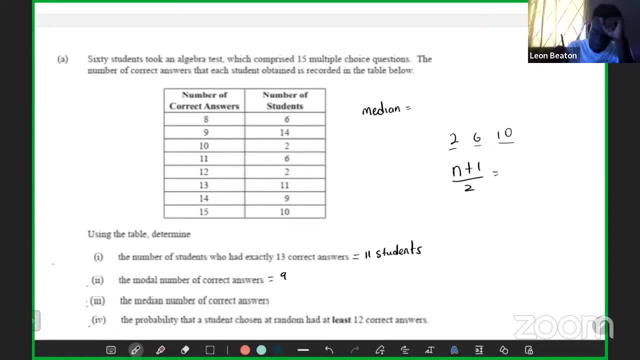 n would be the number of um elements that you have, or the number of people involved in the question, or whatever. so this will be n plus one, which would be three plus one divided by two. three plus one divided by two will be four divided by two, which is two. so the second element would be the median, in this case. 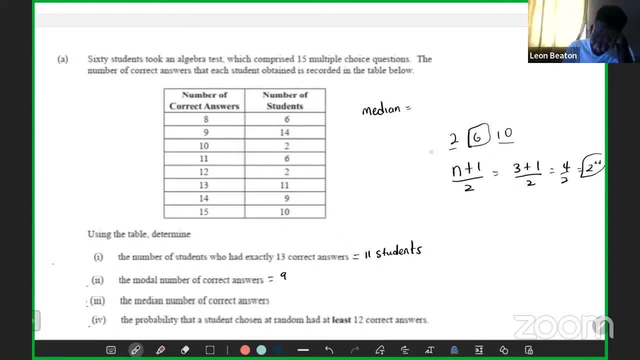 that is how we find. six is the median. all right, so this this will help us when we have very large um, a very large population or a sample anyway. so we got to find the total of students, so we got to add up all of this here to find the amount of students in this sample. 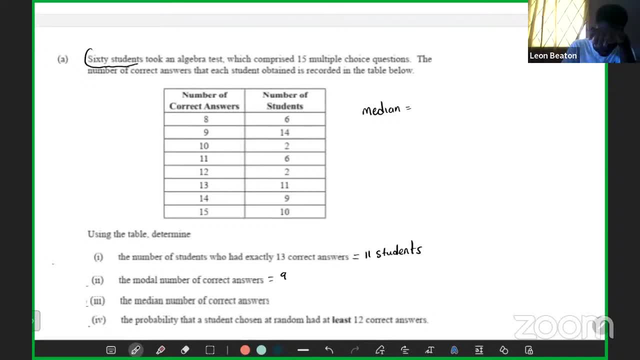 actually. no, we don't have to. we don't have to, we know it's six students, so it'll simply be 60 plus one divided by two. so 60 plus one be 61 divided by two, it should be. 61 divided by two would be um. 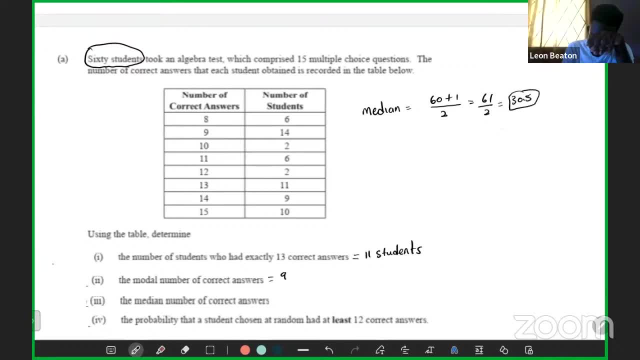 30.5, right, so this will be between 31 and should be between 30 and 31, the median between here. so we got to find the 34th- sorry, 30th- and the 34th student, the 30th and the 34th student and then, you know, find the middle of that. so let's see the 30th. so 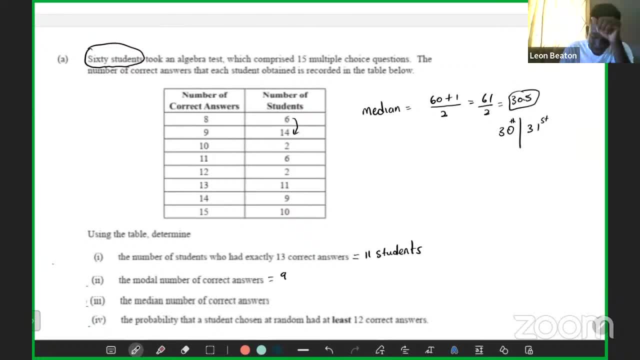 let's see where the 30th will fall. so we know 6 plus 14 would be 20, plus 6 plus 1 would be 20, 20 plus this would be 22, 22 plus 6 would be 28, 20, 8 plus 2 would be 40. 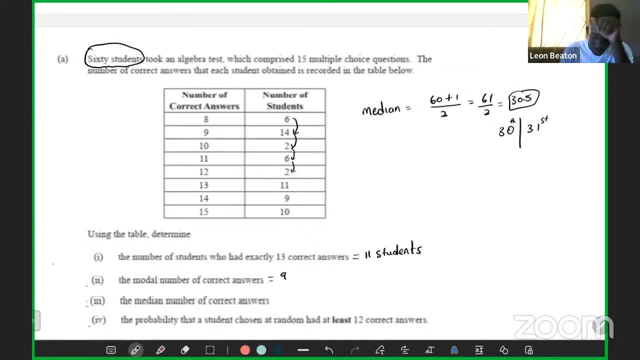 so here will be 30.. and so it. it will be between here, right, it'll, between 12 and 13.. because that's the position where it falls, so 20. so the median would be 12 plus 13 divided by 2,, right. 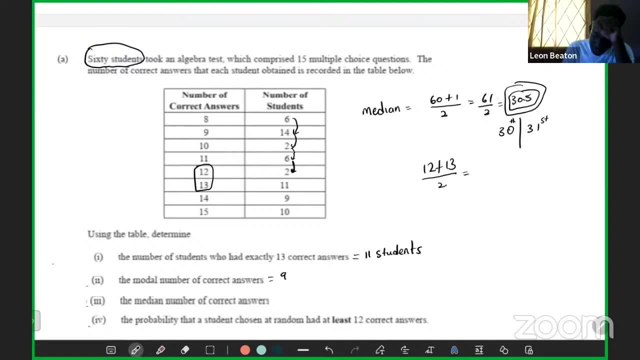 This thing that we found here is the position in which the median is Not the exact median. it's the position, right, It's the position that you can find in the median N plus 1 divided by 2, that is the position. 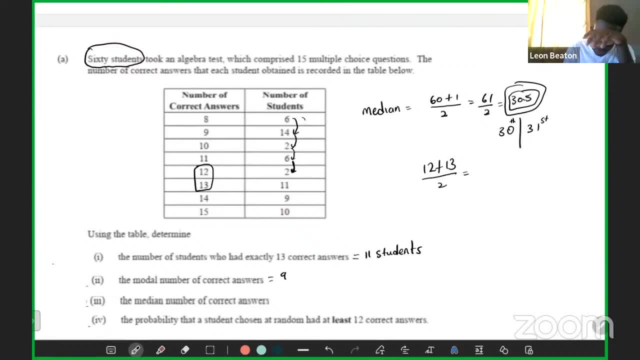 So when you count the numbers you know that would give you the position. So we see it falls right in between. Let me do it over again: 6 plus 14 will give you 20.. 20th student: 20 plus 2 would be 22.. 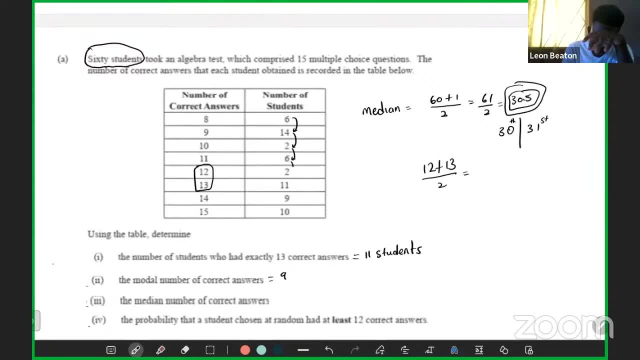 22 plus 6 would be 28.. 28 plus 2 would be 30. So this is the 30th here, And then the 34th would be right here. So it will be between 12 and 15, right. 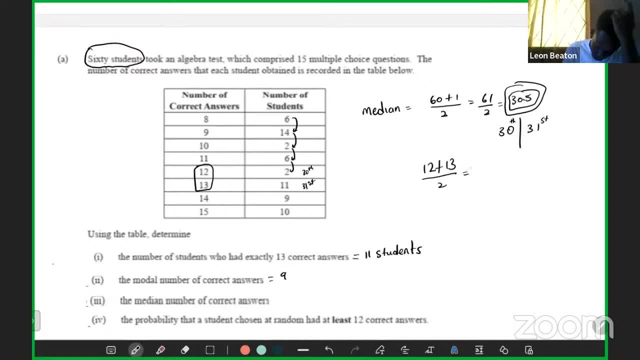 If you write all these numbers, you can get that. So 12 plus 13 would be 15 divided by 2, which would simply be 7.5.. 7.5.. Everybody go there. Yes, sir, Sir, it's not 25.. 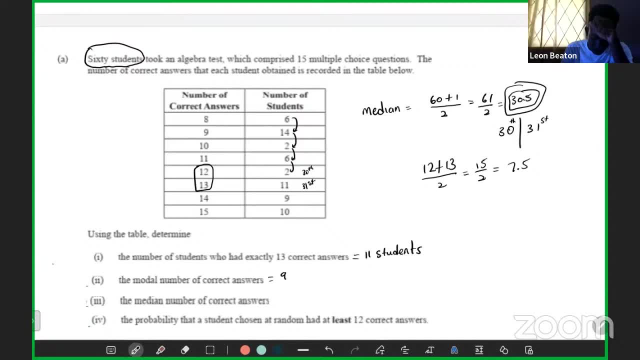 25.. Where you got 25?? 12 plus the 13.. Good, Remember, you got divided by 2, right. So you got to find the. it falls in between the two, Remember, it's like if you got, if you have it, it's like if you have the number 2,, 3,, 4, and 6, right. 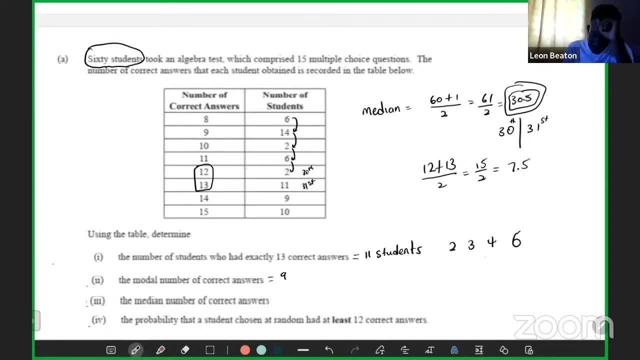 And you want to find the median here. right, The median would be these two numbers, right, It would be between these two numbers. So what do we do Out of 3 plus 4 divided by 2.. 3 plus 4 is 7.. 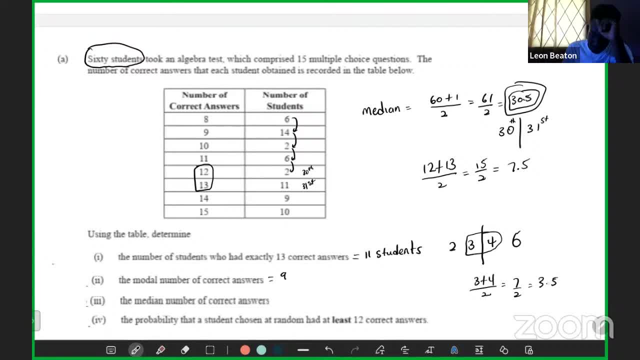 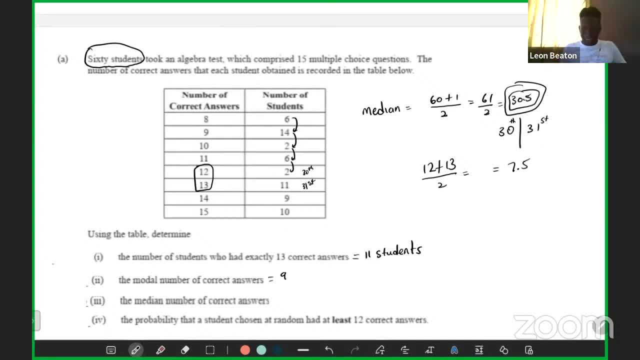 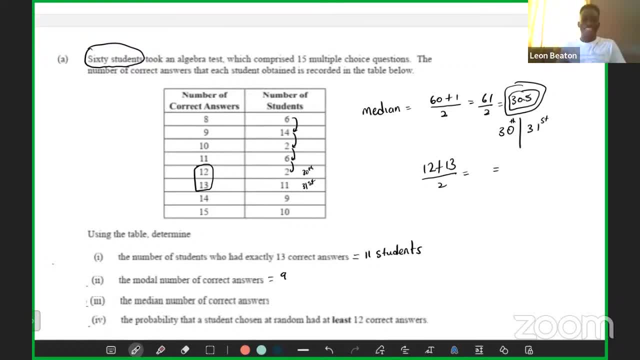 It's stumbling. Yes, yes, yes, That's correct. Yes, yes, Yes, yes. 325.. 325 divided by 2 is 12.5.. The coach is stumbling right. The coach is stumbling The other five. 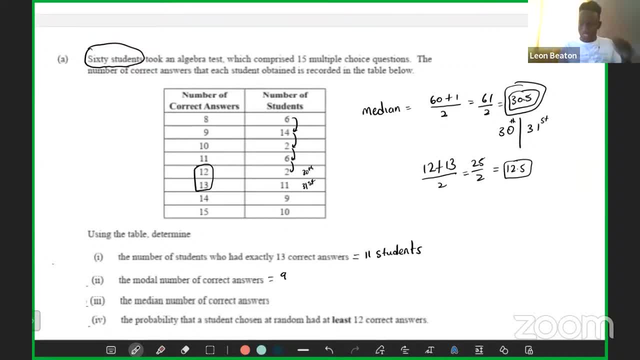 We've got to come and help the coach. Yeah, yeah, So that's correct. Thank you, Tosito and Elizar. Yeah, so the median would be 12.5.. Yes, Yes, So don't do like that. 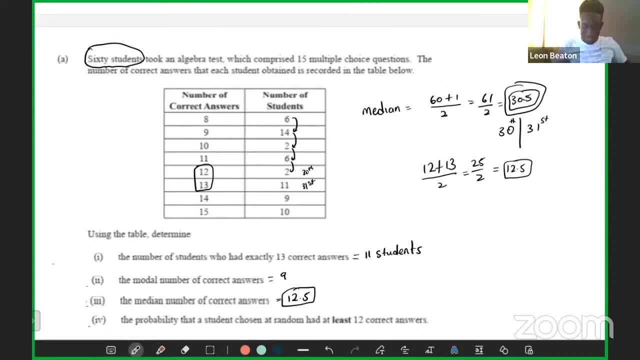 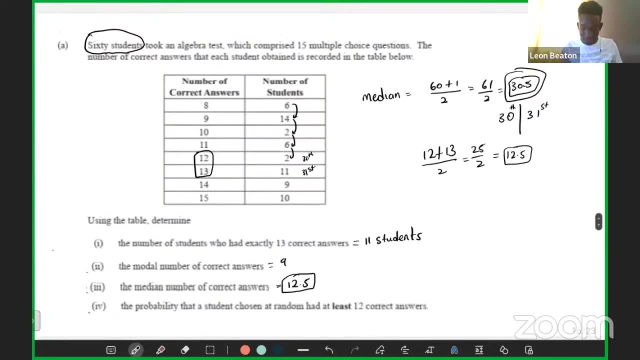 Don't do that in your exam. You know double check. So last one: the probability that a student chosen at random had at least 12 correct answers. At least 12 correct answers. So let me erase. So at least 12 correct answers meaning at least we can have 12 and more. 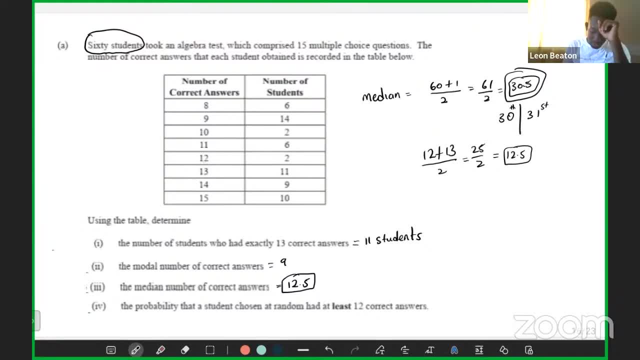 All right. So we got to take all the students from here, At least 12.. So at least 12 would be 2 plus 11 plus 9 plus 10.. And 2 plus 11 plus 9 plus 10 will give us: 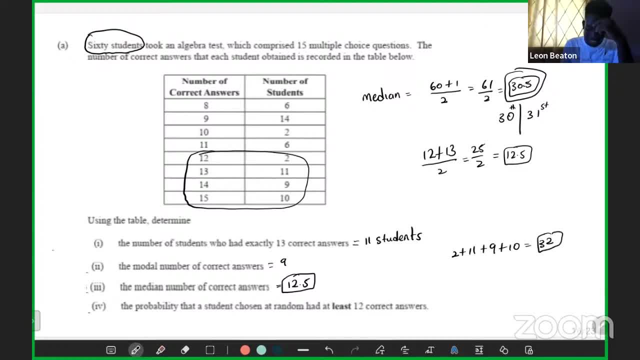 32. 32.. So 32 students had at least 12 correct answers. So the one probability that if I choose a student at random, you know it will be either one of these 32 students. So to find a probability that if you choose a student at a random, it will be the total number of favorable outcomes, which would be 32.. 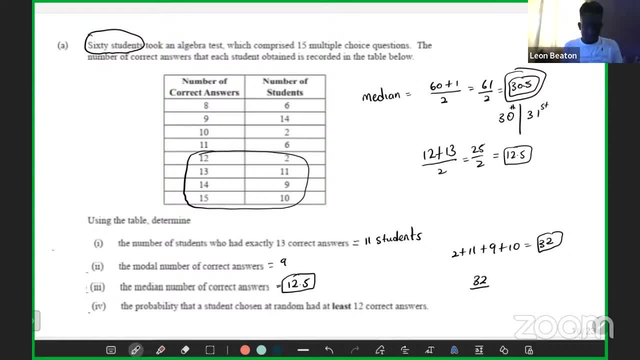 You know, 32 divided by the total number of possible outcomes, And that would be the students that we have in the class. The total number of students that we have in the class, which would be how much, How many? 60.. 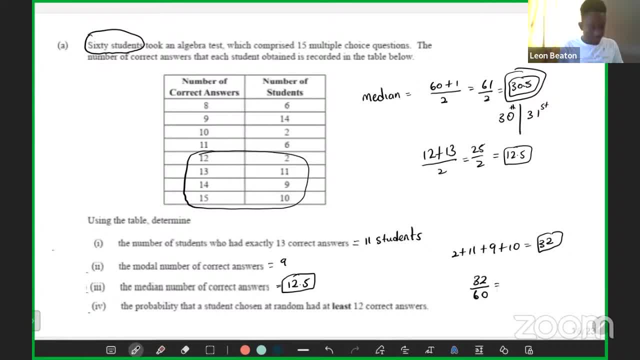 So 60.. So 32 divided by 60 would be- Let's break it down. So let's do this: Yeah, 0.533.. So let's break it down, Let's put in a fraction. So what number can go to 30 and 60?? 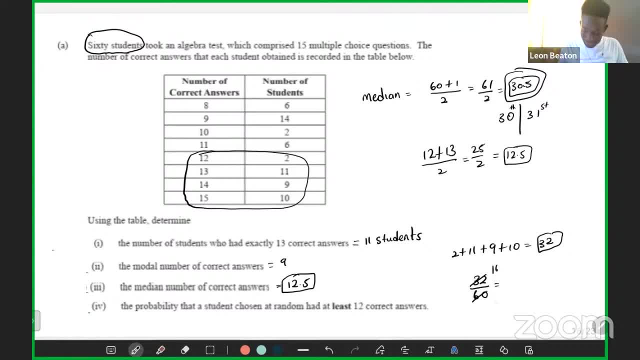 2. 2? All right. 16. And then we got 30. And we can break this down even further: 8. And we're going to have 15.. It's 8 out of 15, right. 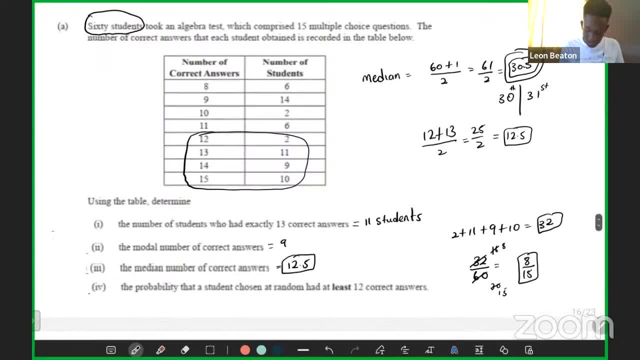 8 over 15.. 8. 8 out of 15.. All right, At least Wait, wait, Hold up, hold up, hold up. Is that correct? At least 12 correct answers, Yeah, at least. 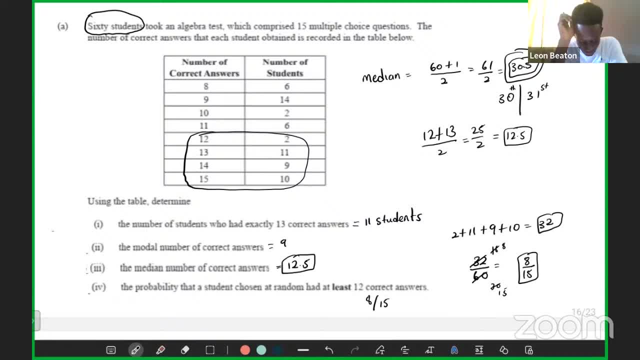 At least Meaning. So it's like much more than 12.. Yeah, If you want at least $100.. Yeah, it can be $100.. If somebody say you're having at least $1,000.. To buy something, $1,000 is going to be the least amount, right. 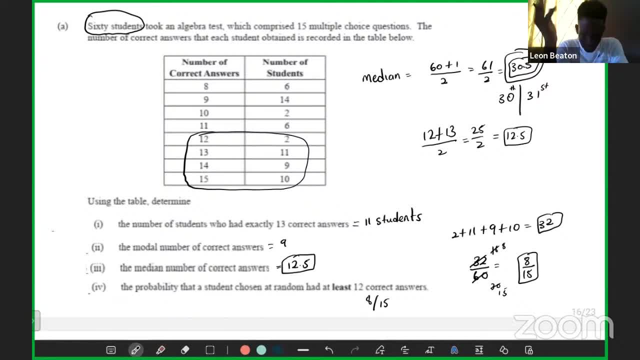 It's going to be $1,000 and more. Yeah, so there's one way you can think about it. Yeah, at least Everybody good there, Everybody good there. Yes sir, Yes sir, Let me see Yeah. 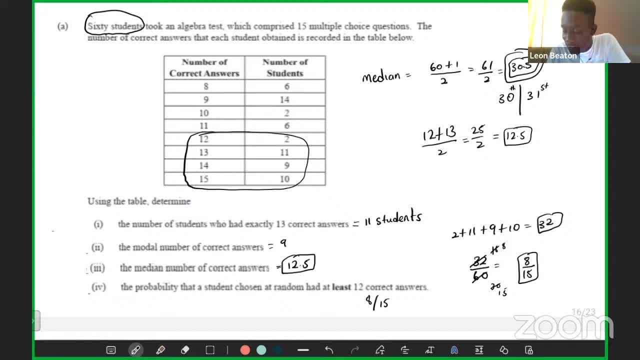 Yeah, there's one way you can think about these kind of questions right. If you kind of get confused with the difference between at least and at most, I think you don't put yourself in a situation You know somebody's selling a phone. 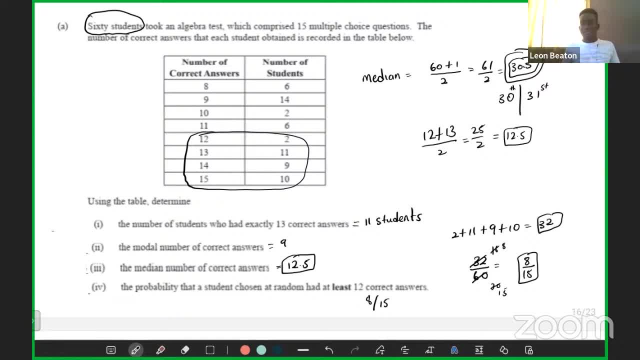 They say, hey, you got to bring at least $32,000.. Meaning you can't work with $15,000.. The least amount you could bring is $32,000.. So you could bring party, You could bring, you know. 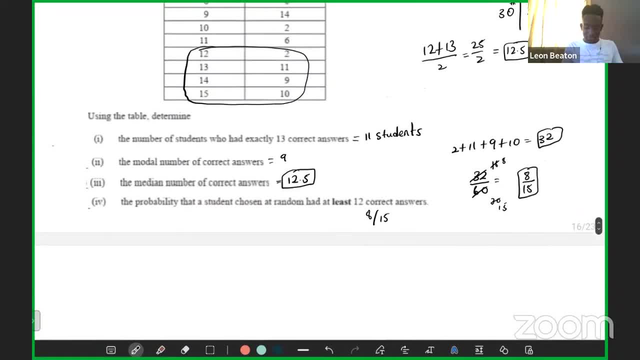 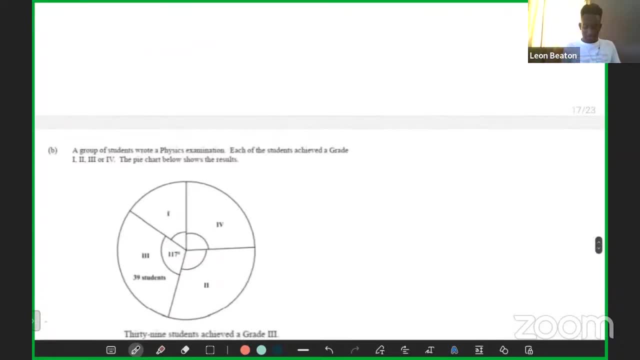 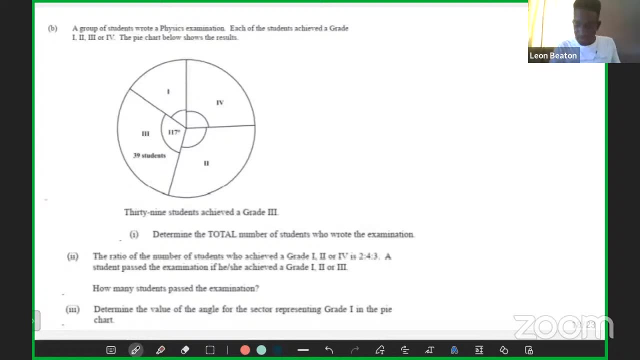 Yeah, So that's it for that kind of that question. Let me see It's going to be short. Nobody seen it, So we continue with our statistics. So let me get somebody else to read this one. I think I'm going to get another volunteer. 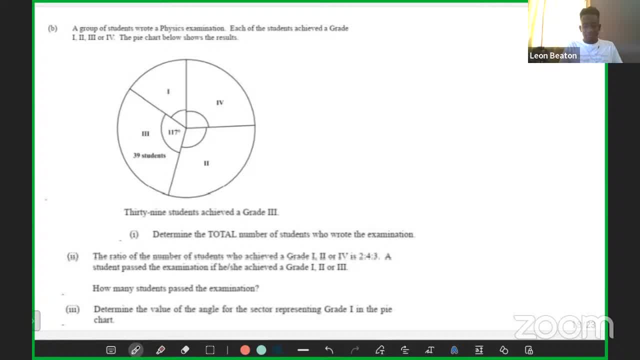 Wait, let me drink some water Anybody, So can I read it? Yeah, go ahead, Okay, Go ahead. A group of students wrote a physics examination. Each of the students achieved a grade I2IIIV. The pie chart below shows the results. 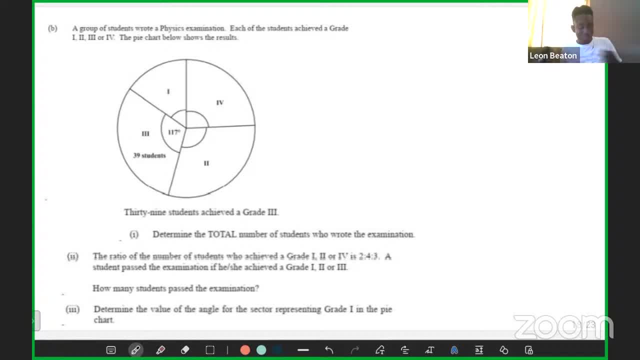 Okay, So grade one, grade two, grade three, grade four: Right, So the pie chart shows grade one, grade two, grade three, grade four. So let's see. So nine students achieved a grade I2IIIIIV. 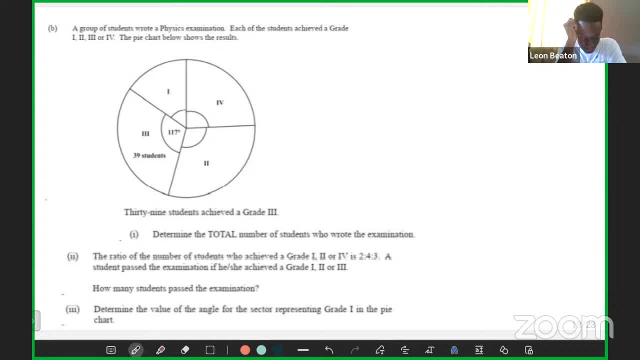 So determine the number students who rode the exam. So behaviors seaweed significant. Okay, So nine students achieved a grade I2IIIIIV And it wants to determine the total number of students who know the exam. How can we find that? 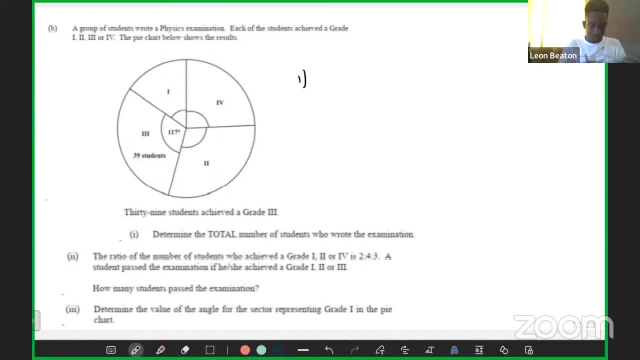 Good, Yes, okay, There you go. Okay, I'll smell. We will not be asking you to answer this one. I think you had to answer more questions. Yes, We took you. Okay, That's great. How can we find out if there are nine students wrote? sorry, there are nine students achieve a grade three and they gave us some information about these nine students. 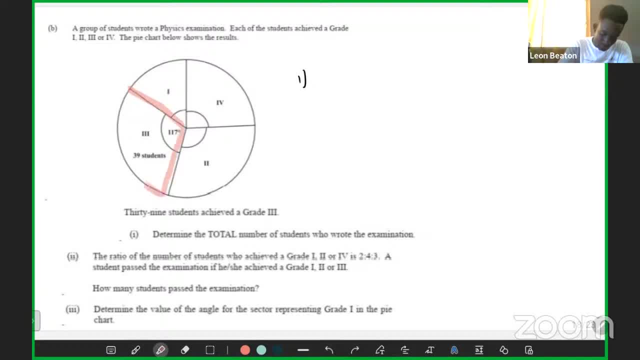 They gave us some information here. How can we find how many students wrote the exam? How many degrees did our nine students took up 117,, sir, So 117.. So how can we find the amount of students here now? 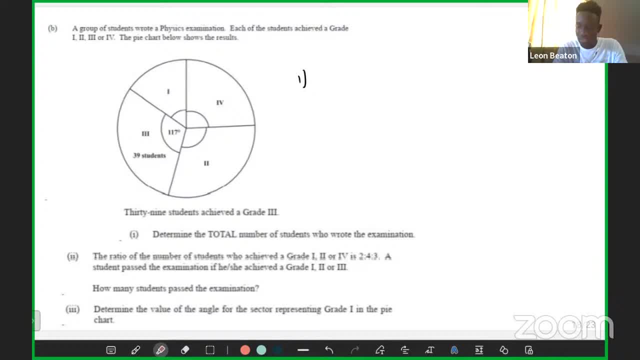 Out of the 117 degrees, let's throw the nine students. How can we find total number of students? We can say 39 multiplied by 360, which is the total number of degrees in the circle divided by 117. There's the amount of students that 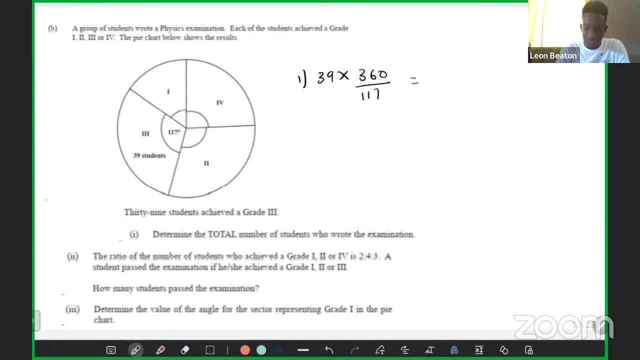 The total nine students will be the amount of degrees for the total nine students. This will be 39 times 360 divided by 117, and that will give you 120 students. sorry students, Remember: 360 is the total number of degrees in the circle and 117 is what you have already. 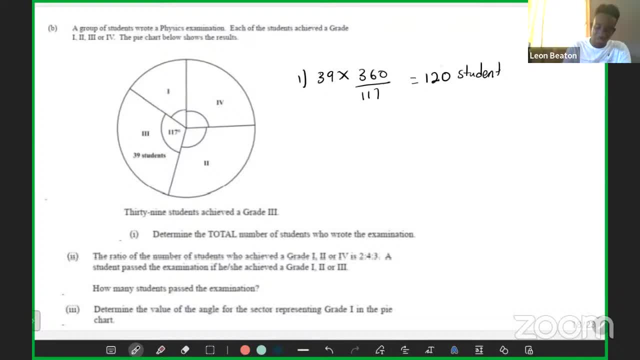 So you know, you put the 360 over that and multiply by 39, and that will give you total number of students. All right, There are other ways you can do it as well. Anyways, everybody go there, Everybody go there. 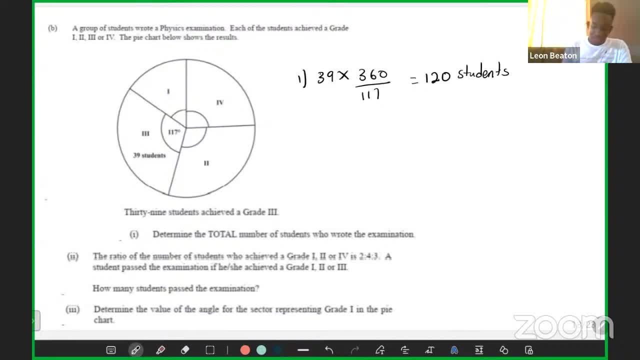 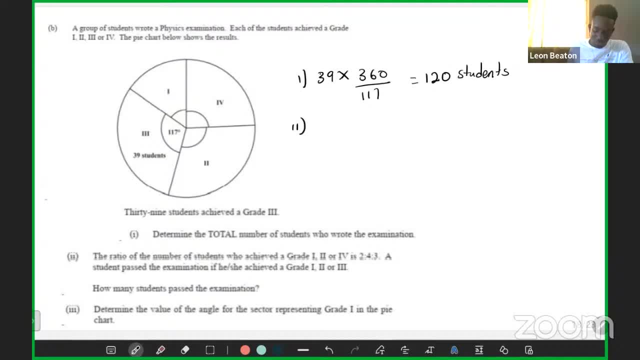 the ratio of the number of students who achieve a grade one, two or four. Very good Ratio of students who achieve a grade one, two or four is two to four to three. A student pass the exam if he or she achieved. 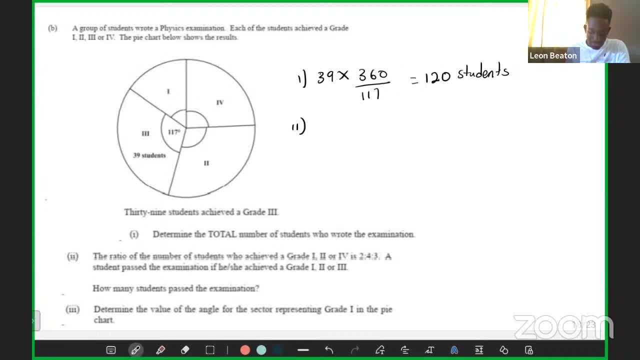 a grade one, two or three, How many students pass the exam? So they gave us a ratio of grade one, two to five, and that ratio is two to four to three, right? So they want us to find how many students pass the exam. 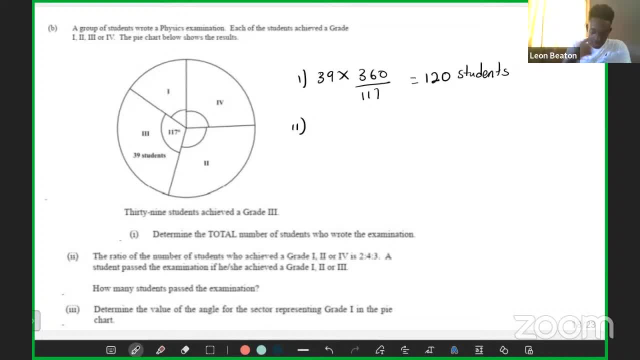 So they didn't give us grade three. So that means this ratio here. it doesn't cater for grade three. So what we gotta do, we gotta take out the number of students who achieve the grade three. So we know we have 120 students in total. 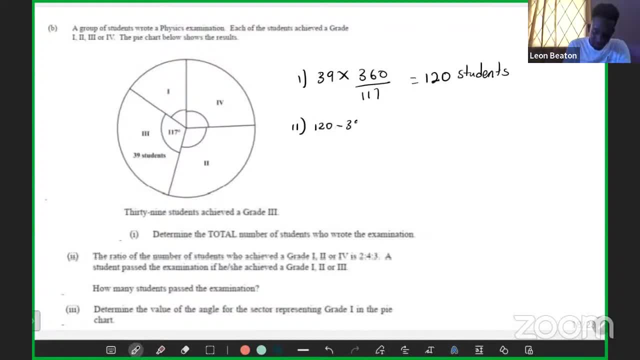 So we have the 1,000 students, the students who achieve the grade three, minus the number of students who go out of the grade two, which is 29.. That will equal to 120 minus 39.. That would be 81.. 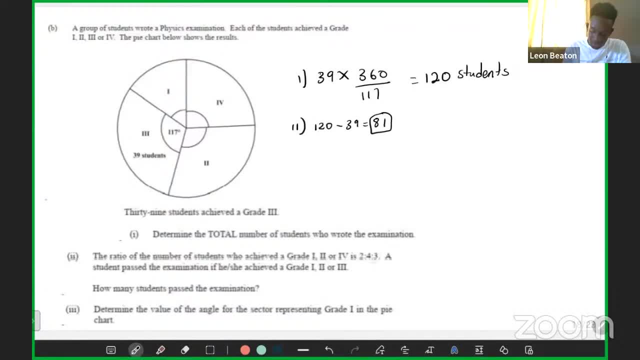 So this ratio caters for 81 students because it's grade one, two and four. So they told us this ratio is two to four to three. So let's find what each one of these ratios worked. each part is worked right. 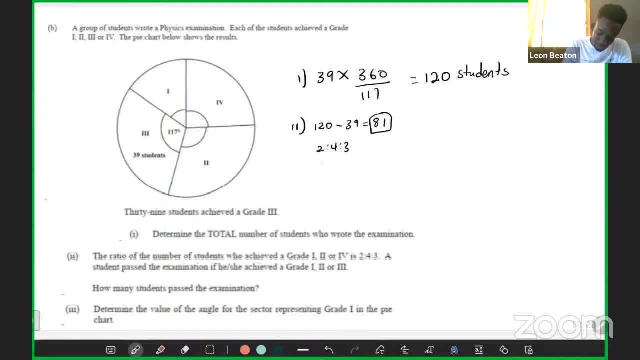 So two to four to three, one to zero to 3. now to be 2 plus 4 plus 3, and 2 plus 4 be 6. 6 plus 3 would be 9. so it's 9 is a total share. so to find a value of one of these shares, it would be 81. 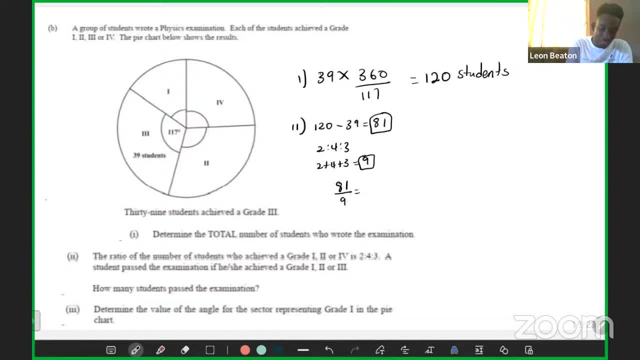 divided by 9 to 81, divided by 9 would be 9. that's the value of one share. one share is equal to 9. so to find the amount of students who pass the exam, we gotta find the amount of students who gain a grade 1 and a. 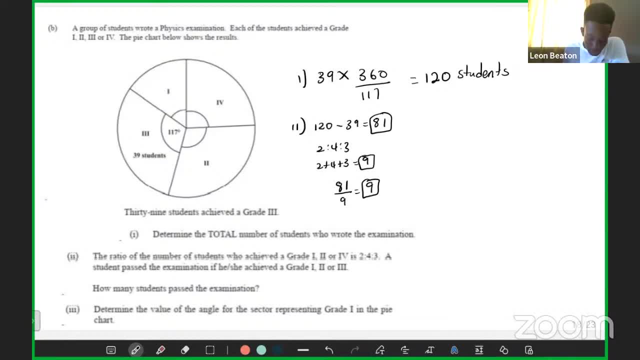 grade 2 and a grade 3. so let's see the amount of students who gain a grade 1. so the share for the grade 1 is 2. so so grade 1 it would be 2 multiplied by the value for one share, which is 9, which is equal to 18. amount of students who gain a. 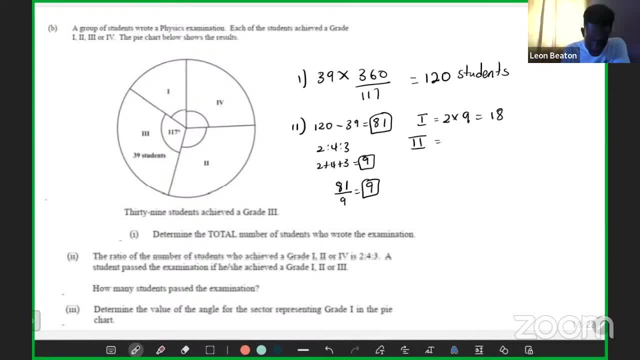 grade 2 would be 9. how many is the share for grade 2 and 4? so it would be 4 multiplied by 9, which would be 4- 9, star to 6. and then we already know the amount of students who gain a grade 3, because it told us it's star to 9. the amount of students who gain a grade 3 is star to 9. 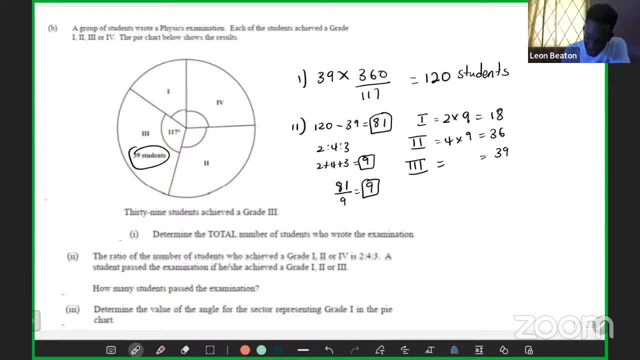 so to find the amount of students who pass the exam, we add up all of this and 18 plus star to 6, plus star to 9. how many students was the exam? 93, 93 students pause the exam, so we can say, therefore, 93 students. 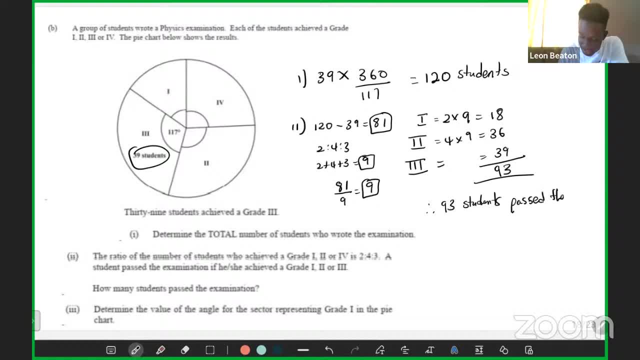 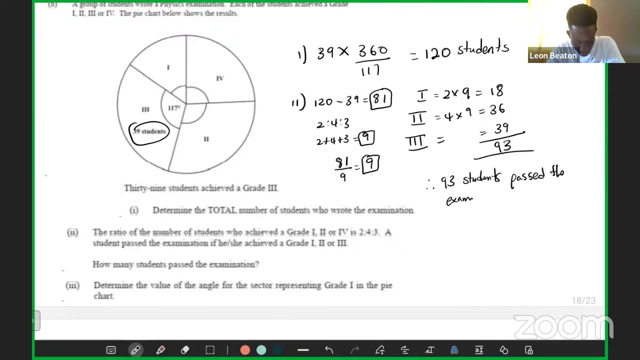 pass the exam because you can pause the exam at a grade 1, 1, 2 or 3, so we need a grade for it. pause the exam, you all right, everybody go there. yes. so, last but not least, determine the value of the angle for the sector representing grade one. 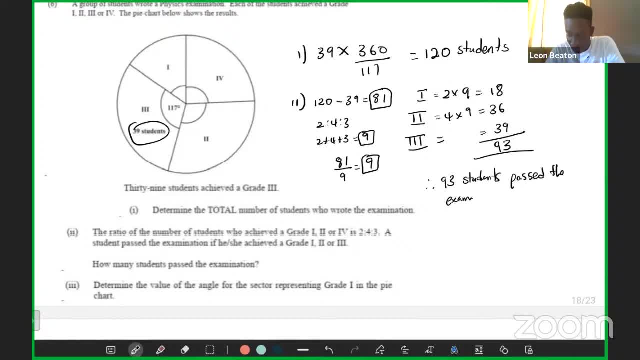 in the pi chart. so you want to find an angle now. so, um, so we know, we know the amount of students who gain a grade one is 18, so it would be 18, so let me write this number three. we know 18 students gain a grade one. 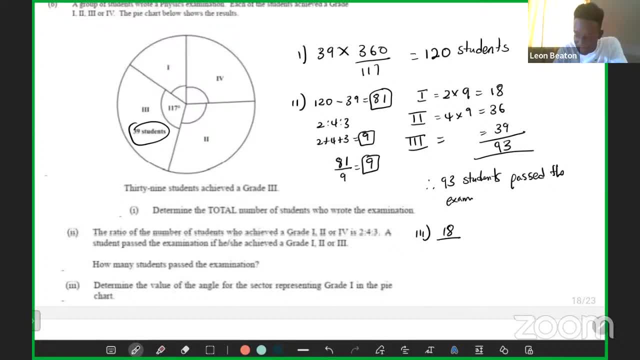 so it'll be 18 divided by what? are we dividing the 18 by 18? divided by how many? this is total number of students. we have 120, 18, 18, 18 divided by 120, and we're multiplying this by to find the amount of degrees. 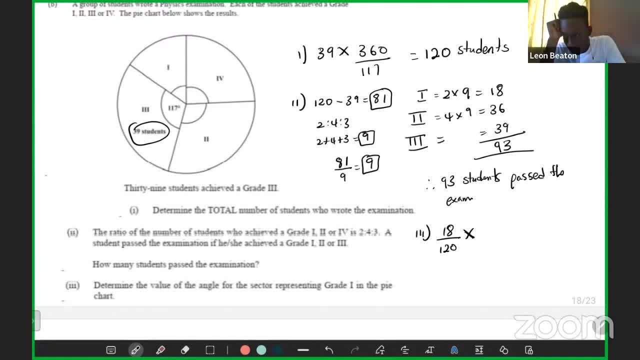 divided by 120, and we're multiplying this by to find the amount of degrees divided by 120, and we're multiplying this by to find the amount of degrees, that is, 18 will take up. so 360, yeah, 360, right, 360.. so 360, yeah, 360, right 360.. 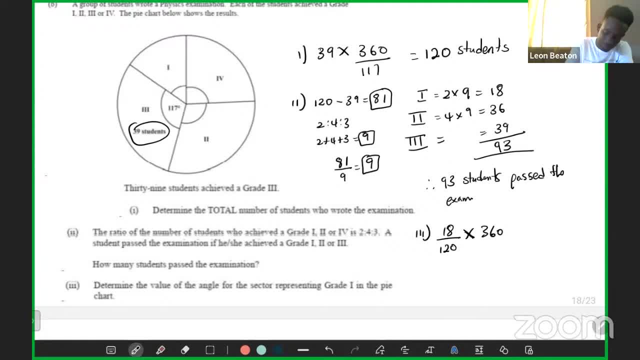 so 360, yeah, 360, right, 360.. it's 18 times 360. it's 18 times 360. it's 18 times 360 is equal to six thousand eighty, is equal to six thousand eighty, is equal to six thousand eighty. six thousand four hundred eighty divided by. 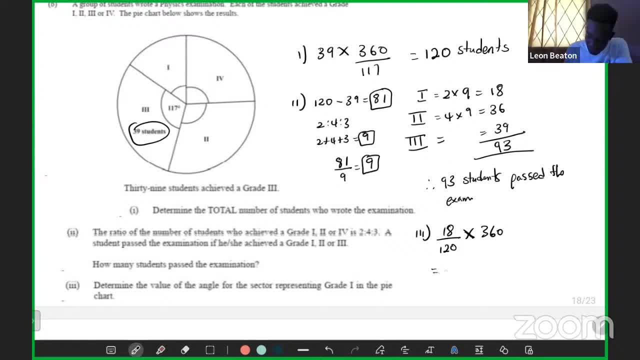 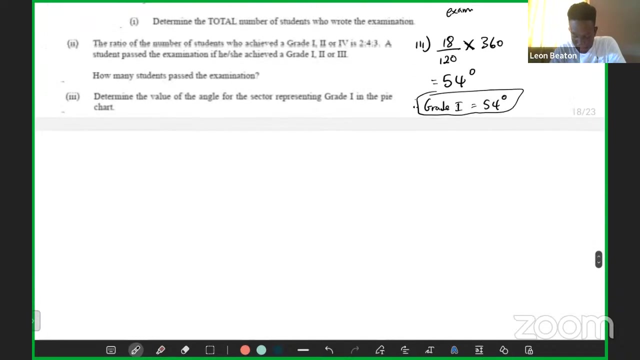 six thousand four hundred eighty divided by six thousand four hundred eighty divided by one, twenty one, twenty, that would give me 54 degrees. it's therefore grade one is equal to 54 degrees. right, and that is it for that one. okay, ready, go there. yes sir, yes sir. 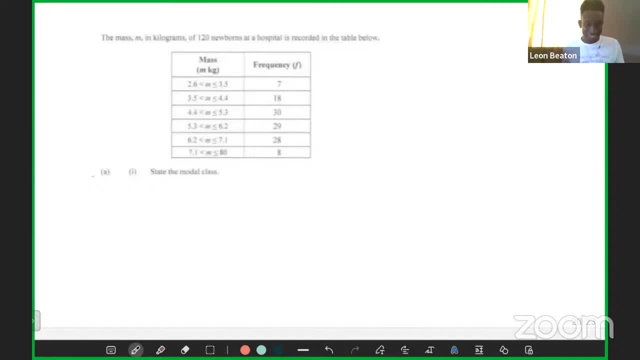 let's go. yes, my friend from region one, my friend from port kaituma, where are you? it's the pier. yes, sir, all right, you're buckling, you're buckling, or you're? you're running strong, we're strong, you're inside, all right, all right, all right, let's go. let's go. 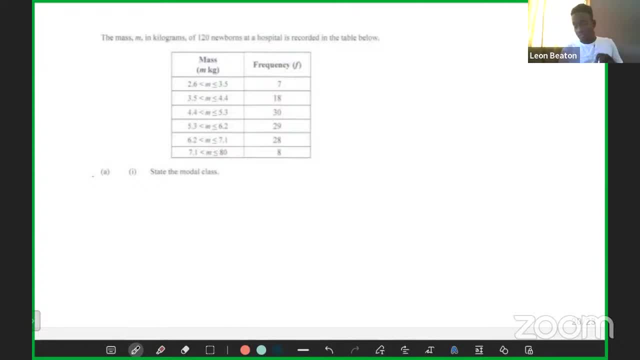 arleno, read this for us, read the instruction for us, or two. the mass m, sir, but then you must m and in kilograms. the mass m m in kilograms of 120 newborns at the hospital is recorded in the table below, and the frequency and so on. the frequency tells you the amount of. 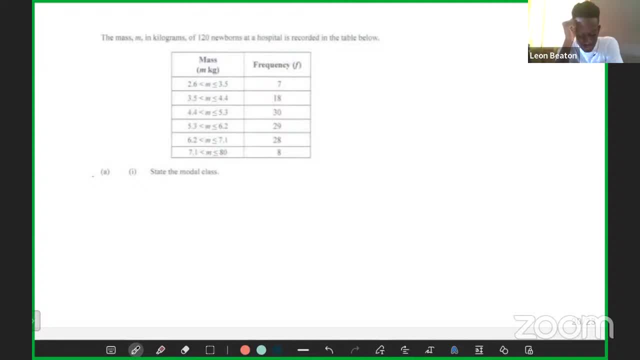 the amount of um babies that fall into the, the range, the, the group data. so we got 2.6 to from 2.6, 3.5 and so on. so stay the modal class. so to be the modal class here. what will be the motor class? which one got the highest frequency? 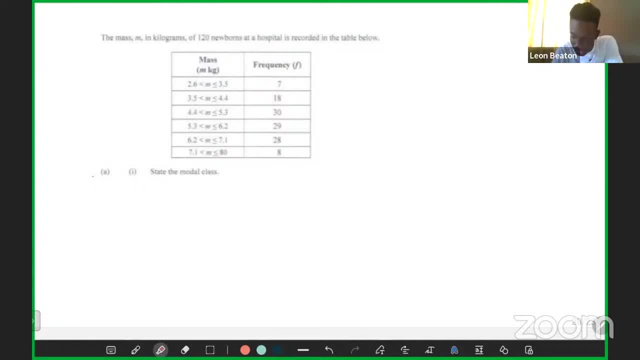 let's see if anybody said it in the chat. yeah, so emmanuel said 4.4, 5.3. yeah, so, yeah, that's the motor class. this would be 4.4, 0.5, 0.6, 5.3. right, nice and easy one mark. 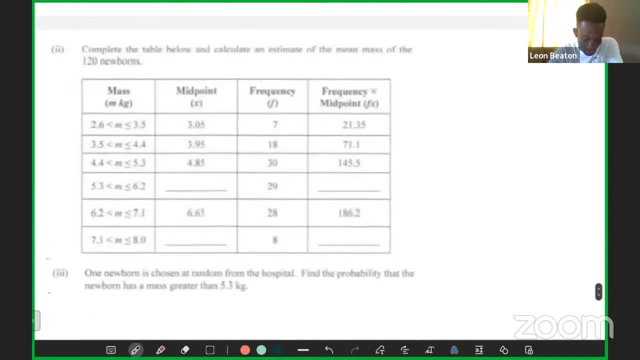 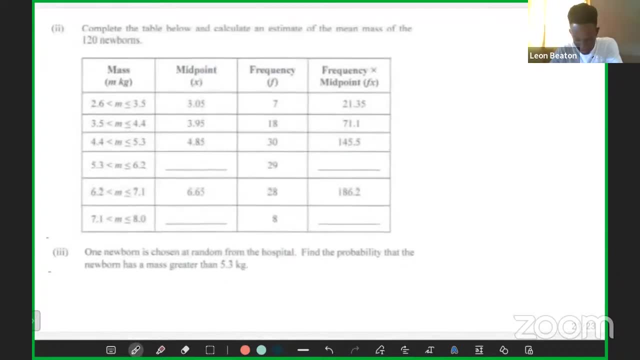 is it what? so? complete the table below. calculate and calculate the estimate mean mass of the 120 newborns. you gotta complete this table, so i will complete it. um, so you don't have time to draw it. so now the thing about these tables. right, what i? what i would encourage courses. 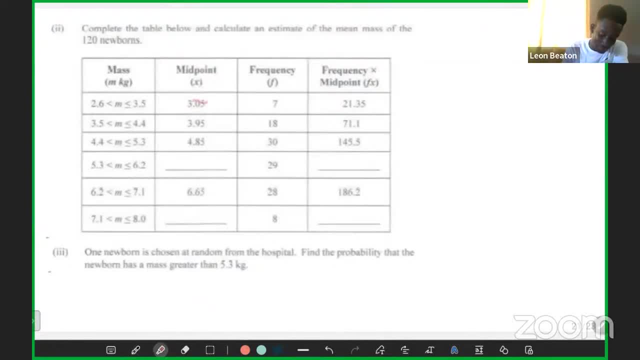 to do um. you see how the code already gave you um. they already give you this answer here. they already gave you the midpoint. here they already give you. you know the frequency times, the midpoint. you know what you can do, what you can do, let's say you can't remember how to find midpoint. 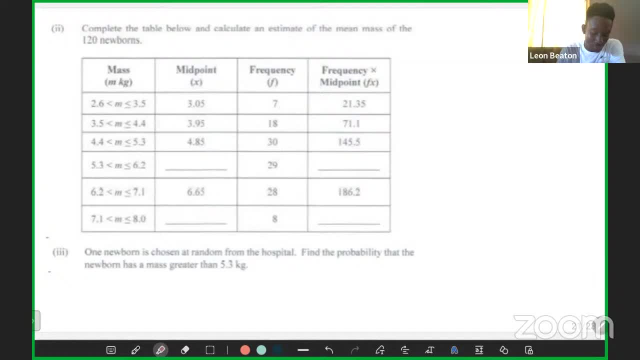 some reason, what you can do: see what, see what they use on the table and see how you can find midpoint from what they did in the table. so what you can do, you can just take these two numbers, or you know, and see if out of them i divide by two, see if you'll get this, and that's how you can. 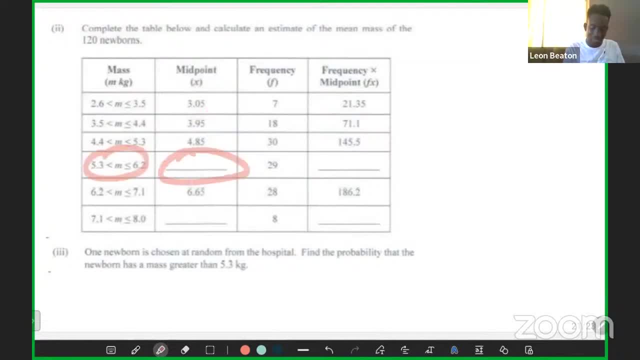 check. and then you, you know you use the same thing and you're playing for this year, all right, so you can check: 2.6 plus 3.5 divided by two, and perhaps you know you have that answer, but that's what you can do. one tip: you know if you're given a table and they already completed. 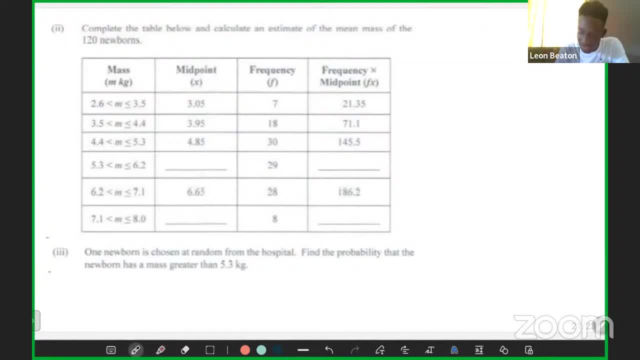 parts of the table. for some reason you can't remember how to work or try to see what they did anyway. so the midpoint for this year would be 5.3 plus this one would be 5.3 plus 6.2, all divided by two, and that will give us a value of 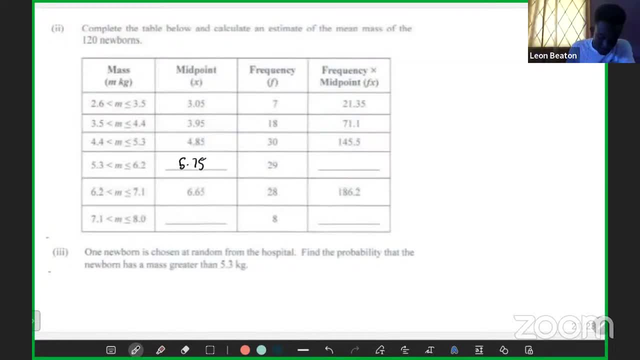 5.75 and the same thing here: 7.1 plus eight divided by two, give us seven point seven point five, five. all right, and then the frequency times, the midpoint, which is fx, so it's basically this number multiplied by this number. so it'll be five point seven, five, five point seven, five multiplied by 29, and 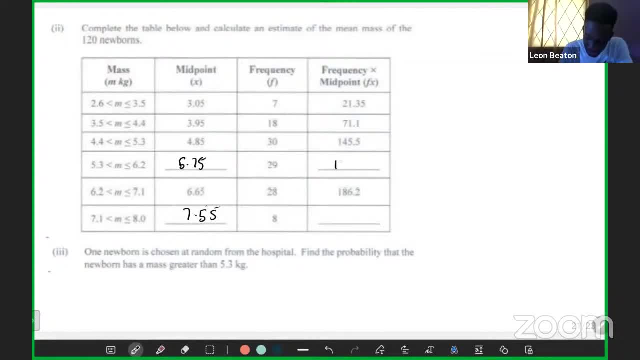 we can see the wrong needed art. so this would be one sixty six point seven, five, and the same thing here: seven point five, five multiplied by eight, that will give us a value of sixty point four. all right, and that is how you complete the table. easy marks, easy, easy give remarks. any complete of. 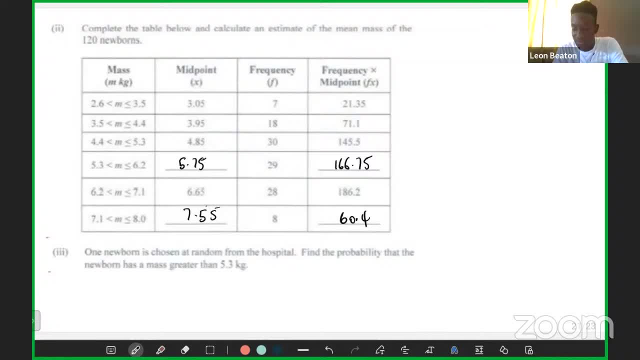 any table, you know you should maximize on the amount of marks for those, all right. maximize on All right. maximizing those marks One second, All right. so that is how you complete that table. The next one says a newborn is chosen at random from the hospital. 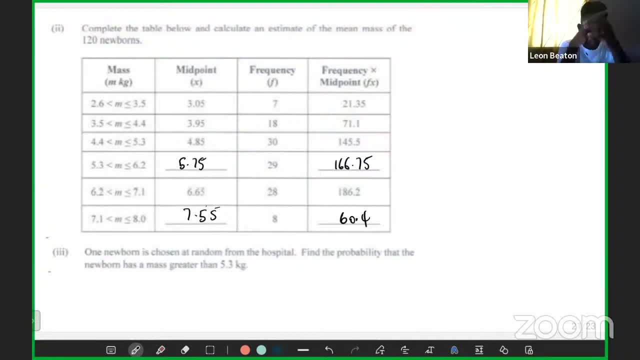 Find the probability that the newborn has a mask greater than 5.3.. Greater than 5.3. 5.3, so we have 5.3 here. We want to find greater than that probability that if we choose a newborn at random, 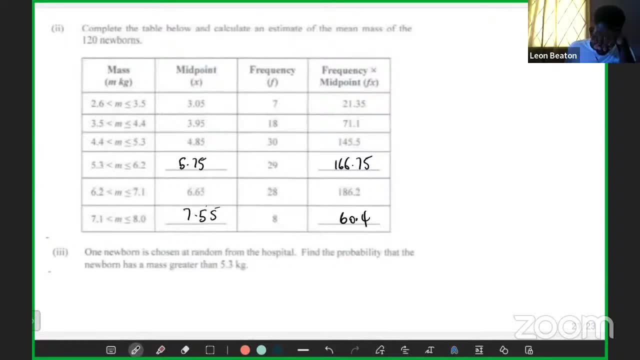 the newborn has a mask greater than 5.3.. So anybody in here? how can we Find that probability? my probability is the total number of favorable outcomes divided by the total number of outcomes. So what can we do there? Anybody here? 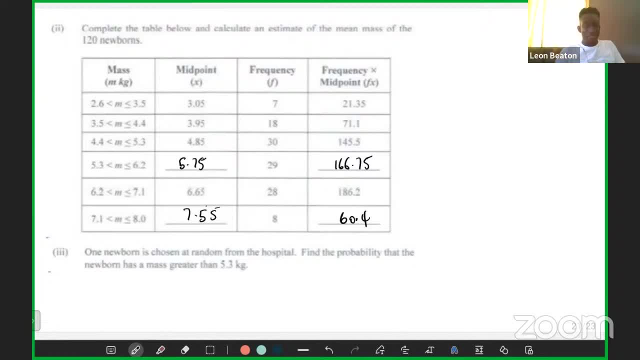 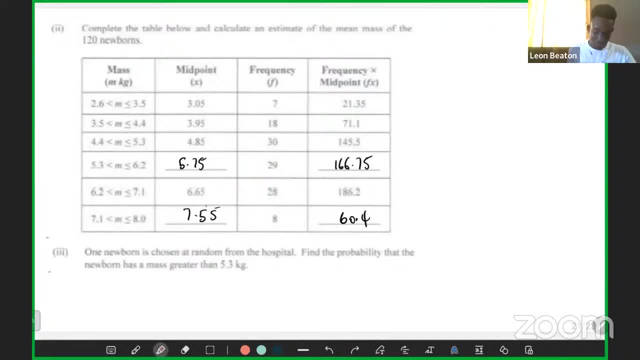 Greater than 5.3.. Greater than 5.3.. All right, so what we add in which set of numbers, Midpoint, times, frequency, Midpoint, Midpoint, will tell you the midway, right, Midway between the thing. 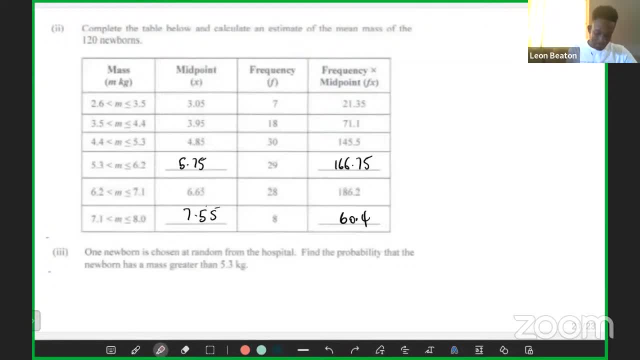 Midpoint times frequency. What does frequency tell you? Midpoint frequency tells you what. sorry, adding the frequency times, midpoint, all right, so you're wrong. the frequency tells you the amount of babies that um fall into the fall into the range, right? so if you want the amount of babies who gain mass greater than 65.3, you? 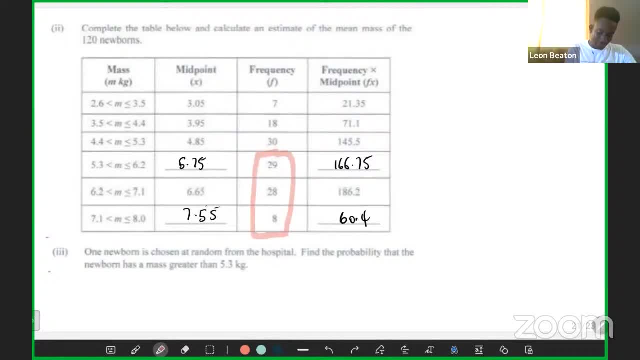 gotta add up all the mass, all the frequency greater than 5.3. so the frequency will give you the amount of babies, right. so you gotta add, as um manual says, 29 plus 28 plus 8.. so to be 29 plus 28 plus 8. 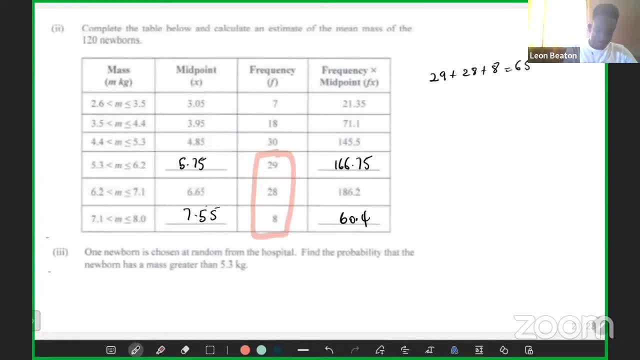 65, right, so it's 65 babies got um mass greater than 5.3. so but we wanna find the probability, so my probability is the total number of favorable outcomes, which is 65 in this case. that is, among two babies we we can pick, and the total number of. 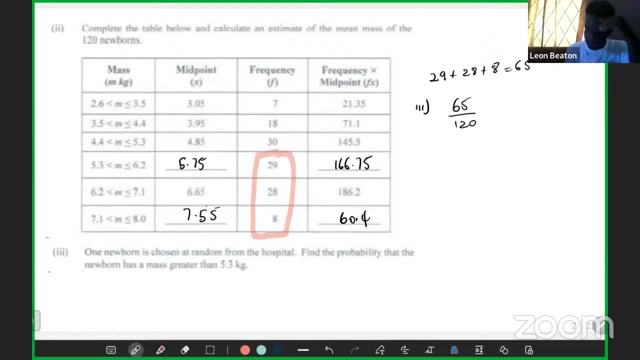 outcomes, which would be to one twenty. so the probability would be: 65 divided by 120 to 65: 120. so you can break this down, i want tobins. so 65, 120, so that's five out of ten, that 120 and two and, uh, 65.. five, five. so five divided by 65 would be 13, 120 divided by five would be. 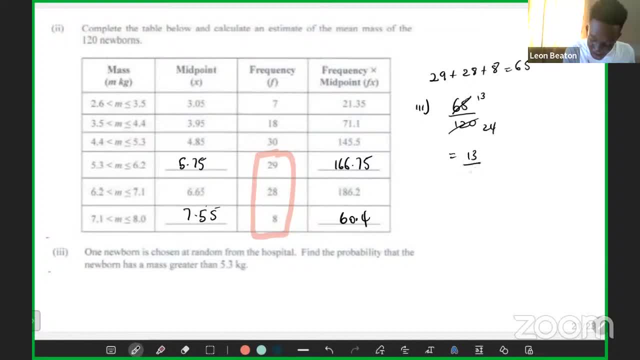 24.. so it'll be 13 over 13 out of 24.. all right, yes, 14 out of 24. so 13 over 24. so 13 divided by 24, it'll be 0.542. but you can leave it as a fraction, you know it looks nicer. so, talking about the, 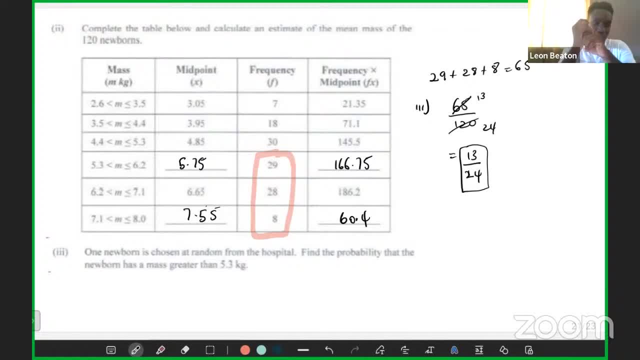 probability is 13 out of 24. but if you choose a baby at random, the baby has mass greater than 5.3. the probability of choosing a baby at random, the probability of choosing a baby at random with mass greater than three- 5.3, is 13- 24- 13 out of 24 over 24.. 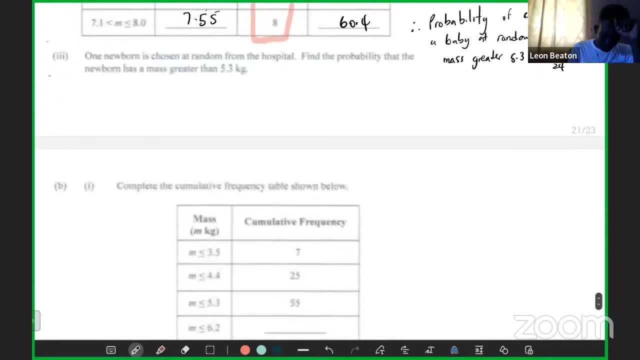 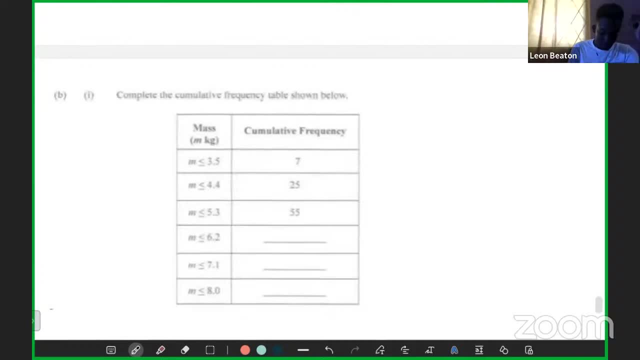 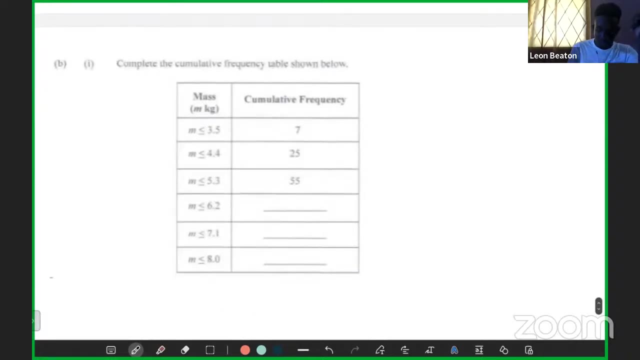 all right, so that's it for that one. so, last but not least, well, for this part, complete the cumulative frequency table. cumulative, hey here. the word cumulative means you keep adding on cumulative. when something accumulates, it keeps adding and building, and building, and building. so for the cumulative frequency table. 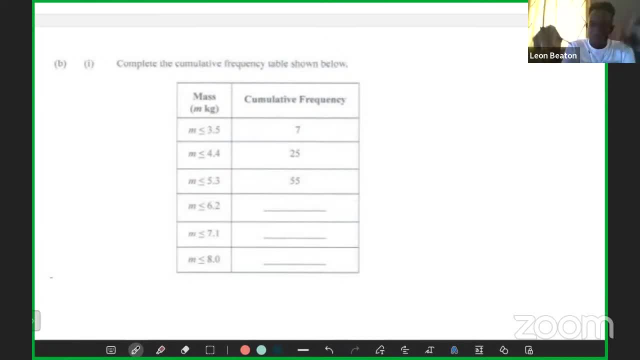 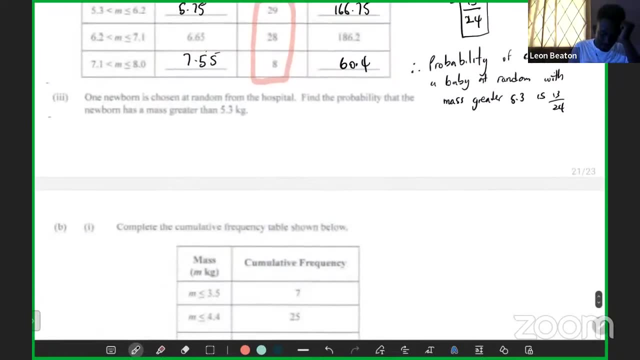 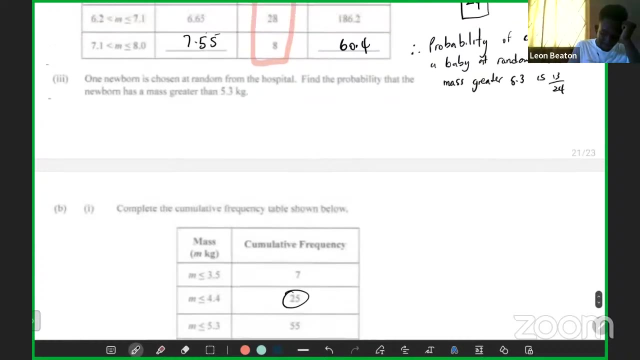 you keep adding from the previous number. so this would be 7 plus 126, and that's it for the cumulative frequency table. so be 7 plus 18, I'll give you 25. and it would be 25 plus 30, I'll give you 55. 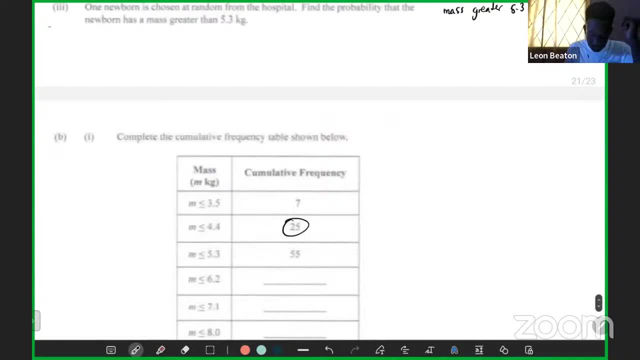 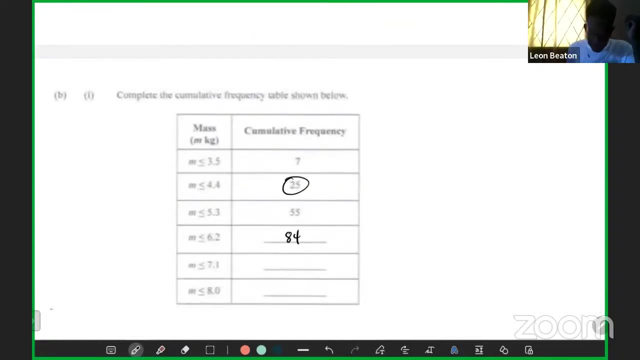 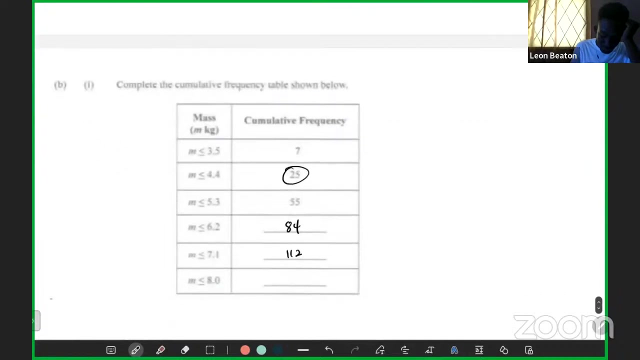 that would be 55 plus 29. 55 plus 29 would give you 84, then it would be 84 plus 28, 112, and it'll be 112 plus 8, which will give you 120. and at the end of, at the end of holidays, you should get, at the end of all this, you should get. 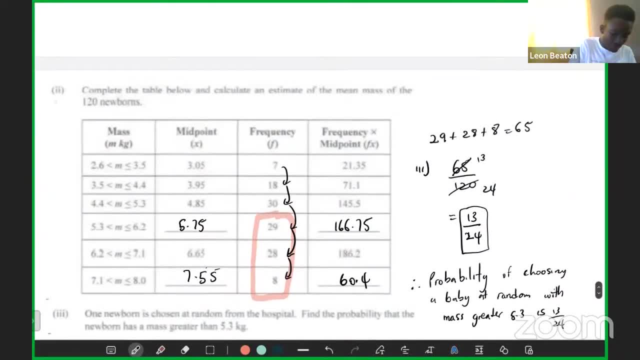 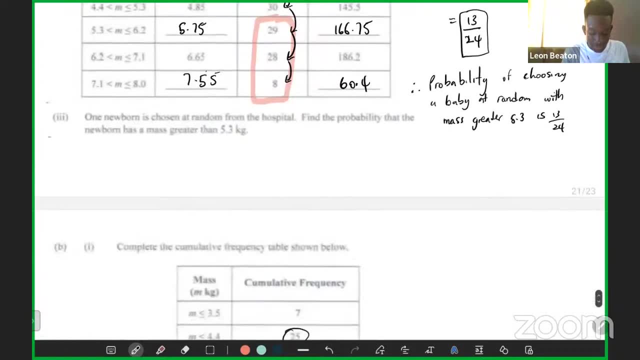 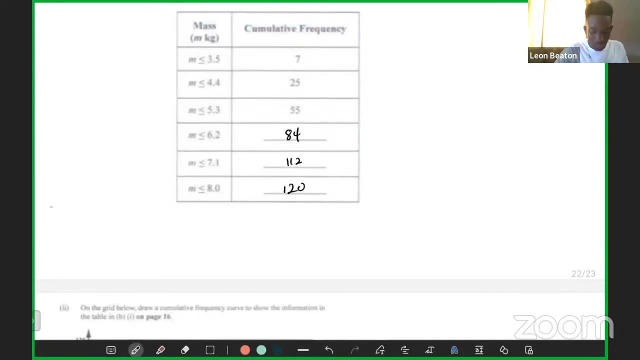 the total number. they have your 120 new barn. so you should get 120 out of all the cumulative. when you you we should find a number in the cumulative frequency. all right, you should get 120. that is how you complete that beautiful table. you're nice and easy marks. 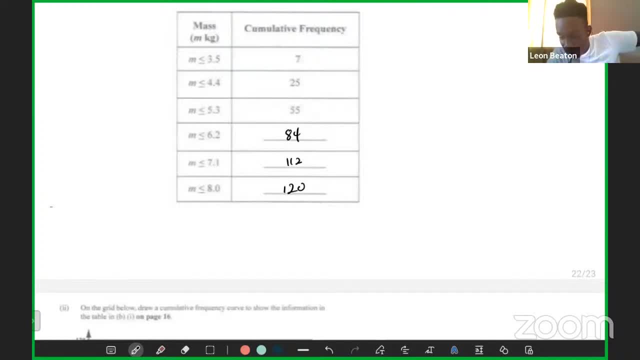 anybody good here? yes, sir, like you're blowing, my blowing. what is marathon? yeah, anybody blowing. who blowing who out of breath? who is out of breath? sharp me, who's that? you're out of breath, sir. i'm hungry, hungry. oh, you want to come this marathon without eating man. 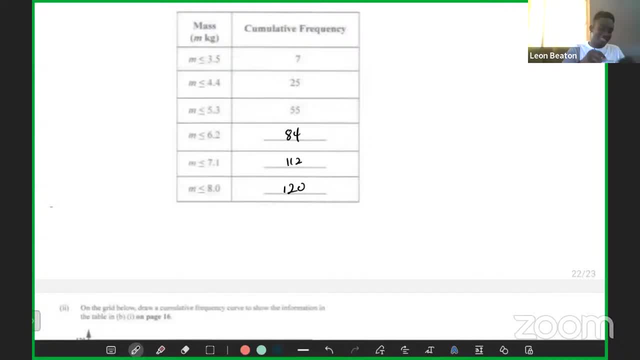 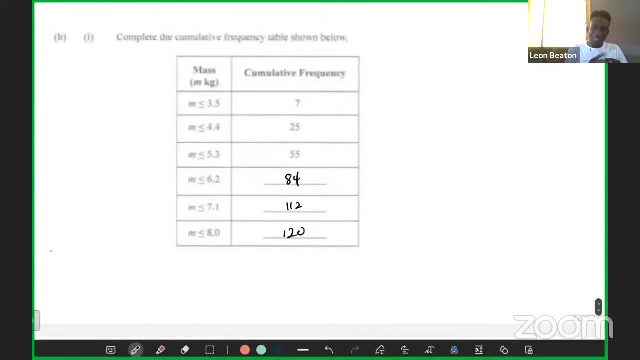 oh, let's come to this marathon without eating, all right. so let's see, i think you got one more. oh, there's a lot. we're on the last page, so this is the last one. all right, and we'll we'll if you stop. all right, we'll stop here. you'll stop here since, well, after this last one, and then 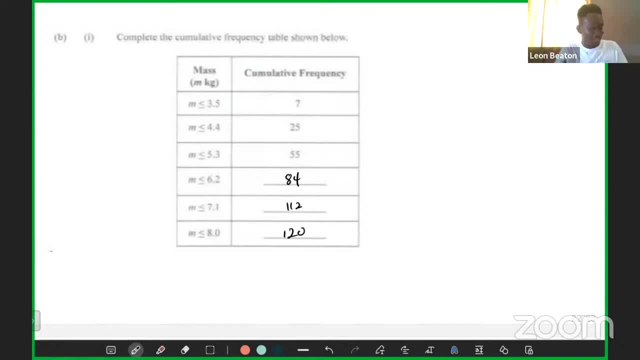 next time when i come to this marathon, i'll try and eat something. who else, who else? who else blowing and and and tired, i see, hey, sir, see all these forces that told me sorry i'm making till three o'clock, so far the more so you can go till night time, as we can stay. we got to work. 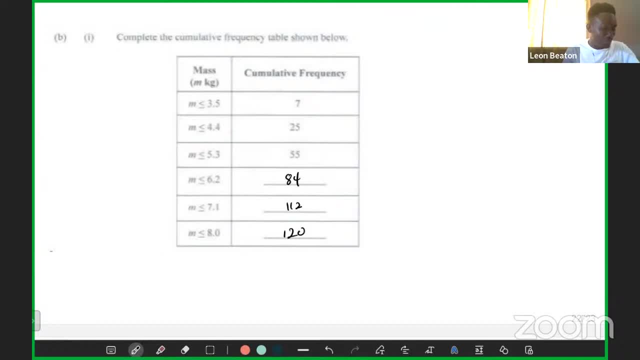 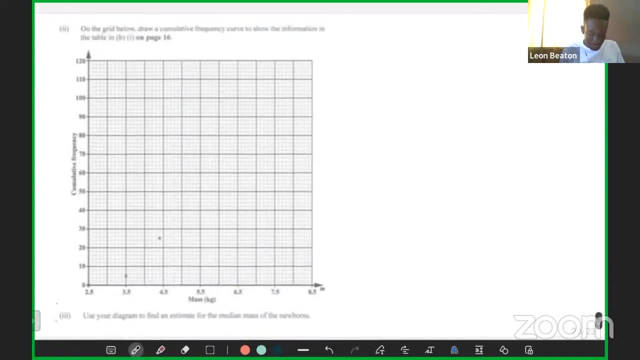 yeah, yeah, like these people that would run these races, you start up at the forest lap full pace and power, and by the second lap you start holding back. all right, let's go last one, so, if you want. um, we actually made it to the last question, so let's see. 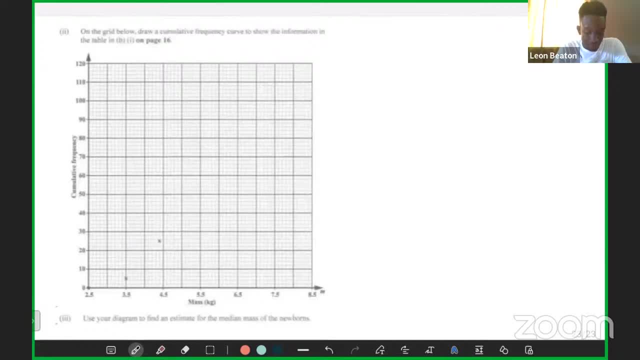 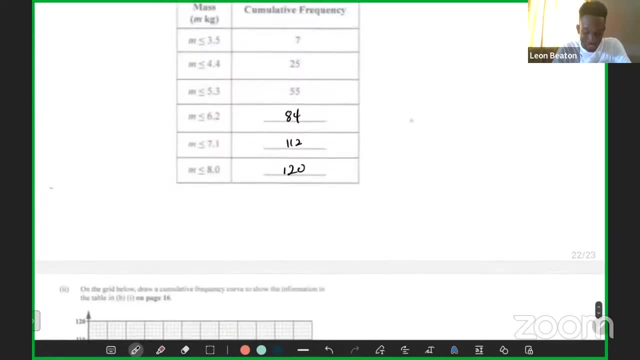 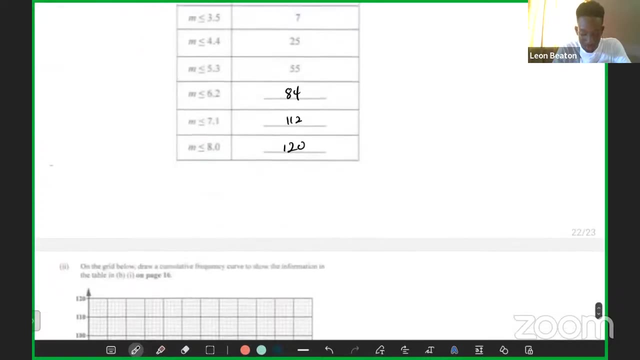 so on the grid um, draw the cumulative frequency curve to show the information in table bi, which is a. this is this one that we did here. so using the upper limit is the upper limit to use. yeah, we're using the upper limit and the cumulative frequency to to plot this cumulative. 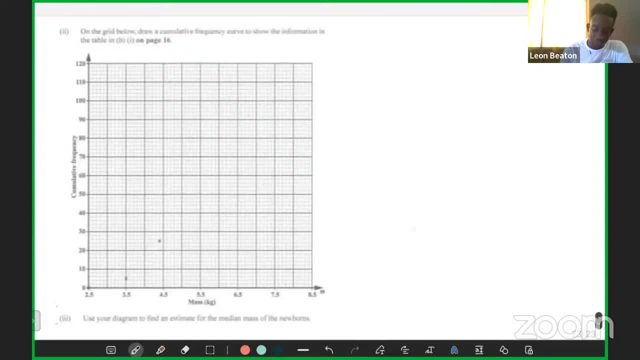 frequency curve. so when you plot a cumulative frequency curve, it should come like this: all right, it should come something like this: all right. that's why i plot it. so if you plot a car for your car or something, if your car looks something like this: let me see, your car looks something like: 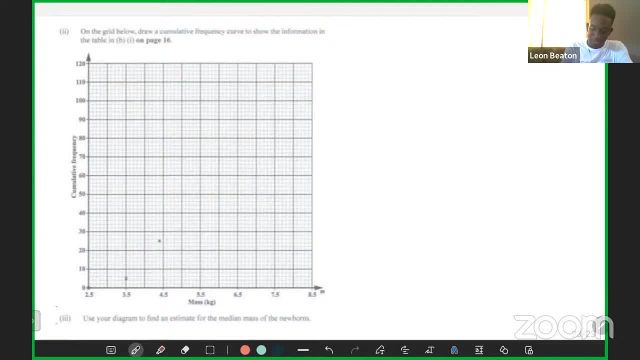 something like that, or your car looks something like that. that means it did something wrong. right. cumulative frequency it should. it should continue going up and up right. it should look something like an s like that. that's how it should look. look anything different. it means deal something around with the core. all right, so let's go so. 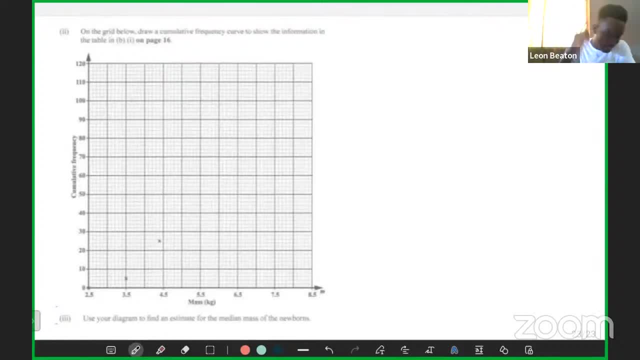 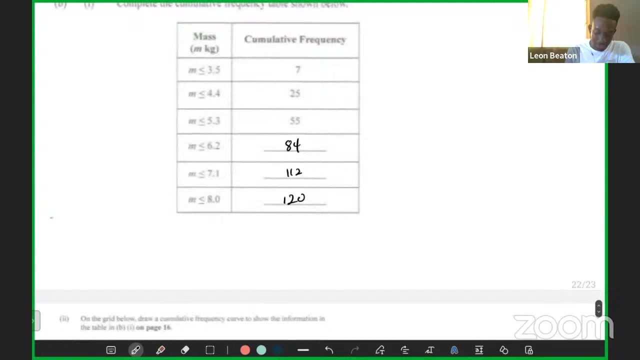 you see, the thing is: watch out, cx, nice man, they even, they even flooded the forestry for you. they flooded the forestry for you here, here and here. you know you're so generous, so next you gotta plot is the 6.2 and the eight four. so you go six, point two: 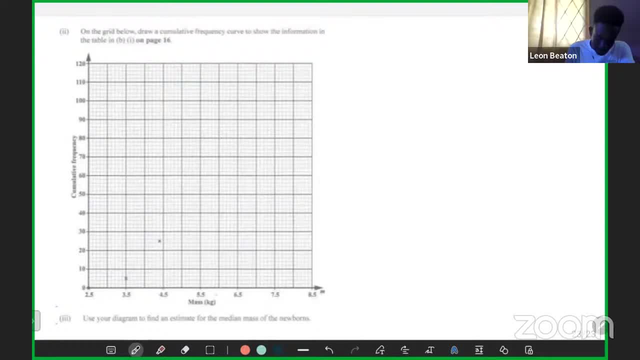 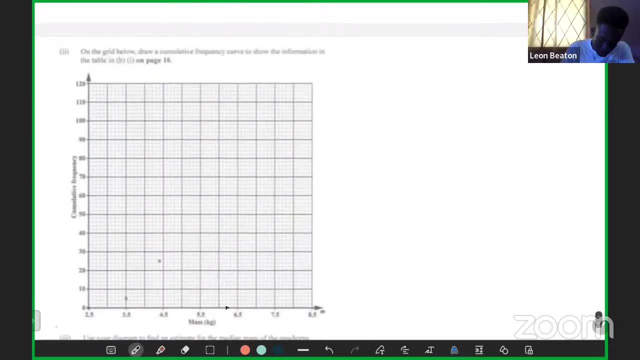 see, here it's five point five, i guess, here it'd be six. so six point two would be here, and we gotta go up eight to four times. so we go straight up to it: the 80, eight, two, eight, four. so eight, four would be here. all right, 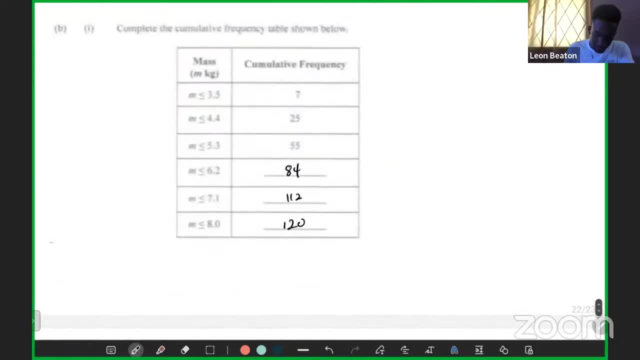 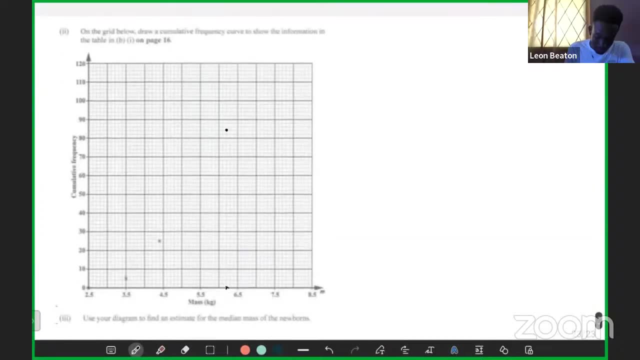 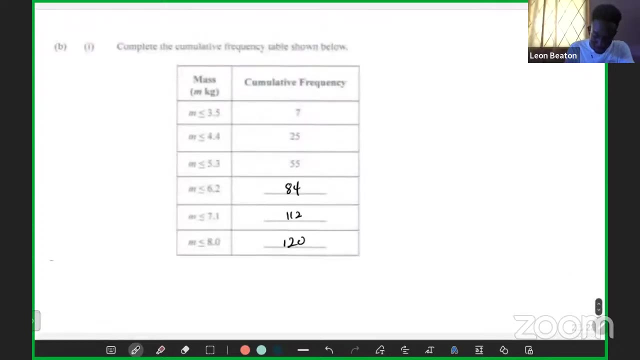 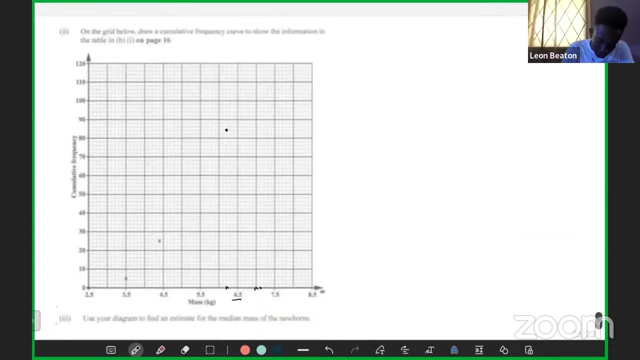 yeah, and then the next one. we go across 7.1 times and we go up one twelve. so seven point one. so here is six point five, here would be seven, seven point one would be here, and then we go up one twenty times one, twenty one, twenty one, twelve, sorry, one twelve. so here is a hundred. 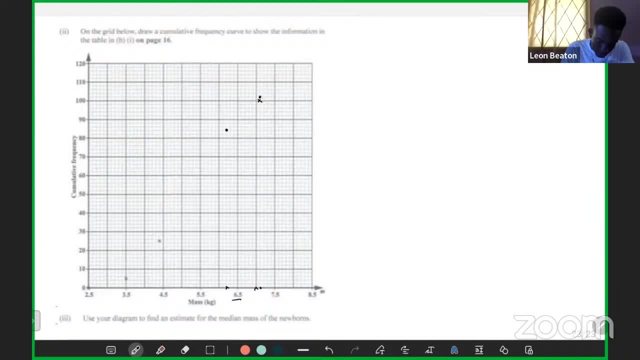 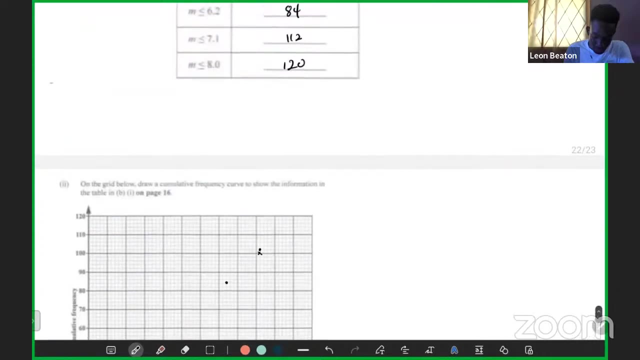 so one twelve would be a right above the hundred, since you're counting in twos, two, four, six, eight, ten. all right, two, four, six, eight, ten, yeah, last one, 120, so it would be eight, all the way up to 120. so it is, if here is 7.5, here it'd be eight. 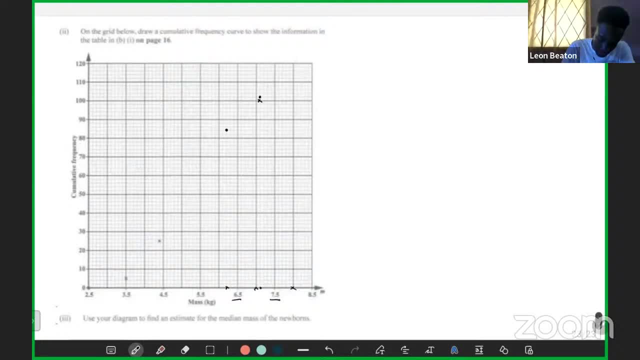 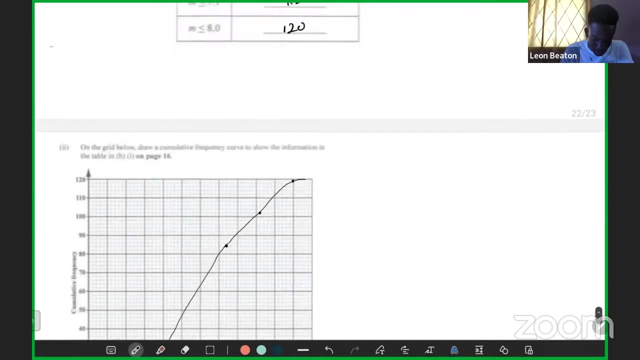 and we go all the way up to 120. so 120 would be right here. so let me connect now see where s will come. it's nice. yes, let me use this last piece, so you put the second to last point from i did. let me see eight. oh, they're supposed to be one twelve. yeah, one twelve. and what did i plot? 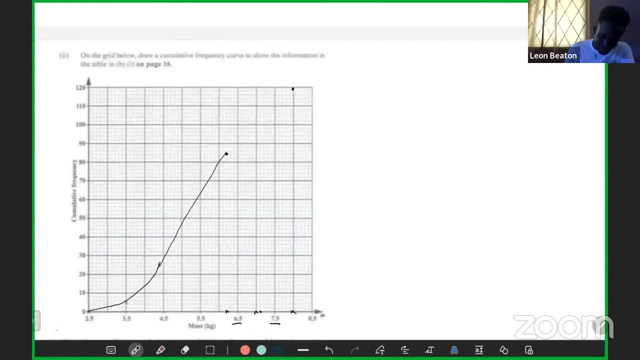 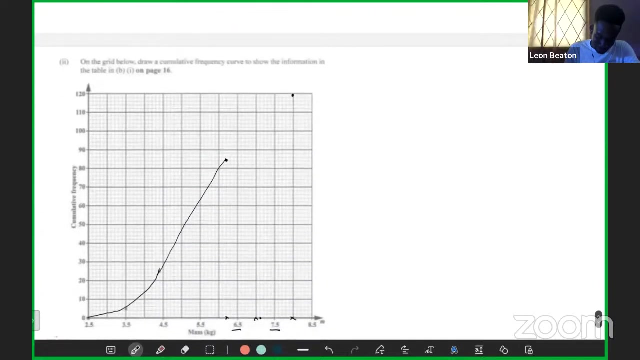 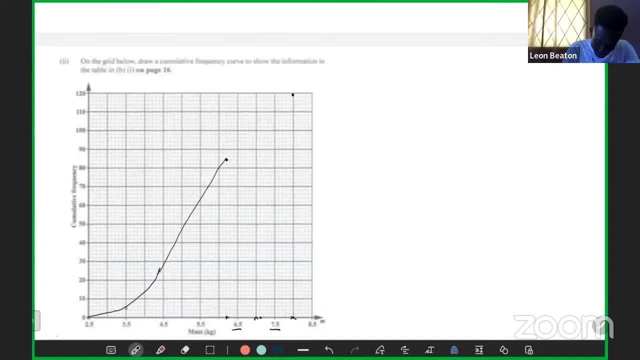 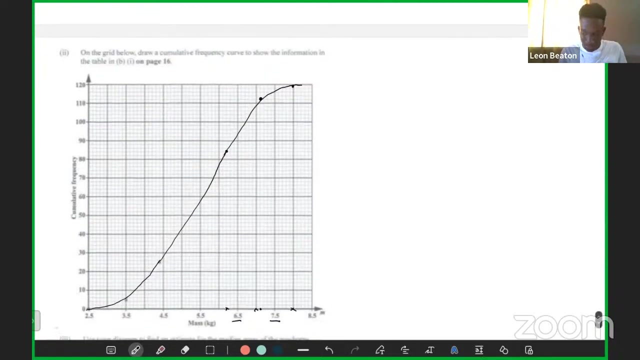 so this is one ten, so here would be, here would be it, right. so let me connect now, then i can go until, um, you said: the curves look nice now. yeah, so indeed, we plotted it wrong. all right, so that is it for that. um, i think this will probably go for about two to three marks. 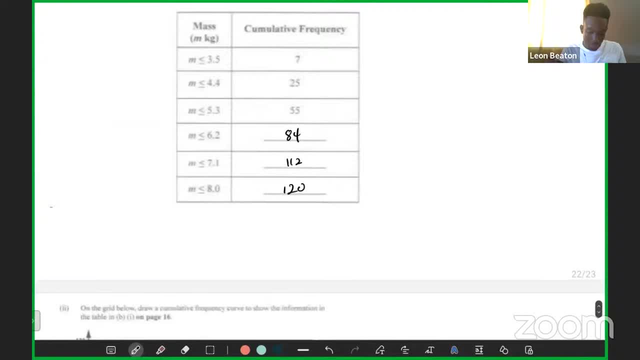 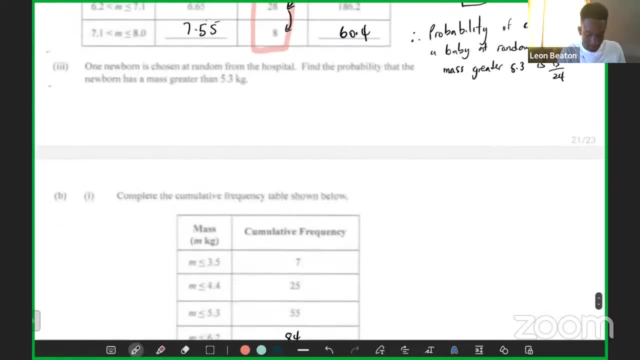 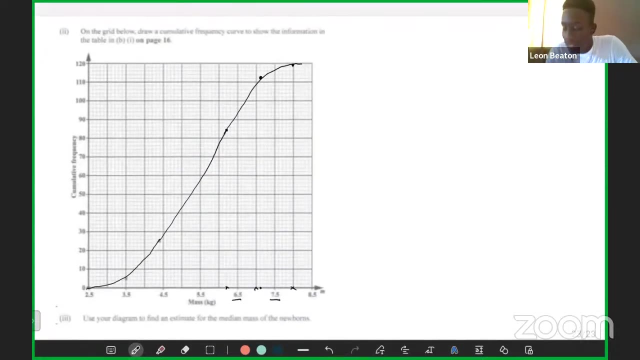 so we want to ensure you plot your diagram correct. use the upper limit and the cumulative frequency to plot it all right. and that is that everybody go there, everybody going in the chat, the people i'm see you, anybody in the chat state from starting in the middle, and then i know, uh, let me see i, you know, let's see the name. let me see the name. i don't. 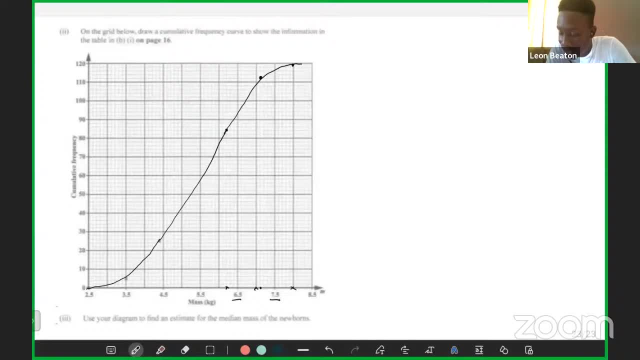 know who's the individual, nicola, and who's the other person, emmanuel, all those persons who are in since the beginning, and few people drop in anyways. so that brings us to the end of our, our marathon. um students indicated that you know they're buckling.